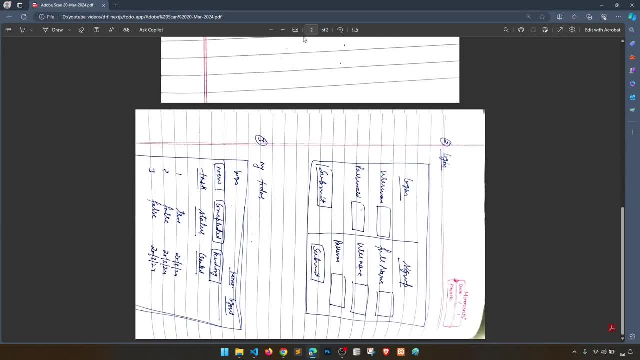 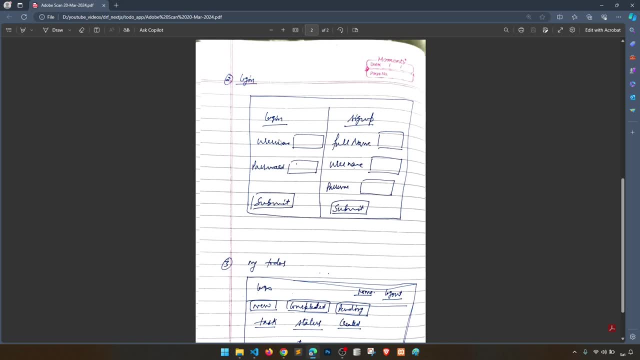 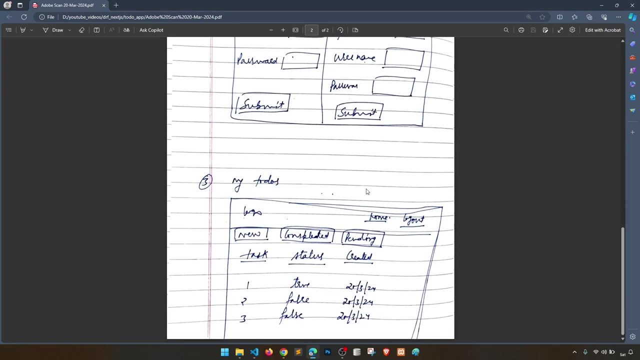 Right And in the second page I have created a two page Right. So in the second page, not second page- we have a three pages total. So in the second page we have a login and in the login we have a login and sign up. And here you can see that in the login and sign up username password and sign up full name, username password Correct And then after login, user can see the to-dos Right Header will be same and then task list Right, Status: true, false. Obviously we will show the checkbox and create a date Right And here we will add a filter: new, completed, pending. 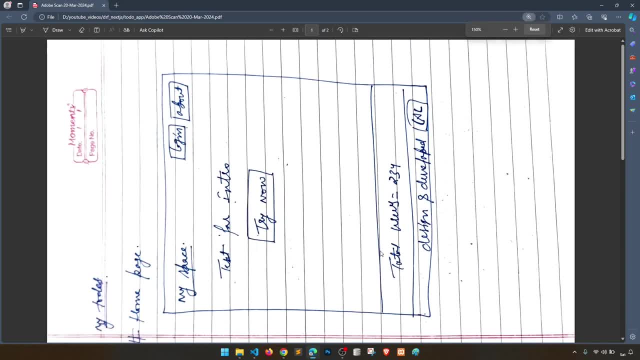 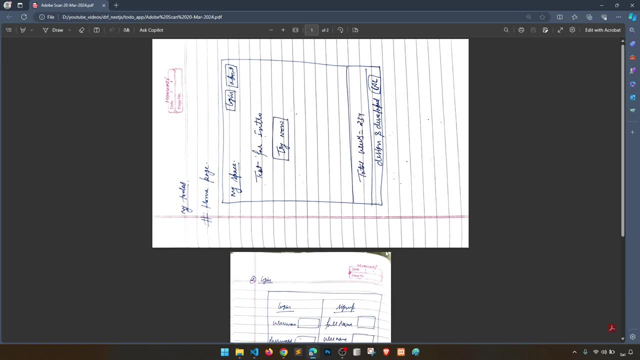 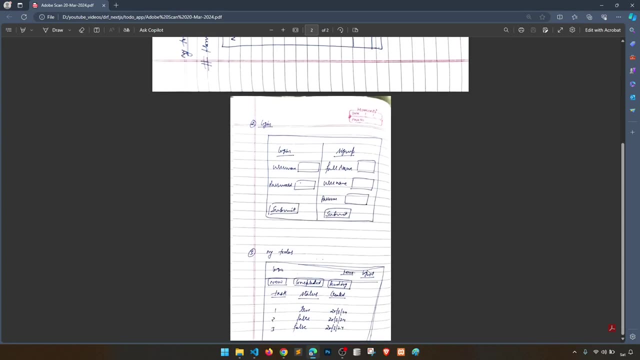 Right. So in this small project we will try to explore the Nextjs and a Rest Framework. One more thing that we will add in this project: we will add a token authentication Right. So when user login from the or sign up from the Nextjs app, we will create a token when sign up and then we will authenticate when login, Right. 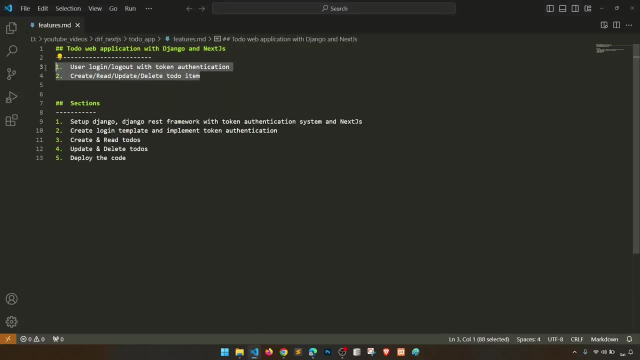 So these are the simple features, two things: login, logout with token authentication, create, read, update, delete to do item right, and these are the sections that we are going to create, or you can say these are the uh, uh, you can say time frame that we are going to create for this video. so setup: the first thing is setup and then 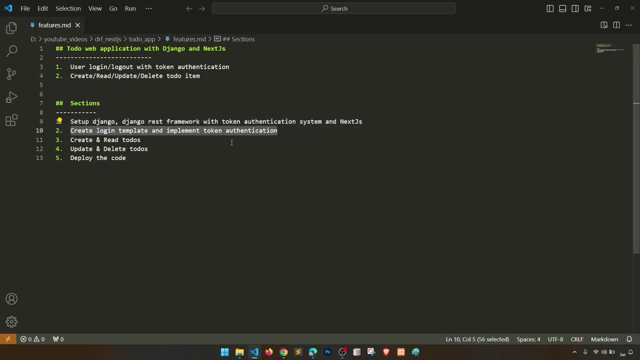 we will create a template log, login and authenticate with the token authentication: create and read to do, update and delete to do, and deploy the code on the server right, like we did in the clinic management system. okay, so i hope, uh, you have an idea that what we are going to create. 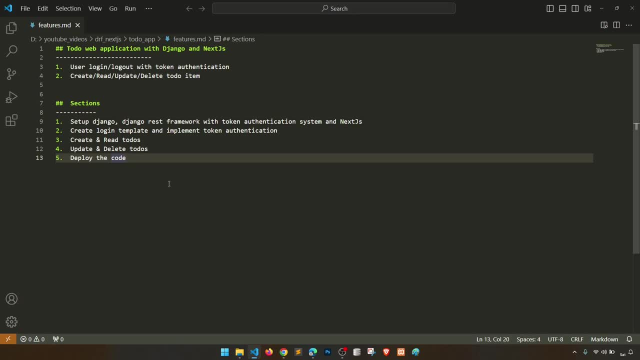 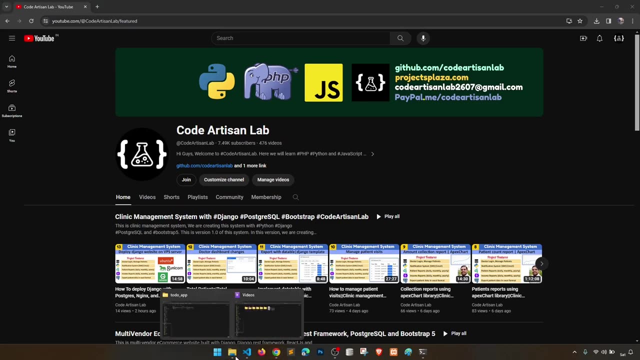 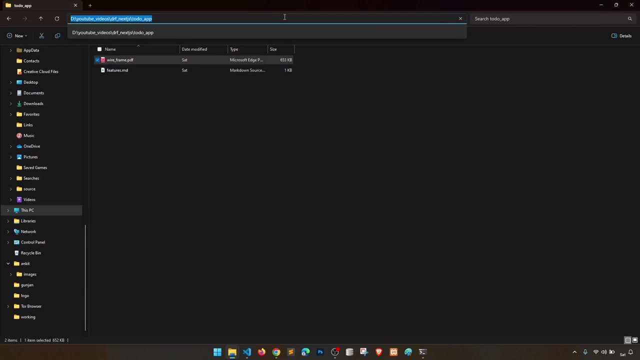 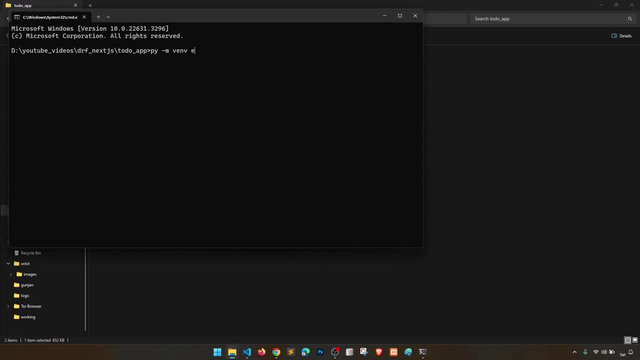 so i think, without uh wasting any time, uh, let's jump into the project and let's get started. okay, so let's start to set up the front-end and back-end system for this project, right? so what i will do, you I will do. let's go to cmd in the to-do app and then py minus m vnv in, right, so this is our. 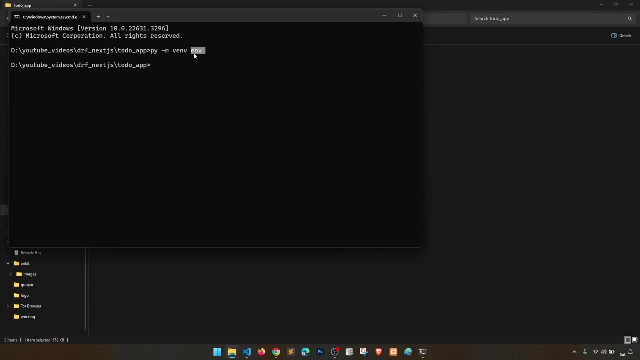 environment name right. and why we need this? because we want to isolate our project so it will not conflict with the versions of django or python or anything, right? so we have this. now we will activate this virtual environment. so script slash activate. so this command is different. depends this command differ from: 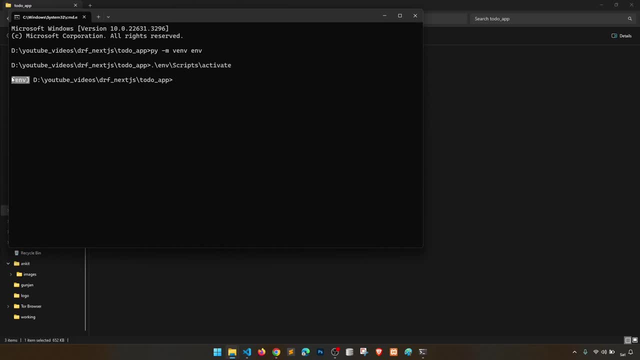 according to the operating system, right? so now you can see here the environment name. now let's create the back-end system, right? so first of all, pip install. now, whatever is we install, we will install in our, in this environment, in this virtual environment. so, pip install django, so it will install the latest version of the django. so, and we will use the uh. 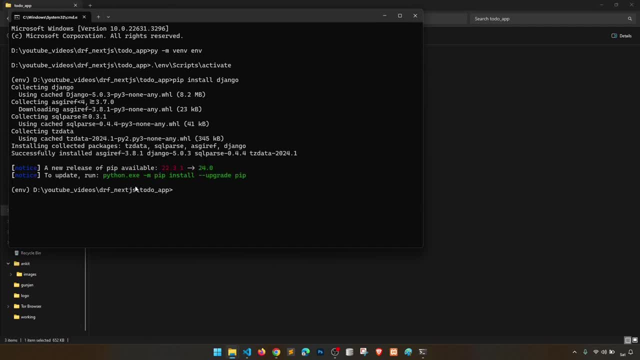 simple uh sqlite, right. so we will not use any kind of uh postgresql, uh big database because, uh, our main focus is to uh api and the next js, and this is small project, so i'm going to use the sqlite which is by default comes with the django right. so to do app and we install django now. 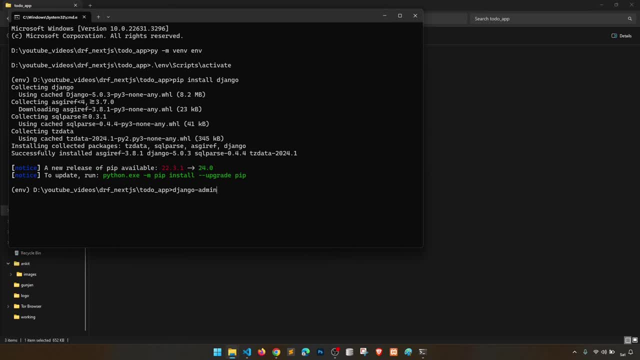 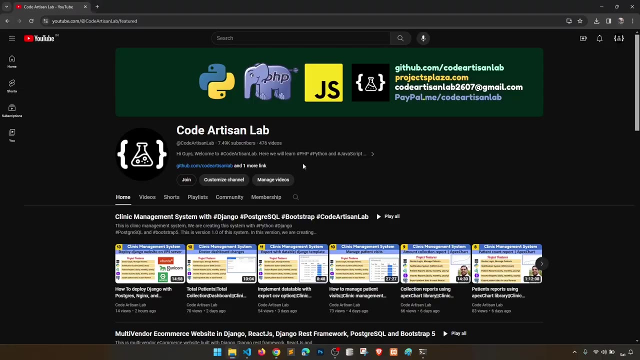 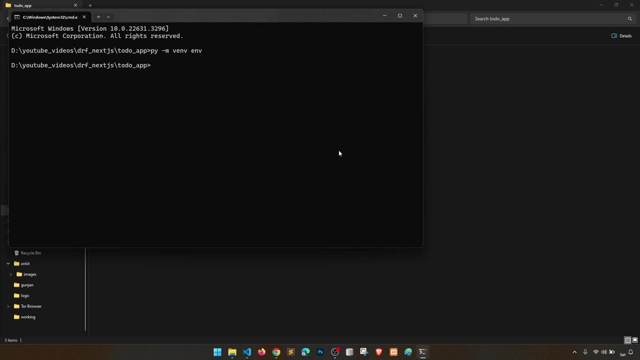 when we once install django, we can run the command django start project and the project name is to do, correct? uh, actually we did wrong thing. we no need to create to do because we are already in the to do what we need to do. uh, we will do. oh, where where are we? okay, now, here we will say backend, correct? so backend, right now we have. 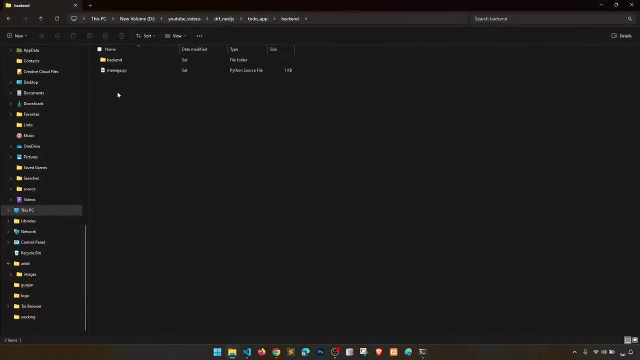 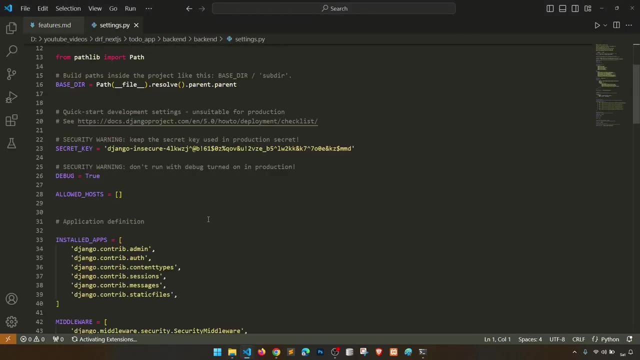 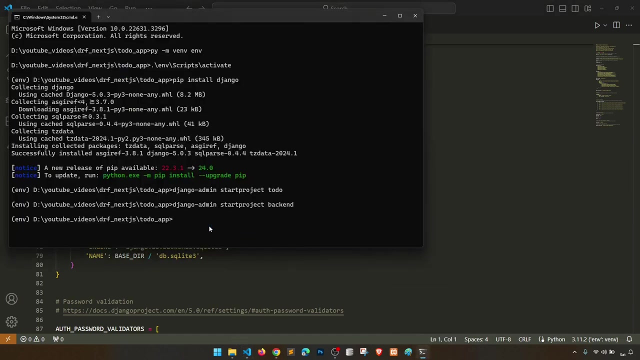 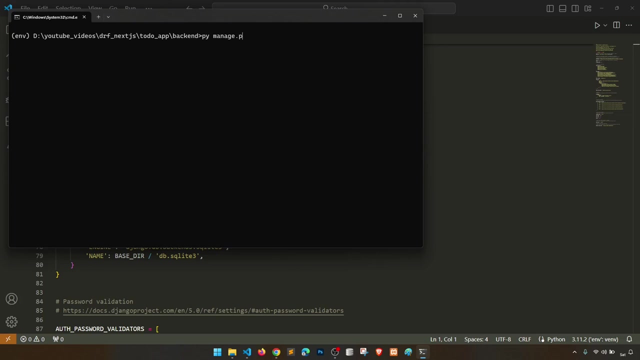 backend, let's go to here and the backend and the settings right. so here we have a settings and you can see, here we have a default database, sqlite, and when we run the migration, so let's go to in the project right, and then run the managepy, make migrations. 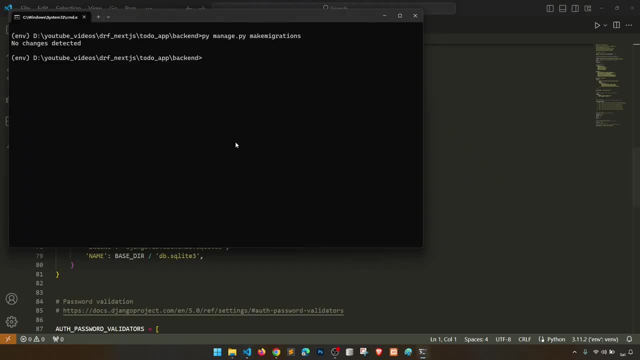 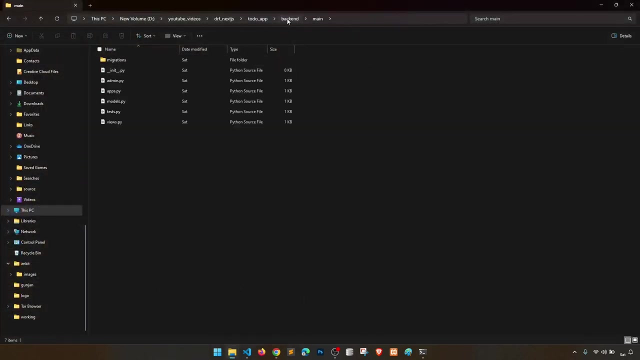 oh, we need to create an app and then we need to install that app. okay, so let's create the app. so, py, managepy, uh, start app. uh, let's say main, right, so this will create the uh application here. this is main and this is the app. right, and we need to. 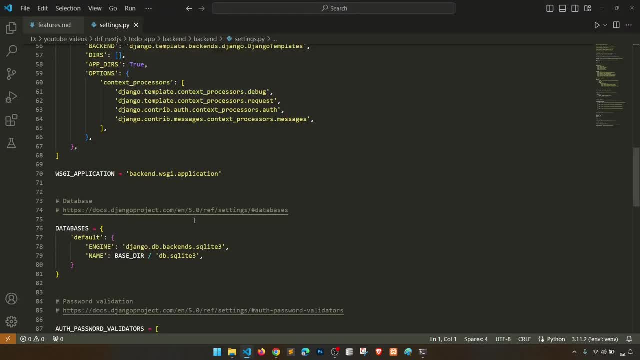 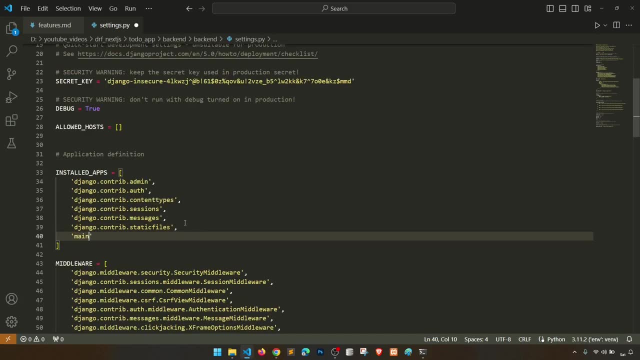 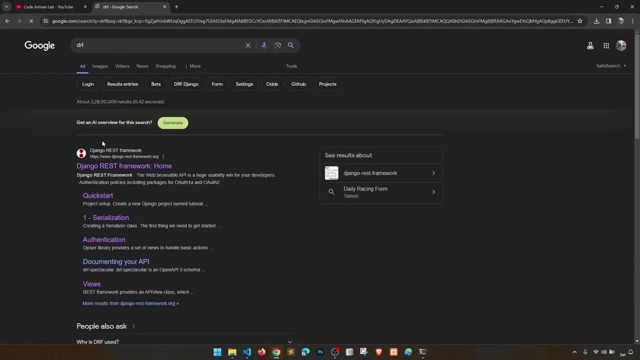 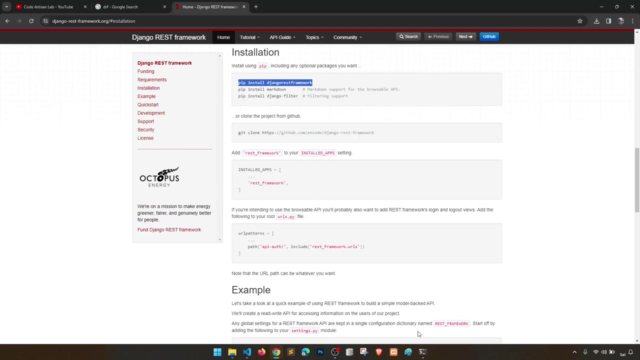 uh, install this app in the project level setting right. so we're here um, here installed apps. i will say main and then let's install one more thing: django rest framework. so we will say drf, jango rest framework installation. so here you can see jango rest framework. so pip install. 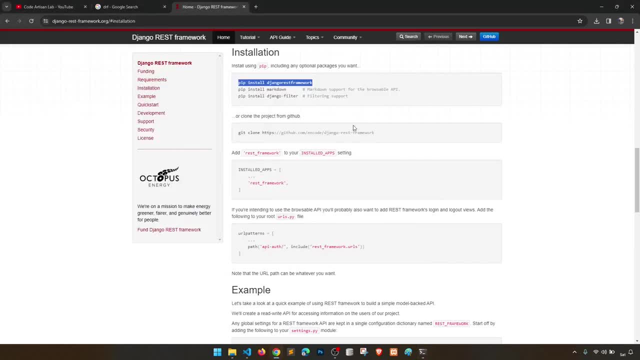 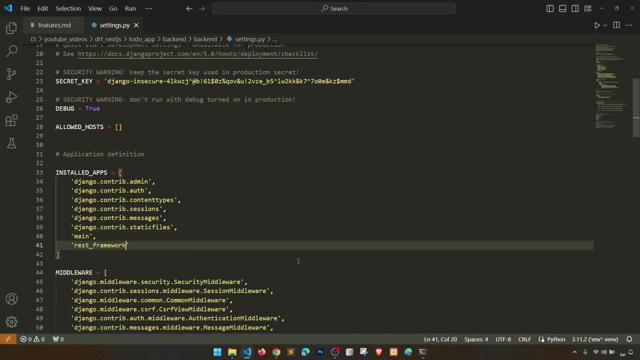 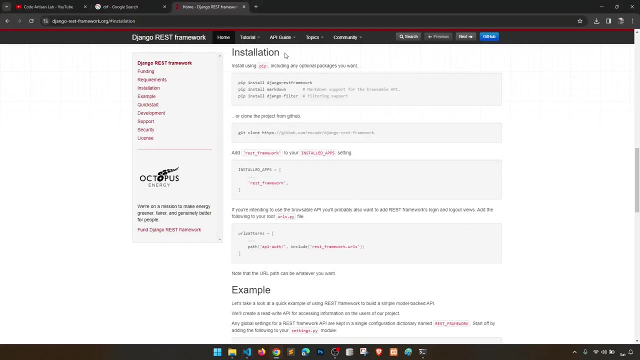 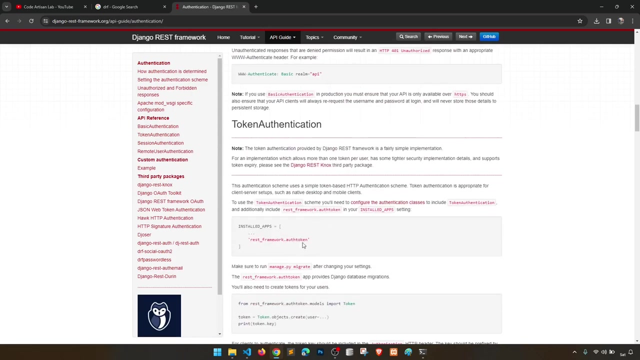 jango rest framework. correct. now. we need to add this in the installed apps, correct. so here, correct now what we need to do. we are going to implement the token authentication, so what we need to do here we have authentication and when we see the token authentication, this is we need to add this in this rest framework, correct. 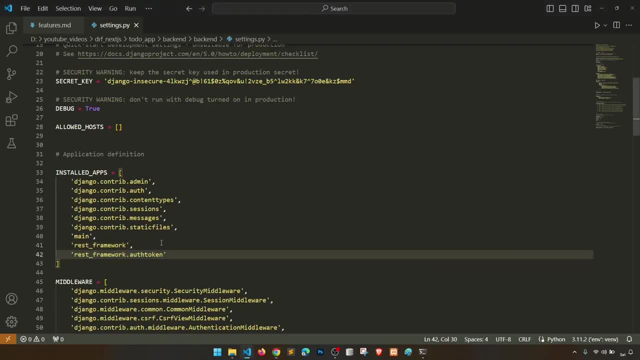 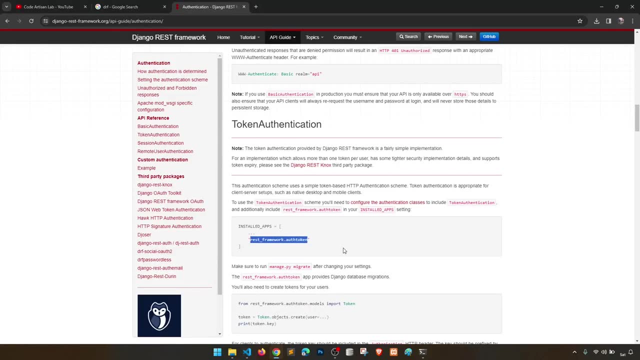 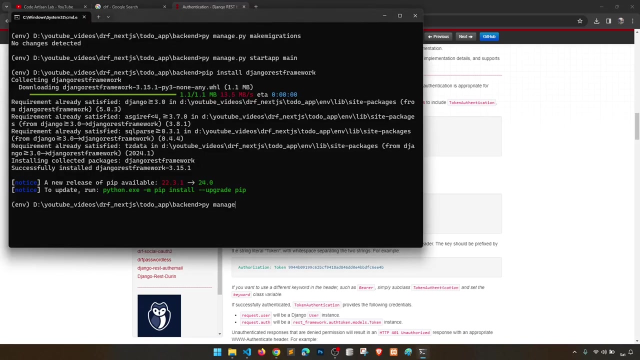 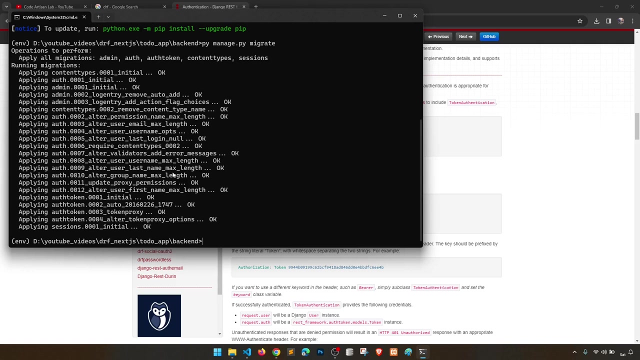 so what it will do? it will create the token corresponding to the user, right, okay? so let's create. let's migrate, right so py, manage dot py. so let's create, let's migrate. right so, py, manage dot, py migrate. okay, so now we have this one. now let's create one more thing: manage dot py. create super user. 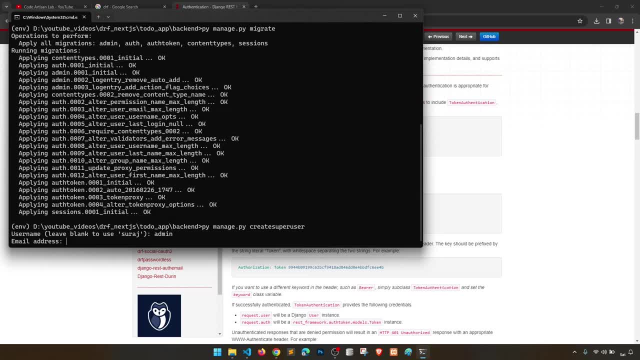 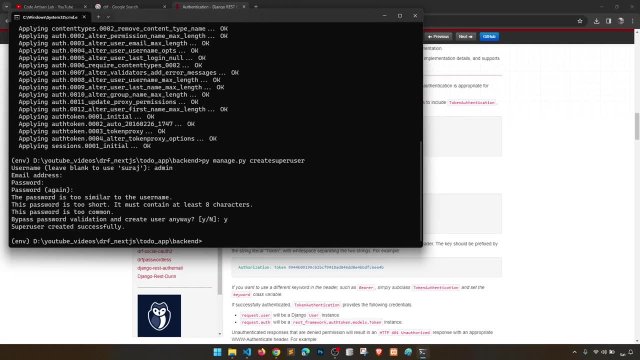 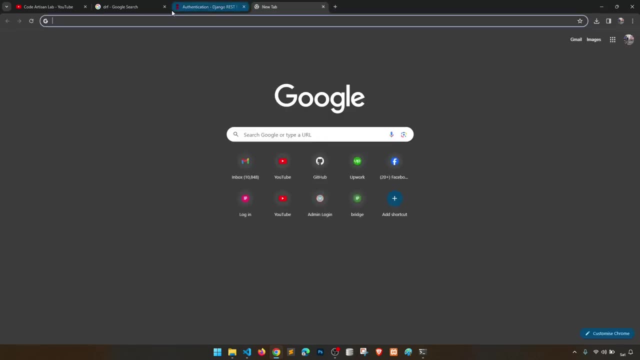 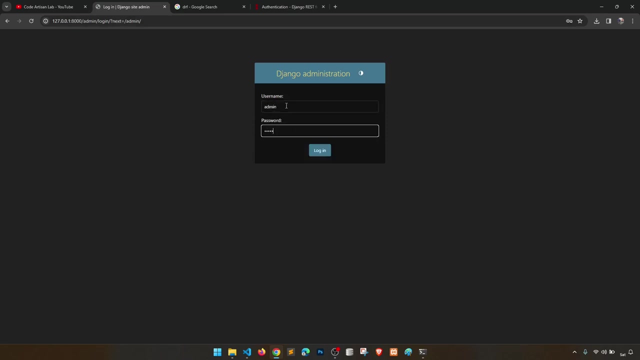 super user is like admin, right, this is one of my favorite thing in jango, right. and then this one: okay, now let's run the server. so server is running, let's run this. here we are okay. now put the passcodes. okay. here you can see we. 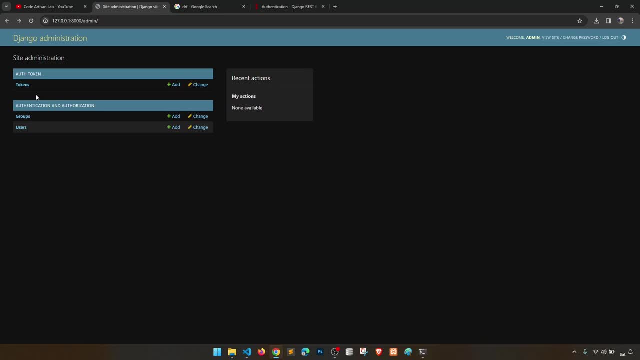 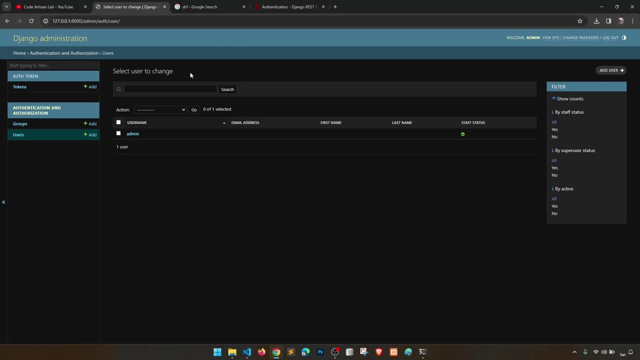 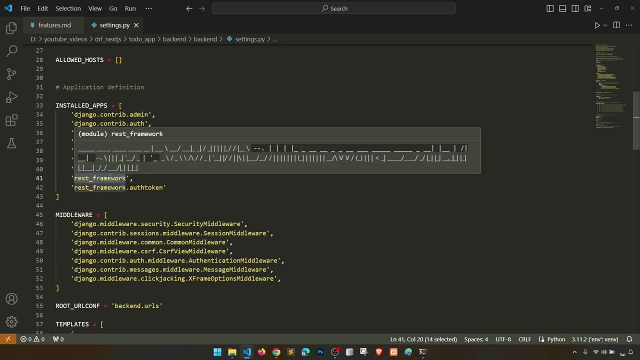 have a tokens right, so it will corresponding to every user right. so we will see that later, but currently we are focusing on how we can set up the things correct. so our admin is set up. now we need to set up the rest framework right. so we have already added in our installed apps. correct now. 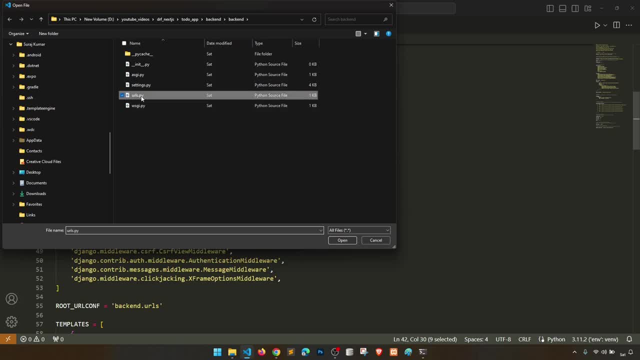 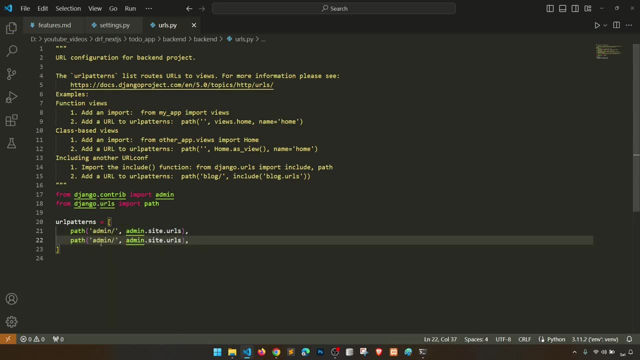 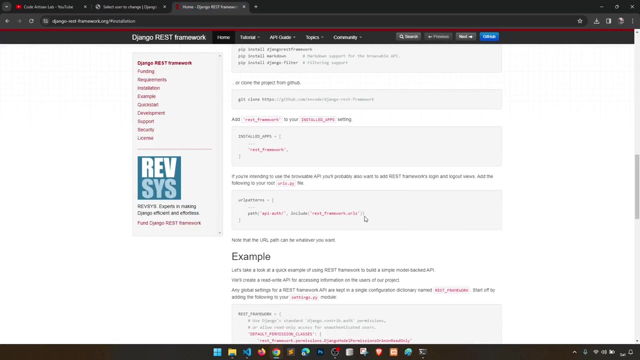 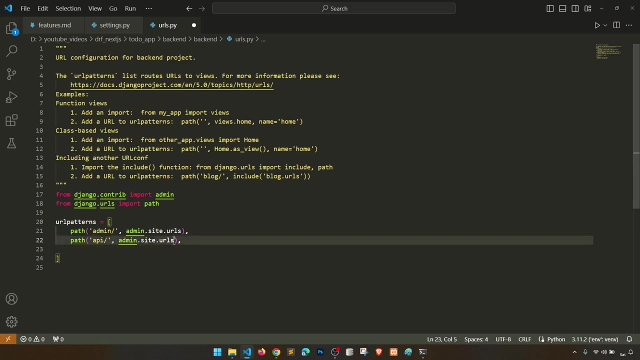 we need to add. let's open our URL, start py file- this is project level URL- and create here, let's say, API, correct. and then let's do one thing. now let's include this one, right? so rest framework framework urls- correct. so here we have rest framework urls and we will import this include. 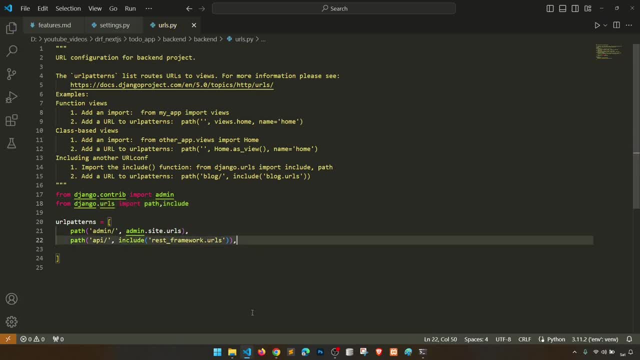 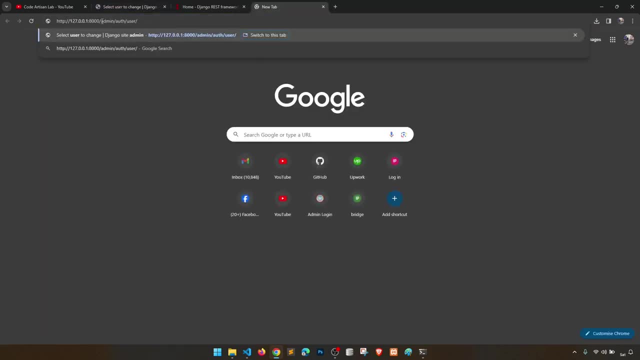 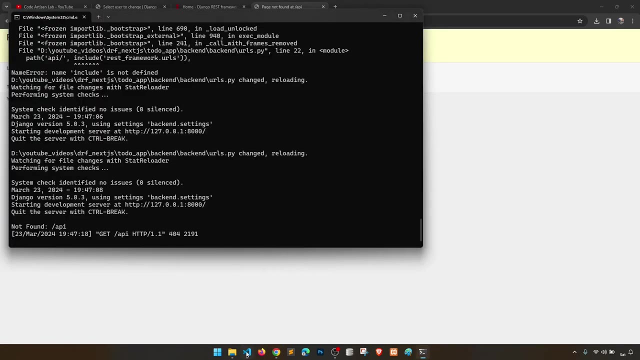 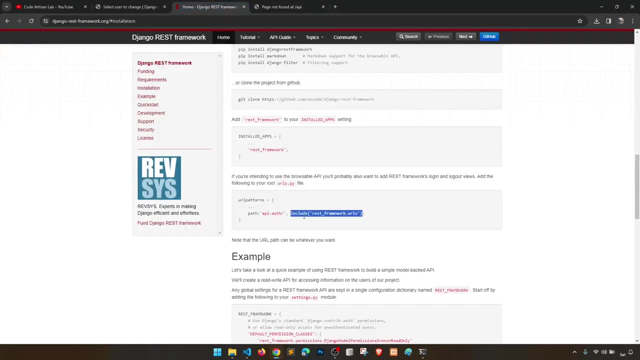 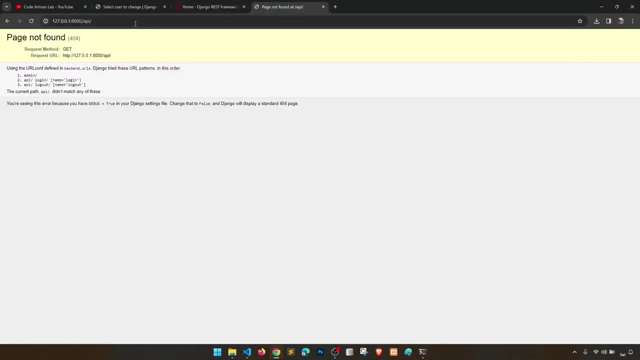 module from the urls right now, whenever we server is running. yes, server is running. so if we copy this and say that API correct, so it is showing nothing, include rest framework urls, it should show: let's go here, that has framework and this is correct and this is also correct. so API admin. 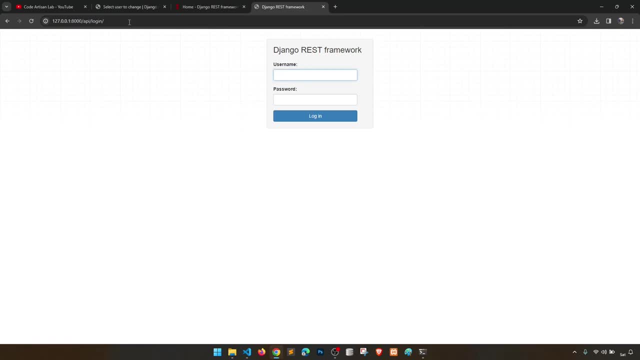 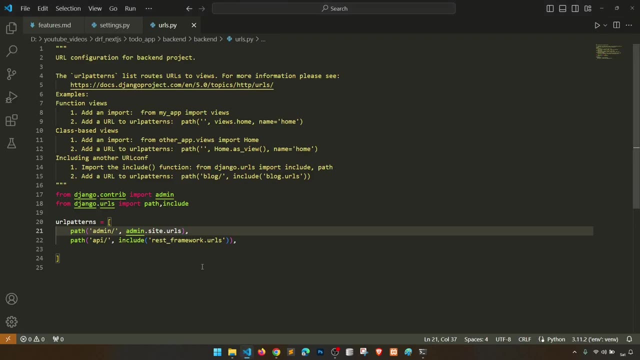 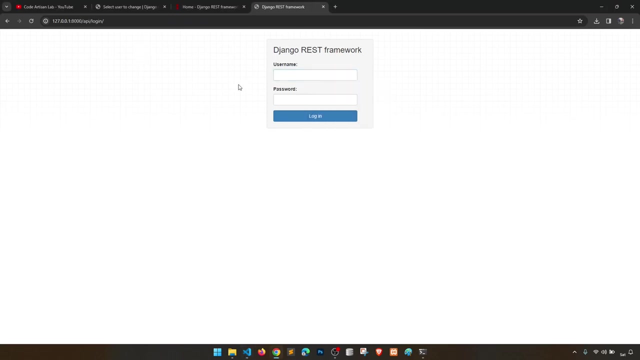 and we will say login okay. so you can see here, actually, on the API it's not we have not done anything, but by default the rest framework urls is login and logout correct. so it means we just need to check that rest framework is properly installed or not. so it is installed right and now it's time to check the. 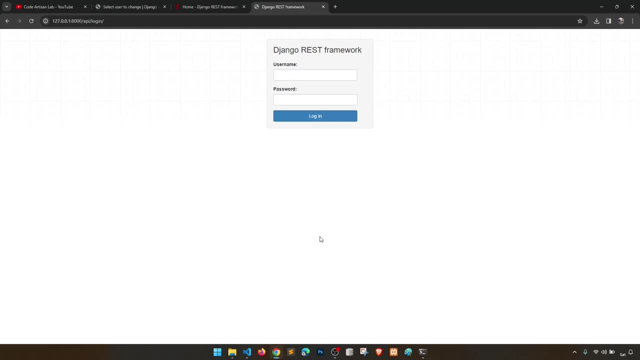 time to up and running the next year's app. right, so our back-end is properly set up. we need to fetch and pull the rest framework urls and we can see here that the rest framework urls is posted- the data we will see that. later we will see how we can authenticate, and all that and now. 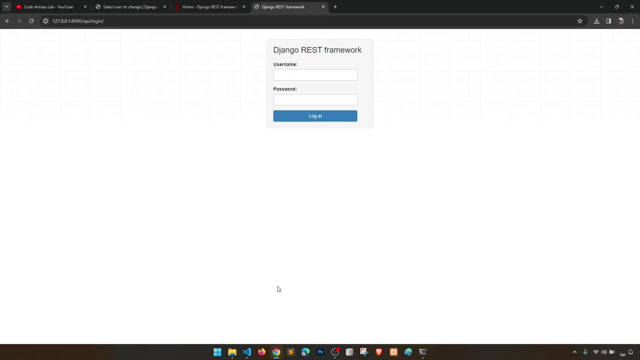 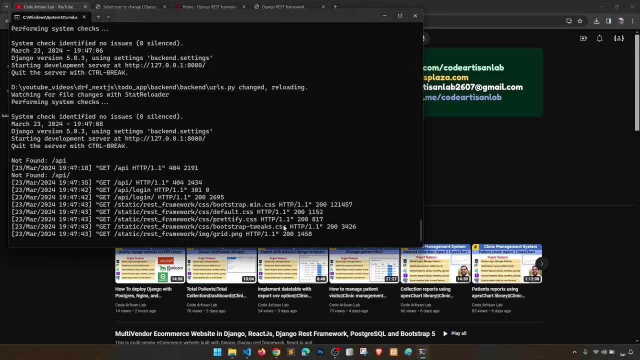 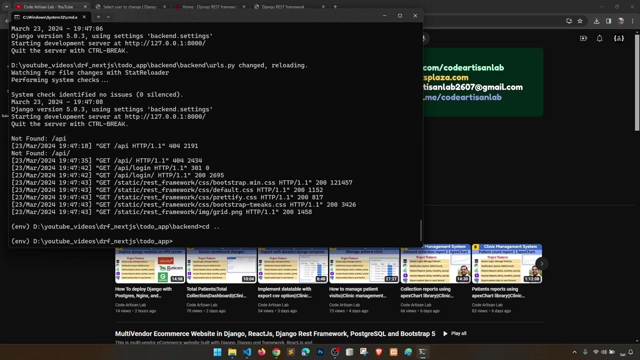 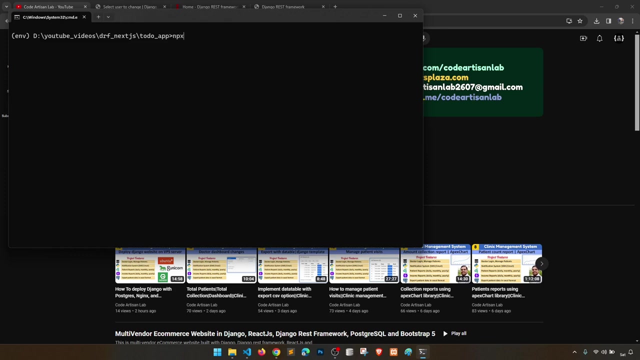 we need to uh set our uh nextjs app right, so let's do that, okay. so for the back-end, uh, let's, uh, let's uh close this server. let's one step back and clear the screen, and let's trade npx, create next app, right, and the app name is, let's say, front end. uh, remember that you should have. 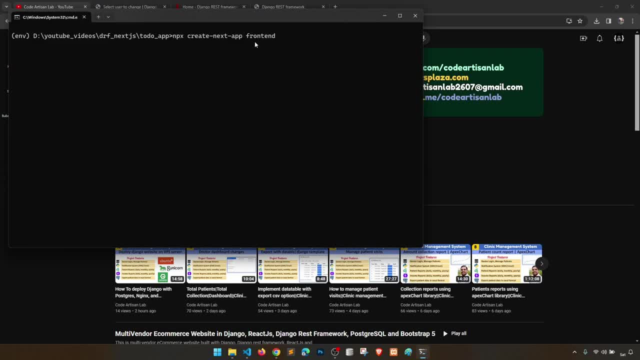 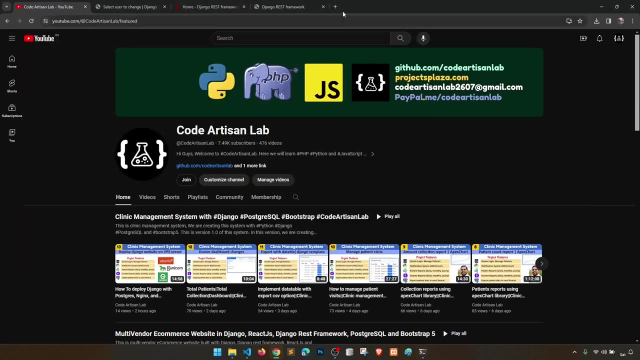 nodejs installed right. uh, i am using uh when i'm creating this video. the nodejs version is 20, or maybe 20 plus, and nextjs version is 14.xx- something right. so please install the nodejs right. you can uh follow the nodejs tutorial right? nodejs, not tutorial. nodejs documentation. 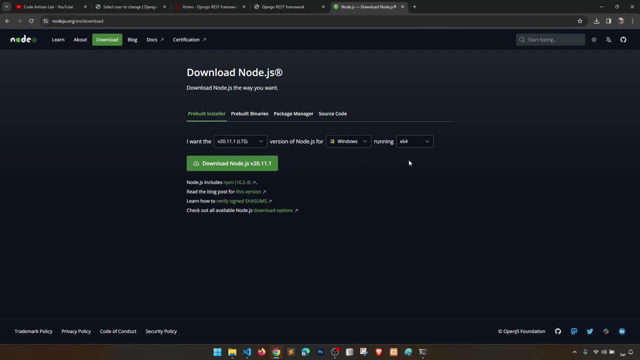 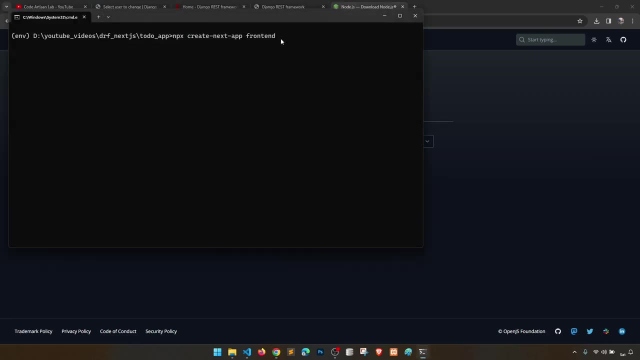 that how you can download, for a connect to your operating system and from that, from there, you can install the nodejs. so i have already installed so and so this is the command to create a next app. so npx, create next app front end. so let's say so. it is saying need to install the following package: 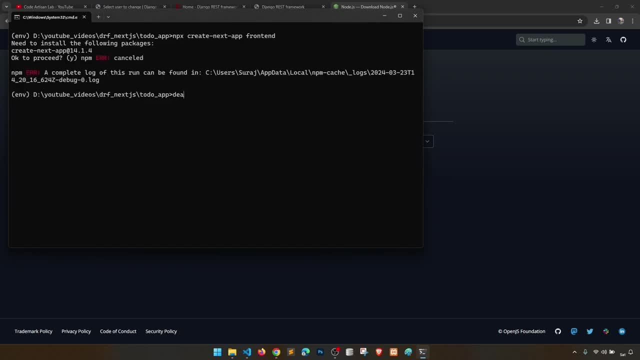 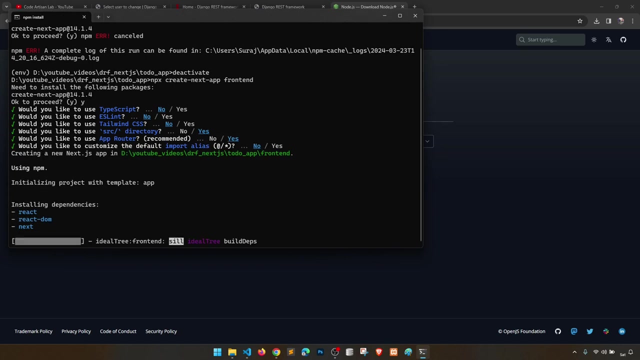 okay, one more thing: let's deactivate the environment. okay, now let's run the command. so i will say yes, would you like? typescript: no. ps: lin: no. tailwind css: no. source directory: yes. app router: yes. so i'm just going through the default settings, correct? so i think it will take. 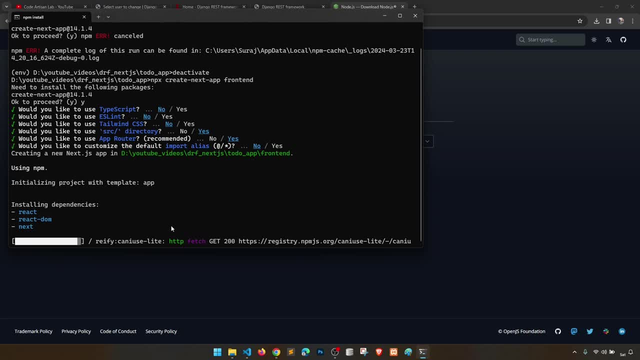 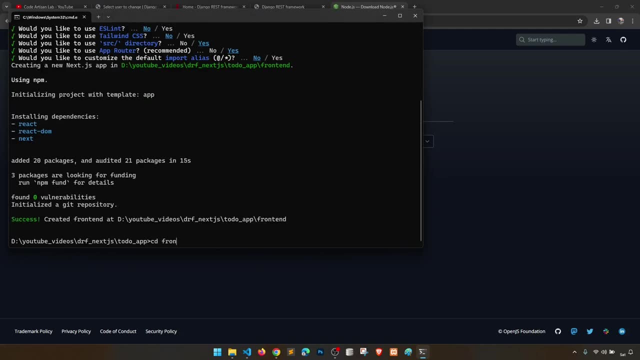 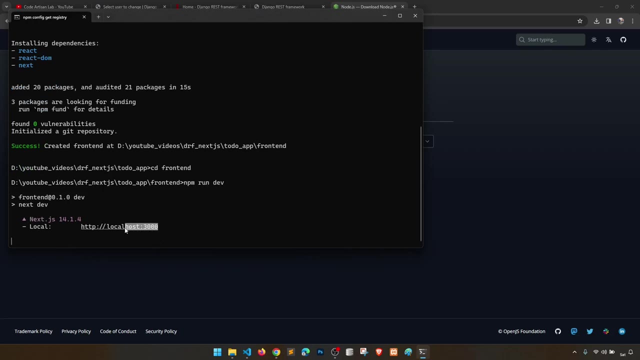 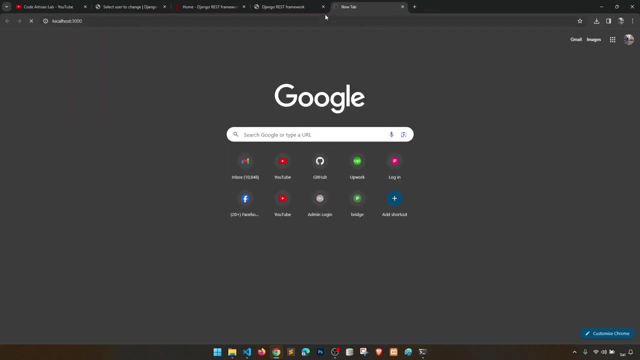 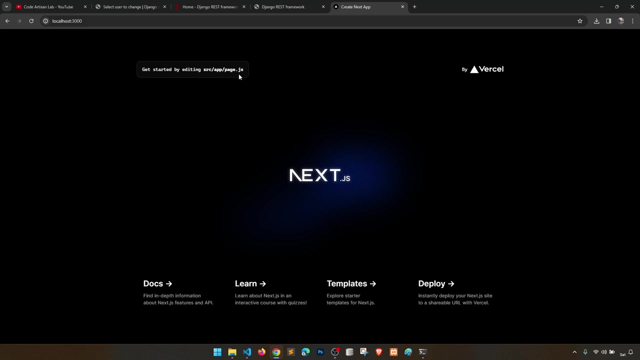 one, maybe less than one minute, so let's wait a few seconds. okay, so it's created. right now let's go to front end and then npm run dev, right? so let's see localhost 3000. copy this and paste it here. okay, so let's see. now read in 2.8 seconds so you can see. so next gs is. 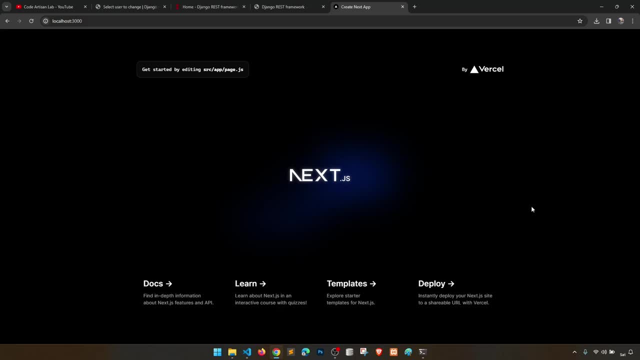 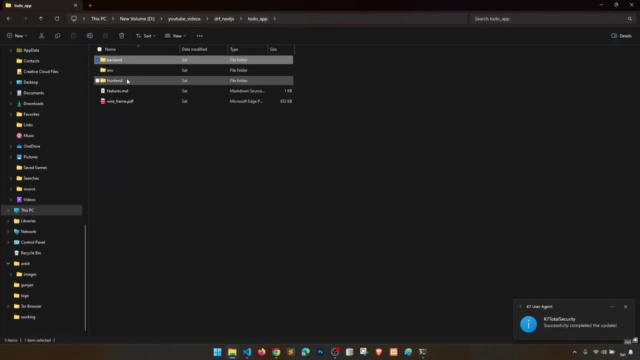 created by a parcel. okay, so it's showing the home page, right. so let's just just for the, because we have set up these things. so let's go to front end. okay, and let's go to source app and this is page dot GS, which is: we are seeing this, so 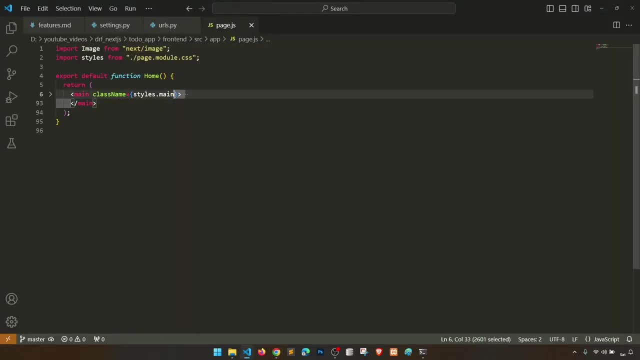 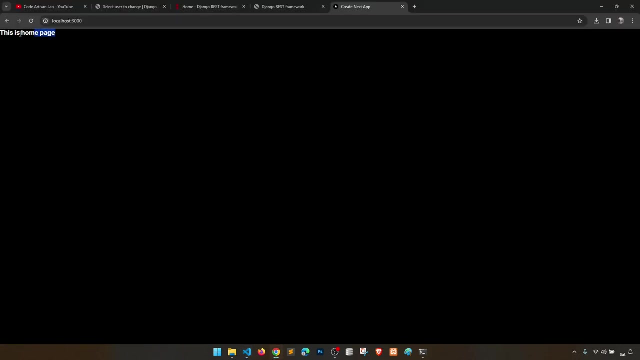 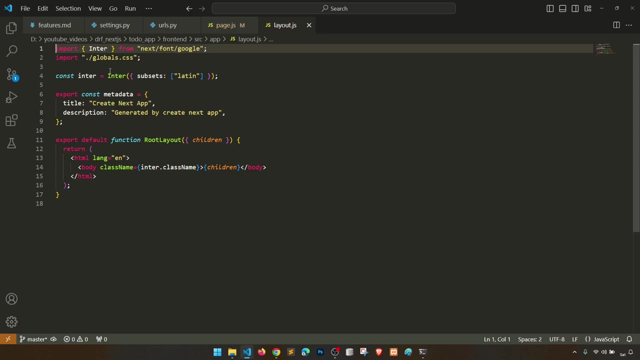 what I will do. I will just remove everything right and remove this thing also and remove this thing right, and I will say: this is home page correct. so you can see, here this black background comes because this page is our children of layout dot GS and in the layout dot GS we have global dot CSS. let's remove. 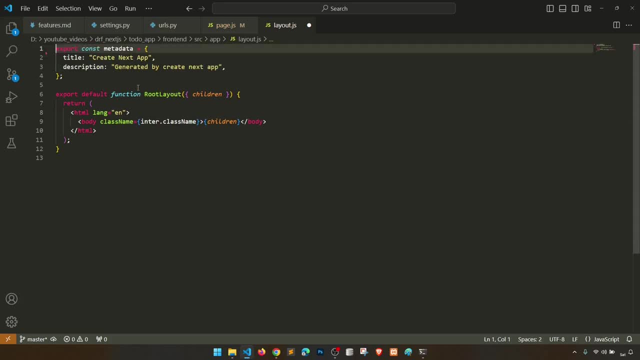 that also let's remove. I just want to keep it simple, right, so let's remove this. so this is the meta data. right, with this meta data, you can define the title and description. this is a very helpful for SEO and but remember, you can- you can create meta data only in. 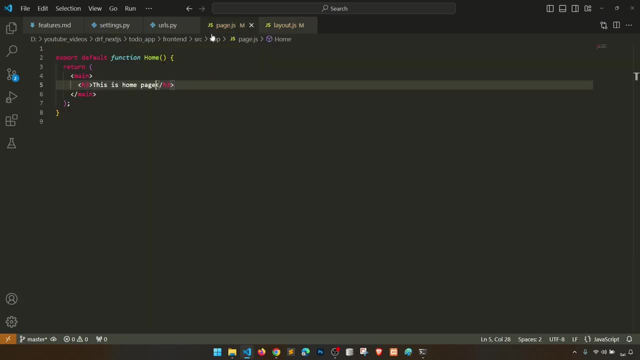 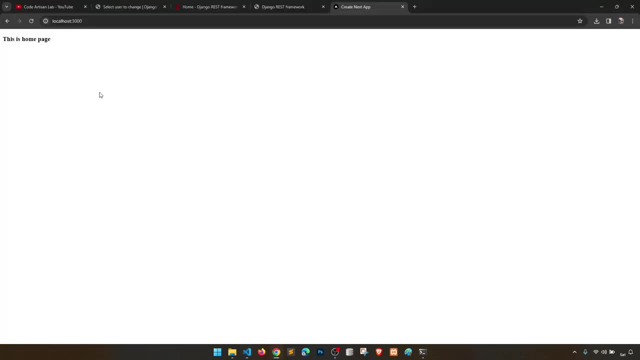 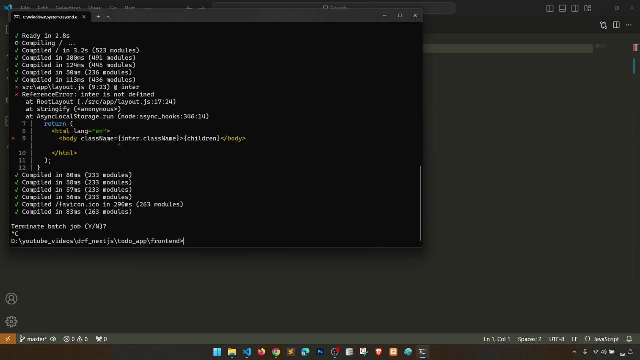 the layout level files, right, not in the children level files, correct? so if I now you, if I see this, then you can see here: this is home page. now let's install the bootstrap so we will install that. so, npm, install bootstrap so it will install the latest version, like we have in Python, we have a pip in the nodejs, we have a npm. 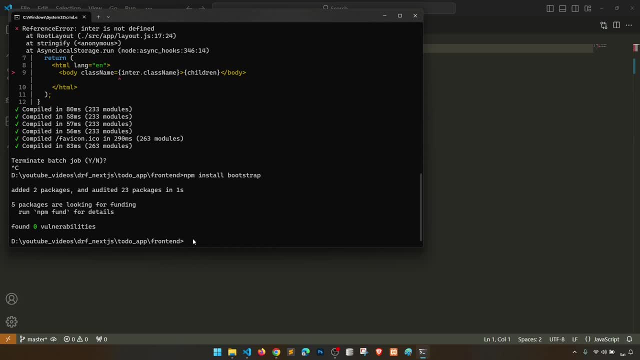 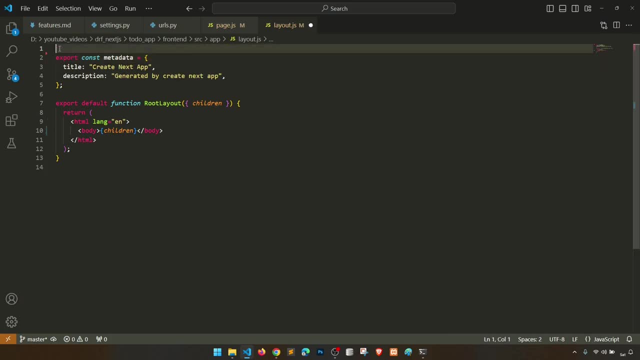 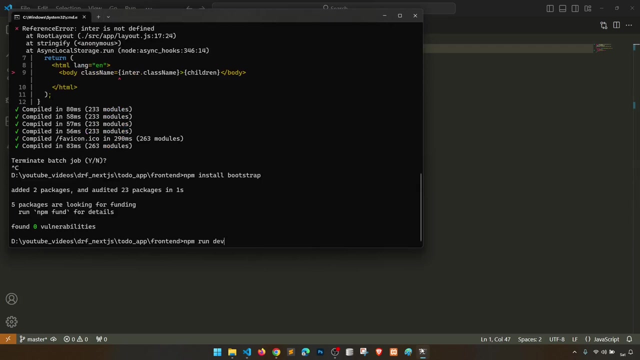 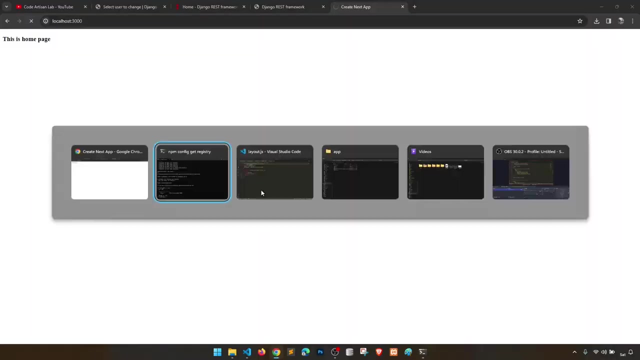 nodejs node package manager: right. so we have installed now in the layout what we will do in the layout. we will do a destruct, unporting, глядing, unporting, import, sanct, import bootstrap. this will automatically comes from the node modules. destruct CSS bootstrapmincss. correct now when we run the app now. so let's see refresh the page work. the вот s symptom: Roberta st uprising. page át la opção. message à dia 8 à 06. 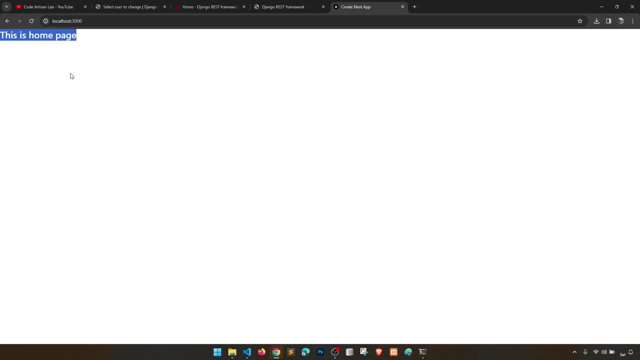 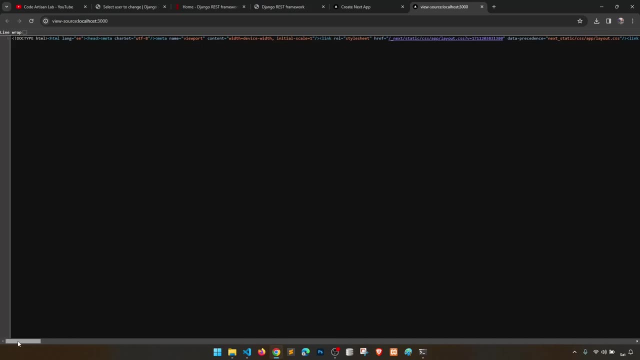 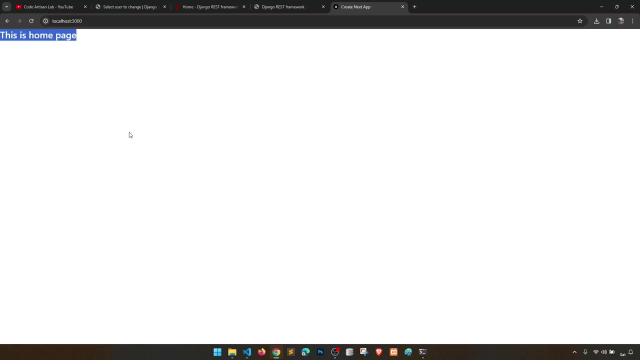 so it's compiling, compiled, so you can see here fonts has been changed. it means bootstrap has been installed, right. so if i, i think it's compiled, uh, node, uh, next, gs compiled all the things, but now it's showing correct. so we have successfully uh prepared our backend, our front end. now it's time. 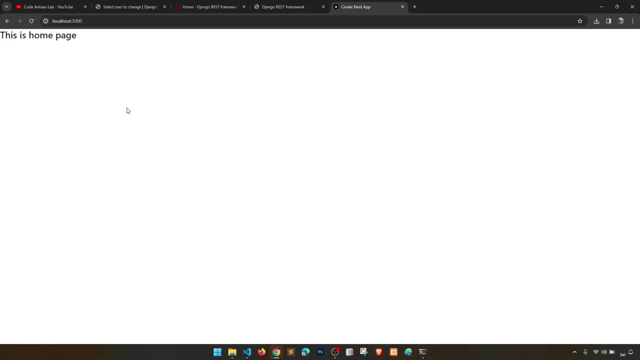 to go, uh, go deep in this system. uh, we will create a layout in the next js, then we will call the. we will create an api, then we will connect our front end and back end with the api. so we will do those things right. so currently we have a separate uh app. uh, like, we have a front end as separate back. 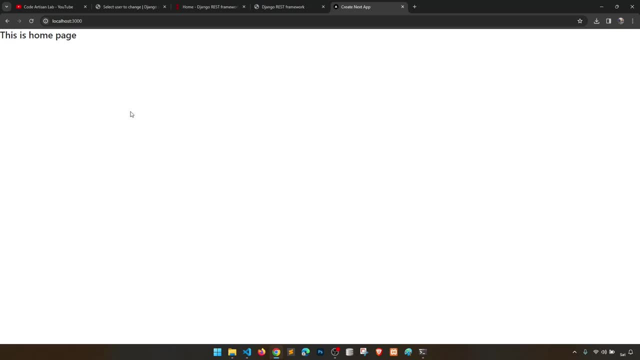 end in separate. now, in the upcoming uh sections, we will see that- how we can connect and how we can do the thing, things right. so let's start to create the templates in the next js according to our requirements, right, okay, so first of all let's create the uh home page, right? so for the home. 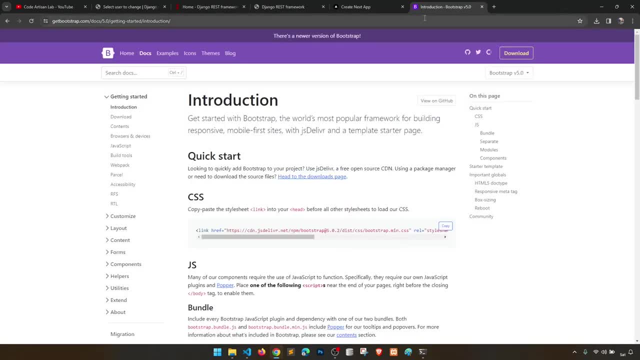 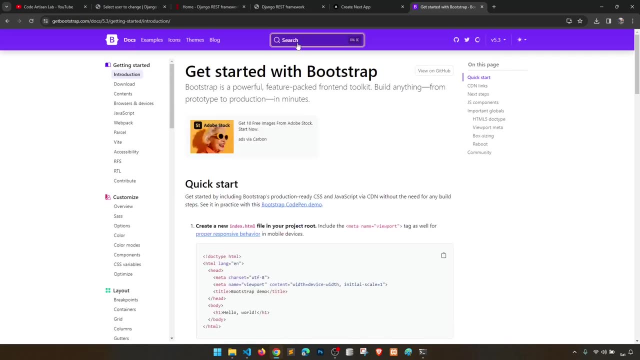 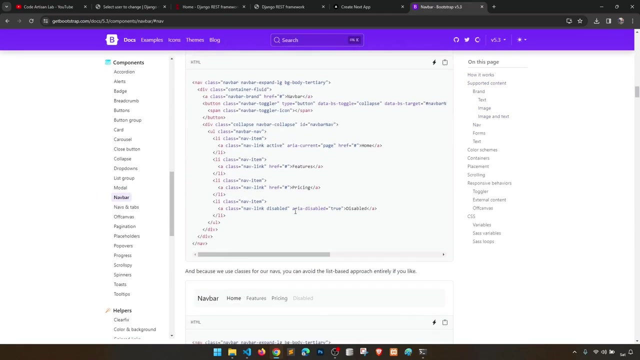 page. i will take reference from the official documentation of the bootstrap. so i will go to home page and i will go to docs and i will go to navbar. so i have a little bit knowledge of bootstrap. so it will, it will easy for me to create the things. but if you have, if you 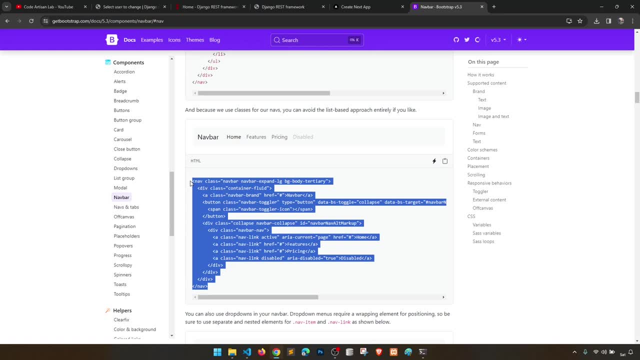 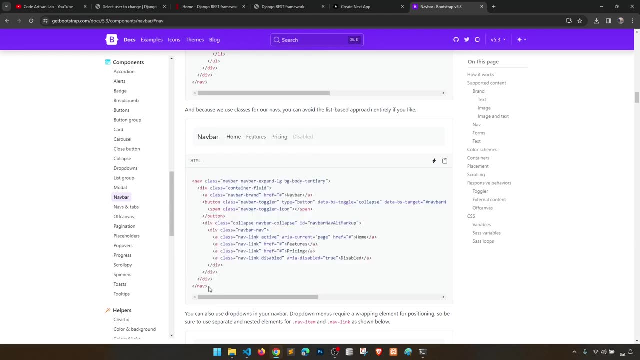 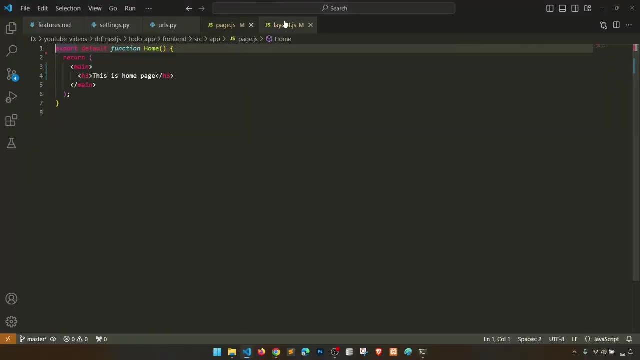 are a beginner in bootstrap, then please go to uh, follow the documentation of the official documentation, and here we have a navbar. so let's create the navbar first, okay, so let's copy this one and in the page- uh, not page- let's create one more thing. let's create a header, right? 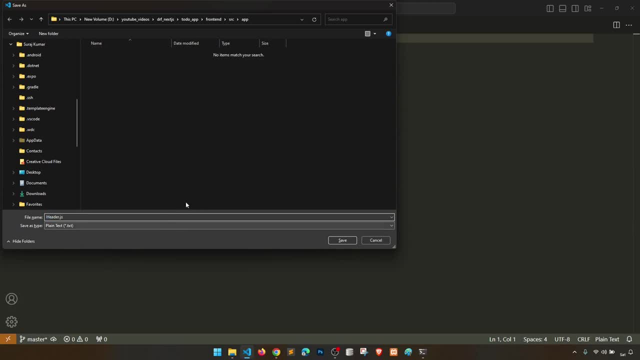 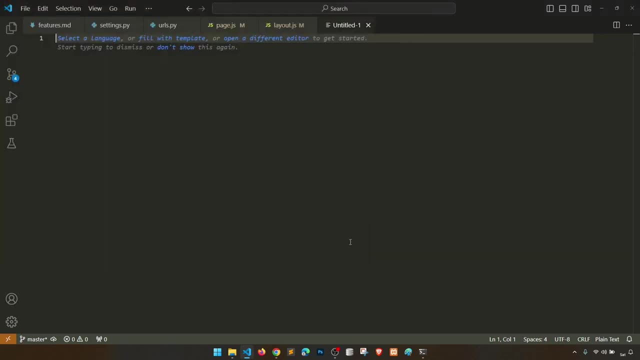 so i will say headerjs. in the app i will create a components, right in the components i will create headerjs, file right, and in this i will create. so i will copy this one and paste here right and i will say it header: and in this header: 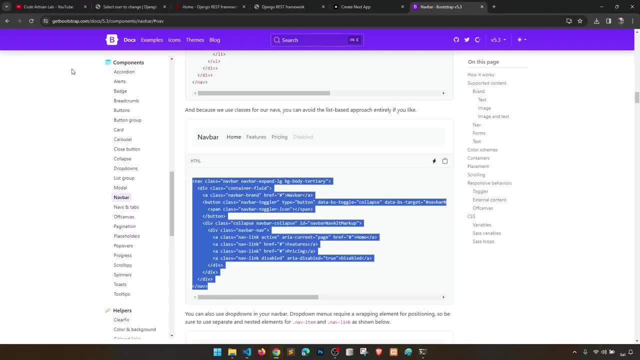 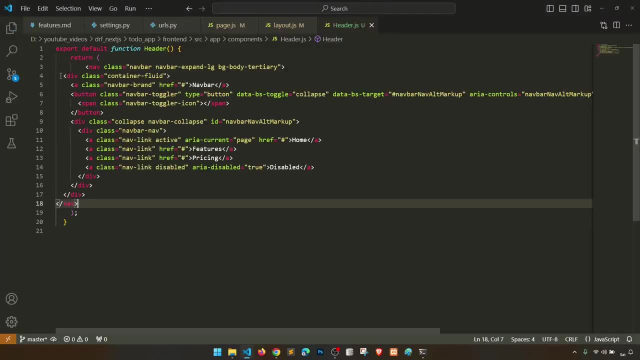 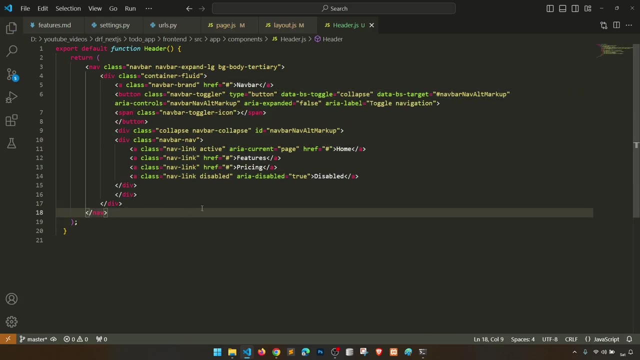 in this header. i will copy paste the navbar right, so copy this one and paste here, correct? so i hope you have a basic knowledge of react. if not, then you can follow my other videos where i am creating the templates and all the things like multi-vendor e-commerce. 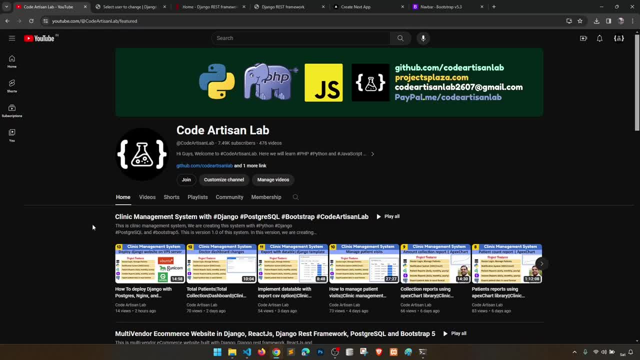 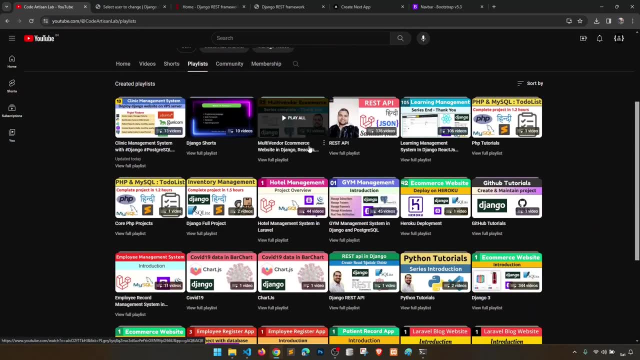 i have created so many projects in uh reactjs so you can follow those if i go to playlist. so here you can see that multi-vendor e-commerce learning moment system. a very nice thing. that 105 videos, 93 videos. so in this i think you will get at least basic knowledge of reactjs and django and api and all these right. so 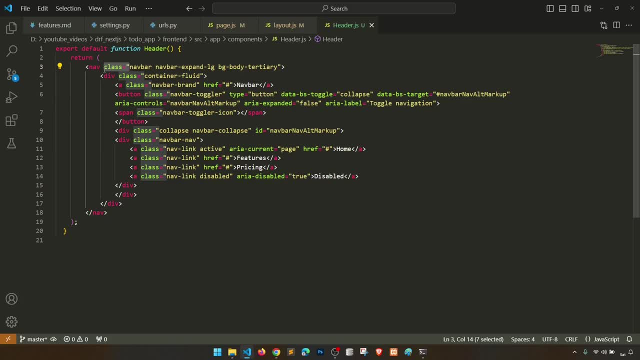 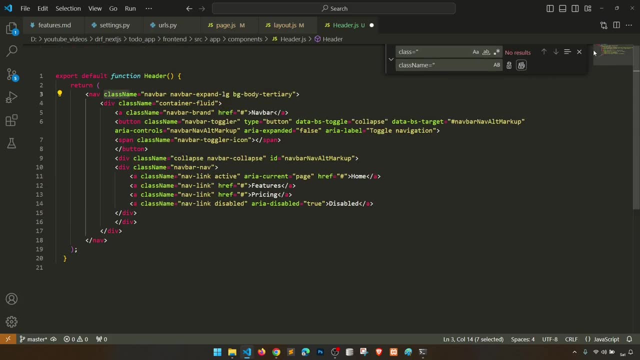 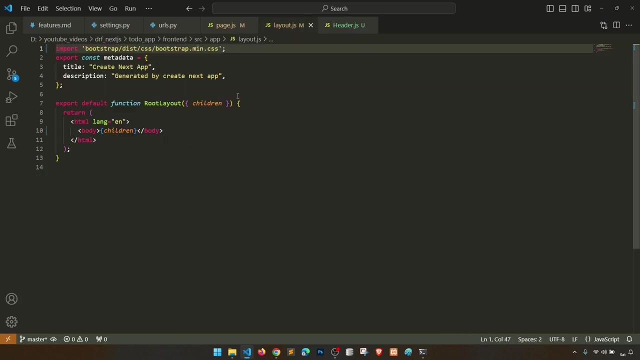 here we are. so what we need to do? we need to remove this class name because it should have class name correct. so this one correct. so now the this is a header, so we need to import the header in the layout. so here i will say header, so this is from component. so here you can see that this is imported. 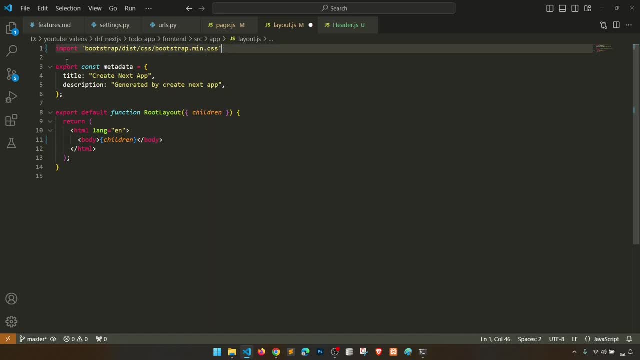 uh, i think we should have it in the page. no, yeah, this is it should have it in the page. all it should have in the layout. i think in the layout. yeah, this is correct. so in the header we have this children and before the children we should have this header component correct. 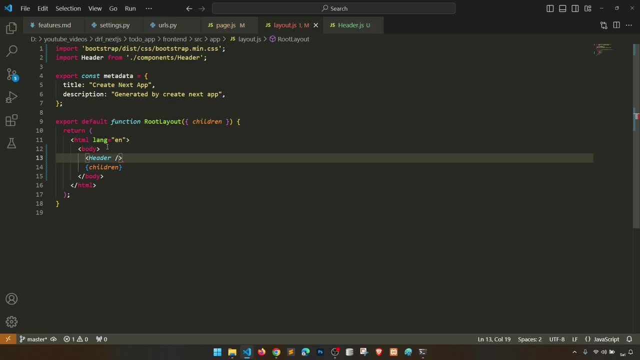 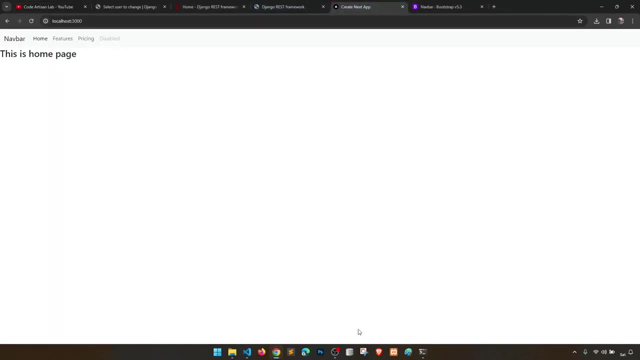 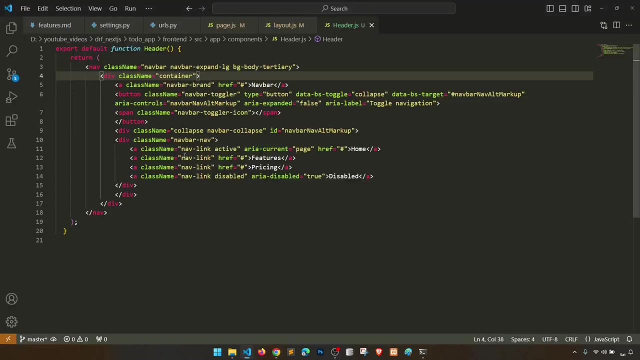 so header component: correct. so we have this header component now. let's see that how this is working. okay, so header is coming. uh, let's remove the page. let's say home: correct, now this header should be in the container. so i will remove the container fluid. so this is nice. okay, now this should be in the. uh, right, so margin start should be auto and 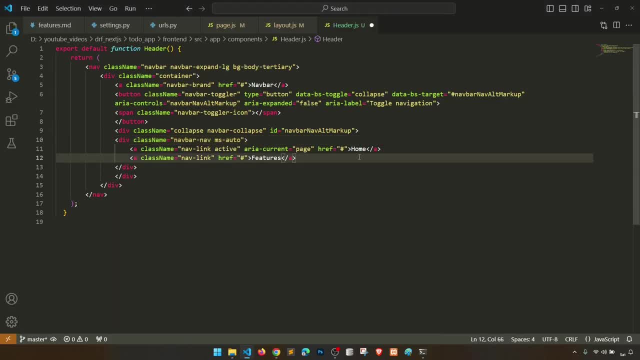 let's remove these links, these two links, right. and then the second one is: uh, let's say login, right so, home, no need for home, i think. or, or, let's say this: the login, and this is about us, like we said in our wireframe, right so? and uh, you can change the uh header of visuals. uh, you can see. 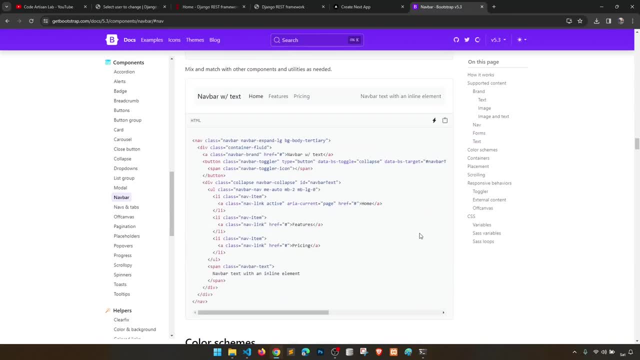 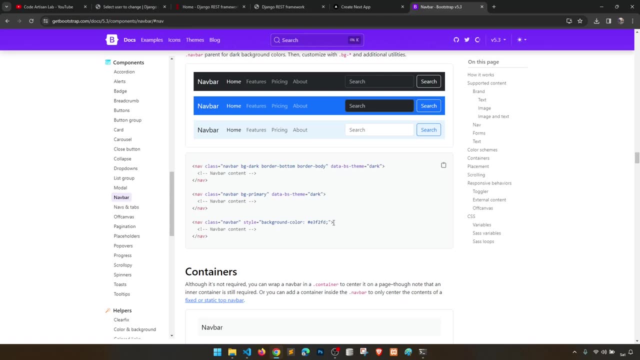 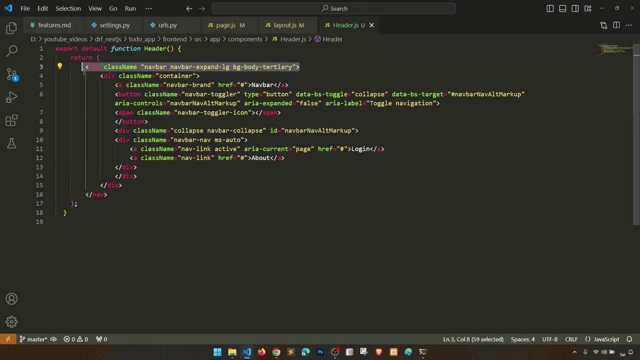 here, the background and all all the things, right? so, uh, nav bar, we have this thing. okay, so, nav bar, you can add the styling, you can add all the things. so if i do this nav bar, this one, then it will be a black nav bar, right, so it will. 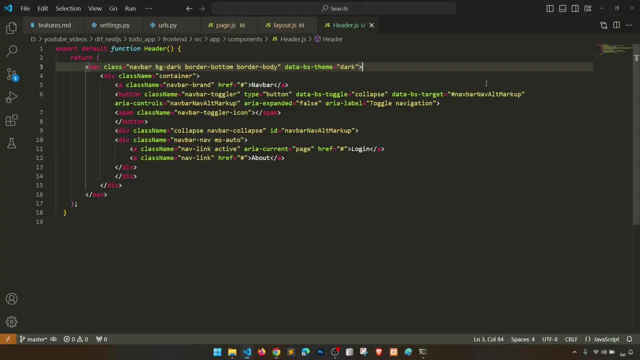 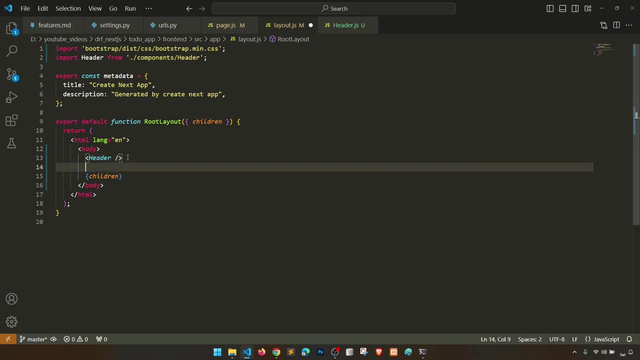 like look like this, correct? not sure why this is doing this icon. if i say this: okay, let's uh make it, keep it. so border okay. so okay, this is fine, and we will say here: my to do right and uh for the layout, uh, we will also add: 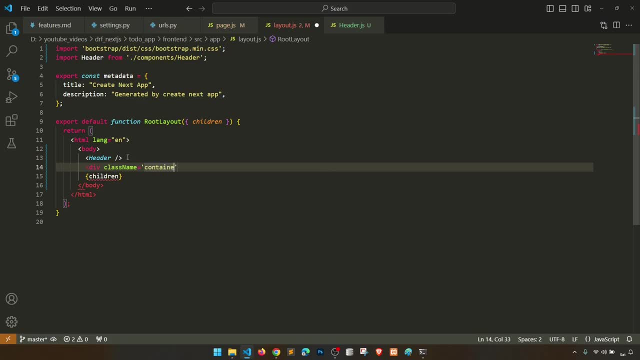 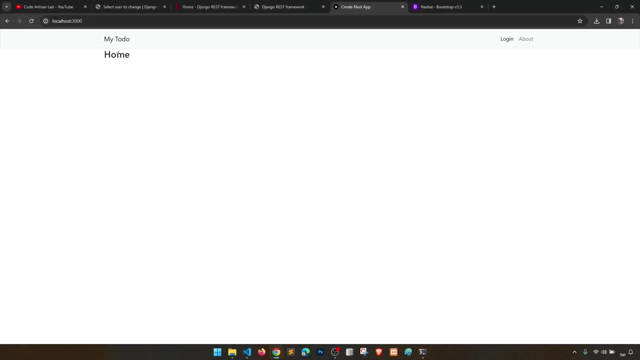 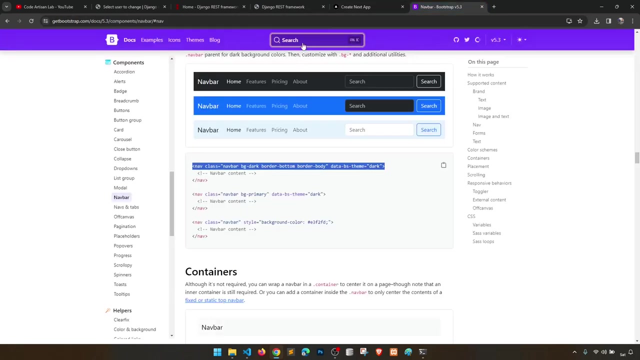 one more thing: div class container: right, so children, all the children's, will be in the container, because i like the container style. all the personal opinions, so this is my opinion. okay, so my to do uh login about uh here. uh, we can add a intro text, something. so what i will do here: 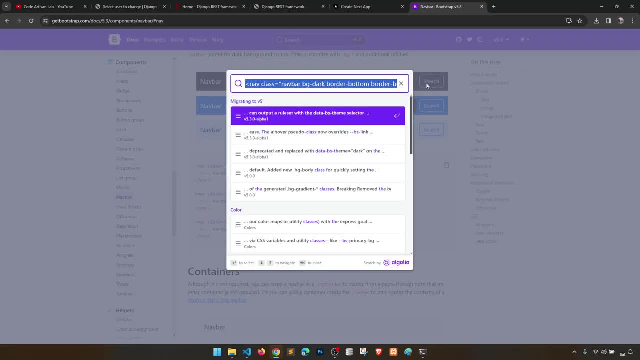 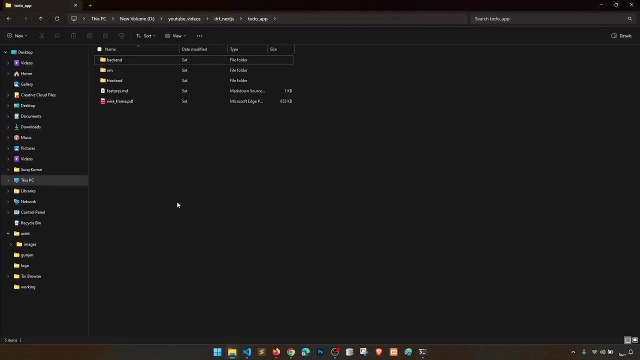 i'm not sure. uh, we can say, let me find something out. okay, so let's create something custom for our home page text. uh, let's open our front end, uh, source, app components, and we have a header. let's go to page and in the page, we have home here, right? 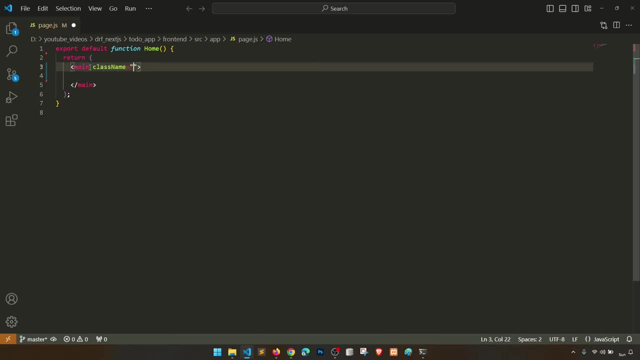 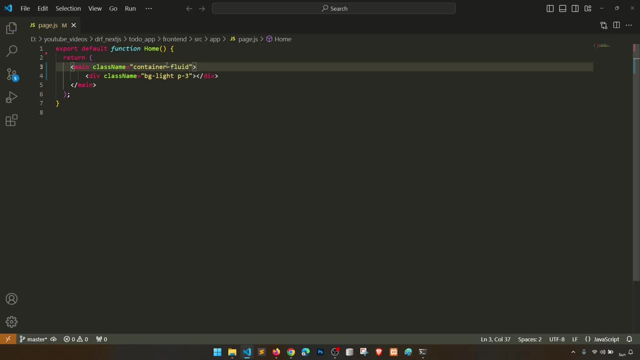 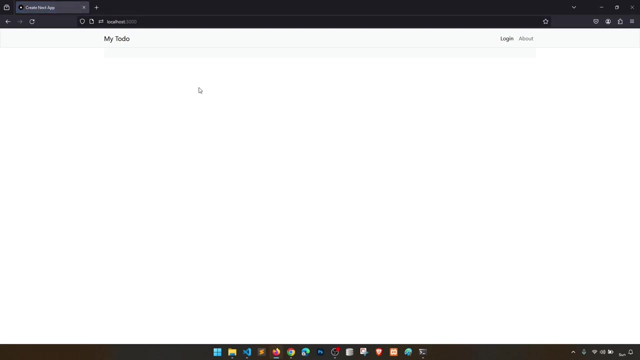 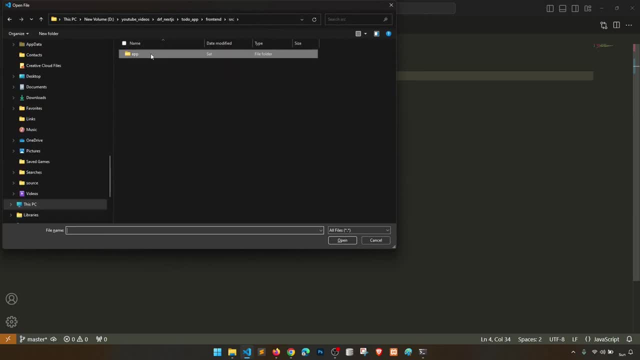 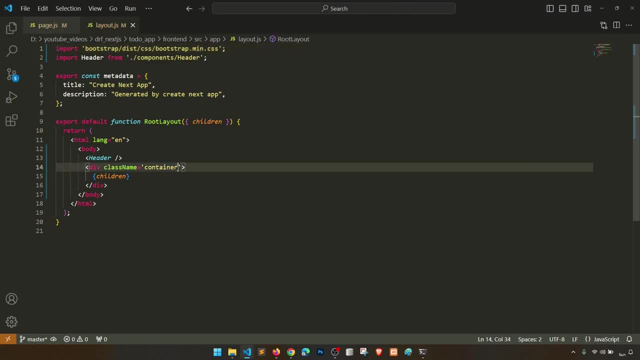 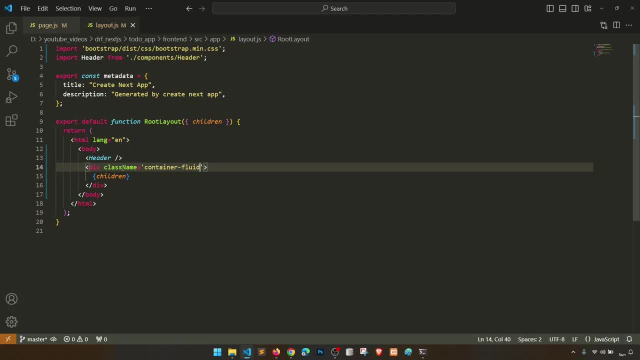 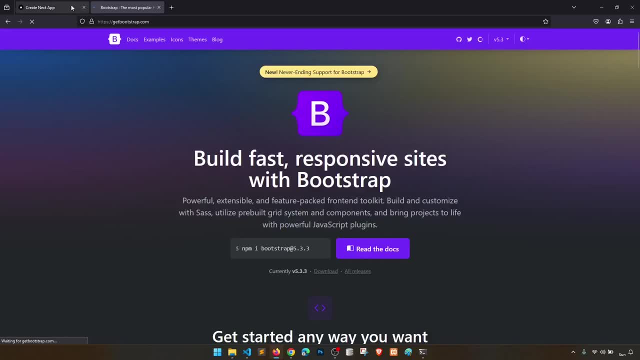 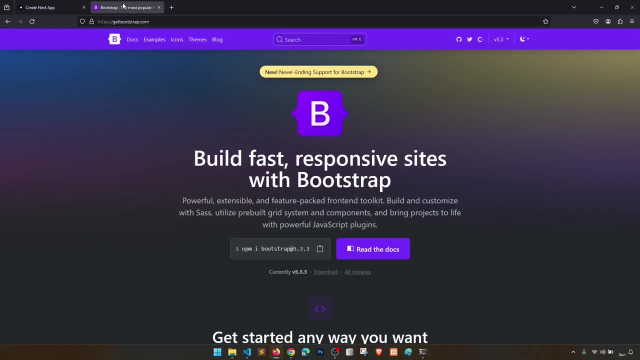 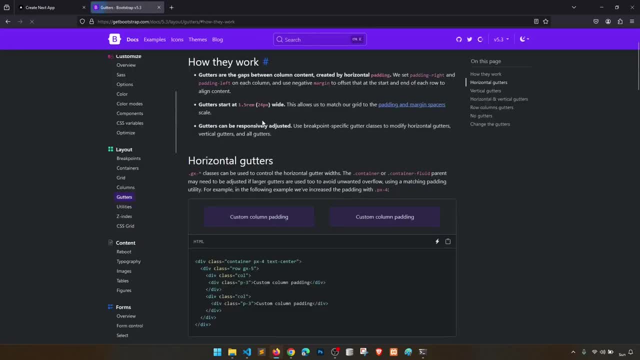 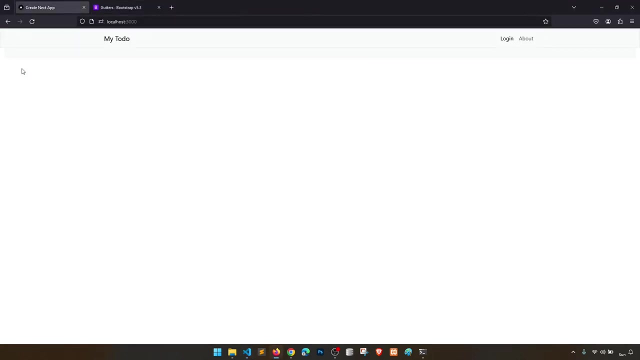 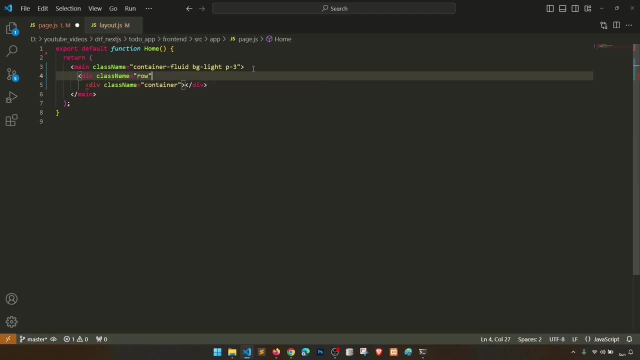 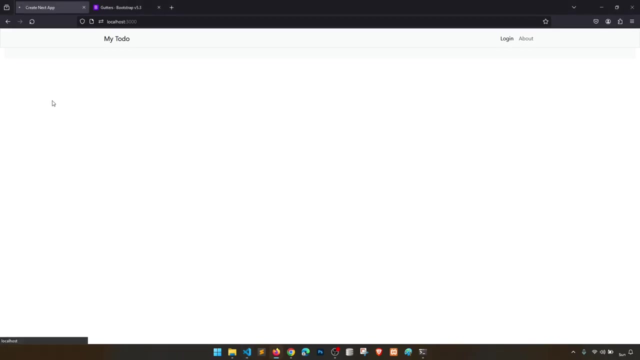 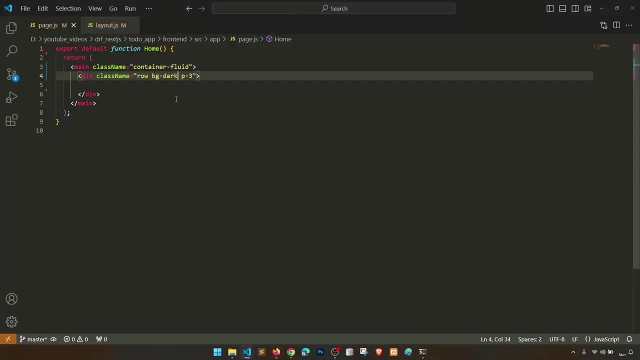 let's do one thing: let's create a row, right, and in that row we will add this BG like: okay, let's remove the container, correct. let me show you what I want to say. see this right. I want to make it G X 0, okay. G X 5 C, right. so this is full now. 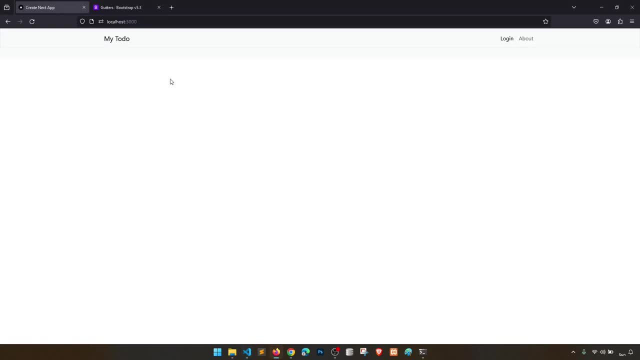 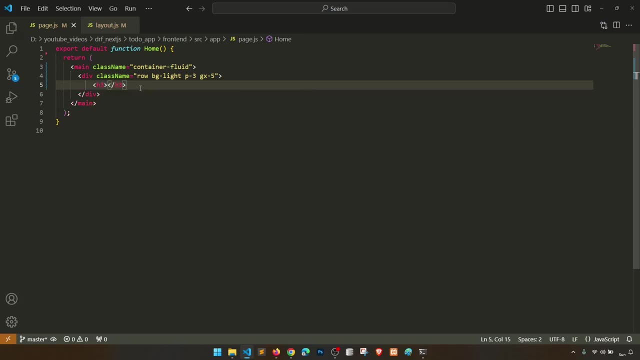 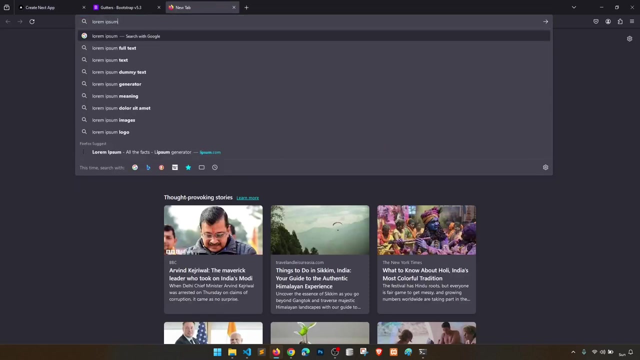 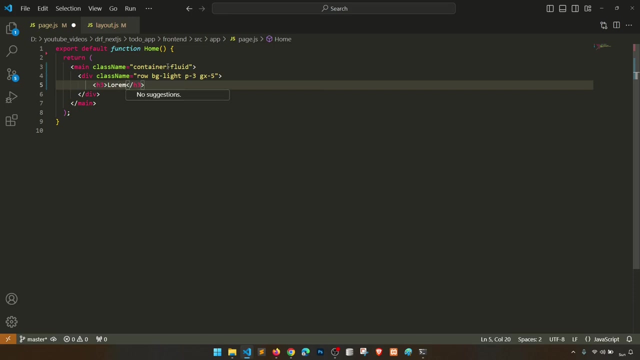 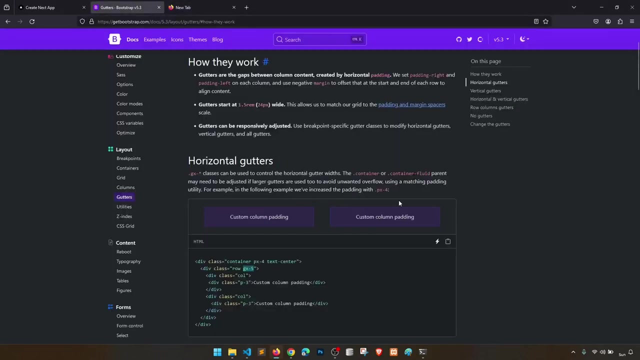 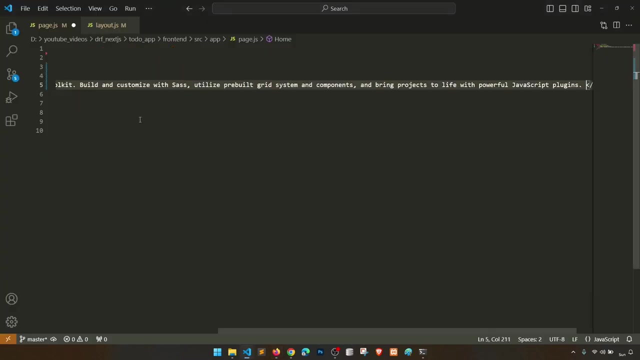 so we can make it light, right? and then we have: let's add a text. we will add the lorem ipsum text, some text we can add from here also. no, no suggestion. then let's copy this thing, star bootstrap. let's copy this one, paste here. see this right, let's make it. 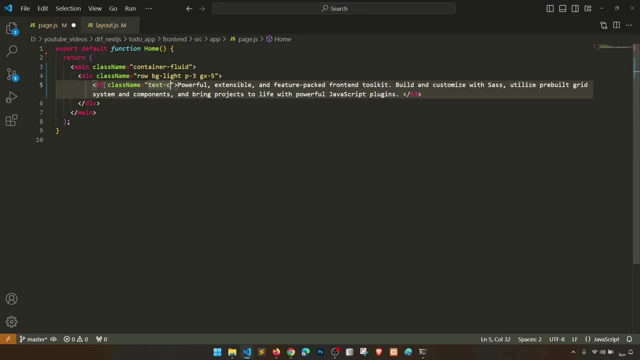 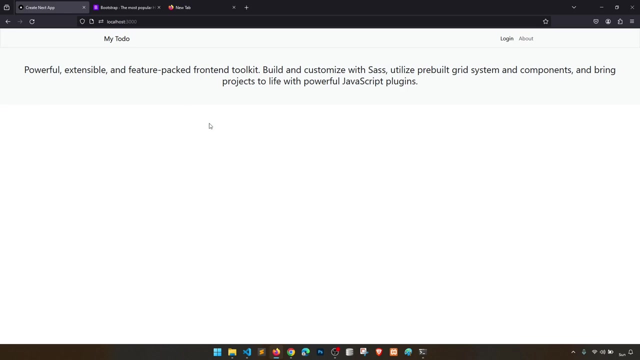 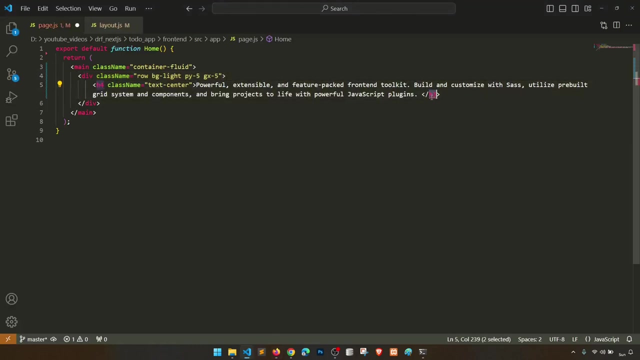 Center. right, we can do margins. why more than? yeah, this is nice, correct. compress the transparency you're seeing here. yes, make it snug, just sometimes we should. I saved this just for its own property and for update to our saves. so itガ Pascal, now here you can. we can give any kind of you know introduction when user visits on the site, like I think we should give our own, get a stir visit on leumpok. sessionslovesEc into Dunlop task tableulnow. here we can create our space for our to-do tasks. okay, we can. we can create our space for our to-do tasks. hey, I think I should give you our own. so let's add this: we so this is 것이 app and here we can open it. 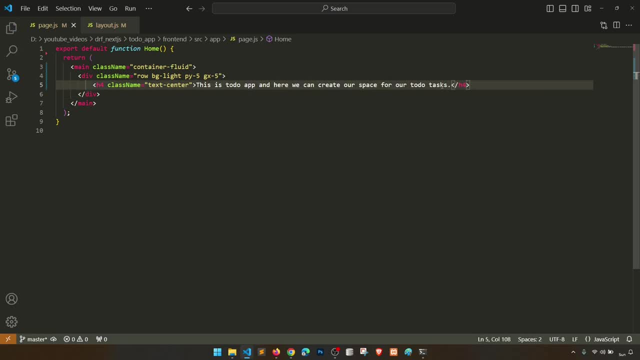 and we can. we can, we can perform actions like create, read, read, update and delete. right, okay, and now let's give a button button and we will give a class button button, dark right. and then we will say: right now, and we'll give a text center to the row. 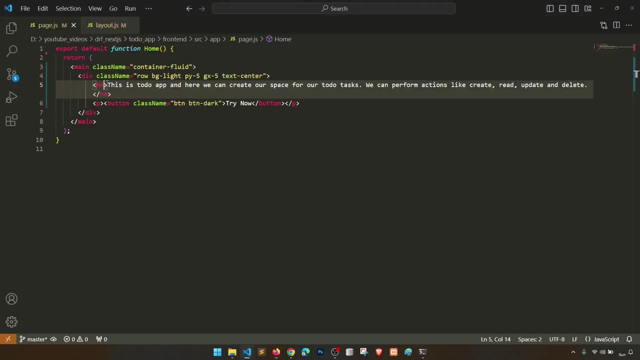 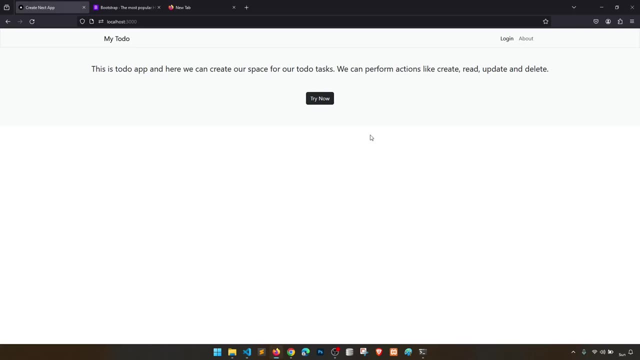 okay, so this one, and let's give some margin. okay, so this is nice, all right. now, when we click on this, then it should be. it will go to the login page, correct? so I think home page is enough for now. let's create one more thing. when you. 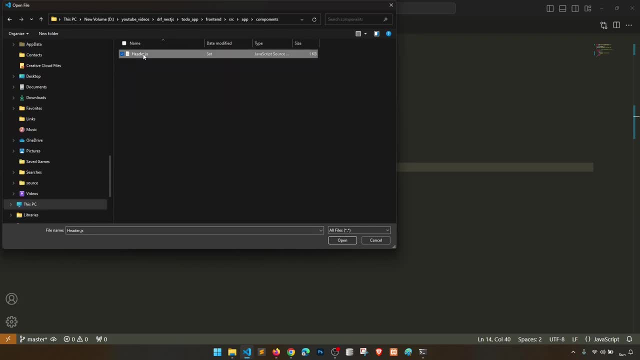 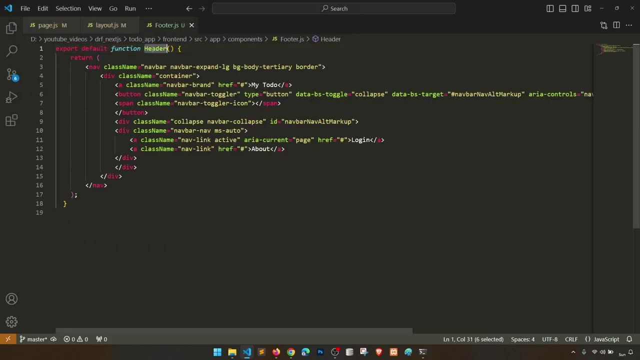 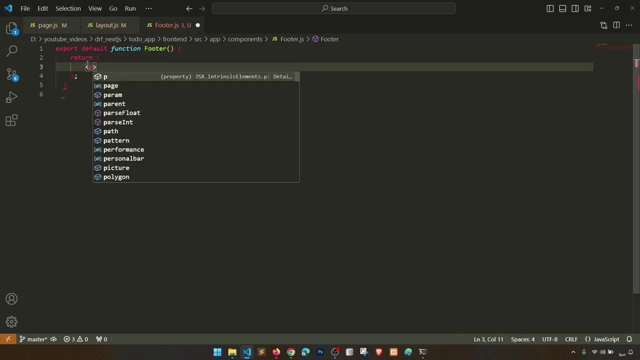 need to create a. we need to create a footer, right, so let's create footer dot JS and in the footer we have this one and we will create simply design and developed by code: artisan lab code. artisan lab code. artisan lab, right, yeah, and we can give her anchor here. so this one, correct, and in the 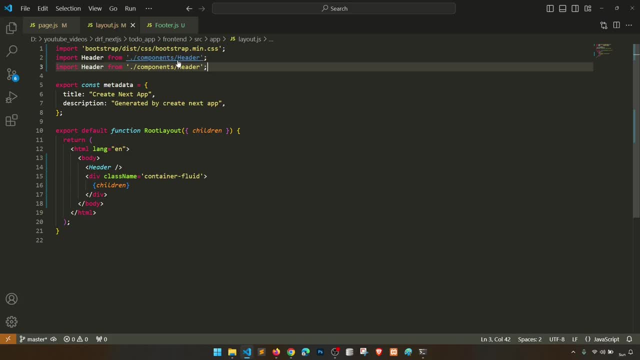 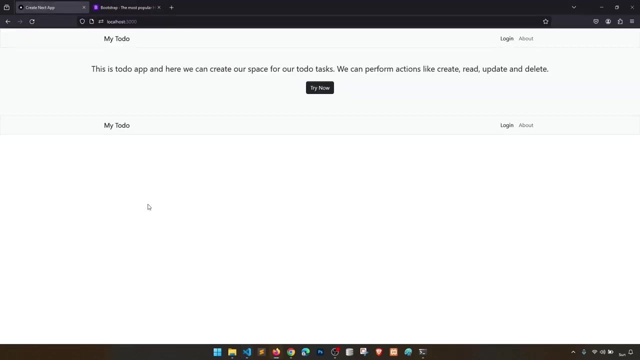 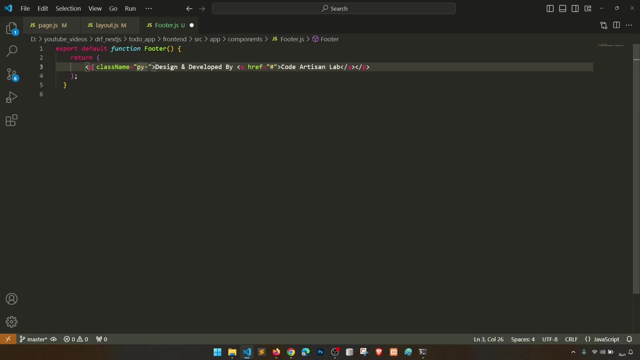 layout, we will import the footer and we will give the footer after the children, right. so here we are: give some mark, give some padding, padding what is not a vertical food right? and is that layout footer? export default footer. oh sorry, right. and then we have this text Center: correct design and worldwide code artisan lab. 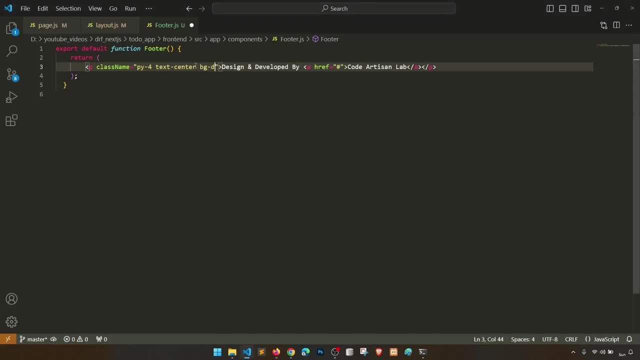 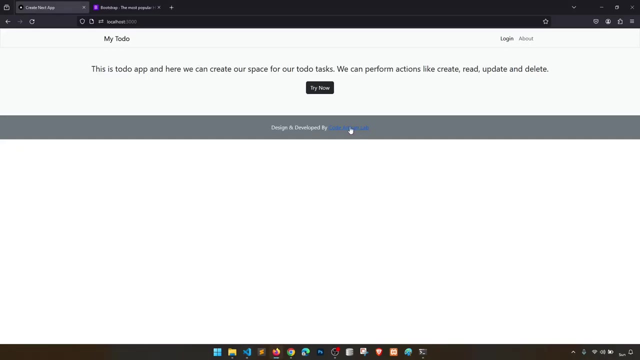 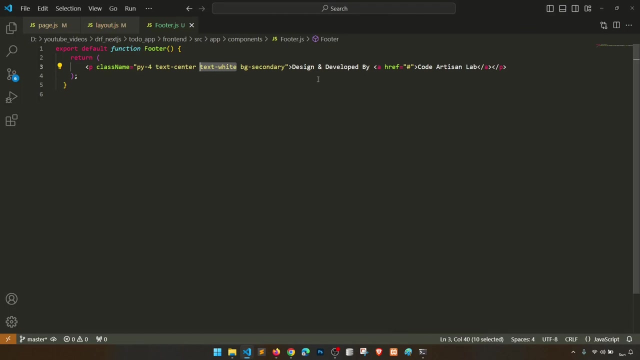 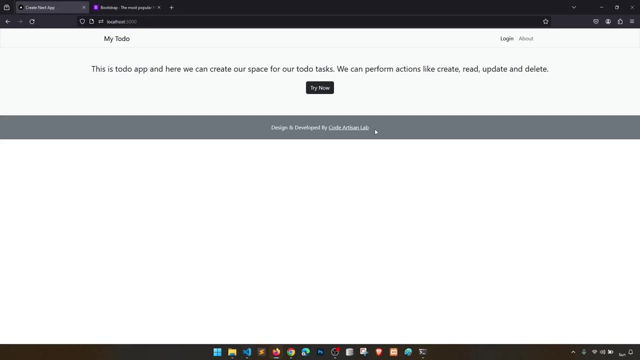 and let's give BG dark, or you can say BG secondary right and will give text color white. so design and developed by core artisan lab. and this is you blue, so let's give it a class text white, right here we are. so design and developed by code artisan lab for, like, we're discussing wireframe. okay, so this is our 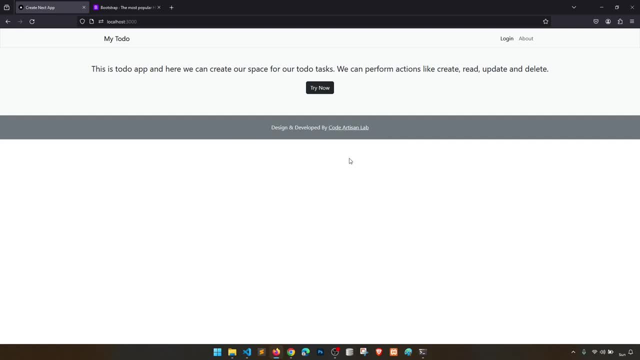 home page. I know this is not very functional, but yes, because we are creating this to do app. so from here we can navigate to the try now. try, now we'll go to the login page right, and if user is logged in, then if we go to the home page, then we can say: 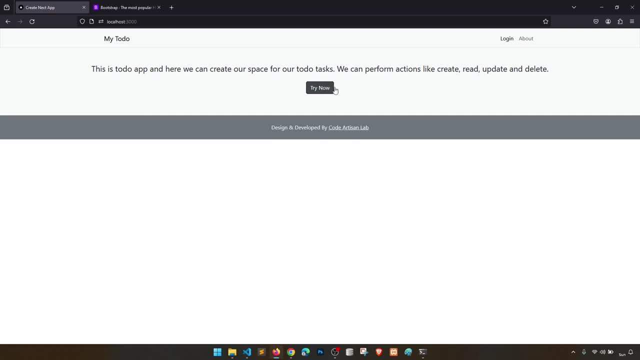 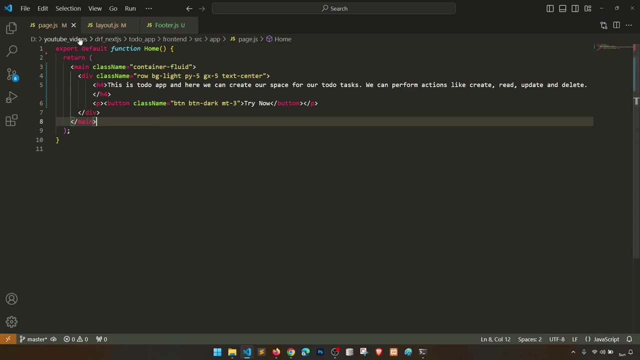 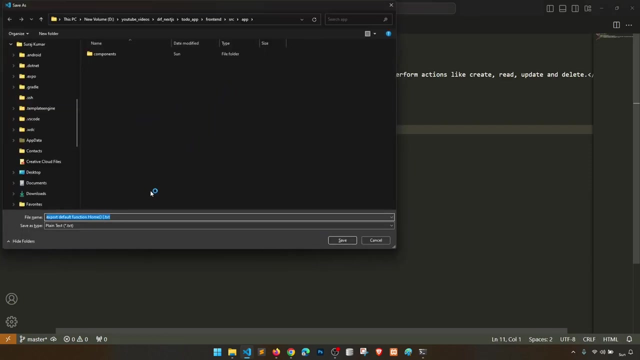 here. see my to-do list. we can see here right now: let's create the about us page also. so for the about us page, what we will do in the in the header: okay, so let's create a, let's copy this page and create a new and we will say: we will say: 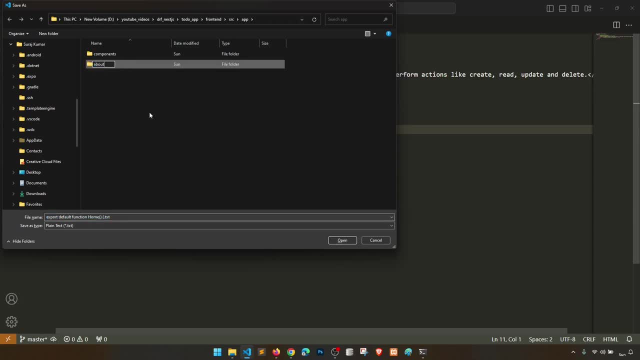 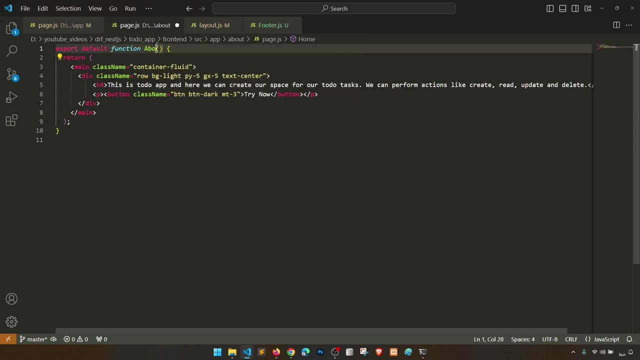 here about right and in the about where we need to create a page dot: yes, right so, page dot, yes. so here we are okay and we will say here about: and this is same thing, but we just need to remove right now and here we will, we can keep the. 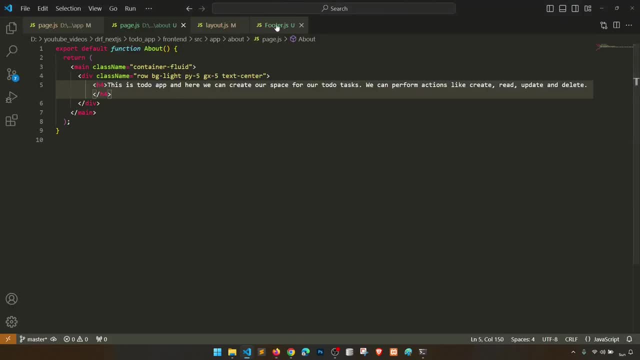 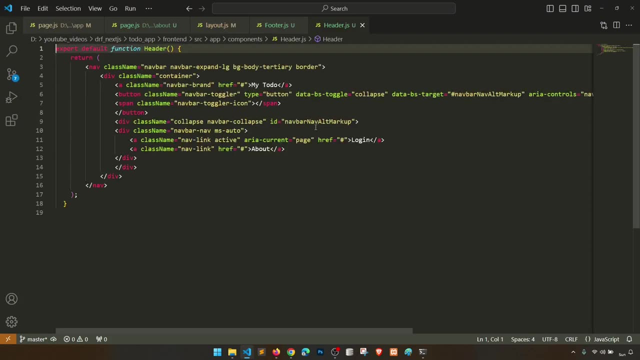 same thing for the about the speech. now in the header we have to route the. we have to add the pages router which comes with the default next year's, next year's world work as a next year's router. work in the pages right like. I have created a folder. 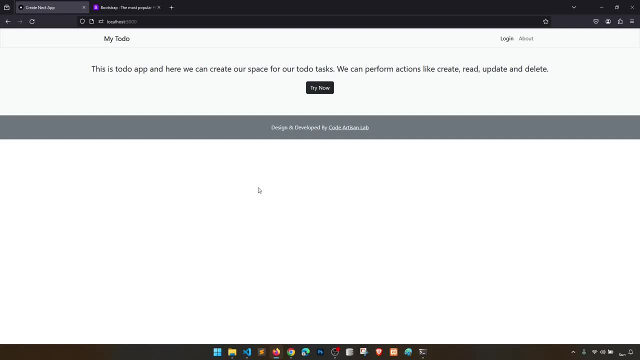 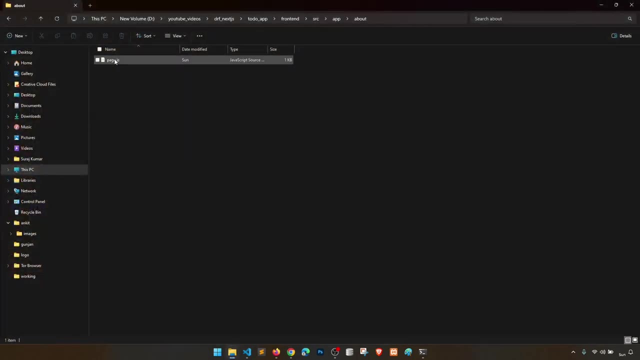 about and then created a paid page dot J, a page dot GS. so when we space this about then it will automatically try to find the try to find the about us page, about the folder, and in the about folder we have created page dot GS or you can. 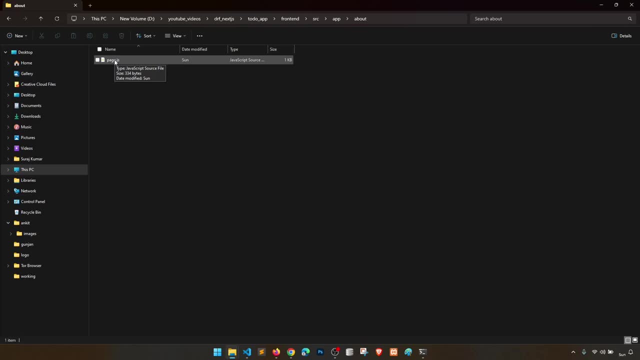 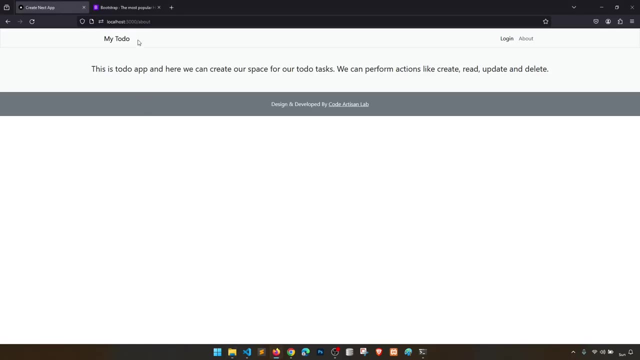 create a page dot GS and then create a page dot GS and then create a page dot with. so now we have this page and now we. so we have this page where we have written. so now we are going to move the scene delivery. I will add: and this is what we know, and now we are going to go to our page. 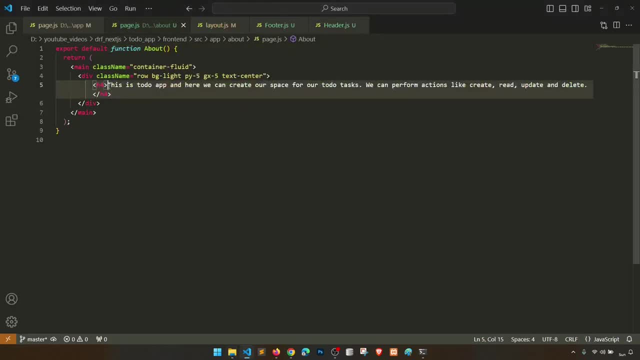 checkout, moving the feed boundary we are going to choose. this is a fifth buddy, what you see here, for which is the page we are creating quite to every page: 新加way, and there we are taking this page. you see, you can adjust it. so, numéro quirka D, you can adjust whether you want thisj trabajar for details. 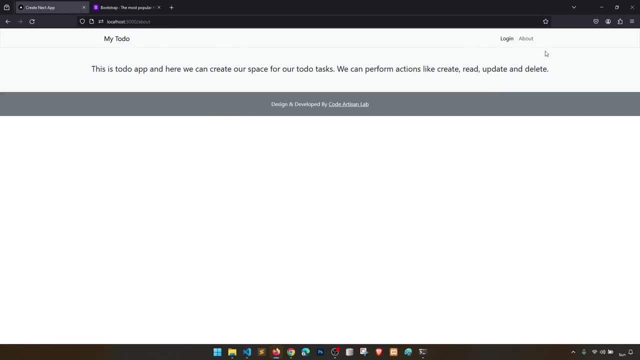 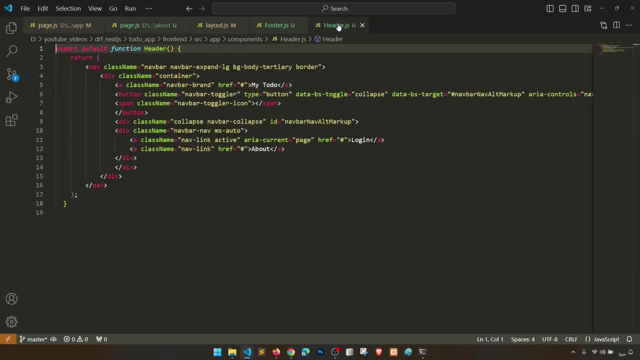 category or you can make it with, so you can create a home dot. yes, so it will be the have when we go to. okay, so currently we are going to this page from the URL. now we need to link this right, so we have header here, so I'm going to import our 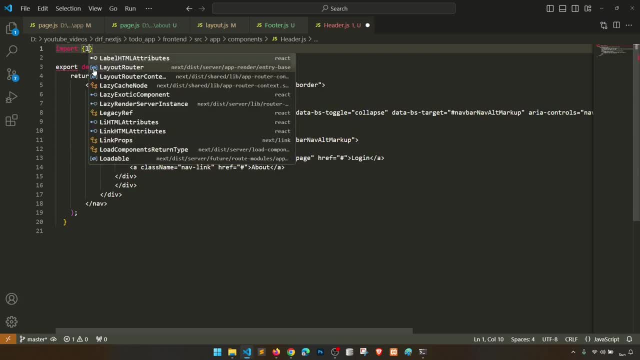 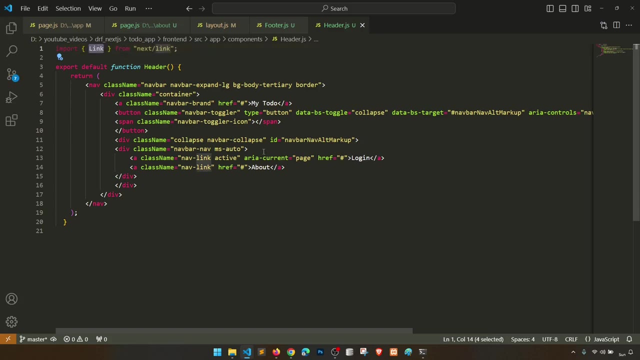 module import link. import link from- sorry, link from this will be link, so link from next link. so what it will do? it will optimize our anchor URL or you can say the link tag: okay for the route, okay, so link and the all the all. thus one minute, okay, and all the things are same, but this tag will change, correct. 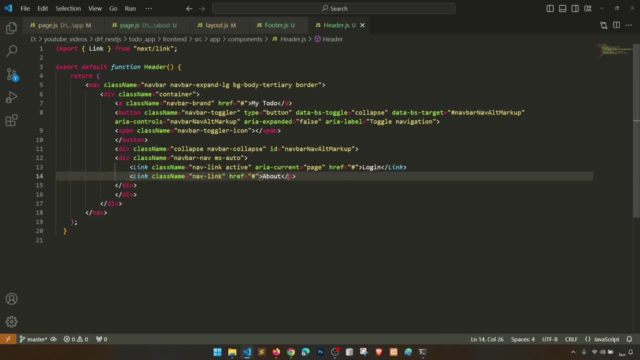 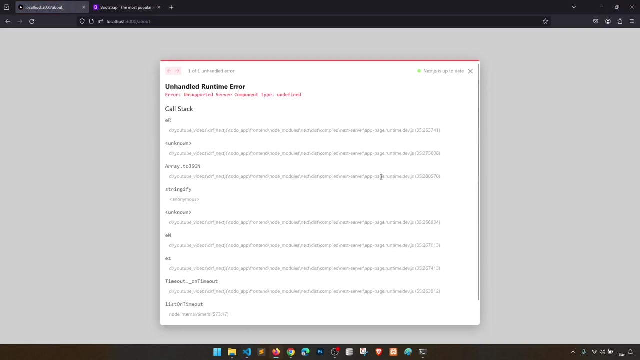 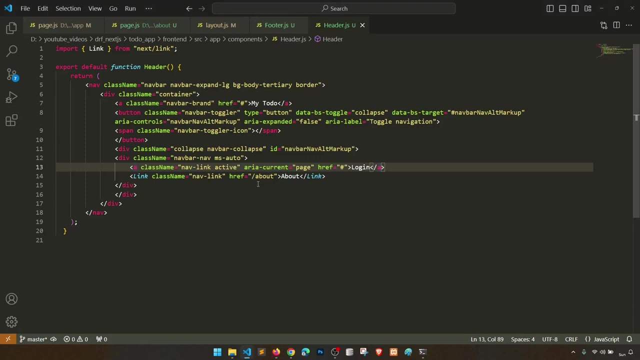 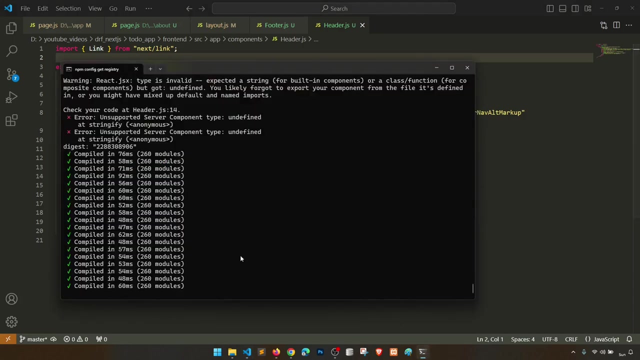 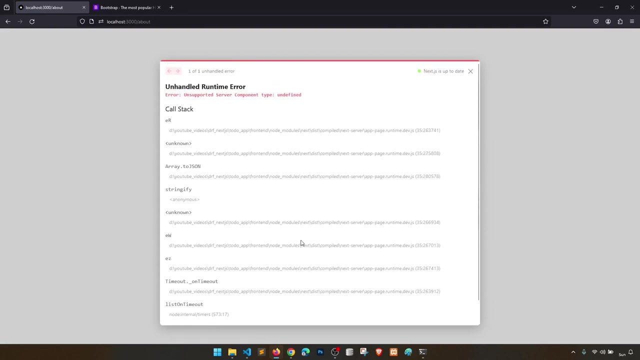 so we have this link tag right and we will see here about. correct. so server is not defined. let's keep it anchor, all right. so it is saying next is up to date, undefined why this is undefined. it should be link next link. this is correct. let's see here now. this is also correct. 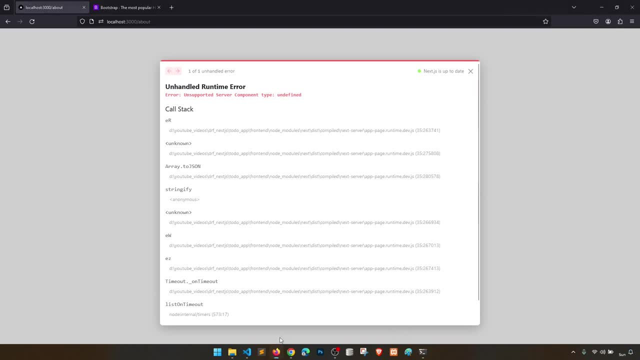 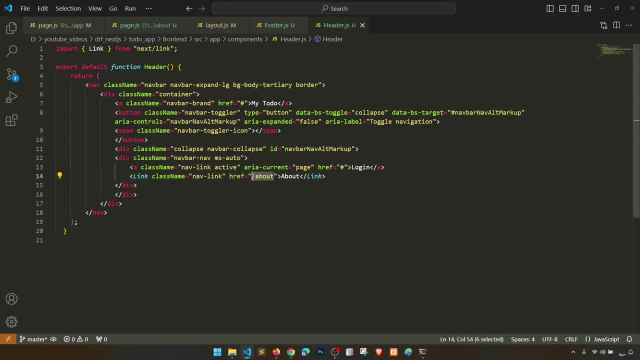 let's check it. while this is undefined, showing link href of about. if I say here, has them, why this is, this thing essentially looks to become of saying: Next, you have everything is going. So then, myänger of Voice and all, next, what we're gonna do is we're gonna say here: 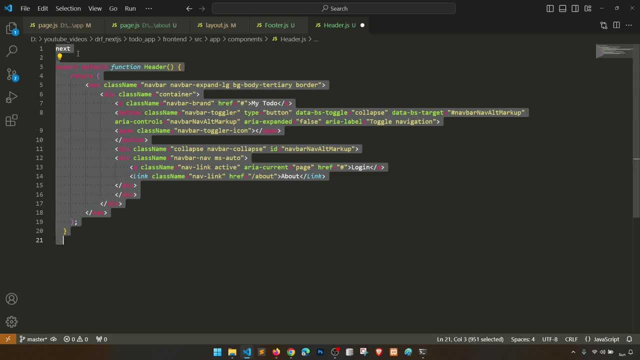 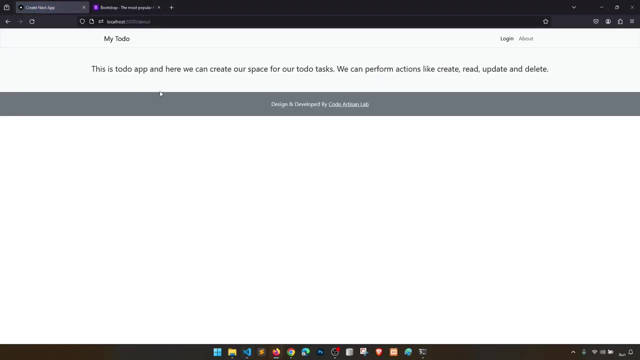 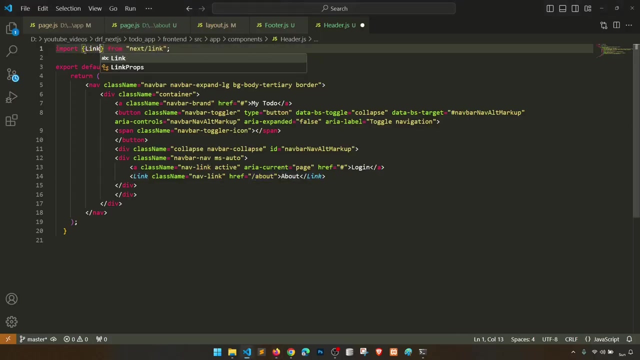 link bug, So on 100, rates. So we'll say one minute, we'll say link next. oh sorry, we need to import this like a different thing, different, with a different style, right? so here you can see that now we can say about before we are importing like this, like a constant or like a package, but now we need to return. 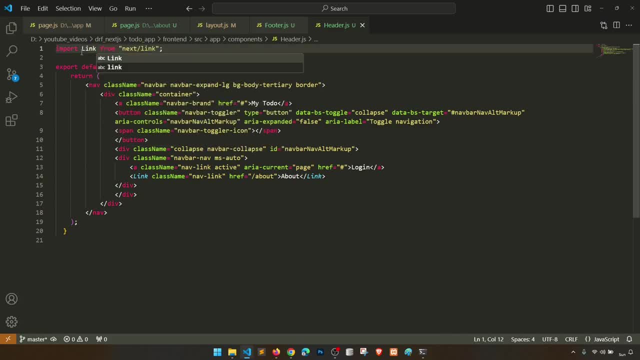 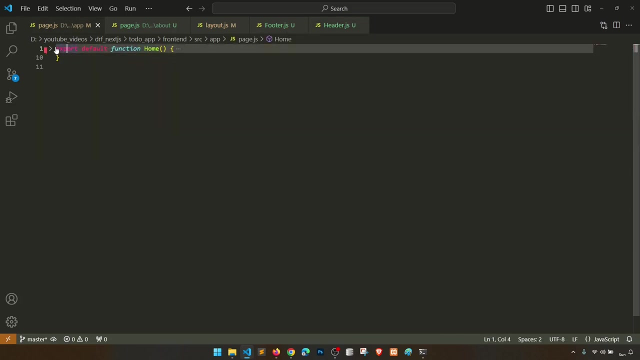 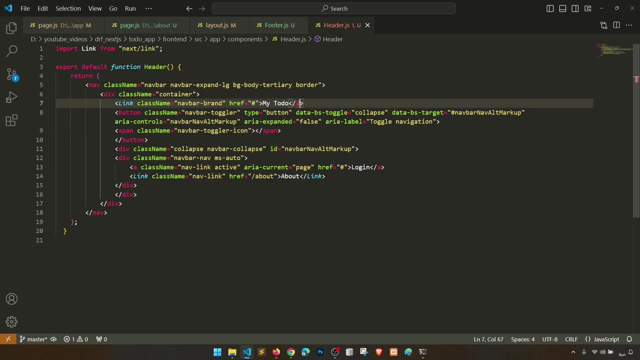 now we need to import like this, right, so now it will work. okay, so when we click on this, it will go to about. we also need to add this in our page dot: page dot js file. main page dot js file. so we can one, not page dot. we need to route this here. okay, with a slash, so it will go to the home page. 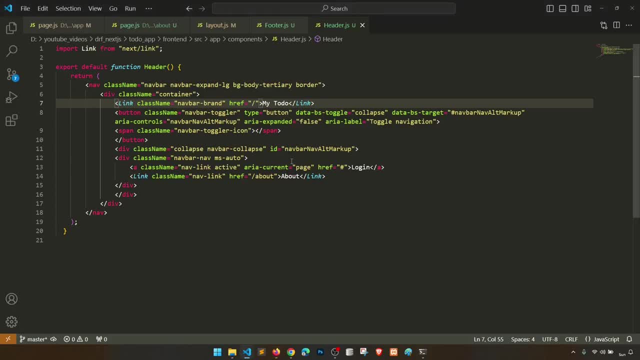 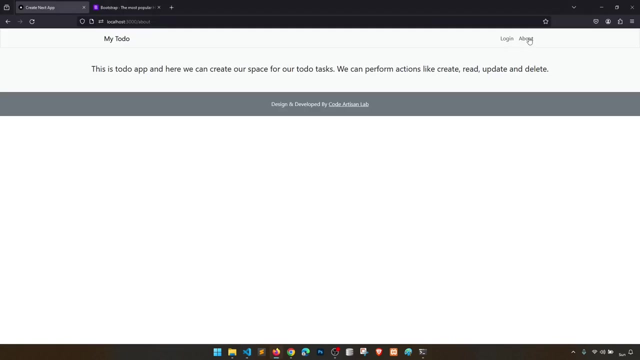 so home page about right. okay, so let's remove this active. okay, let's remove this current page. all right, so login- about right. so now what we need to do. when we click on this login, it should load the login page. so let's create the login page now. okay, so for the login page. 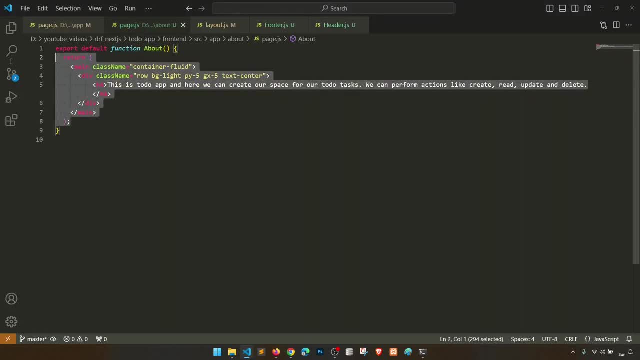 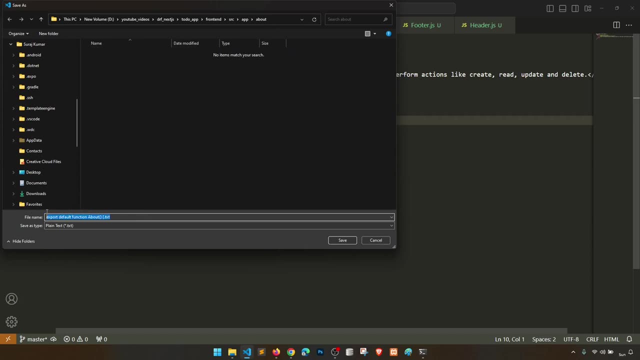 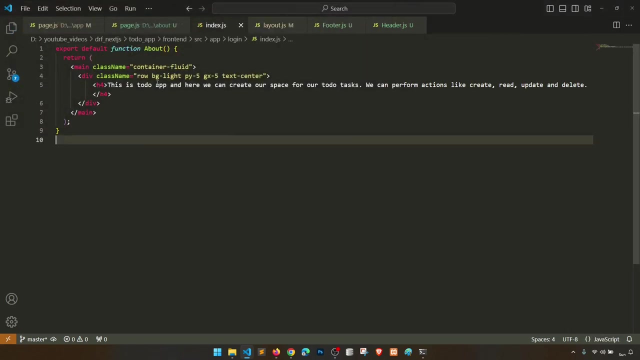 let's create and let's copy this one. copy this, paste here and we will say here: login. in the app we need to create a login and then in this we will say we will say this time indexjs, right, and we will say login. and in this we will just simply define. 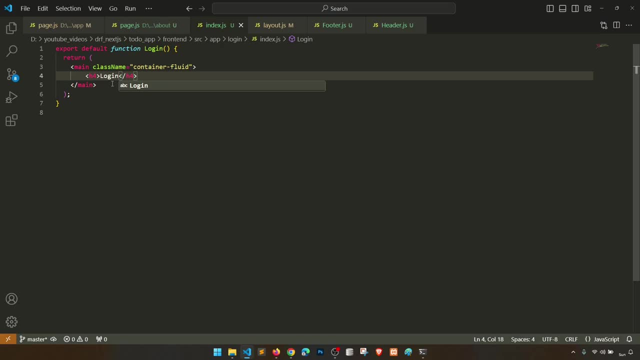 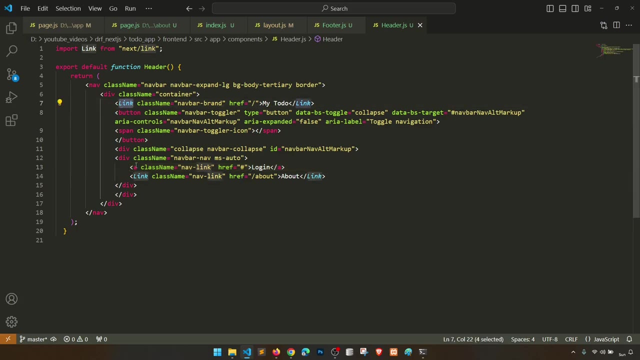 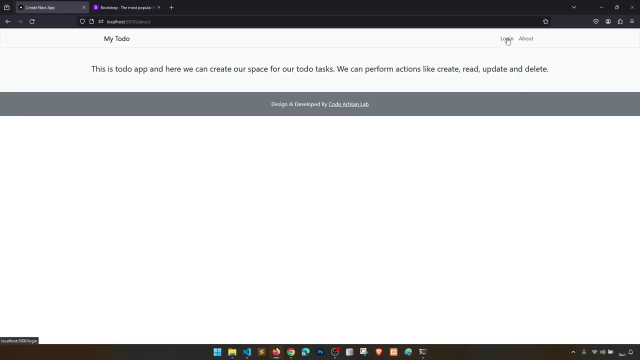 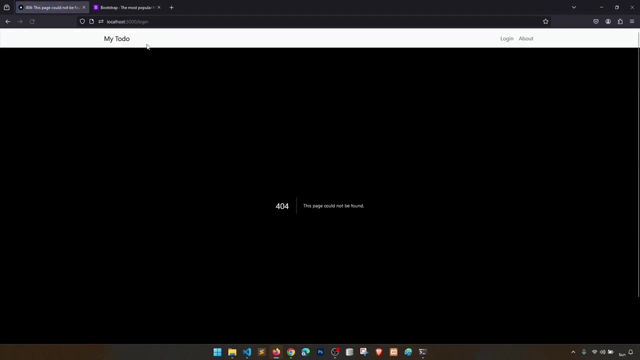 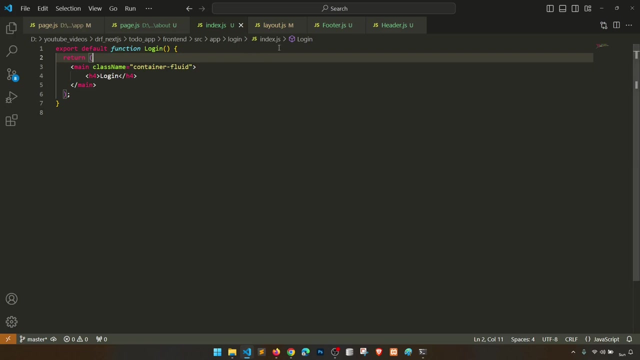 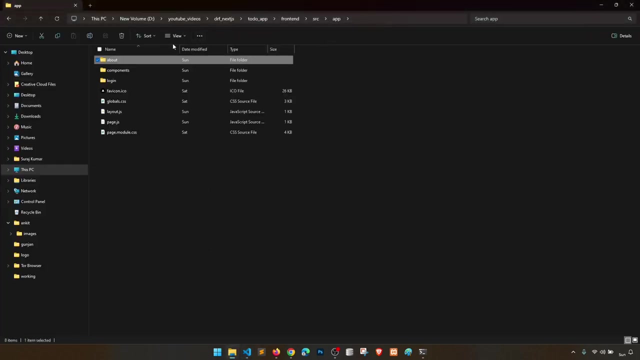 h4: login correct. and uh, from the header we will give a link: correct for the login, let's say login correct. when we click on this, it is saying: oh why, this is, it's not loading the indexjs file. login. uh, this is login. okay, let's rename this then. uh, home login, let's say homejs. 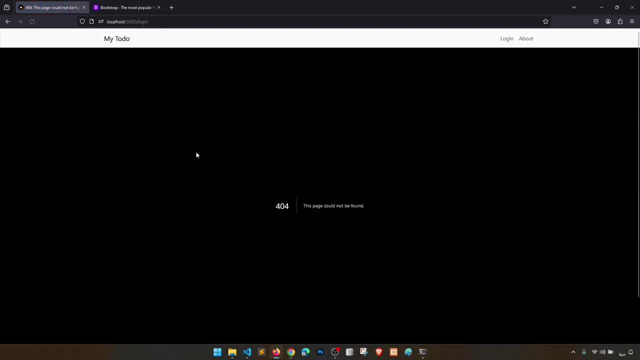 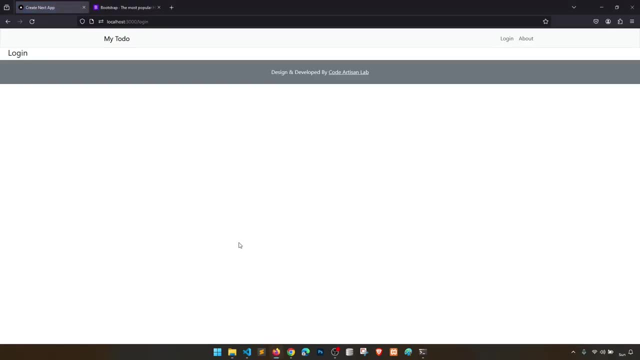 let's say homejs, now okay. then let's say pagejs, okay, now it means only pagejs. is login all right, then I think I have read something different. okay, no problem. so it means we we need for the pages router, we just need to create pagejs, right, but where we have 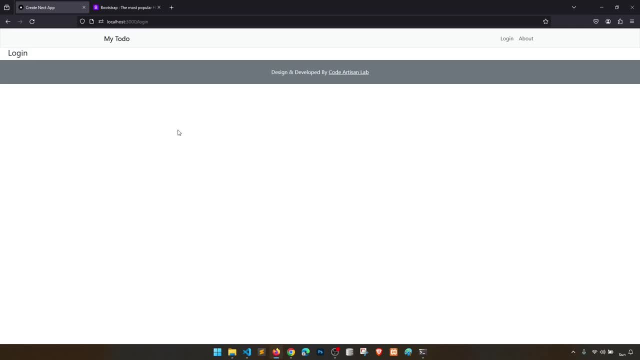 where I have read that home or index will also work. okay, no problem, we'll see that later that. uh, what was that? okay, so now we have a login. uh, where is that login? and entãoona vez que temos umiş것 cái że? okay, so now we have a login. where is that login? page? page about let's go to. 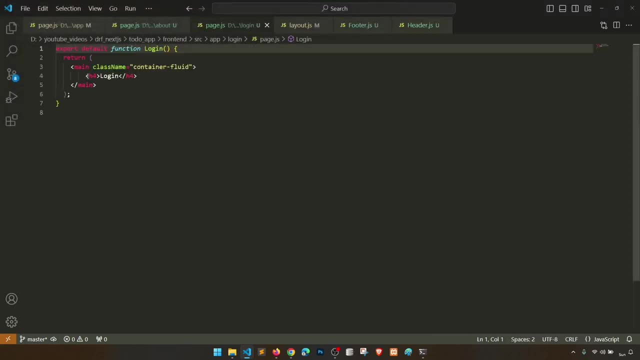 app. let's go to login, let's go to page start of it. so here, right. so now we need to create a container right, and in the container we should have row right, all right. so what we need to do? we need to create two columns, like we define in the. 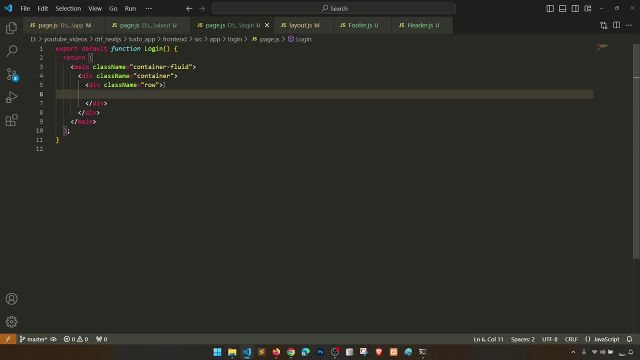 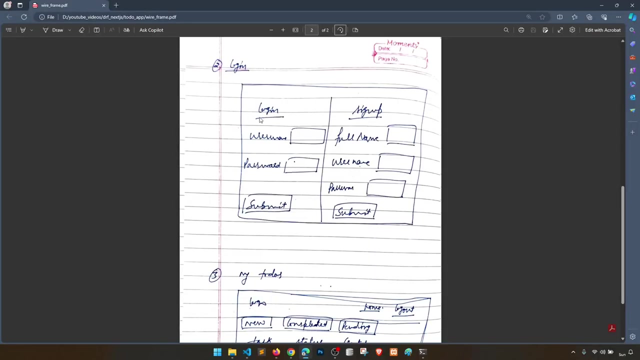 like we define in our, in our app. let me show you. let me show the app one minute, okay, so in my rough wireframe, you can see that I have created a simple layout. you can see that I have created a simple layout: login and sign up in a single page with the two columns. so let's create this. 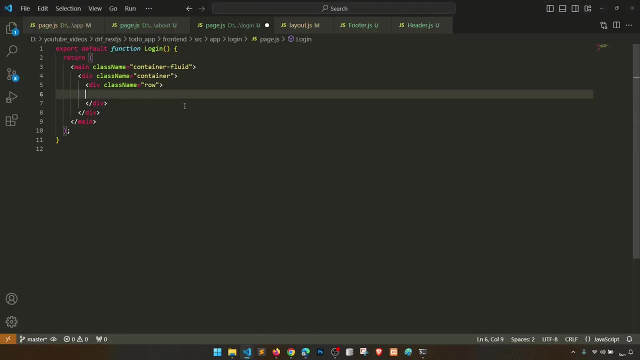 kind of thing, right? so I have a row right and in this row I have a class. let's say call six, what is this? so call six, and I will say call six now again. so we'll say login and here we will say sign up. great, okay, so sign up and log. 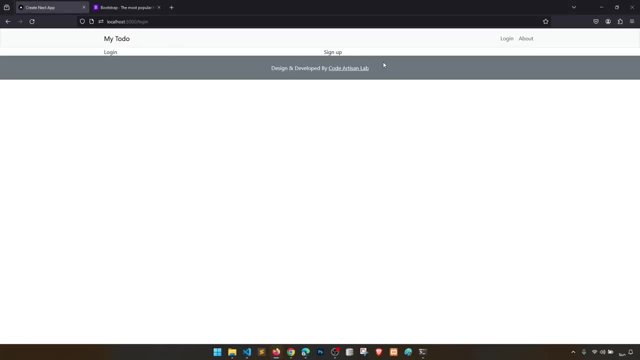 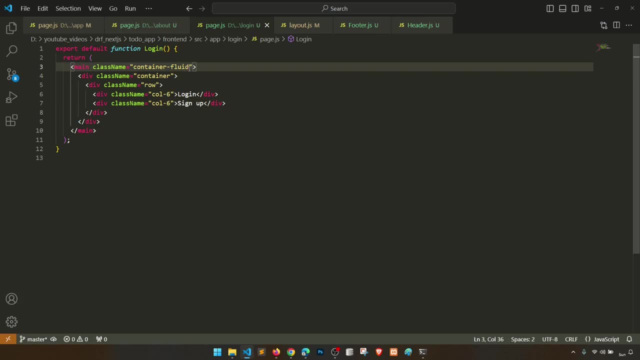 so let's go here and you can see here, sign up and log correct. we will give for the container float, we will give some for is vertical padding, this kind of thing, and in the container also we will say text center, text center. let's give text center. okay, let's create a form. we will 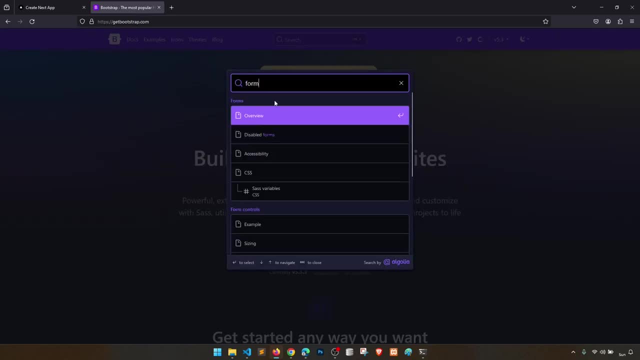 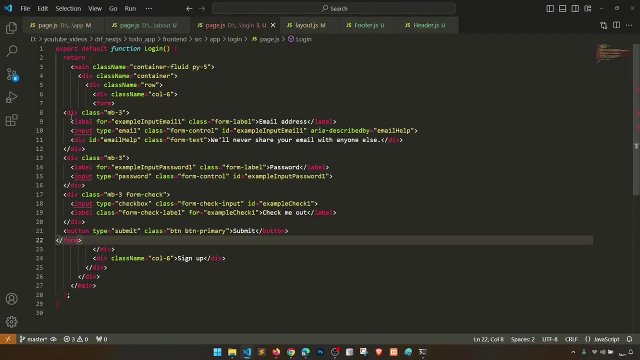 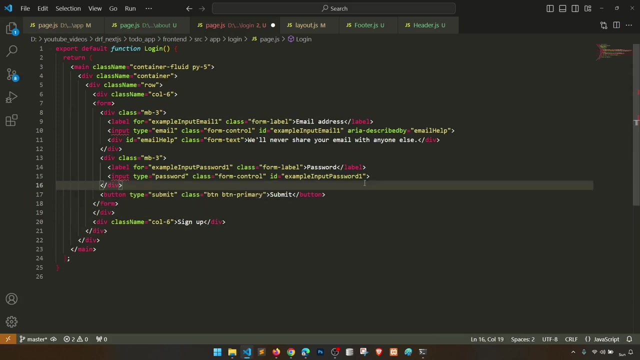 see that. so for the bootstrap form will give overview. we have this kind of thing so we can copy this right. so we are creating a simple thing, so we don't need the remember functionality. so I'm going to remove this and we need to close this tag. 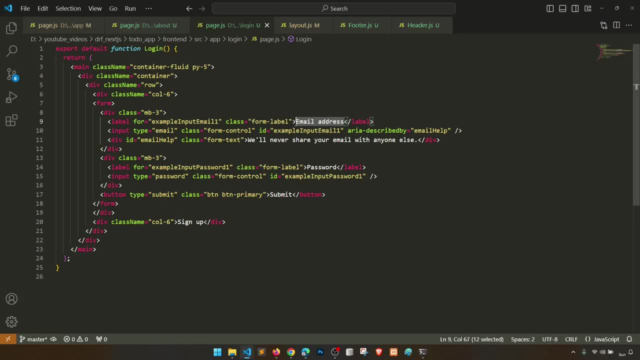 right, so yeah, so we are going to add email address, so we'll say email and remove this line. type email is correct. let's remove this thing. will keep it simple email and password. so let's remove also we. let's keep it a simple password password here. ID will give a email. let's give email here and then we. 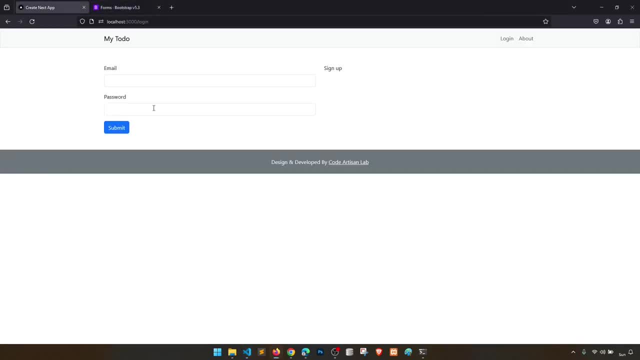 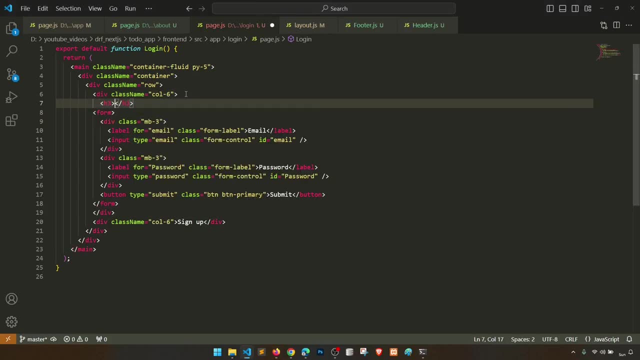 have some. ok, so let's see here: email and password: right, so we can give here one more again. correct? so this form will go, this line login and we begin. give elle填 right so we can follow all the individual as already agreed right to which is I'm going to write here. so, etc. whatever you want to stop later here. 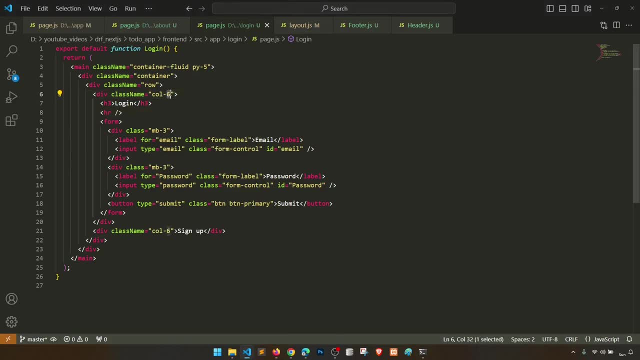 together, uh, so we have given he's right open. we already wanted to have a paper. uh, and tree test and dé телефон, you get reason to really attach. But I have. this is also five, but offset, offset. you can say one, so offset two. okay, all right, so we can copy. 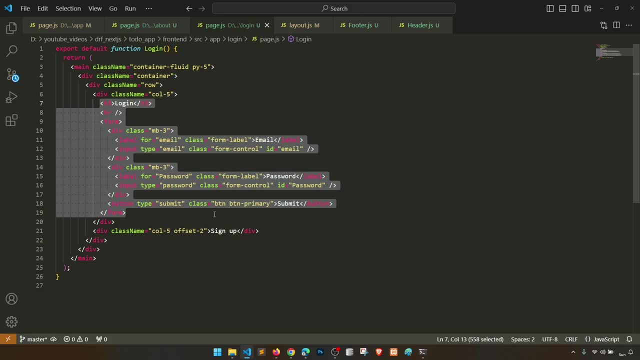 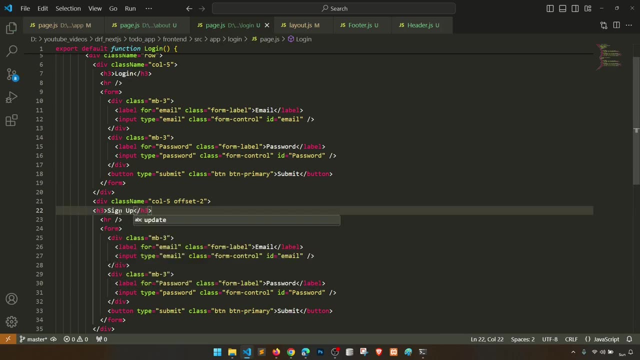 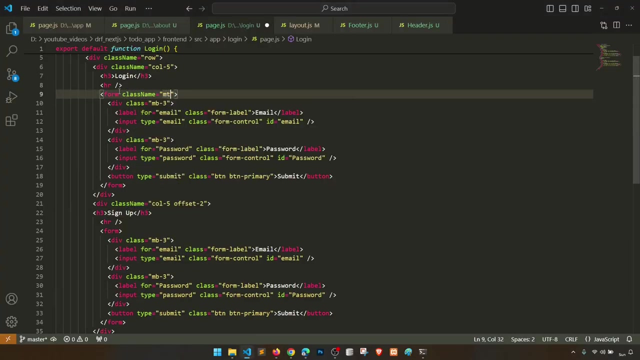 the same thing, same form here from here to here, okay, and here we will say: sign up, correct. so login and sign up and we'll give some margin for the form margin. top three, you can say correct, and we'll say class name three: all right, so margin. 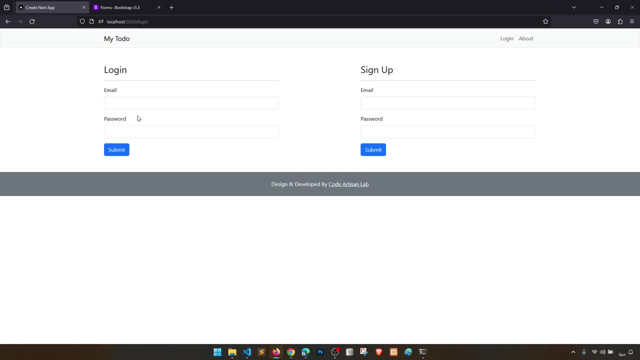 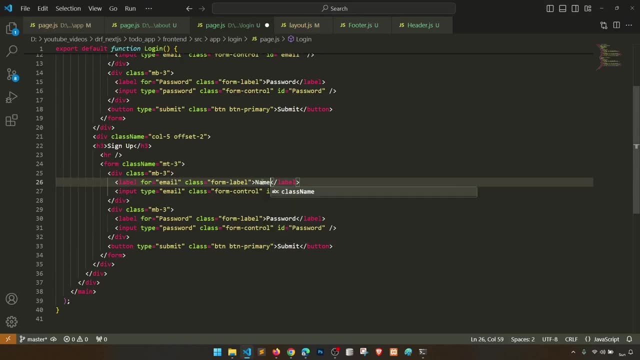 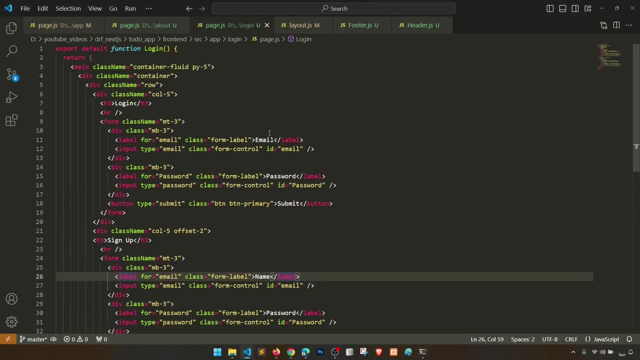 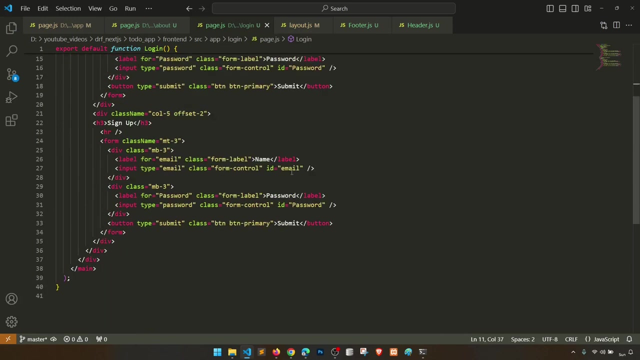 okay, so let's discuss about the login form. so email password is correct, right, and for the sign up we need to add name. uh, what are the name, username and password here? login, username and password, so let's say username. then, if we have username, then let's say username. okay, so username and. 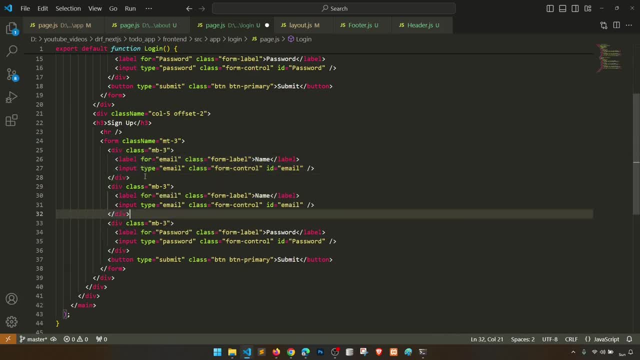 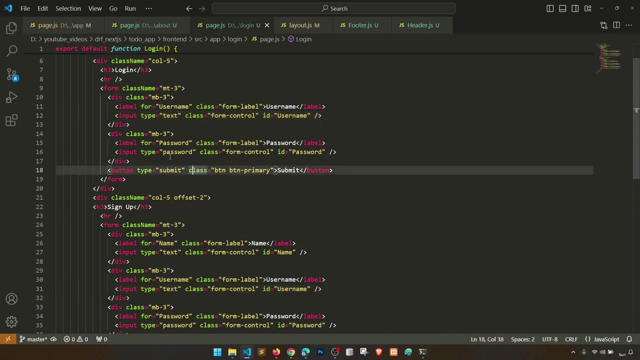 password. so we'll copy this name and paste here and we will say username, correct. so this one and name will be name, name text, so name and this will be text and this will be also text and for this will be also text, correct? so username password. submit name. username password submit. 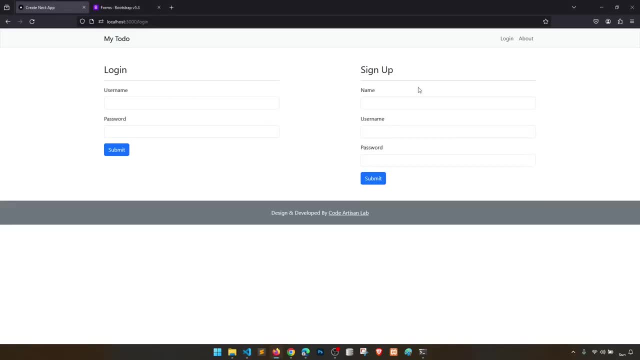 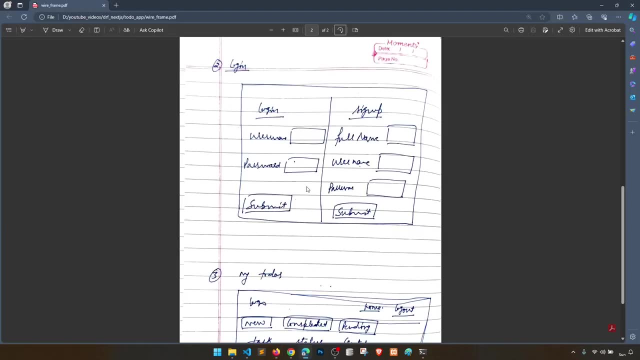 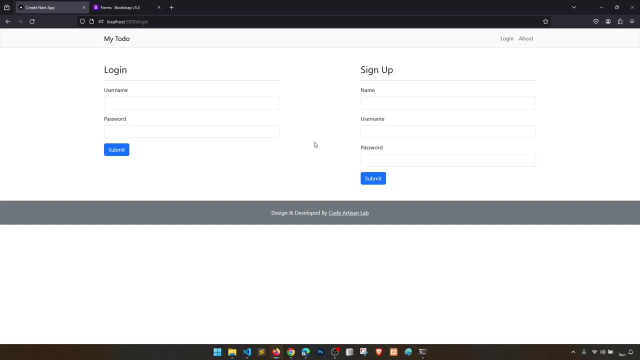 right, so this is our login form, this is our sign up form. great, so we have created this, this thing also. now we need to create this template, my to-do list, right? so after login, after login, user will see the to-do list. okay, so let's create that template, all. 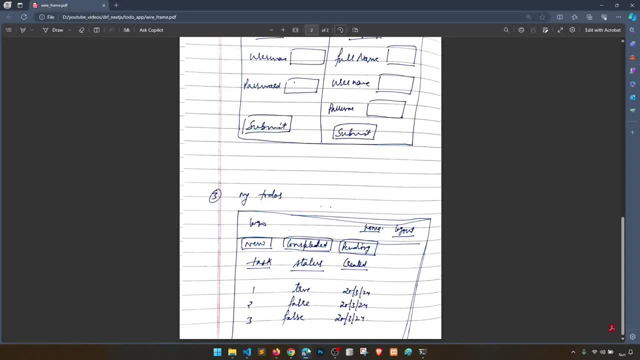 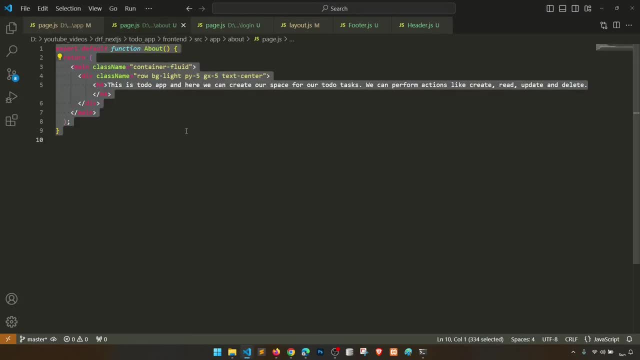 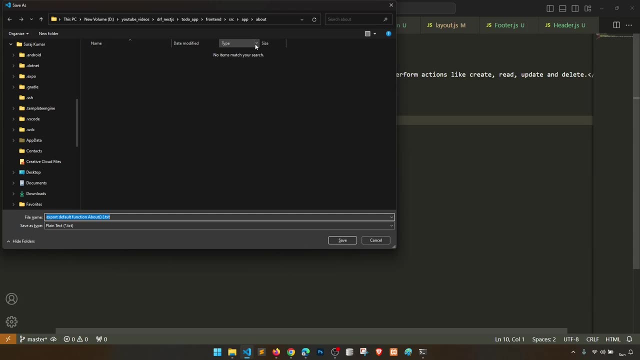 right, so we need to create the this one. is that, yeah, this to do. so what we will do, we have about us. we will copy this, paste it here and we'll go to: okay, so we'll save this in the app. we will go to here and we will say: my to do's my to. 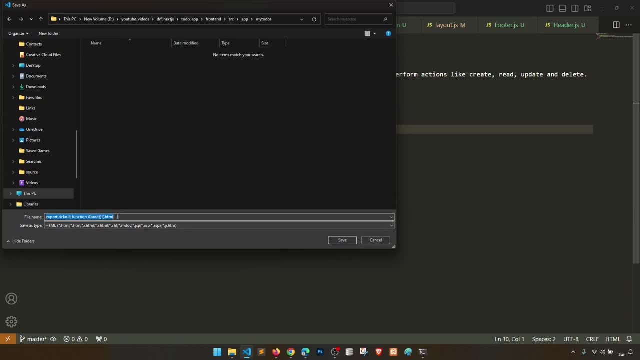 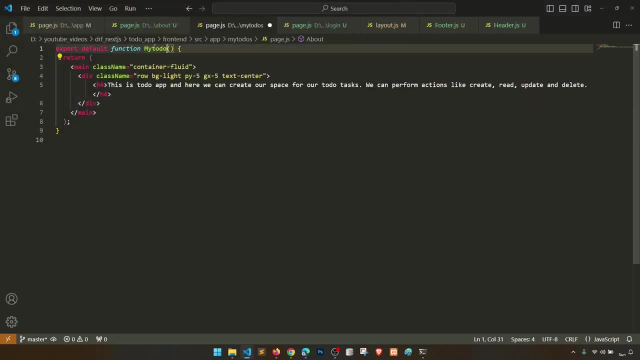 do's right. I mean this my to do's. we will create page dot J's right, and here we will say my to do's, okay, and then in the container fluid we have a lot of things. so let's remove this and let's create a file. 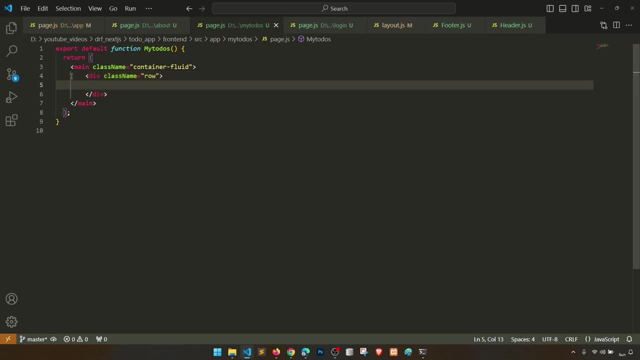 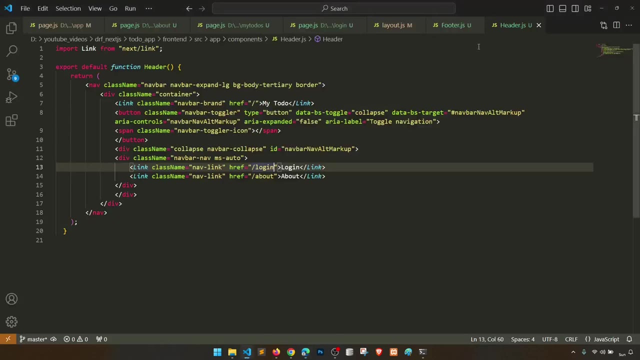 festive great will create a row right and let's set the router also. so for now we need we will just create a link in the header because we are not implemented the authentication. so let's say my to do's right. so here we will say my to do's great, and then we have my to do's. we have a folder here. 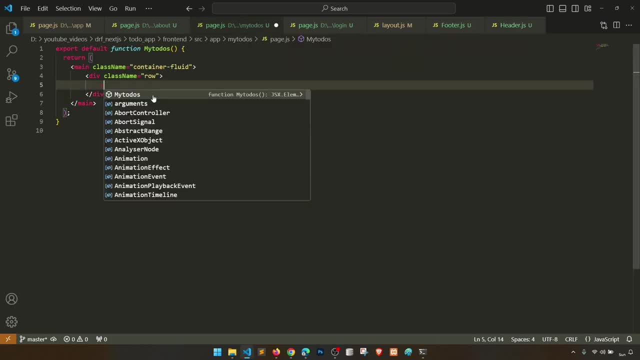 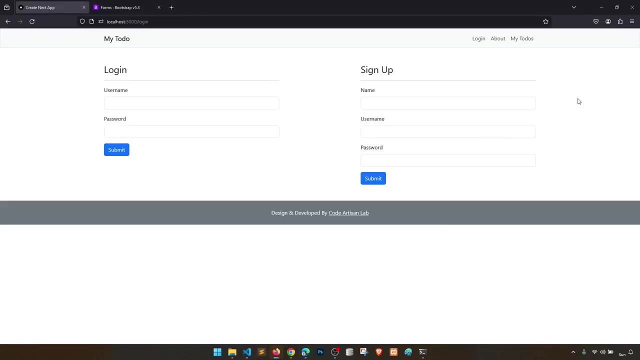 and in this we have this thing okay. so let's say we will say here my to do's great, and let's go here and you can see this link. this link will show only when we logged in, but for now, because we are just designing the templates, so I have 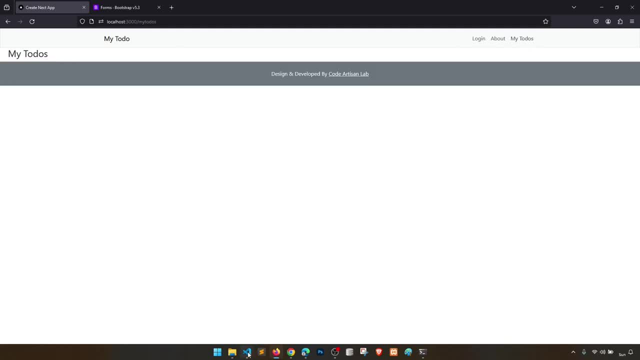 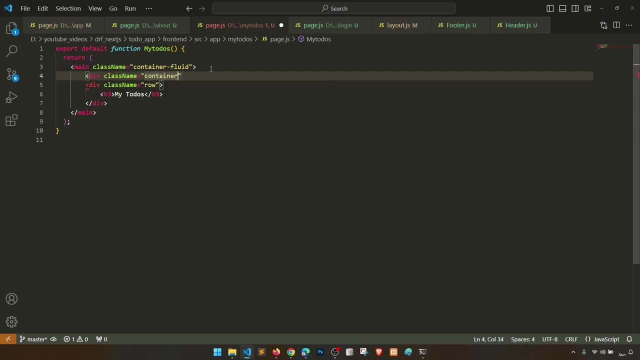 added the link. so when we click on this it is loading the my to do's right. so before that we will create a container, right, and then I will go here. so let's go to. okay. so now in the container, float fields into the same thing will give. 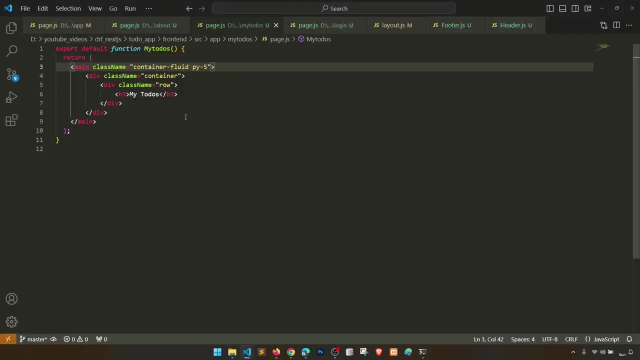 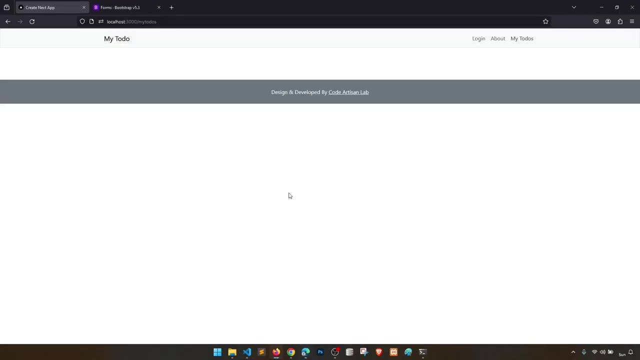 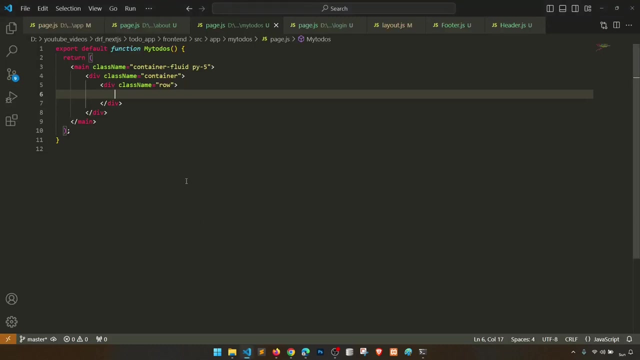 some vertical margin, vertical padding, okay, so in the, might you do? we have a table right, so you can see, here we have a table. a new like this task, status created those things. so what, we will do so in the container, no need to create a row- we will create a table right and in the table we will give table table. 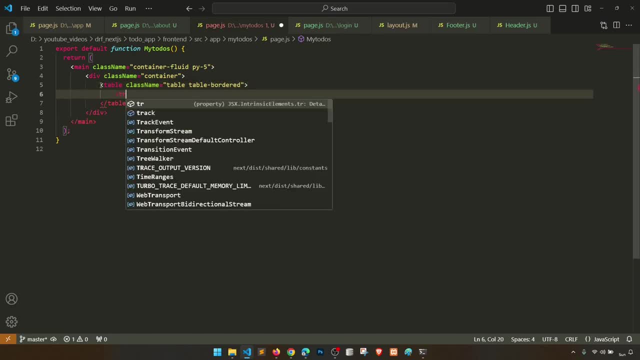 border right, the first row is heading. So we'll give a task, this, and then we will define here the status right, And then we will define here what we will define status, and then created, created date, or we can say created ad right. 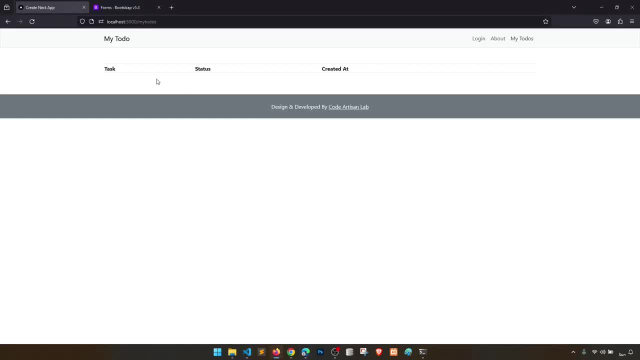 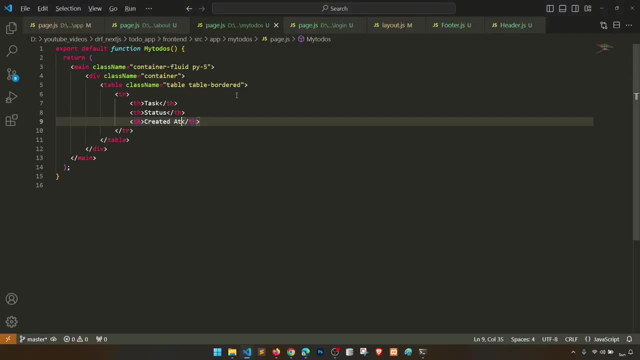 Right, so when we go to this then it is showing like this: right, So let's go to table. table border. OK. so we have this thing and in the table we can say he had, so he had the notes that table heading right. 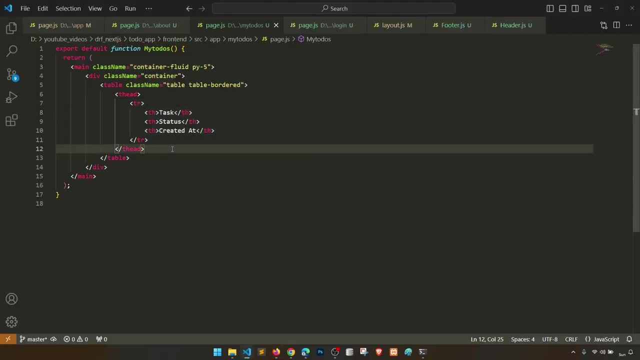 So this thing OK, and then he body right. So in the T body Let's define a constant data equal to array of data. In this array we have, let's say, id 1 and task. let's say task is. we can say task is item 1, right. 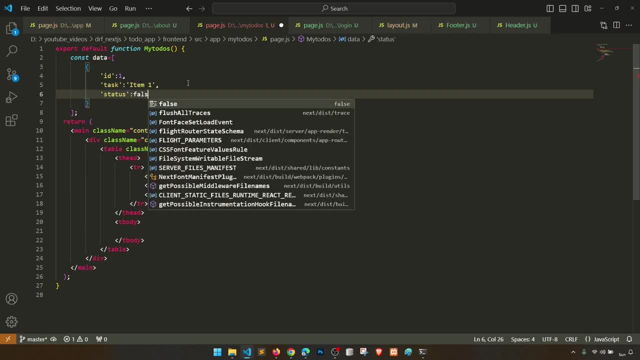 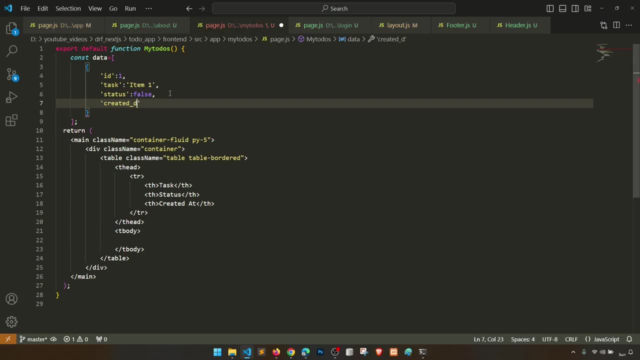 State Status: false right And created at we will say, 23,, 24, right, So this one. So we can do the same thing here, Copy paste And we'll do 2 here, 2. 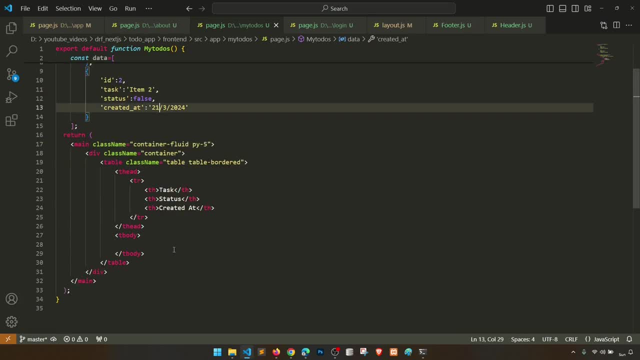 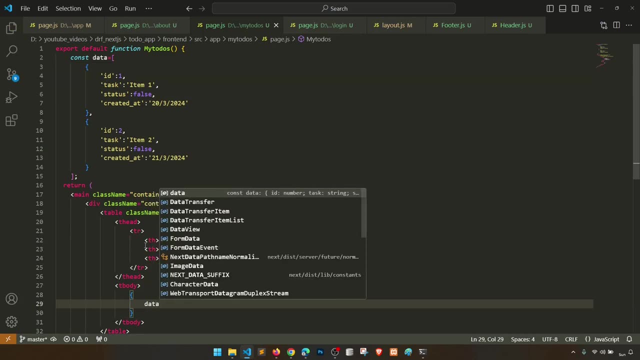 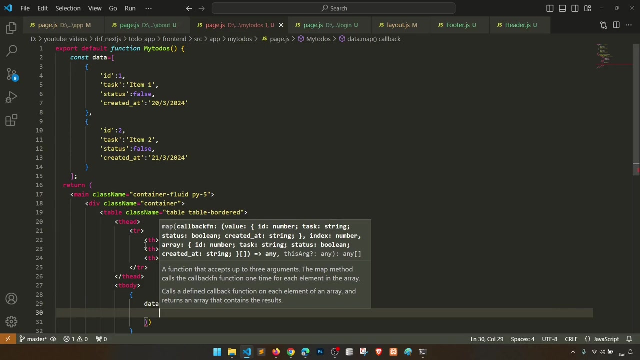 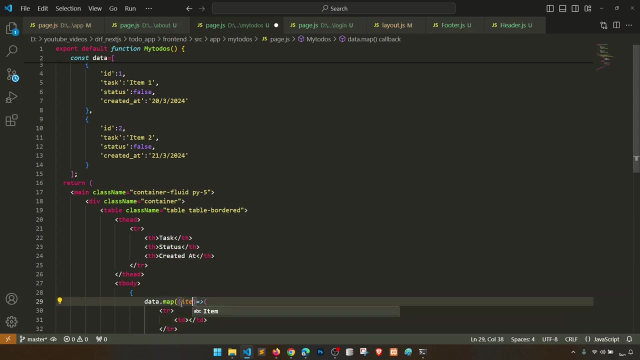 This is 1. Right, And here we can do the simple thing: Data Datamap, And in the map we can return the row, And in the row we have td And in this we have item and then index, right. 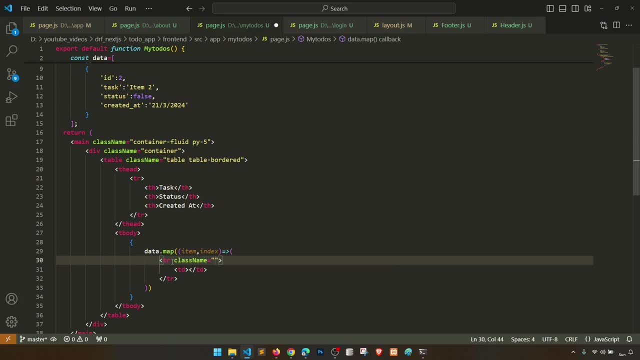 And because it will not, it should not create the sorry key error. so we will define index, sorry index, and this will be our task. So tasktask, sorry, itemtask, sorry, So itemtask. and then status. 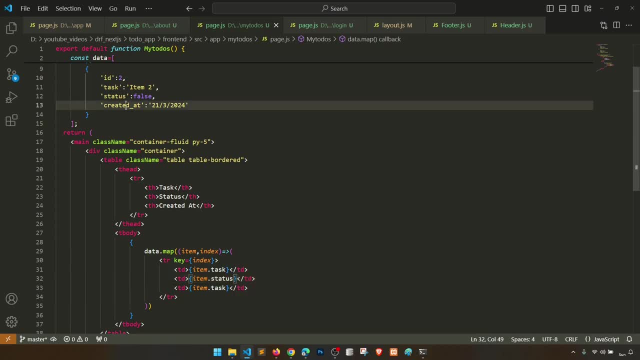 And then create, And then we will return. So we will return itemtask- sorry, itemtask- And then we will return the status that we created, at right, So you can see here status showing this one. Let's define one more thing here. 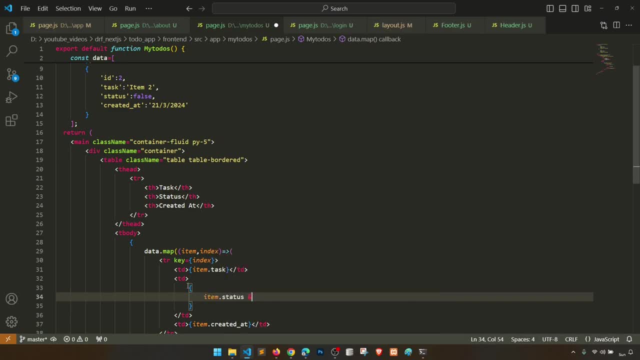 So we say itemstatus, then we will return Okay, So we didn't added the let's say completed, Okay, So we didn't added the let's say completed, Okay, right, and if not, okay, we can do one thing: if this then completed, else pending. okay, so it. 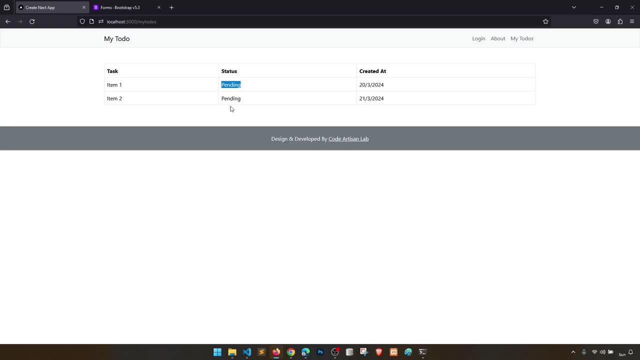 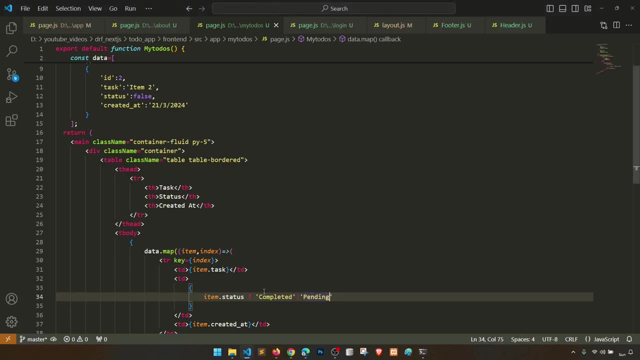 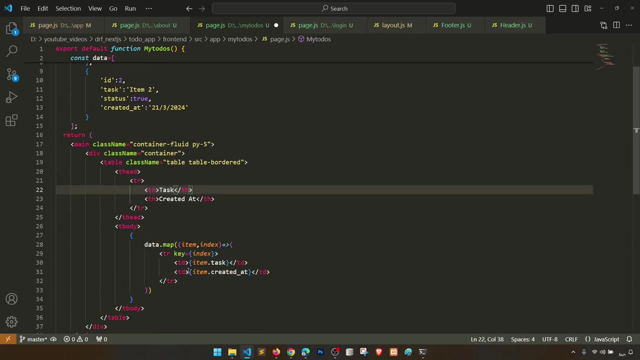 is showing pending now. later we will add the icon correct. so task status and pending correct. okay, let's do true, right, and this is showing completed. let's add here item one. let's remove this one. actually, let's remove this status. we will do something in the task, so what I will do? 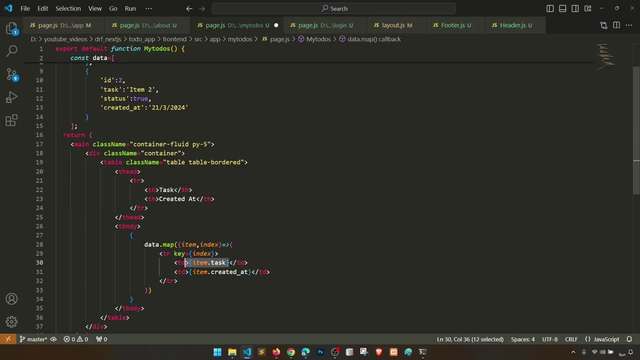 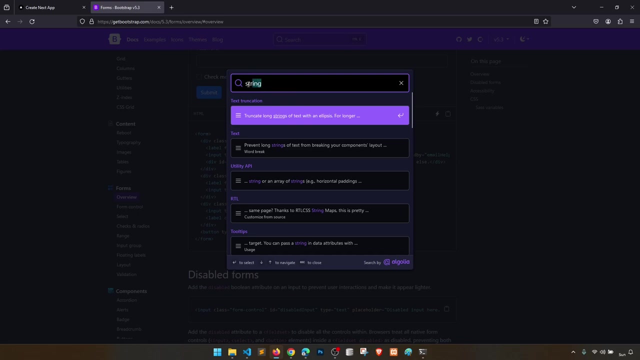 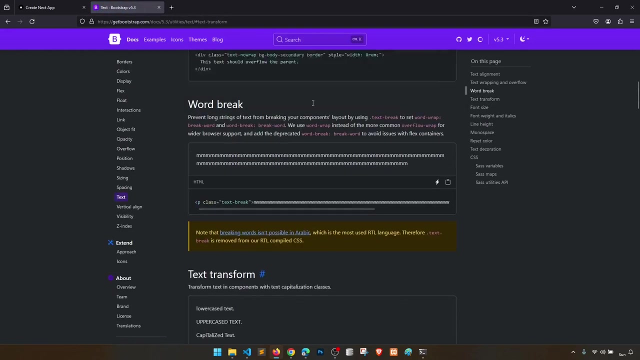 let's do one thing here. okay, so what we can do: item dot status. true, then we will do one thing: span, not sure what is the strike tag, strike, turn it, or you can say text text, transform. okay, so text, text, text text. what we can do with text. 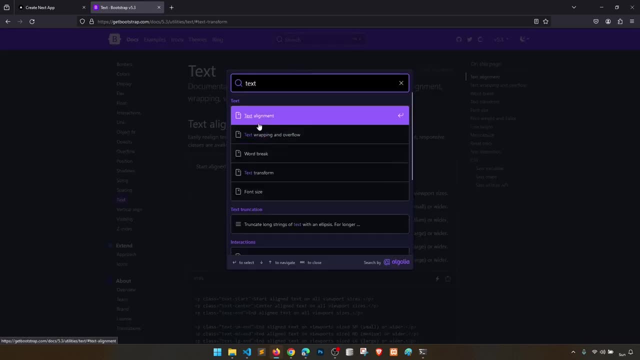 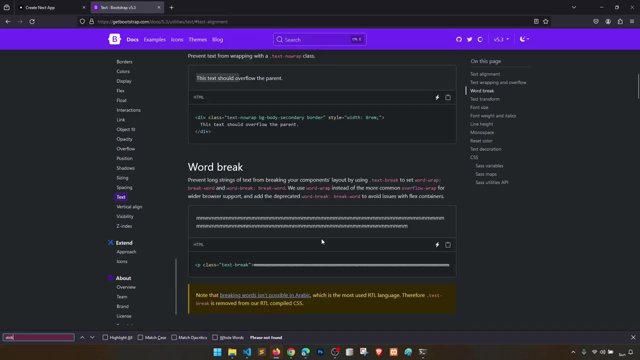 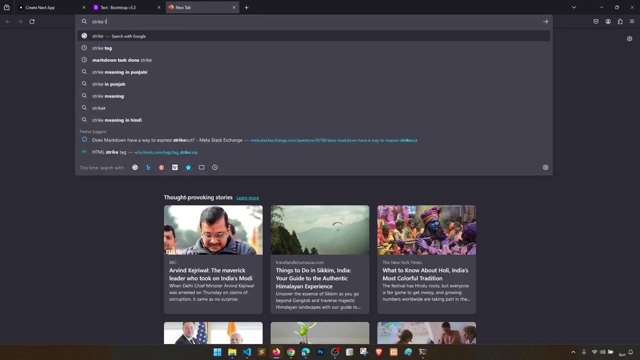 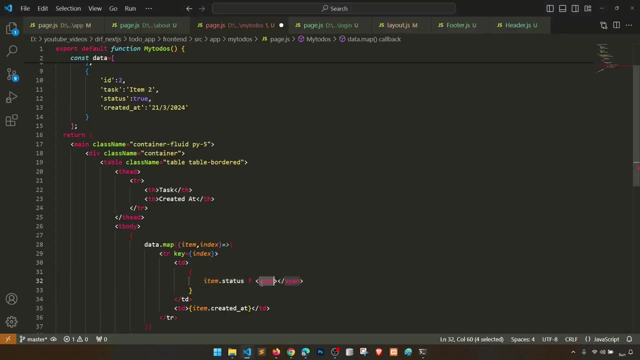 text align. okay, I want to strike the strike text in HTML. okay, so we can use the s tag. okay, so if this is true, then we will add the s And in this we can say item dot, item dot, task, Correct. So if you go here, what? Oh sorry, Sorry, sorry, sorry. Or if not, then we will simply return the task. 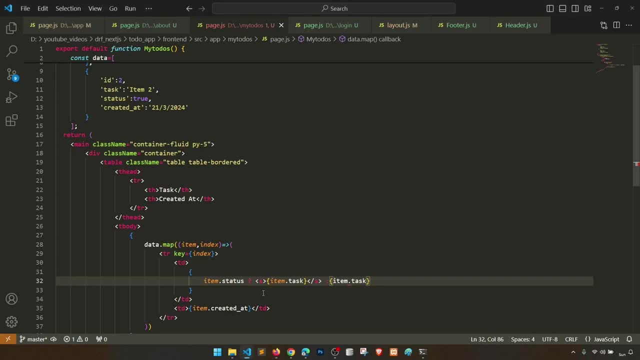 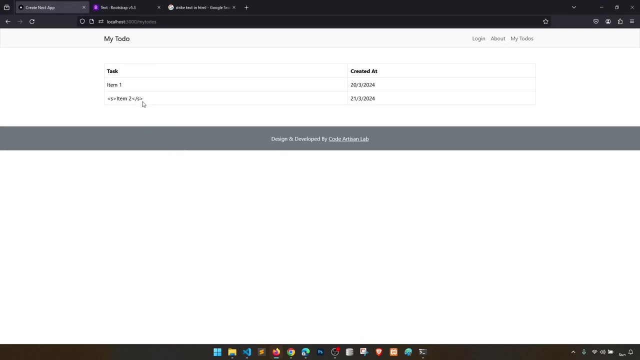 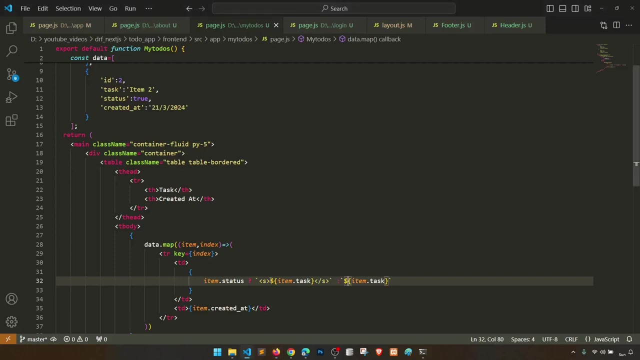 So why this is not showing here? Because this one minute. Okay, let's say dollar, No, not dollar, This escape string, And then we have this dollar symbol. It should work now, Yes, but s tag is not working. Okay, no issues, But we will. we will see something different, But I want to. but you understand that what I want to. I just want to strike this tag right. So not sure why this is returning this one. I want to return the strike text if it's completed, right. 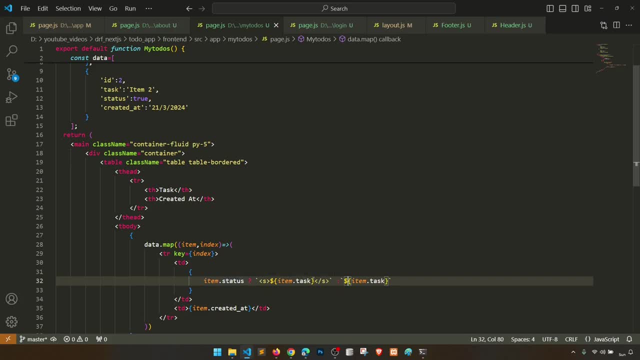 But we can do one thing: If this is state, we can just do one thing: Copy this and paste it here Right And here we can see class Right And class in the class we can say: item dot status. Oh sorry, Item dot status. 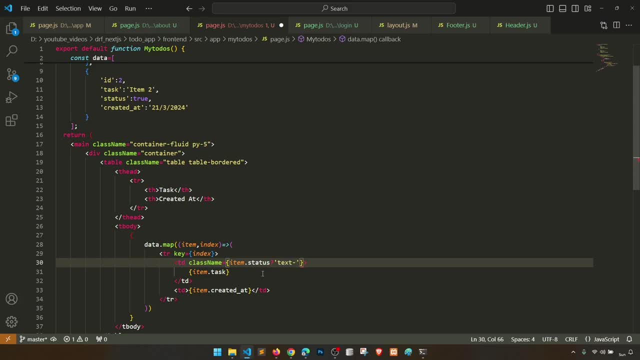 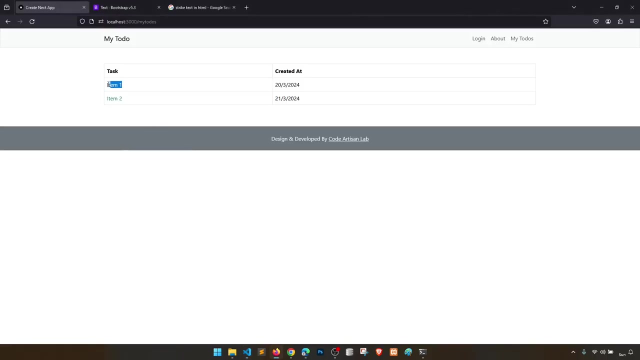 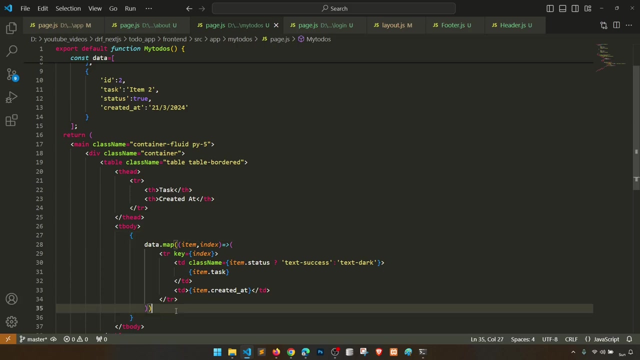 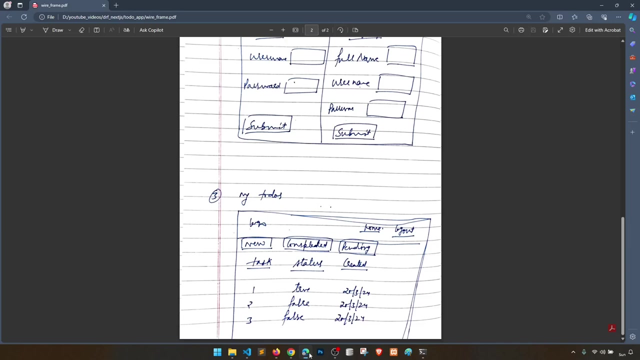 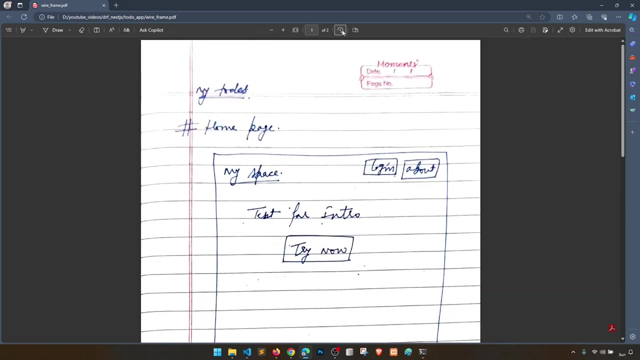 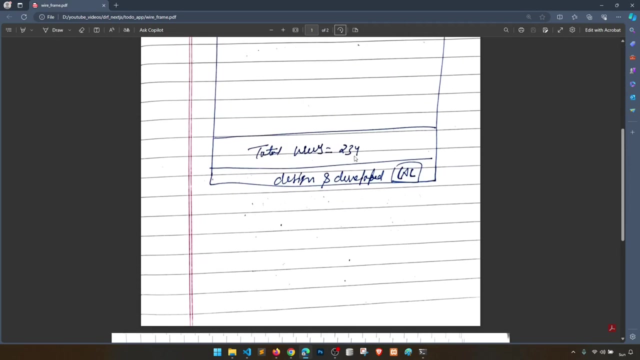 Then we will see something different. We will say text green, else text dark. Right, So if status, then task text success. So success and this stock. I will add the strike tag also. But I will see that how we can, Right, Okay, And if you know the how we can add, then please add in the comment section, Okay, So here we have the task and created, Right. So I think we have completed all the templates. What all? we have three templates, So I think we have completed. Oh, one more thing We need to also add here: Count the visits. So before the design, and well, we will also need to show 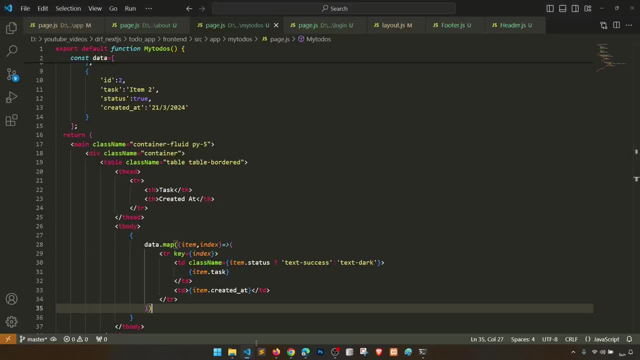 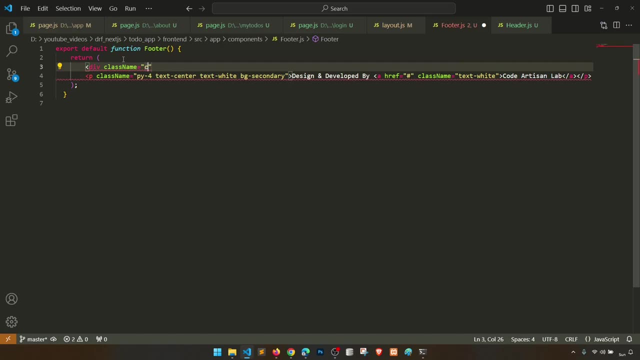 uh, total users. So we can do one thing in the footer. Uh, we can create a row Right, So we can create a container. actually, in the container, We can create a row, And in the row, uh, we can create two columns called six, And in this we can add this one. 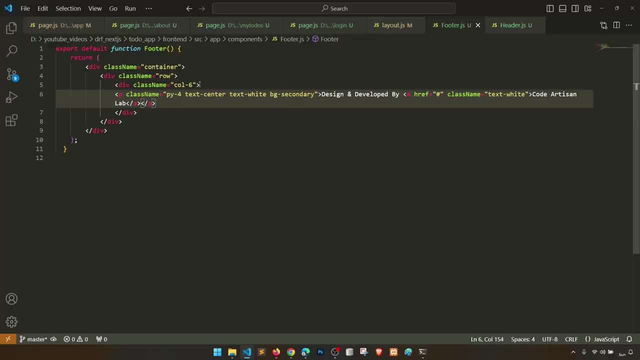 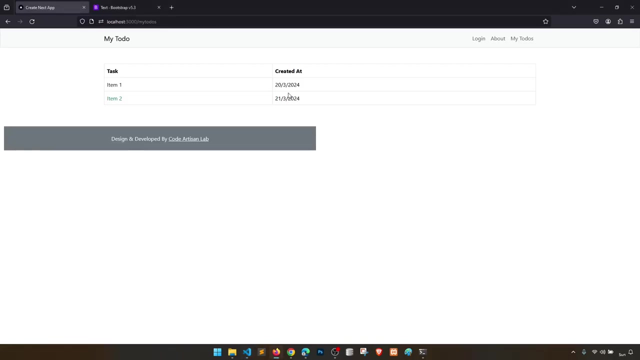 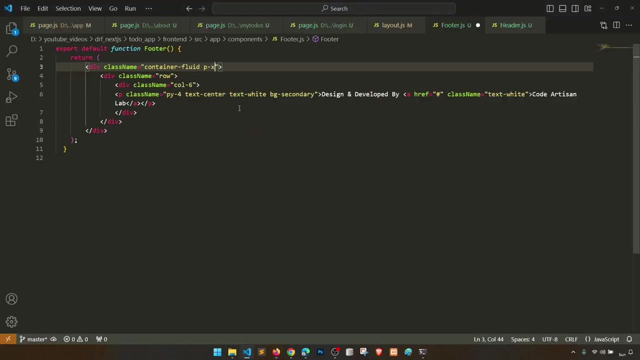 right here. so if I go to this, okay, nice, so what we need to do? container flute, container flute, and then we have to add five container flute. we can't add in the container flute design and developed. we need to do something different. okay, so if I go to give padding X five, oh, leave it now. for now we just need to add the. 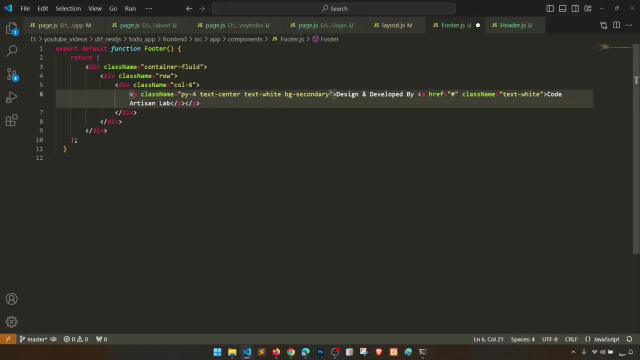 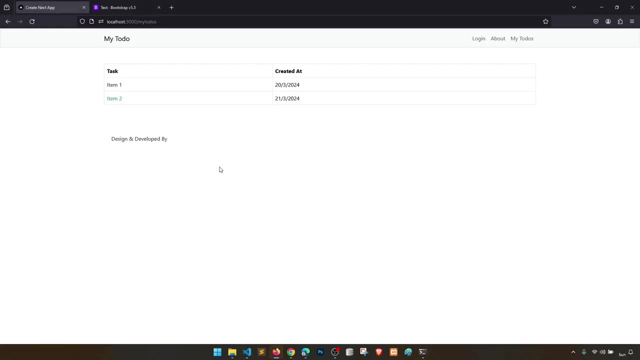 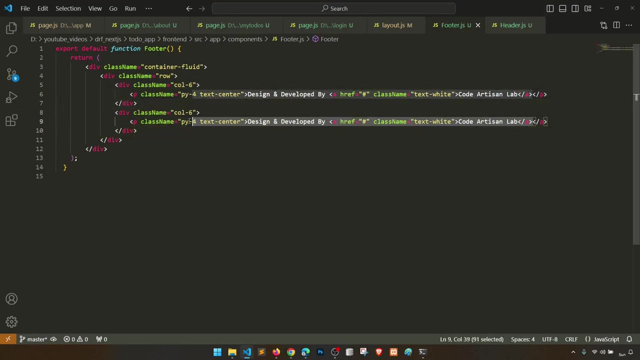 text. so what I will do? I will just remove this BG background, right so text. let's remove this text also. so design and developed by: and one more column. one more column. we will say: let's remove this anchor. we will say: total views equal to and we will show in the code: 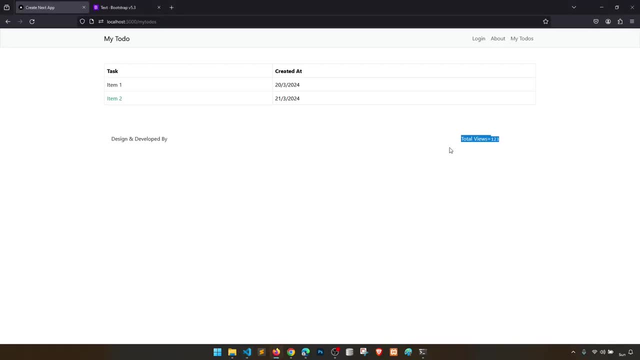 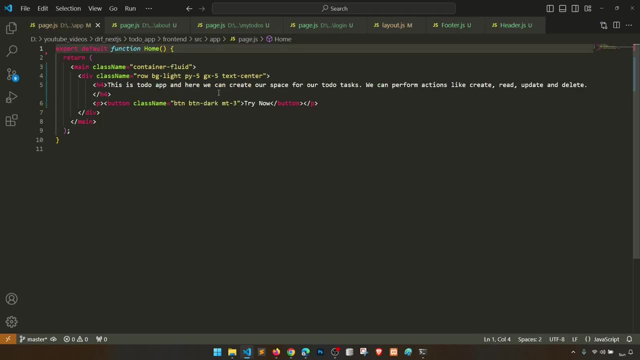 form. so total views this correct. okay, so how we did for the page. okay, so here we have container flute, then row, and then we have this. so where is the footer here? okay, so this is five. so not five, let's say three, right, and then BG light, not light, let's say secondary, and text should. 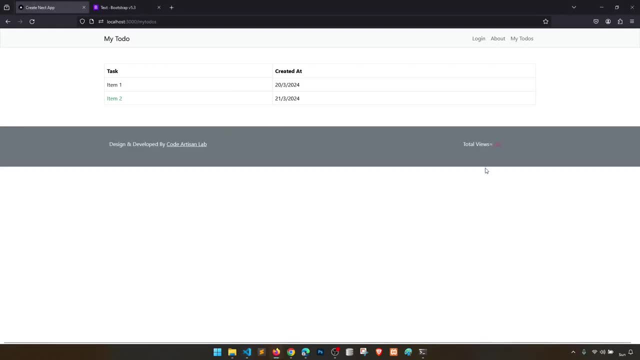 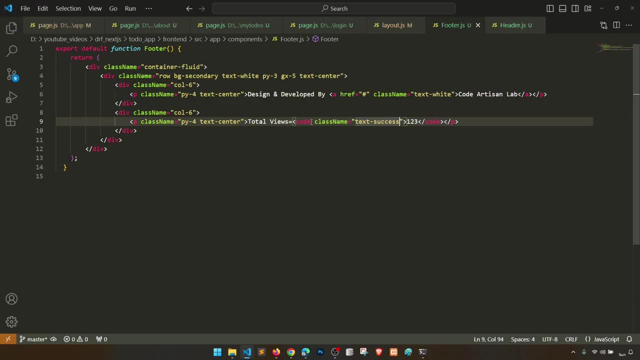 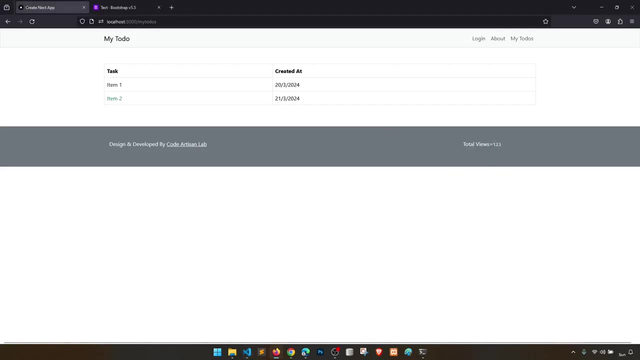 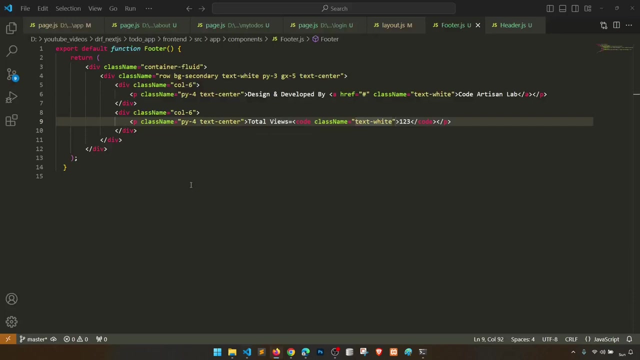 be white, all right, and this text also should be let different color text success. success is not showing. we need to add: okay, so total views. is this design and developed? okay, so this is working right. uh, text center, text center. let's- uh, let's remove this, because we have added in the text center here. 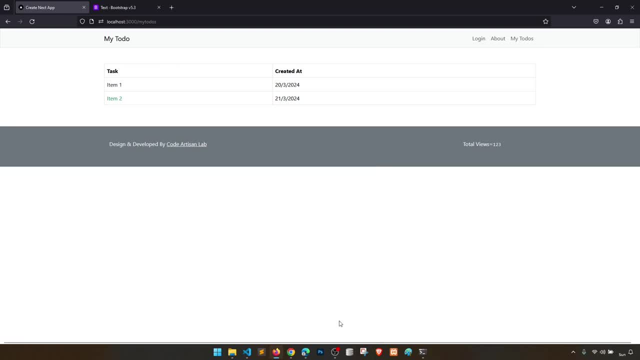 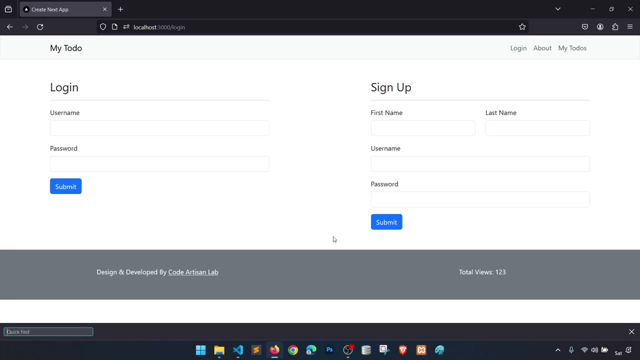 all right, so we have. i think we created the layout. now we need to work on the back-end system, right? so let's work on the back-end system. let's work on the apis, right, so let's start to work on apis. okay, so let's start working with the api. so we will start from the sign up. so what we are. 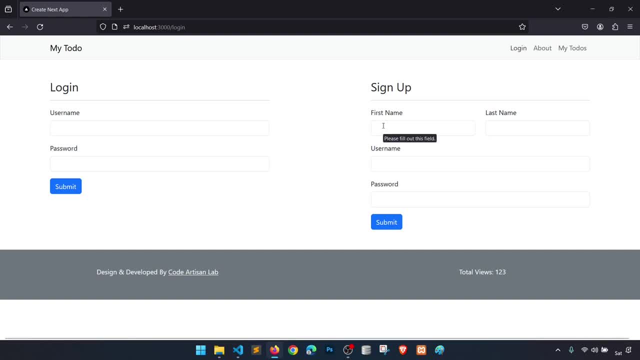 going to do? first of all, we will register user right and we will create the corresponding token for this user right and we will also show the messages that user is signed up or not, or if any error, that we will show and after the sign up we will proceed to. 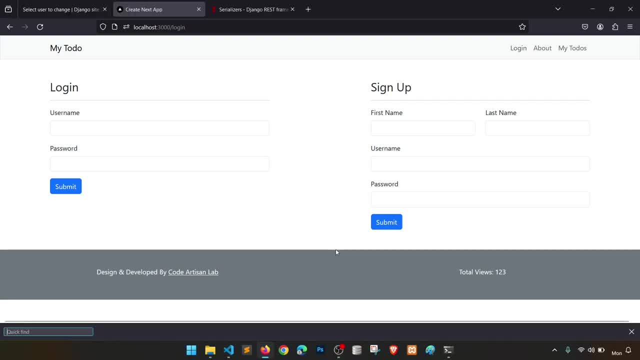 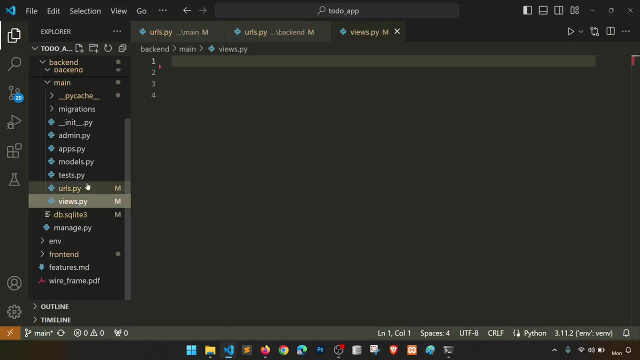 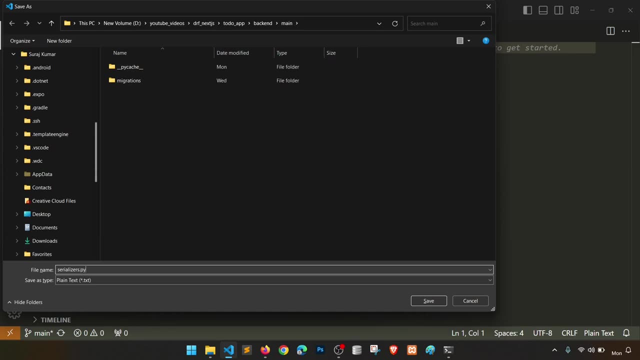 log. right, so let's start with the sign up. okay, so first of all, we will work on the sign up. so what we will do? first of all let's create the- uh, let's create one file called serializer, right, so what this serializer will do? it will convert our model data to proper. 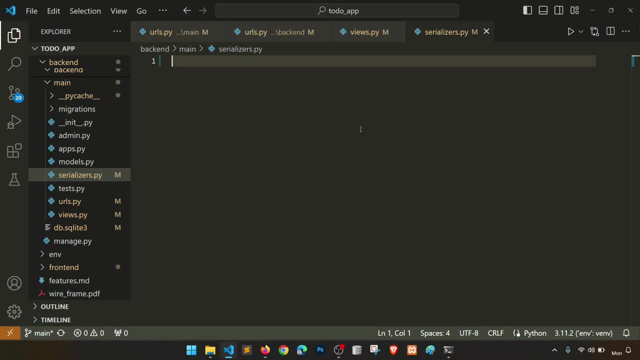 uh, json format: right, so you can say: this is same like a form in a normal django website, right? so this is the same thing, uh, we do in a serializer if we are working with the api, so it will validate the data, uh, it will uh accept the request. it will send the response. 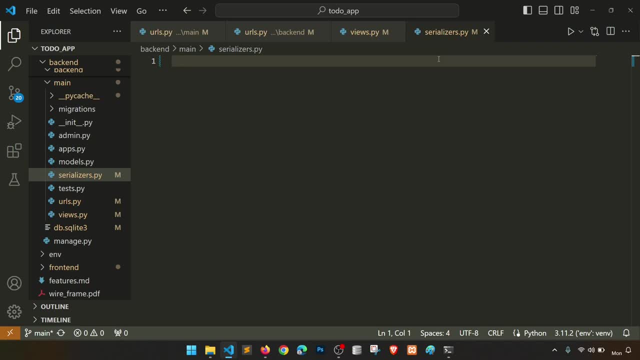 right from model to a client, or you can say two views, sorry. so we will create the serializer for the user model. so, as we know, django comes by default with the user model, so we will use that model for our sign up and we will create the serializer. 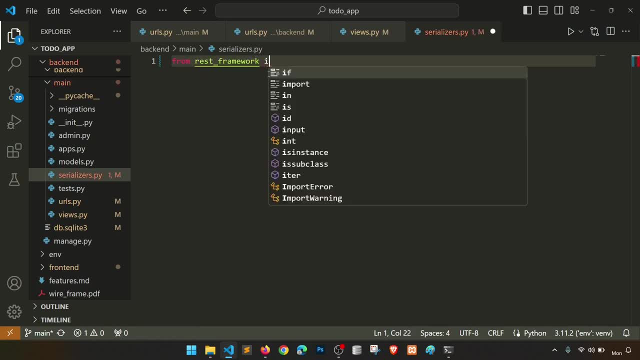 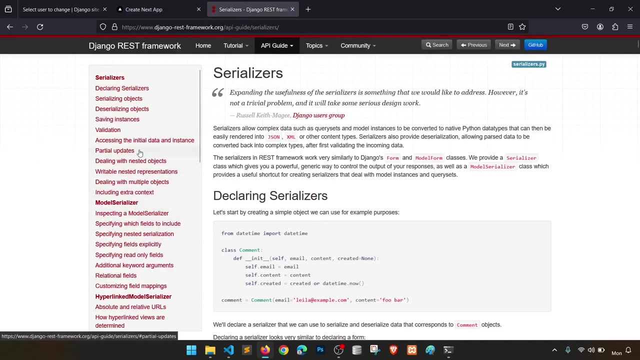 so first of all we need to uh from rest framework we will import the serializers class user. there are so many types of serializer but we are going to use the model serializer so you can check what other types of serializer in the official documentation so you can see here model serializer, uh, here serializing objects. you can define the fields. 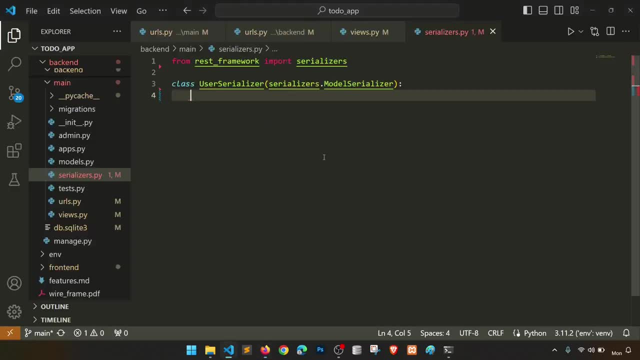 or all the things. right, you can check the documentation. so we will follow the model serializer. it will apply it automatically. uh, accept the model and or do the necessary things, right, okay, so model serializer, class meta. as i said, this is same as model form, so model equal to. 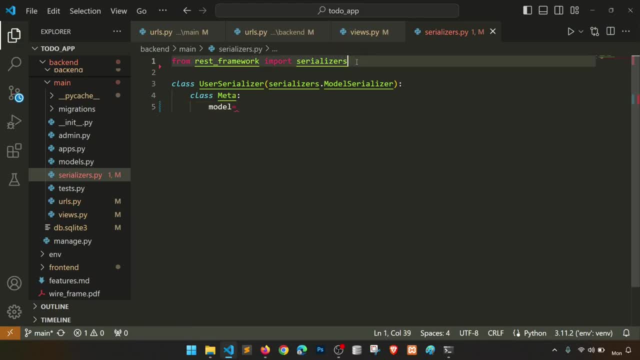 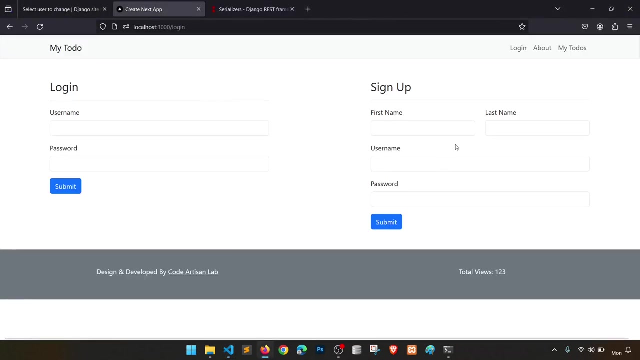 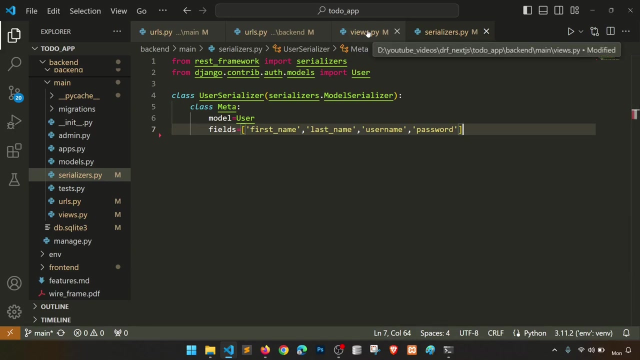 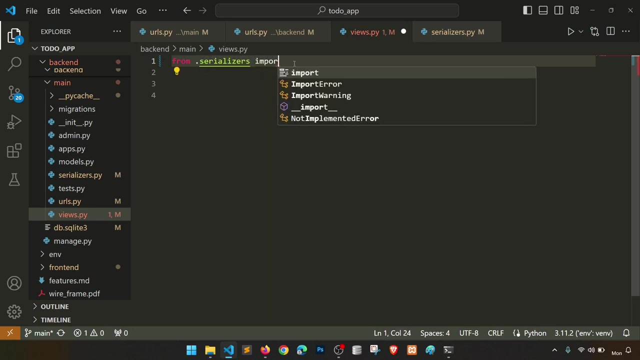 let's import from django dot contrib, dot auth dot models import user. right, so user, and we need to define the fields equal to first name, last name, username, password, okay, uh, what other fields are? okay, four fields correct. so we defined the serializer right now. uh, let's use this serializer in views. okay, so from dot serializer import. 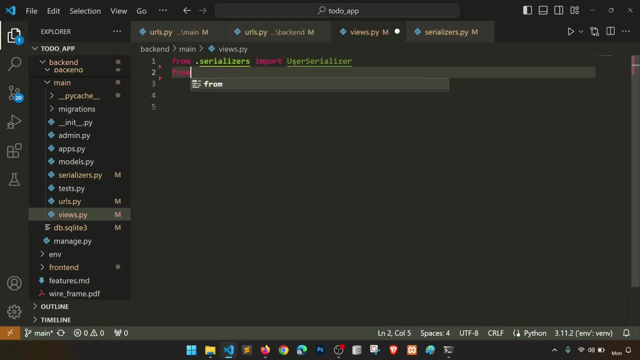 user serializer and from rest framework, let's do what in the test framework: dot gen bricks import list: create api view, right. so with this class, with this class, we can use the api view to, uh, show the all user list. or if the method is post, sdp method is post, then it will create the data, right. 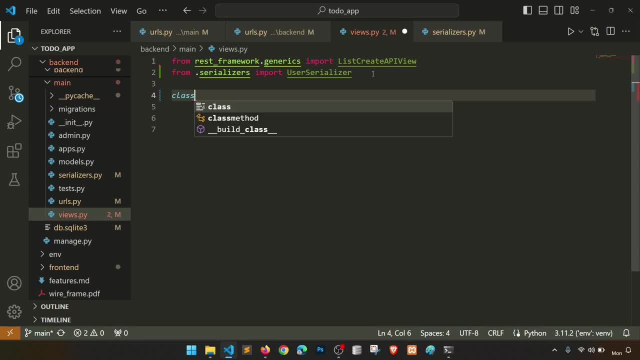 we will see all the things, okay. so class: user api view list. create api view. here we will define first of all serializer class, so user serializer. then do the query set equal to: okay, let's import the user model from here, so users dot, objects, dot of right. so don't be confused, it will automatically. 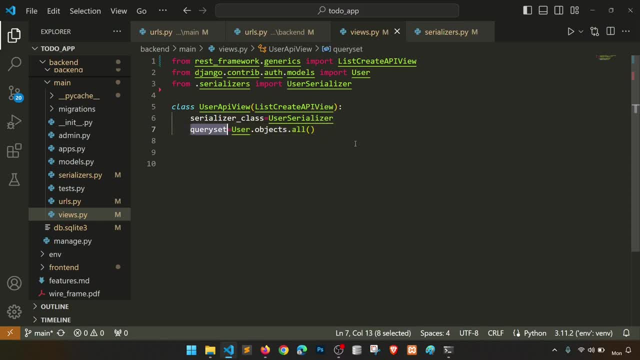 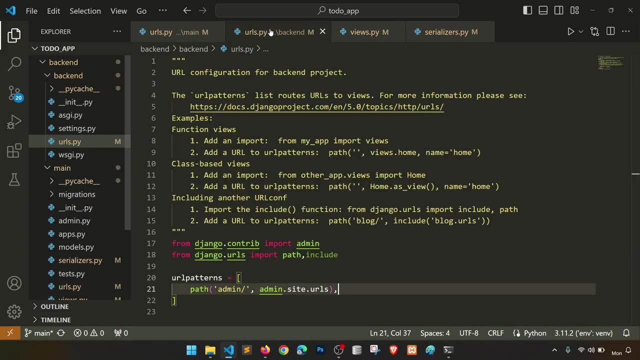 uh, do the query set according to the http method. if get, then it will fetch the data. if post, then it will add the data correct now in the url. ah, this is the app level url actually. all right, this is then we will need to import the query set. então, o Hmmm? 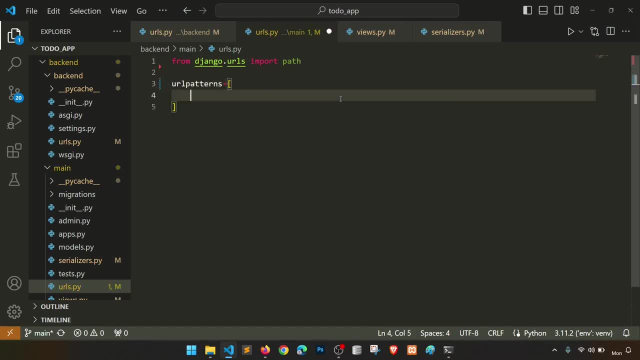 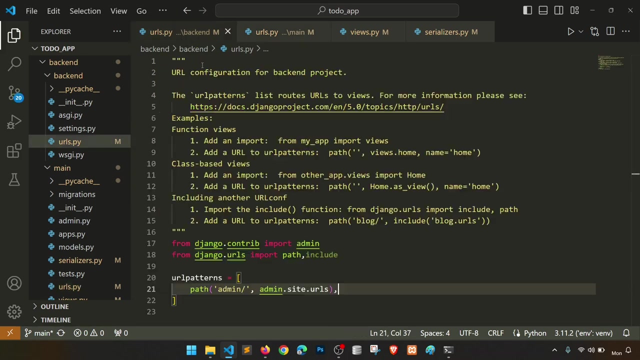 need to do URL patterns. path in this, users in here from dot import views. sorry, in here views dot user API view, dot as view. right, because this is class based view, so we need to define as okay. now we need to include it here also. so path, then API, and then comma include main dot URLs, correct. all right then, if 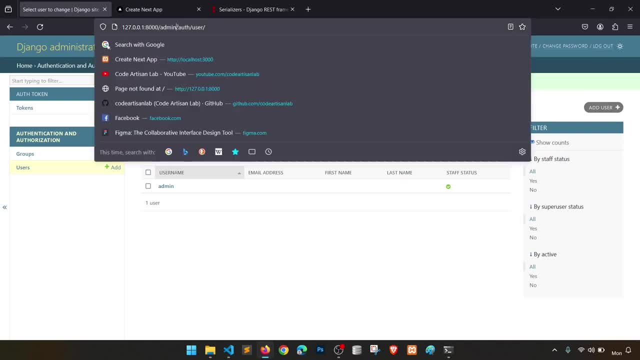 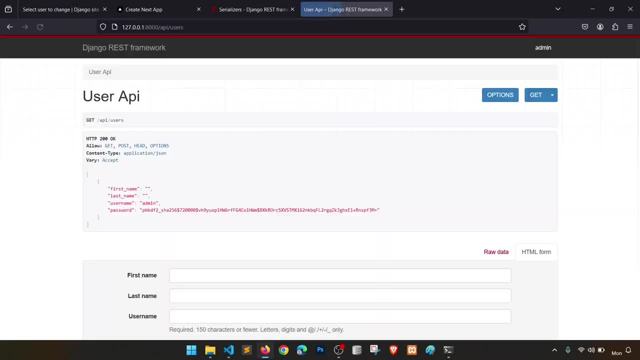 we go to the app and API, it is showing nothing. let's go to users so it will show the users, right? so this is this comes. this UI comes with the very browsable feature. comes with the Django rest framework, so it is helpful for development, right? but if you? 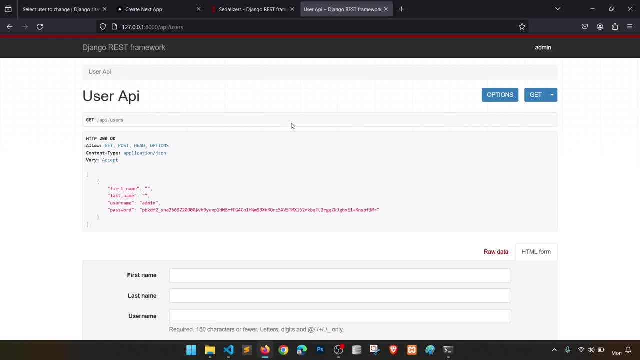 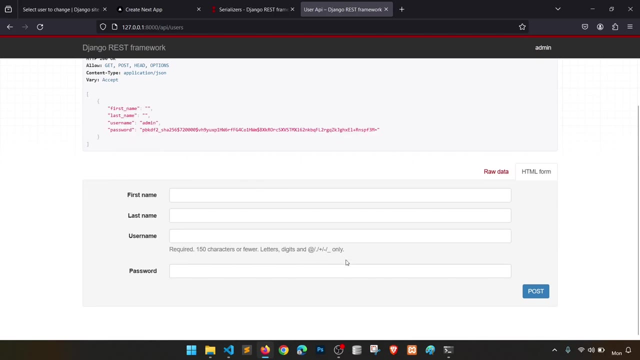 call this API from the next year's or any other front-end framework, then it will obviously show all that data, right? but this is useful for development, correct? okay? so here you can see that it is returning all the data right, and if we post this, then it will. 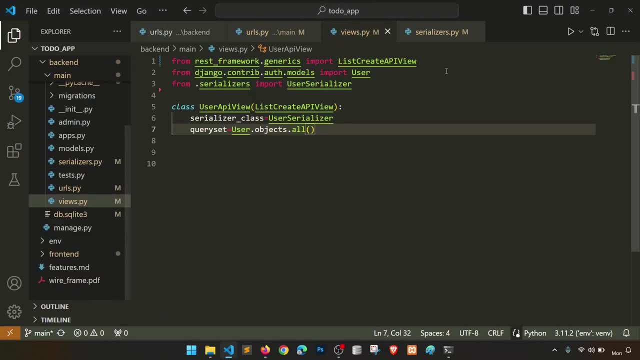 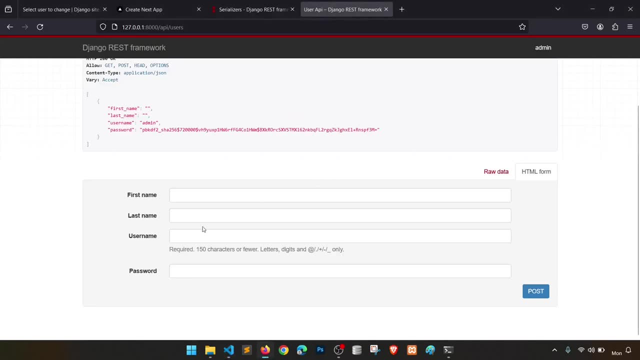 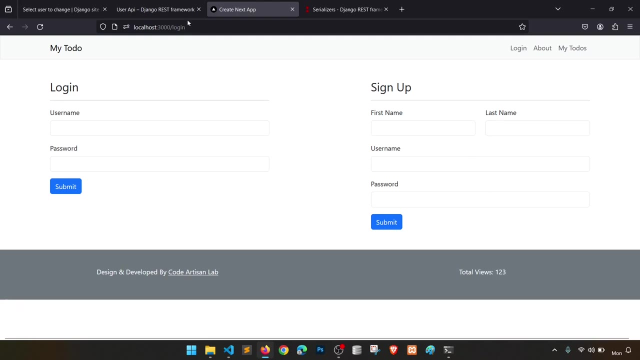 add the data. no need to change anything in the view or anything in the serializer. it will automatically send the data, right, but we will send the data from the next right. so now let's do this from this part and we will see that how we can connect the network to script. so now I will show you how to do this, so vou. 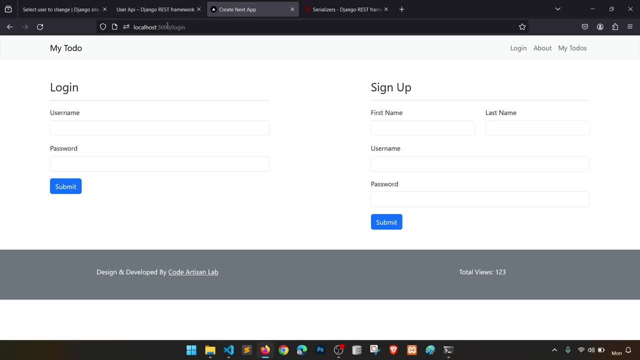 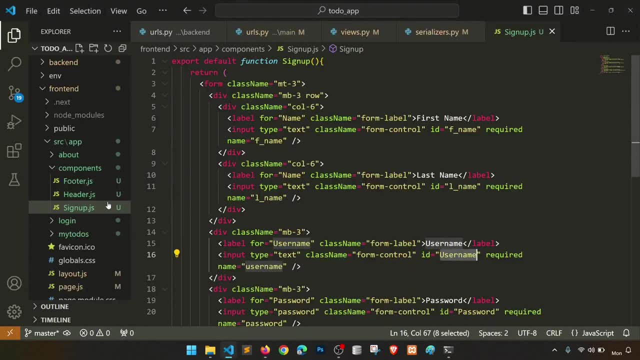 connect to script. i'm going to show you a few ways that we can do this in one nextjs with the django rest framework, with the api, okay, so let's do that. all right, so let's open a signup component. so here we have the component, we have a signup component. so one thing we should: 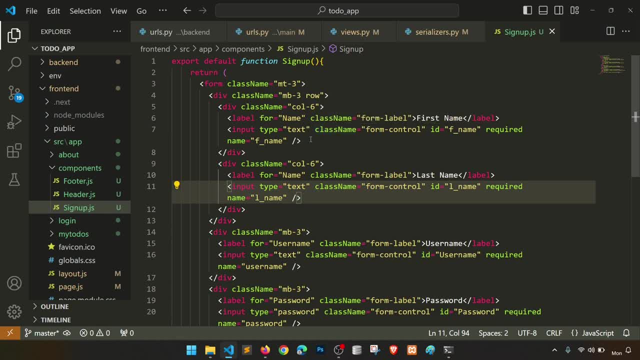 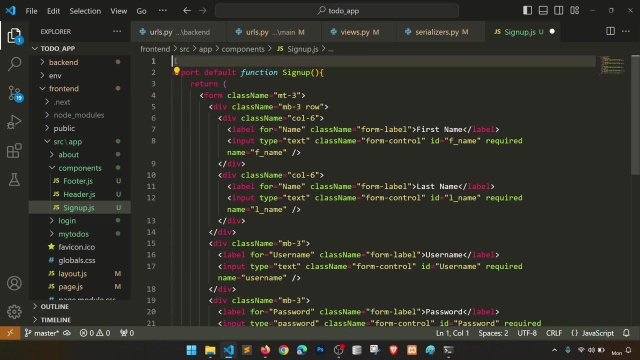 remember by default, uh, all the components and all the things. by default, all the pages are in. nextjs are server rendered, right. so if we want to include the user activity like click or something, then we have to make it a client component, right? so what we will do at the top, 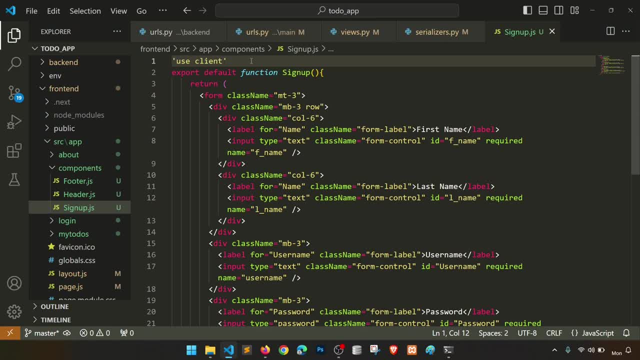 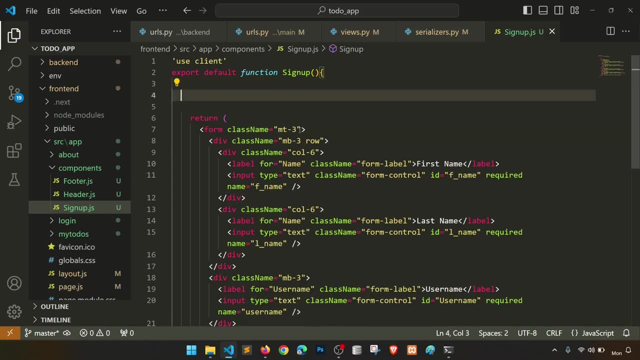 we will say use client right, and then in this, in the signup component, let's create a handler. so on submit, we will say on submit, and before submit, please check that, uh, you have defined the name for every uh input or every element in the form right. so we will say handle or we can say submit. 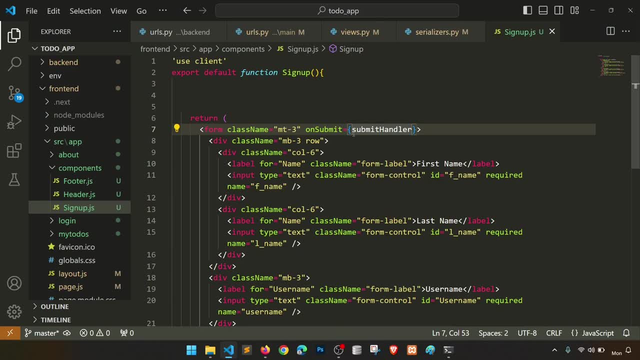 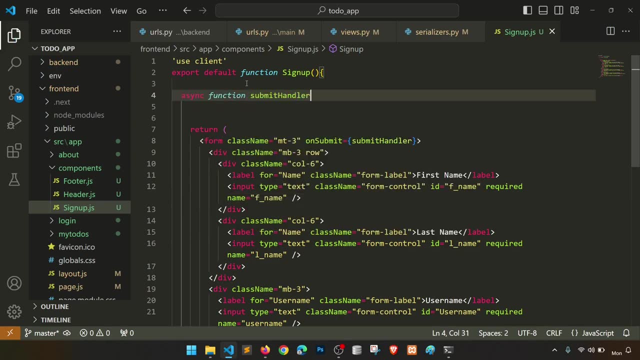 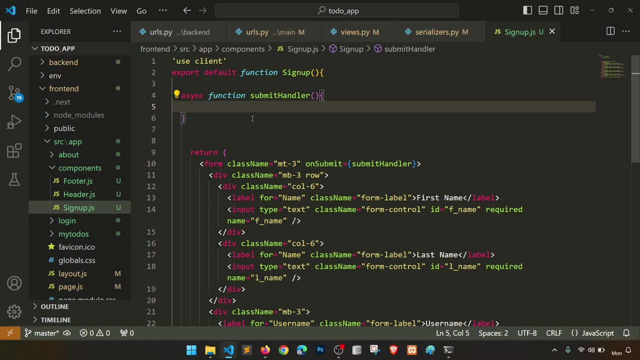 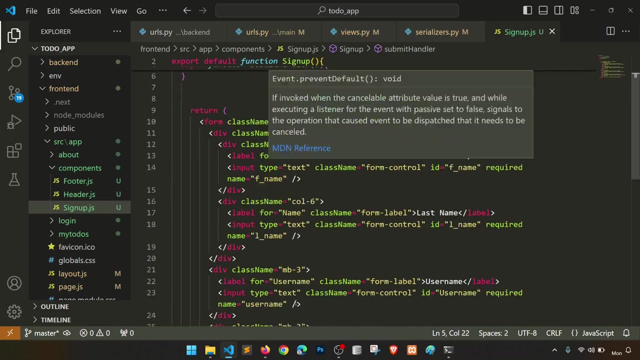 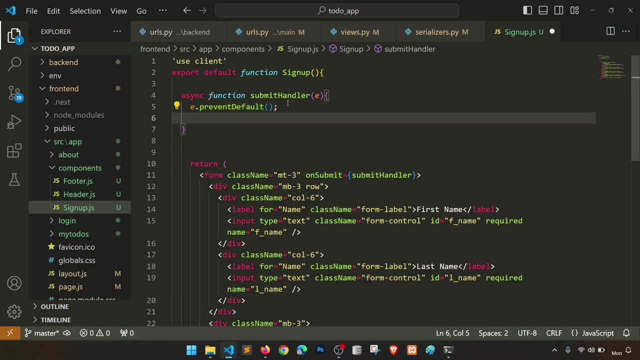 handler right. so submit handler. and we are going to create this function, a sync function: submit handler right. and then, uh, here we will say e. e means this context of the form, so e dot, prevent default. because default when we submit this form then it will reload the page. but we don't want to do that, so prevent default. and then 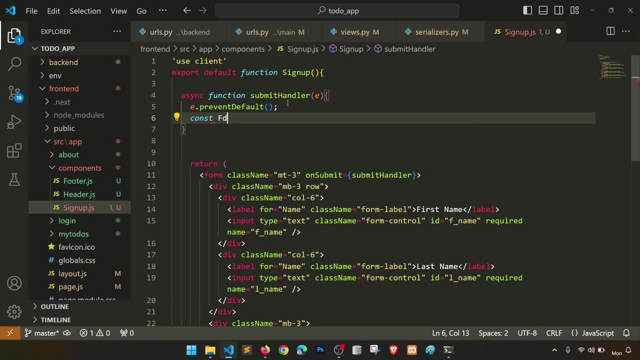 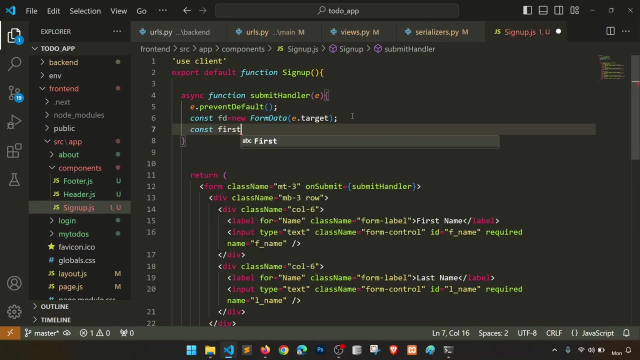 we have defined the constant form data equal to new form data, e dot target right. so what it will give us? it will give us the all form data right now. in from this we need to constant first name equal to fd dot. get the name of this field. 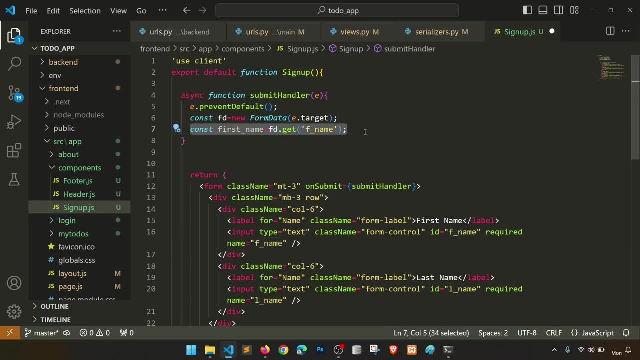 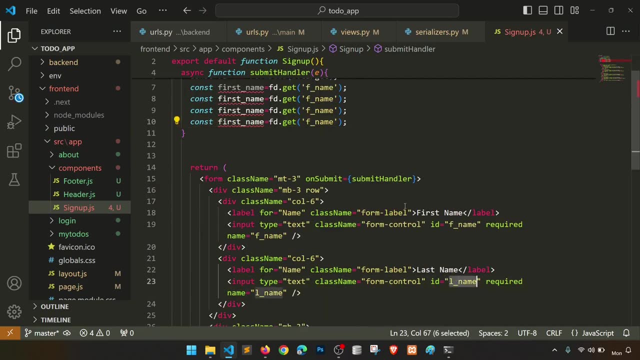 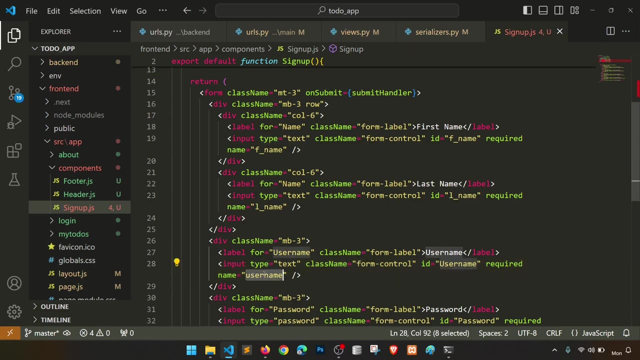 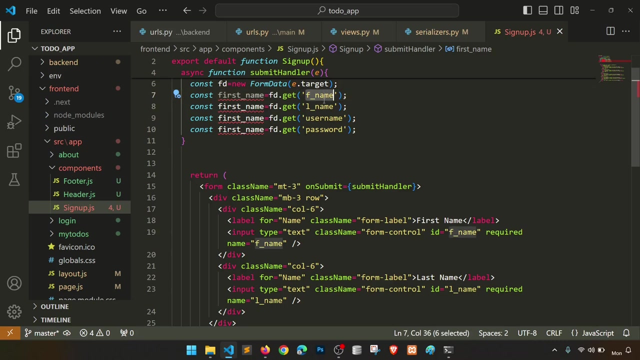 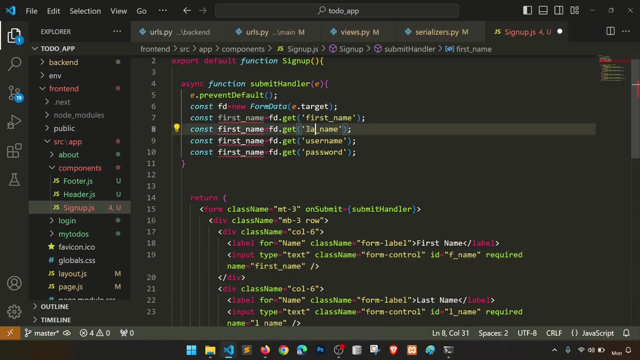 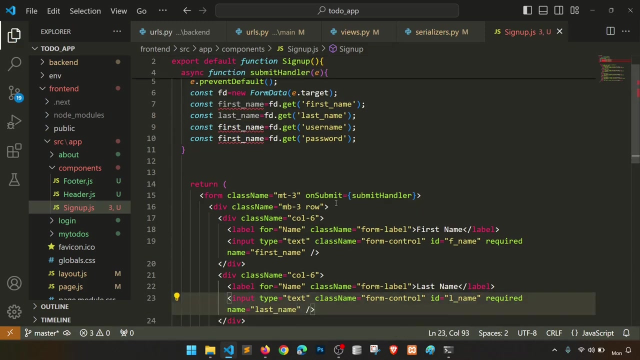 right, and we'll do the same for all four fields, correct, okay? so last name and then username. oh, where is that? username and then password. i think we should give give it the same name. no, so here we will give last name. right? so here we will give last name. all right, then user name. 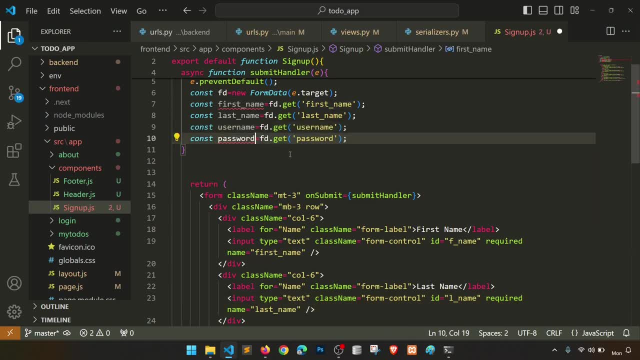 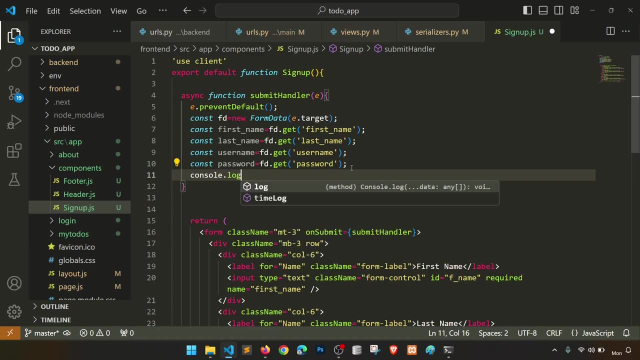 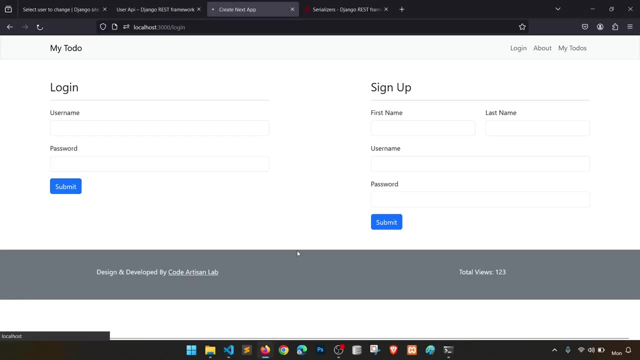 and then passwordZoom correct. so we have this four data. now let's check that this data is working정 right. so we'll go to here, right and here, and let's go to consoleзы а and let's go to console advised running function, and then we will. 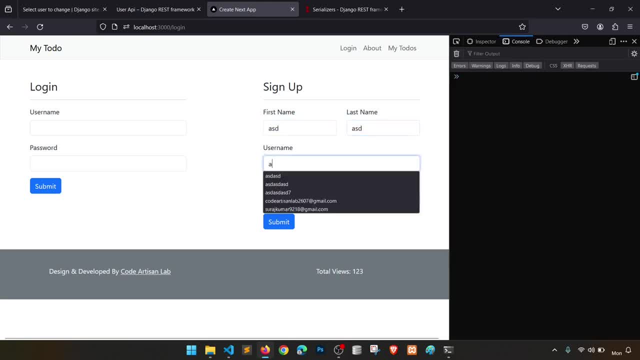 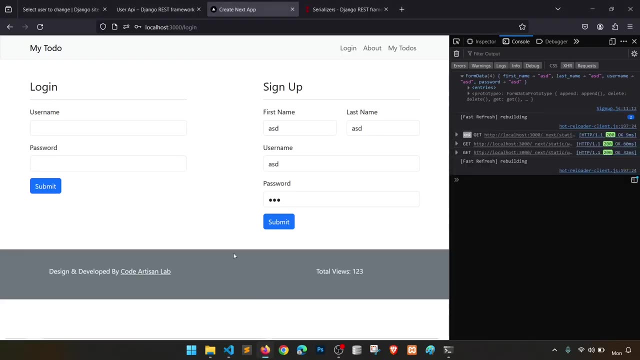 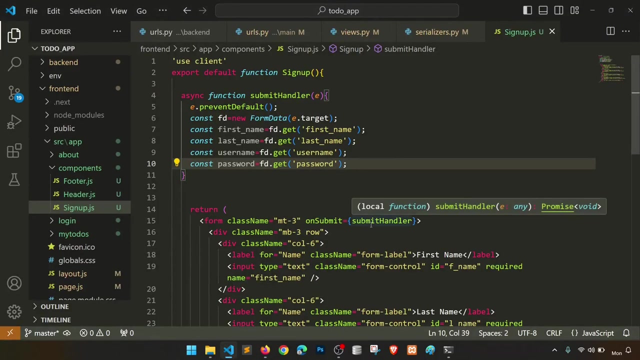 go to console and if I come at this, then you can see. here we have all the data: first name, last name, username and password. right now we need to send this data to the cell, okay, so the server URL is this: right? we need to send this data with a postman method here. so what we will do: send. 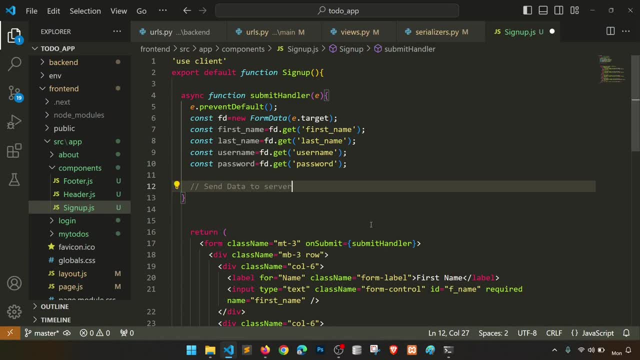 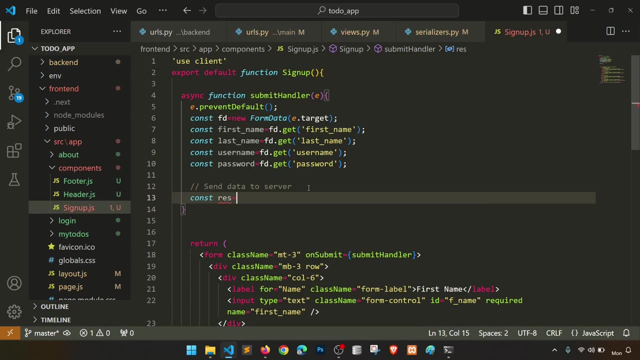 data to server. alright, so here we will do our constant response equal to, because this is a sync function. so we need to fetch. first of all, we need to define the URL, later we will define the URL, then we are going to write more complicated data and you're all. 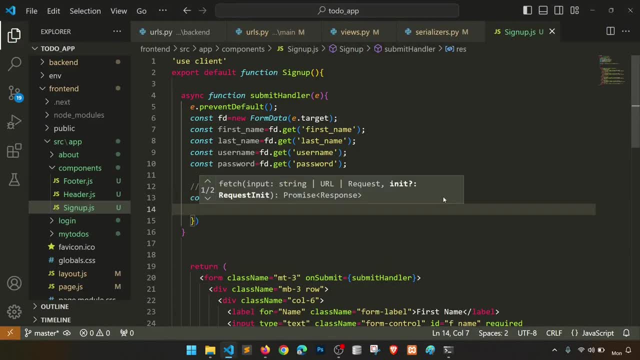 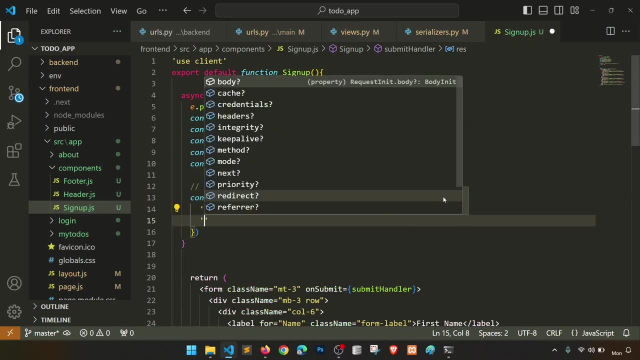 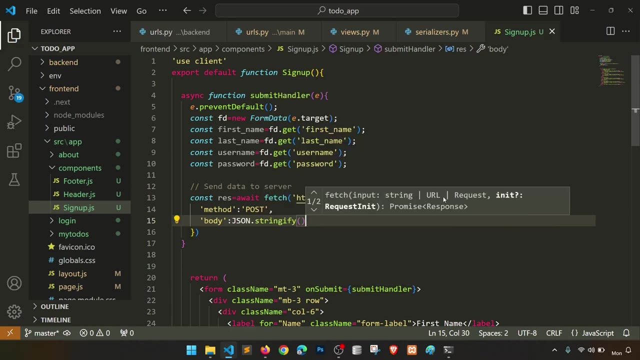 the common variable, then we need to define the method post, we need to define the body, which will be Jason dot string if I and when you define the safety form data. now we need to do first name, last name, we need to do constant form data equal to this. 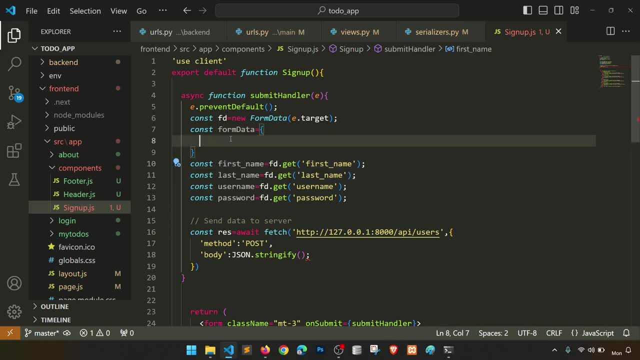 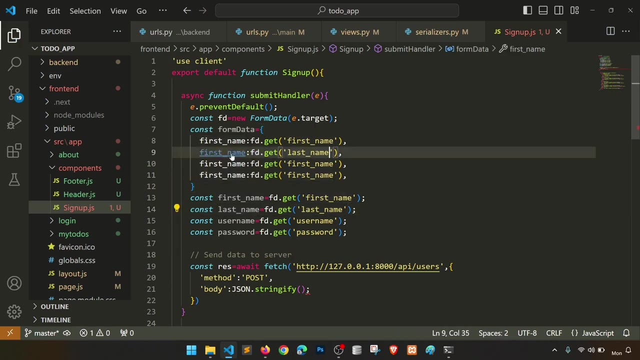 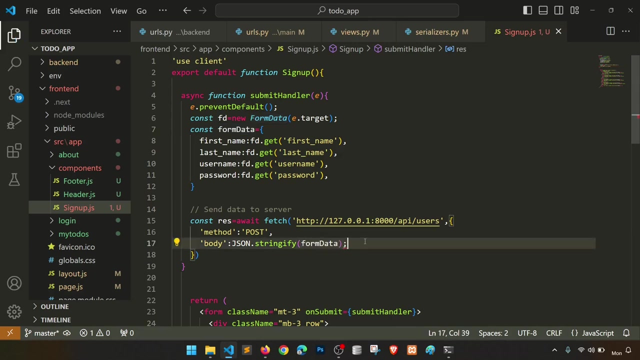 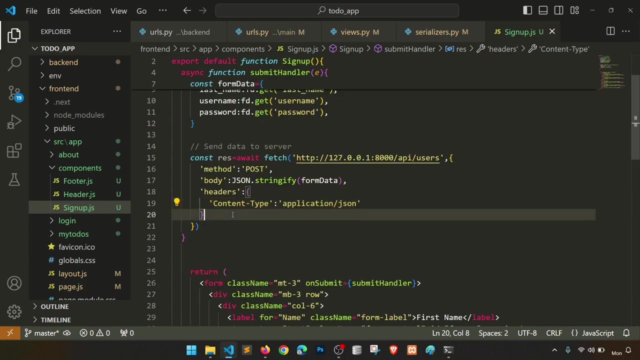 thing we have done wrongly here. actually, we need to do this kind of thing. so one, okay, right then. all right, so here. and then form data here, okay. and then we have to send headers. headers will be content type, application, just right, okay. so this is our, this is our. 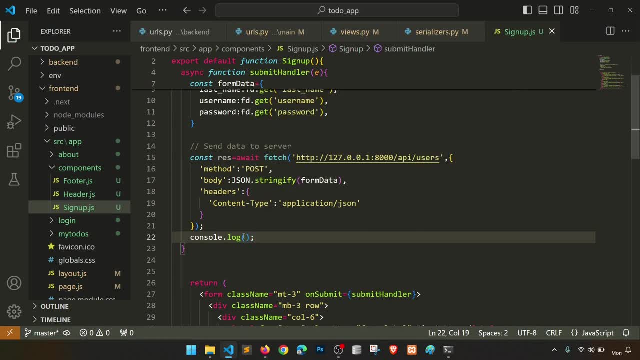 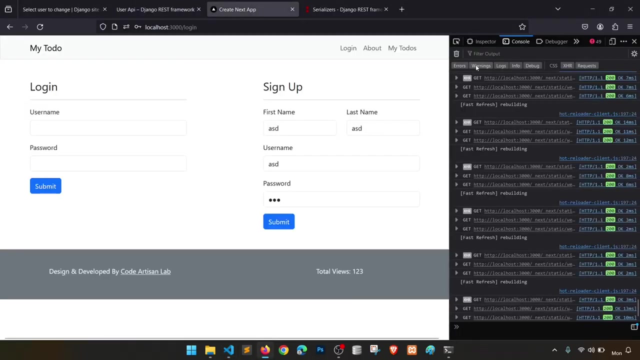 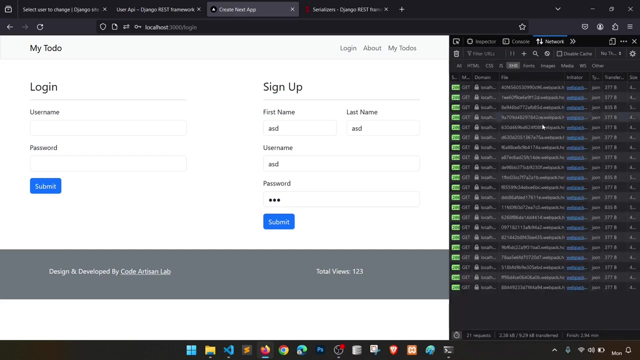 okay, let's see what is returning. we will say response data equal to response dot, which is right. so fit console dot log response dot data. okay, so if everything work, then let's see how it is working. so submit, if we go to work and if I click here, nothing is happening. 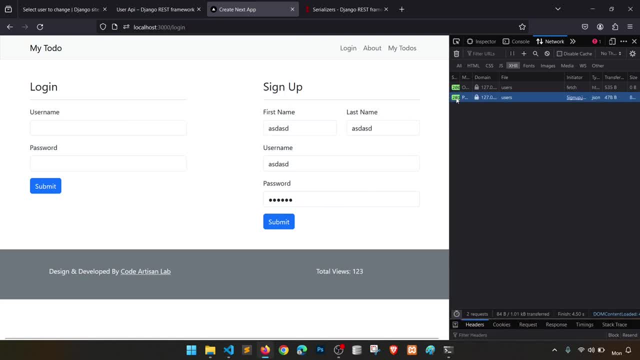 submit users and this. okay, so it is returning all the things requesting. we are this, this, this response is this: okay, so this is 201. right, so it means data is creating. let's check here here you can do the same thing again. okay, all right, so data is creating. right, so we successfully called the API. 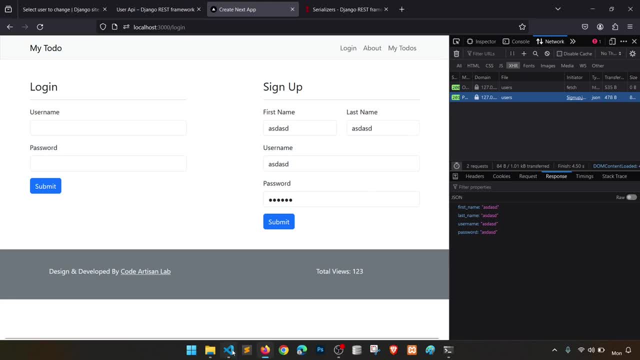 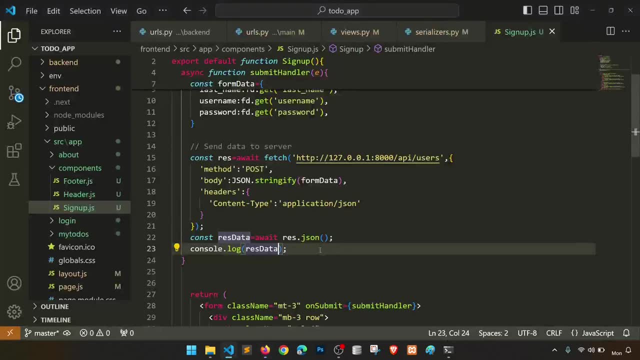 now what we need to do, so we'll see. here we have response. so if we say okay, so if we say okay, okay, all right, so here we have response. so if we say okay, so if we say okay, so we have response. so if we say okay, okay. so if we say okay, okay, okay. 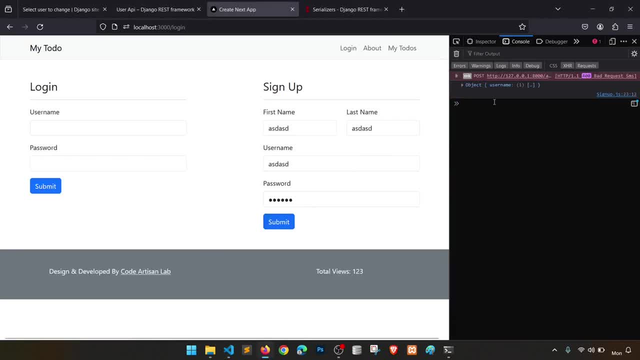 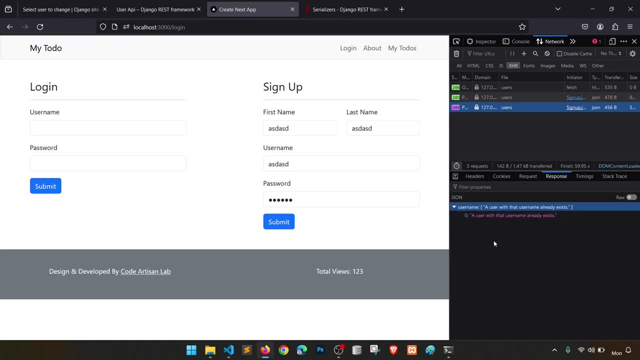 so let's, if i say this, click again. then you can see here: 404. the data is saying that user is username is already exist. so what we need to do: if user signed up successfully, then we need to show the message. if not, then we need to show the. 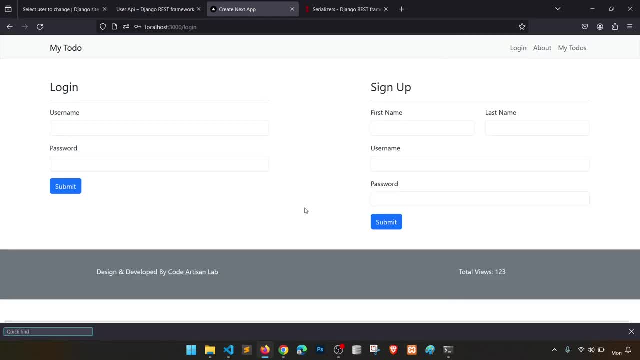 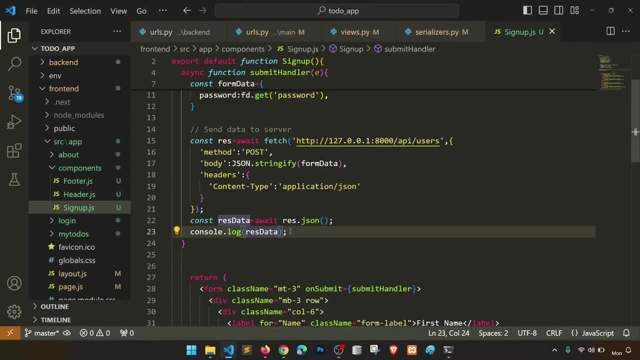 errors, right. so let's do that, okay? so let's show the success and error message for this sign up. so what we will do here. so, first of all, we will see if we will see here, if this response. let me show you first of all this response. 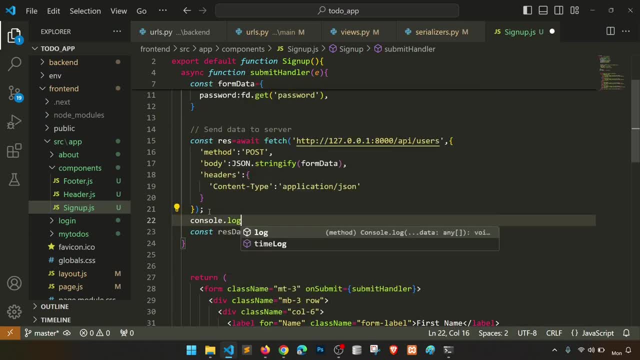 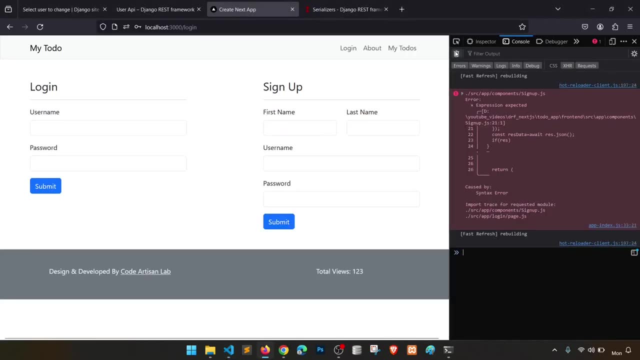 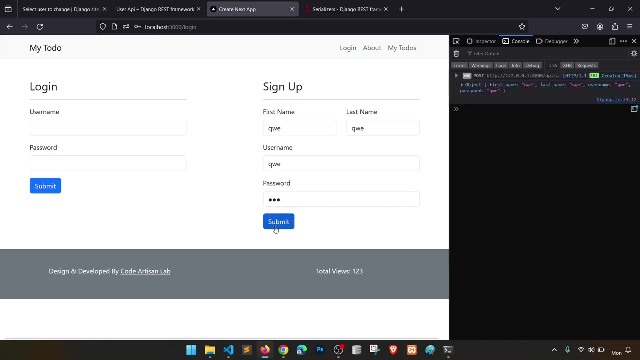 then we will, uh, it will clear to you. all right, so this is response. and if i open this app, well, uh, let's say these three things in the all fields and submit so you can see here. all right, so this is not showing actually response, but we need to do again. let's remove this. 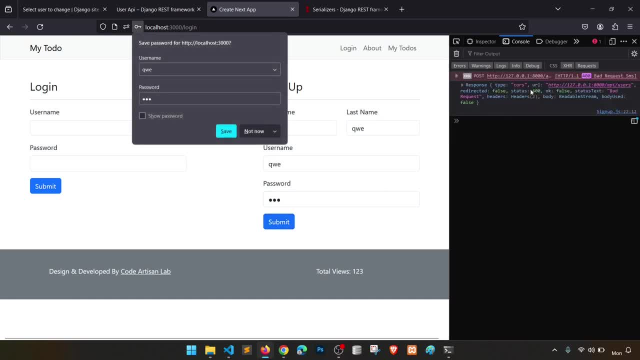 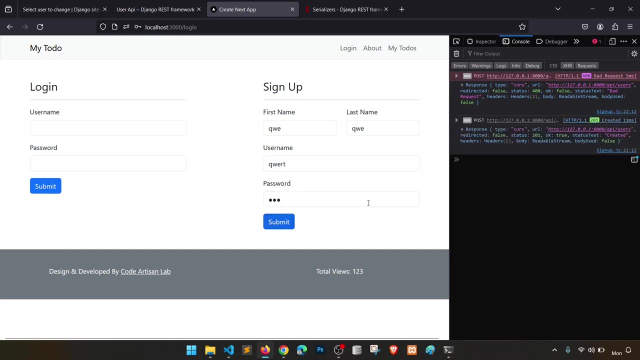 oh, sorry, so submit. you can see here this response. it is saying uh, status 400. uh status text- bad request- right. and if i say uh, let's say rty and submit. it is saying: status 201- status text created right. so from this response we can uh show our success and error messages. 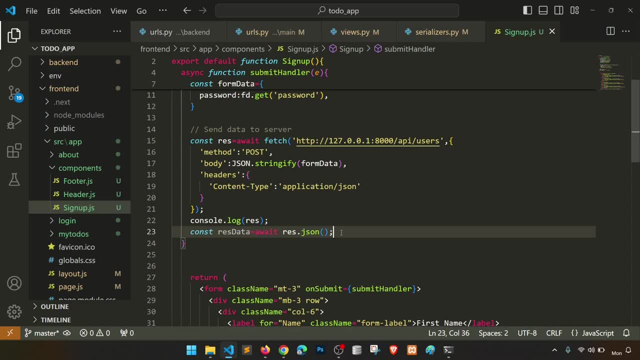 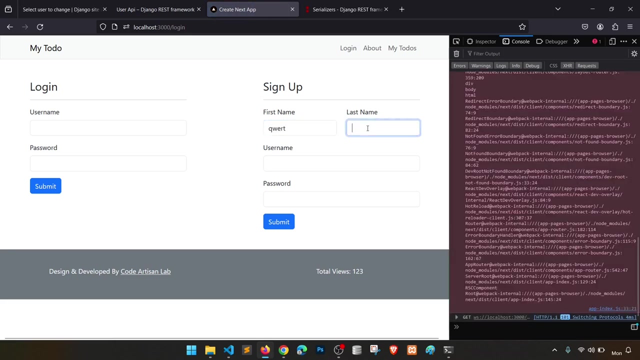 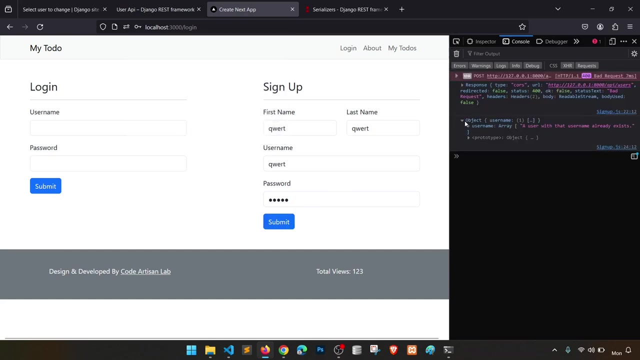 okay, so for our success and error messages we can see here: consolelog, Pep, unwrap response data. right in this response data we should have all the data right, errors or anything. okay, so let's, i will copy this username, same right. and so if i submit here you can see here. these are the 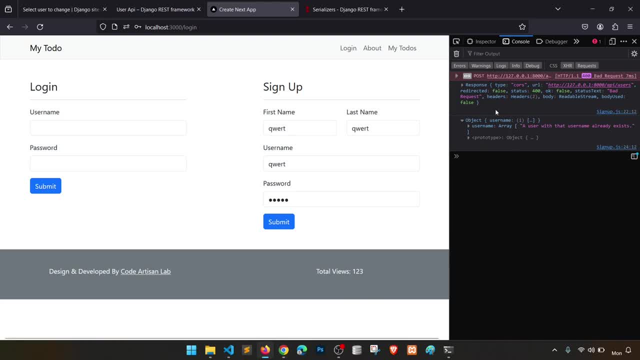 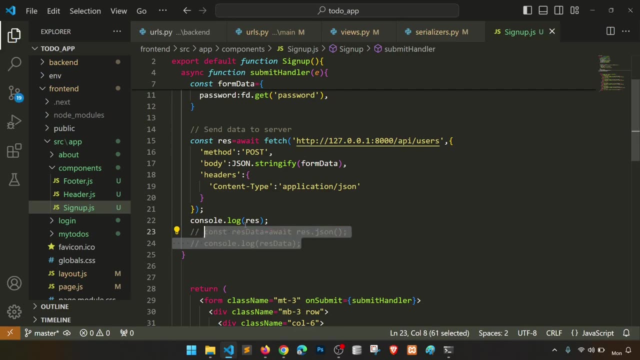 errors right. so we need to show this. okay, and if status is, status is two, zero, zero or okay is true, then we can show the success message. so let's first of all show the success message, then we can see other things. all right, so we will use the user state from the react. so I will 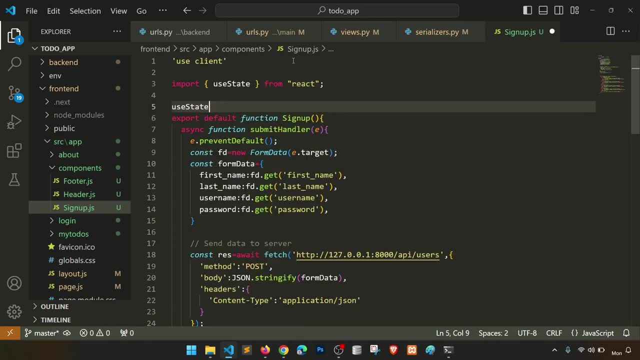 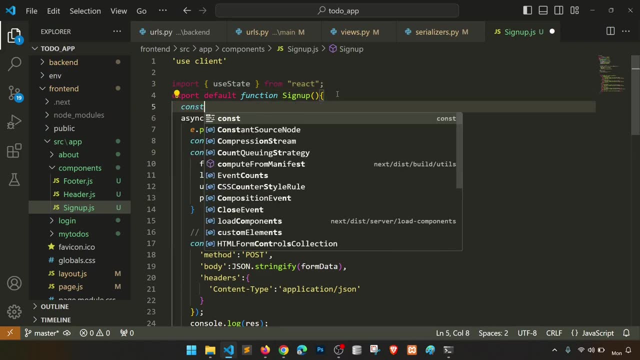 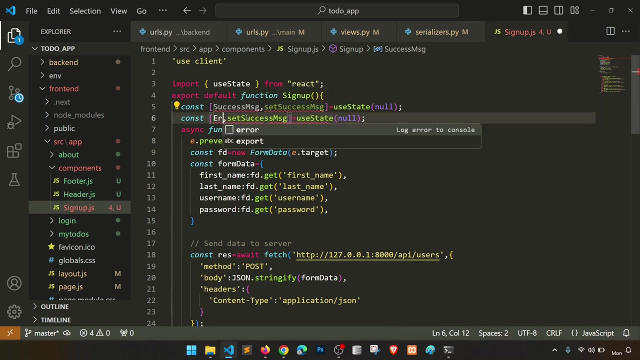 say use state, it will automatically fetch or remove this and from this constant will say success, success message. set success message equal to use state, default, null, right and same for the error message. for the error we can say error messages because multiple error and this will be list and right. all right. so for the 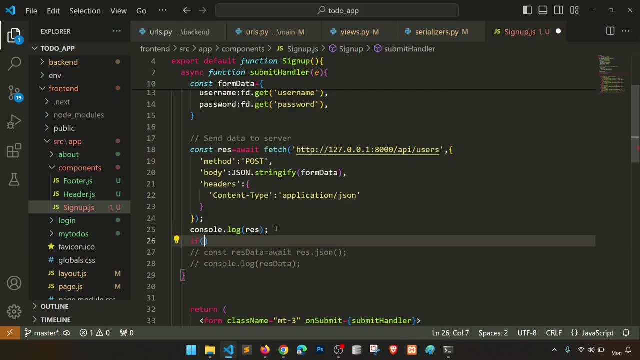 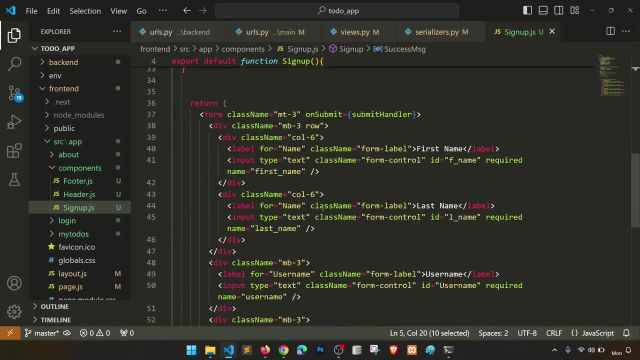 success we can show here. if a response dot, okay, then we can show this data. thank you for registering with us a triggers string with us, right else success message will work here. okay, empty, yes, sorry, any else not right, and then we have success message we can show. 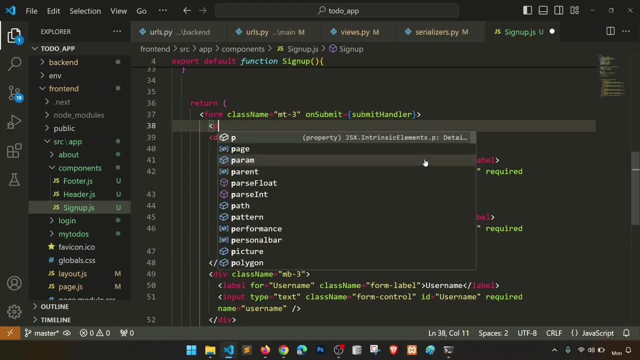 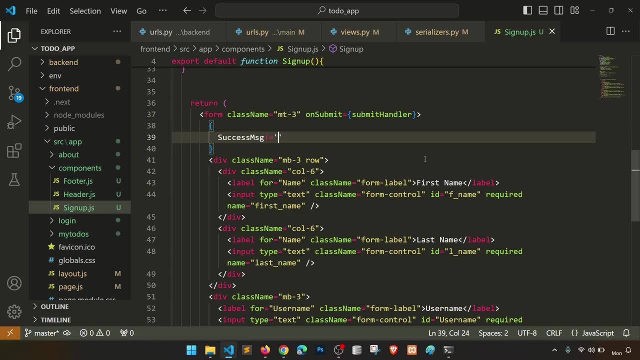 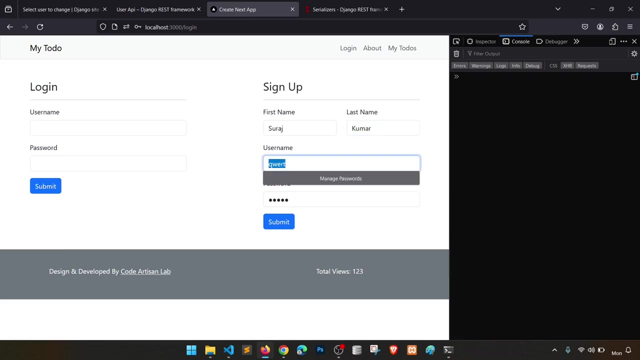 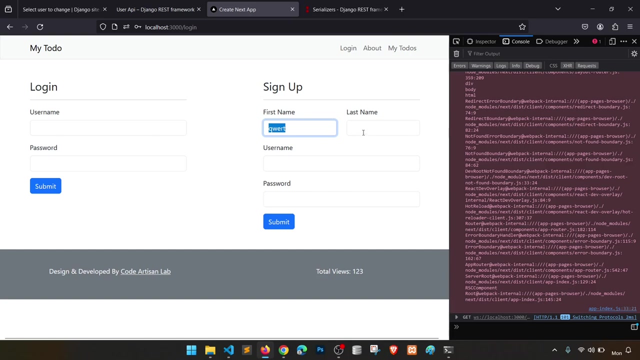 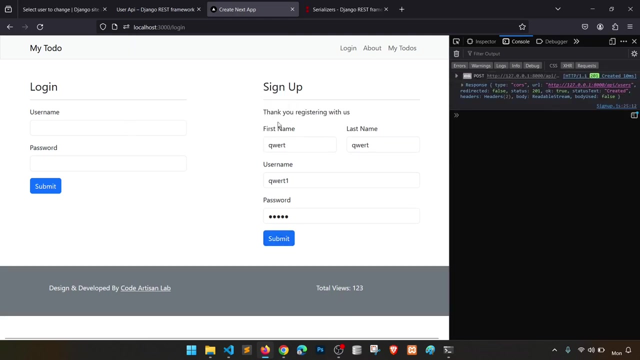 in the form here. so we'll say: if not equal to empty, right, then we will show the message: success message, correct. so let's say correct, submit. oh sorry. so let's say quote t: this one, this one with one, this one submit and you can see here: thank you with the registering us. okay, we also need to add one more class. 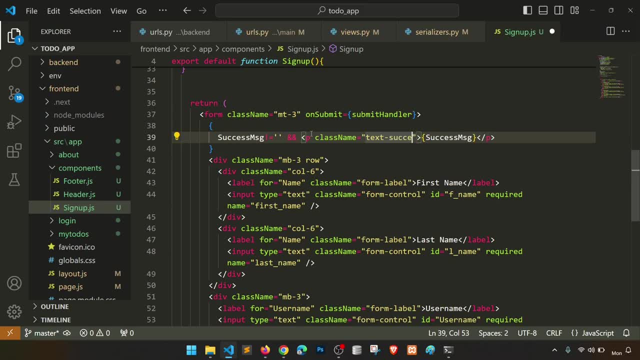 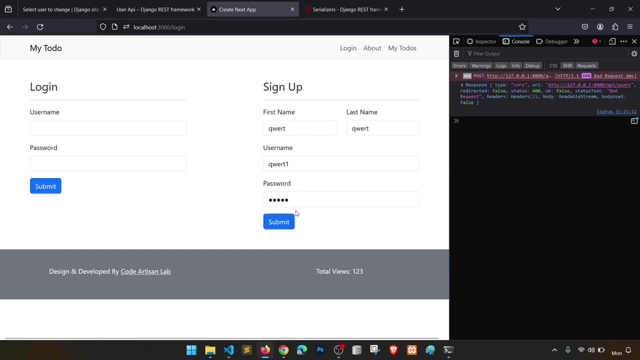 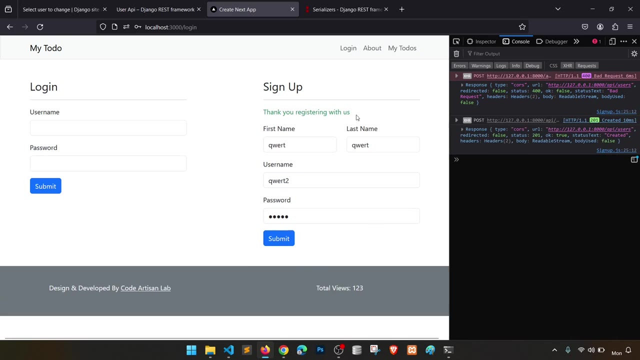 next, correct, submit and you can see here thank you with the registering us. okay. we also need to add one more class. next, success right and submit. so you can see it is not showing, because the error is exist and if i click here, thank you with registering us. okay, because this is another uh data we. 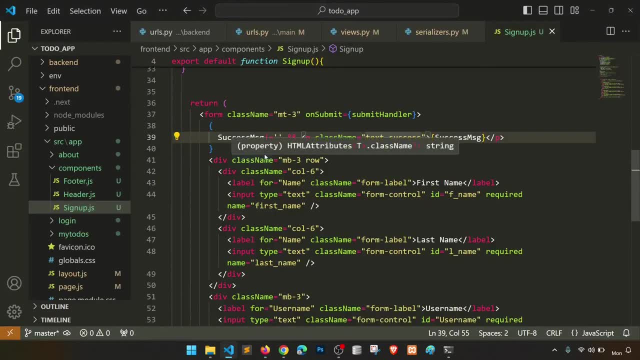 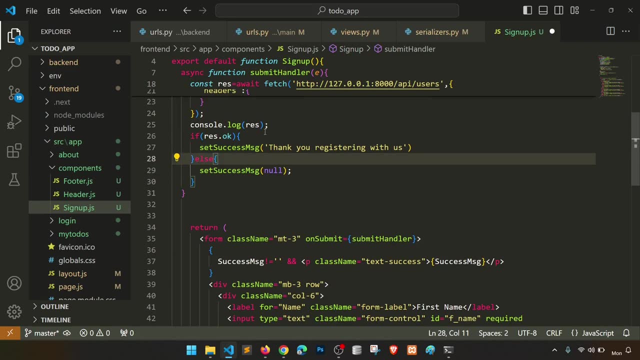 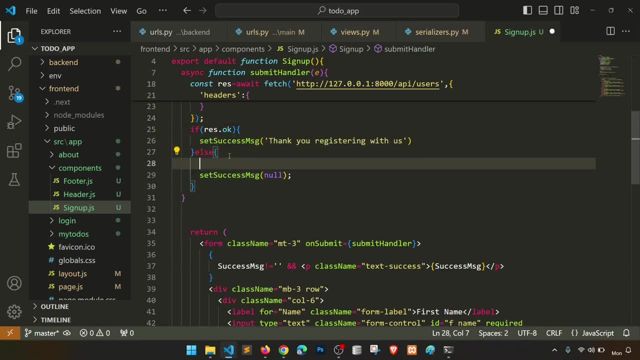 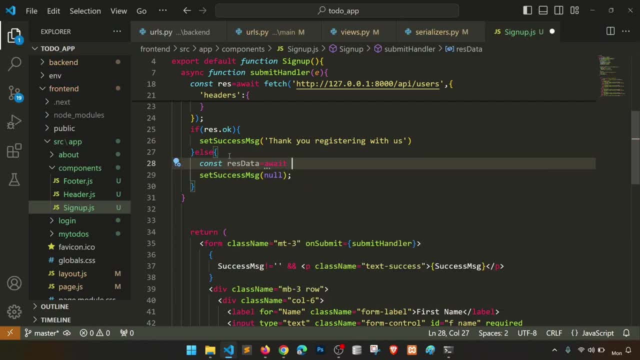 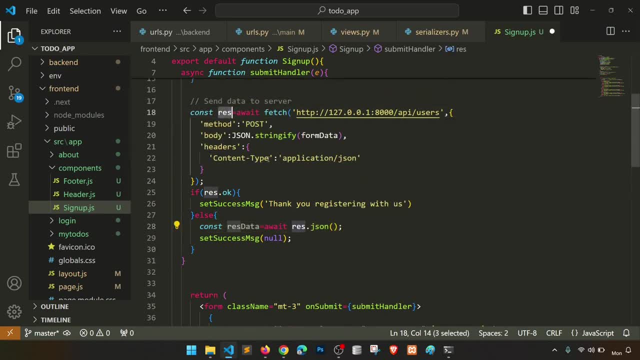 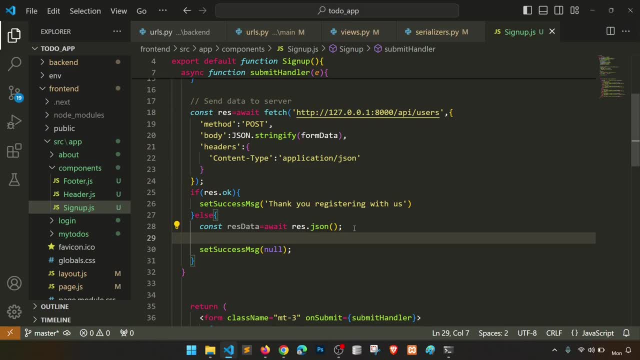 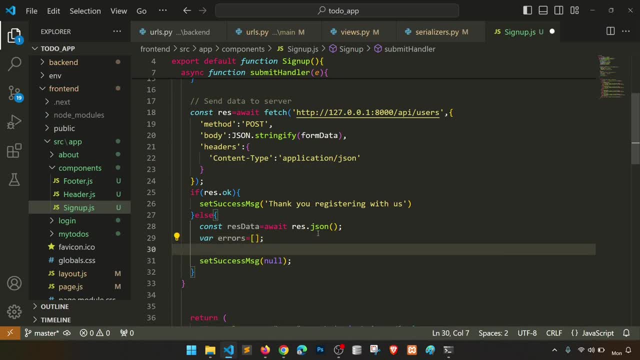 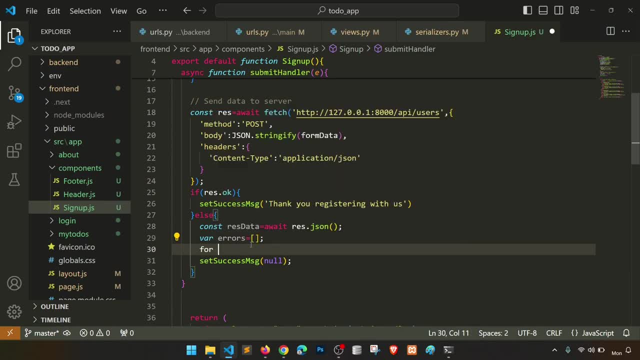 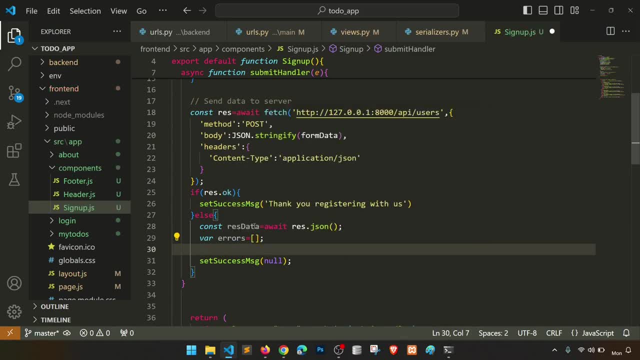 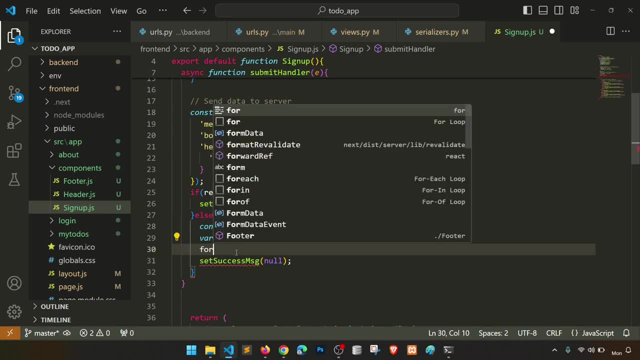 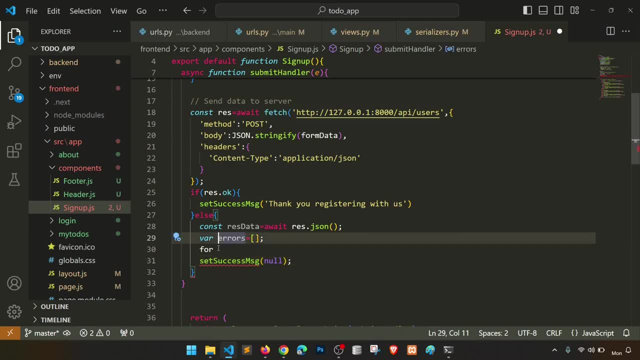 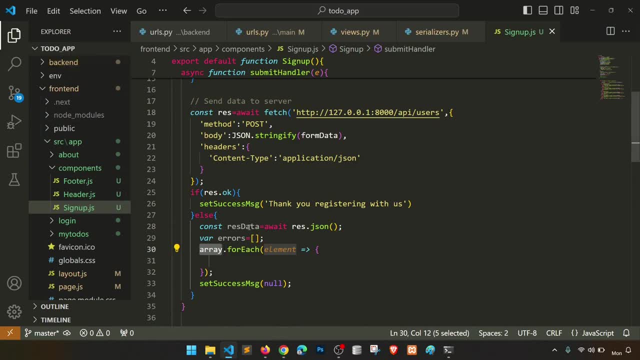 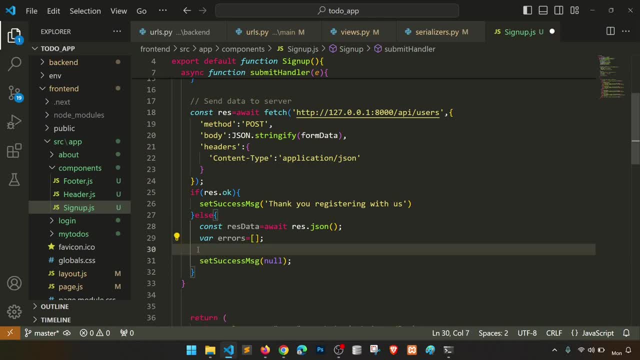 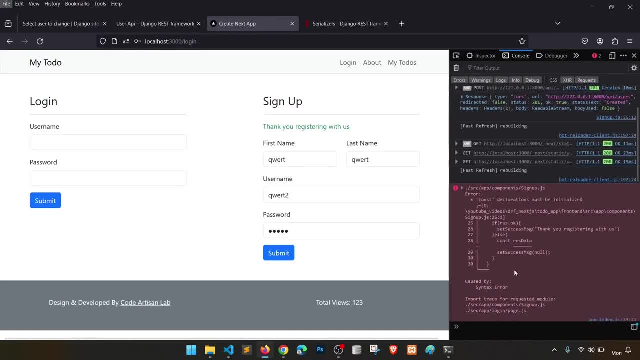 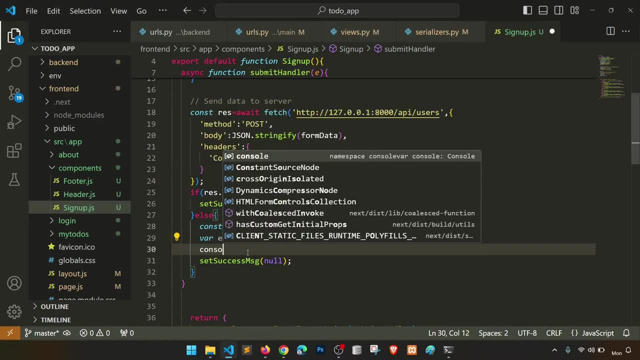 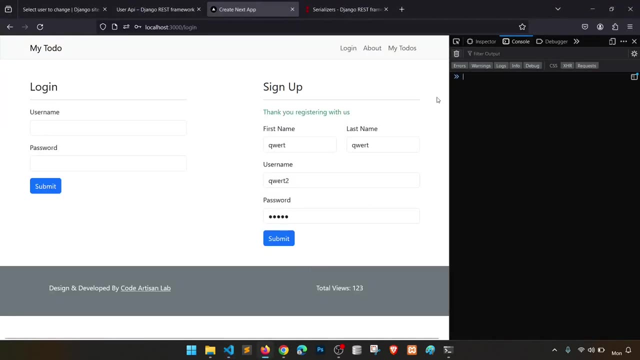 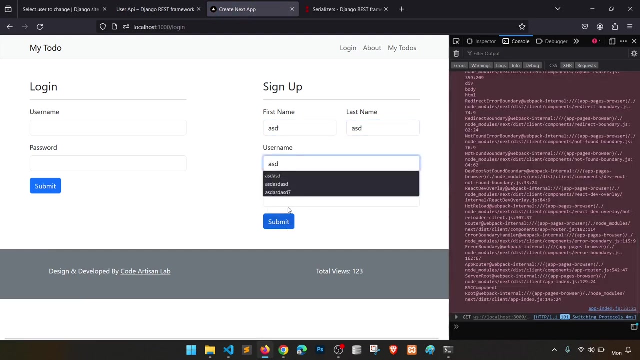 so we will create a where errors equal to list. so we will create a where errors equal to list. you know we need to send. first of all, let's see how this data is showing. so console dot log response dot data. and if I click here right, I see this, this, this: 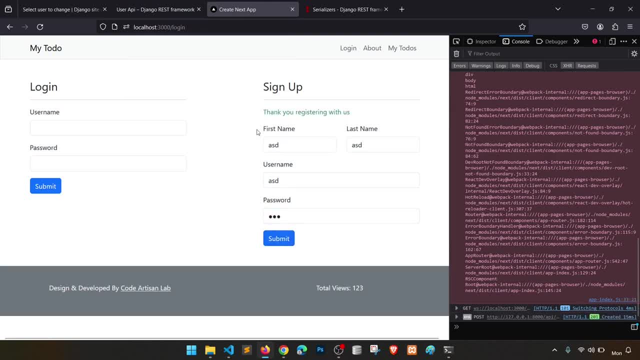 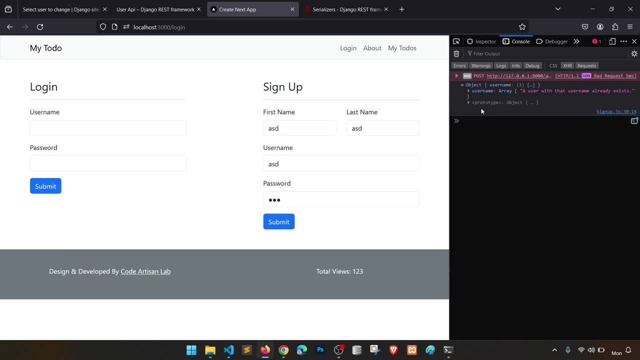 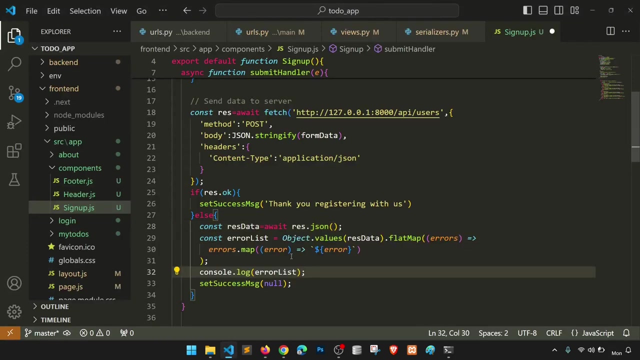 submit, submit. data is registering. if I click again, it is showing the objects right. so we need to run the loop correct. so let's run the loop, okay. so for the errors, what we will do, we will do this thing right. so object dot values. so it will convert all the objects. 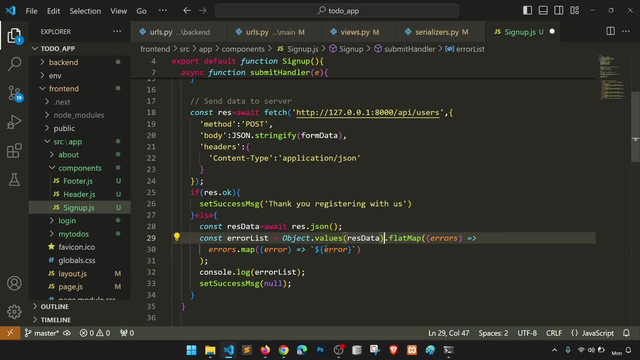 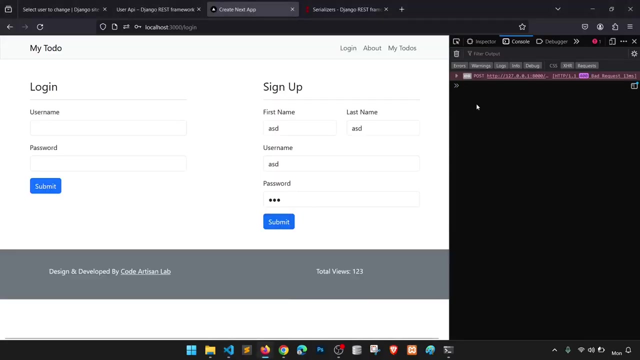 right, all the all the list from the objects. and then we are using the flat map. so what it will do, it will convert all the arrays into single array, right? so this is our single error and it will gives us this error list, right? so if we go to here and click submit, then you can see in the network tab we have here. 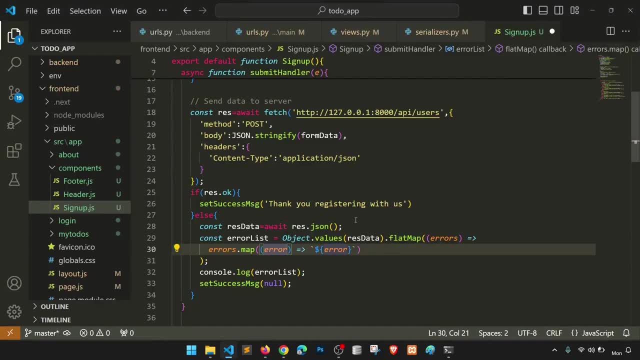 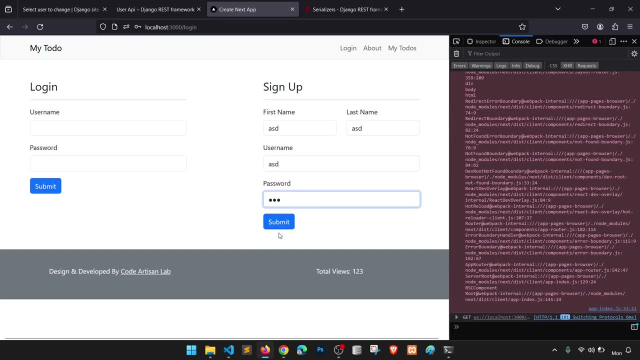 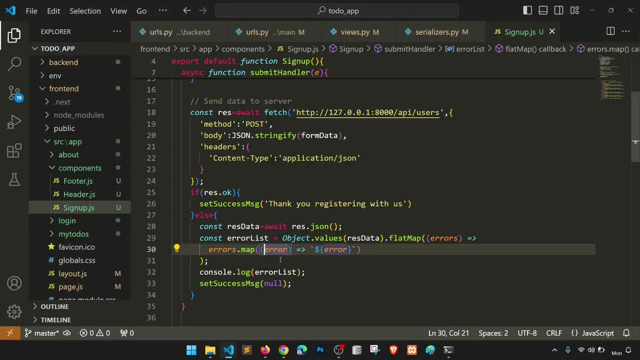 sorry, let me show you this. so SD and this, this, this submit, so you can see here this is showing a single array. now I will convert this array into the string, so we will say error string equal to error list, dot join and let's say new line: right, correct. or we can say he tagged with the P tag. yeah, 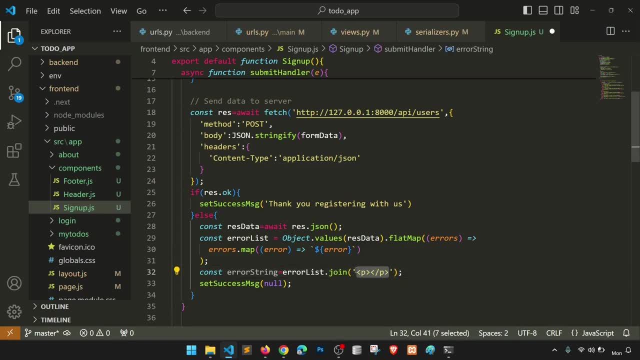 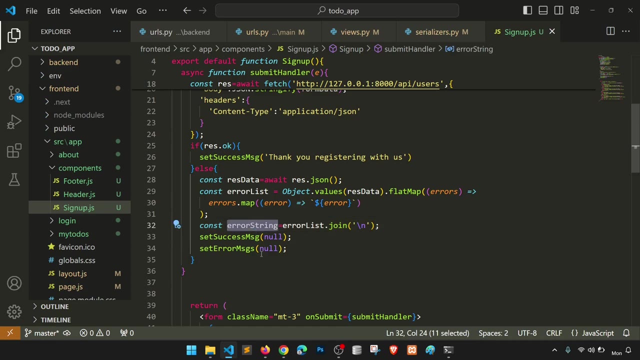 this is fine, new line is fine, right, so here we have new line, okay, and then, as let's say, set error messages, error string, and in the success, error messages will be empty, correct, okay, so all right, so we are ready to show. uh, let's see. oh no, uh, we need to do one more thing. 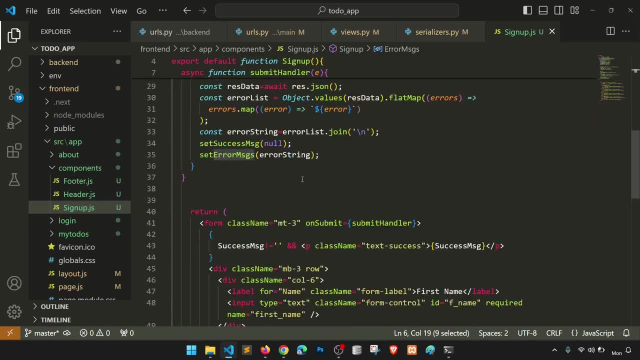 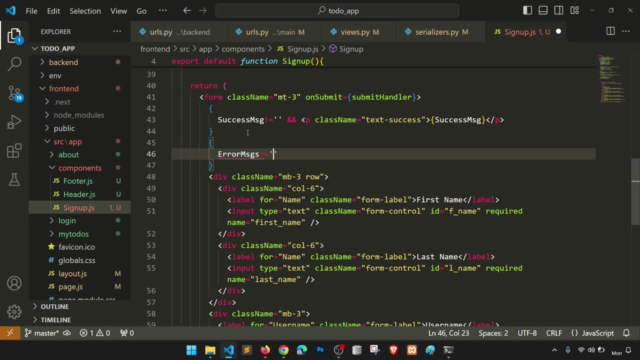 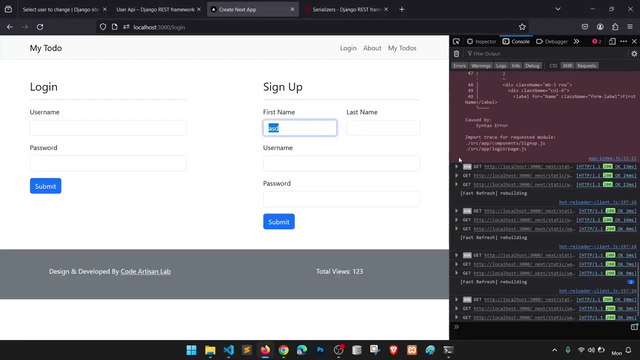 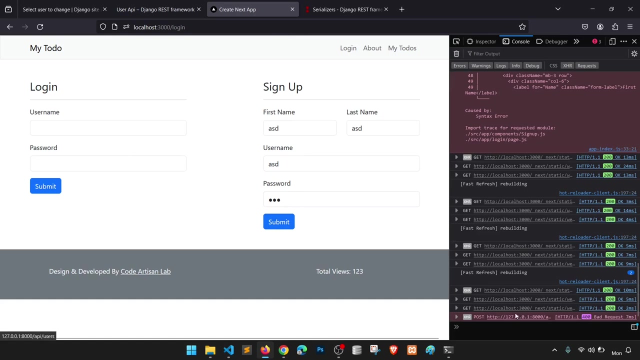 uh, error messages. we will show the error messages here, so we will say error messages not equal to empty. then then we will define div class alert: a lot danger, and here we will show error messages not equal to empty. great, now, let's see, it should work. now submit what is saying: not sure, let's see. 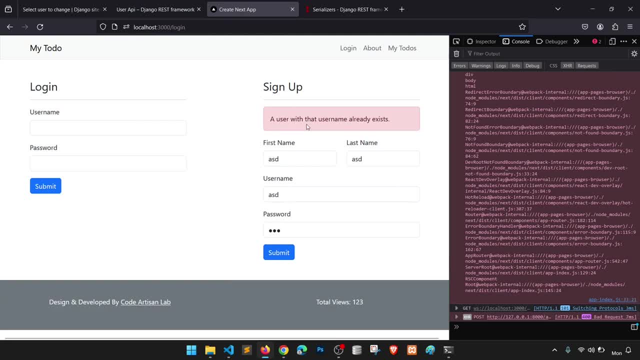 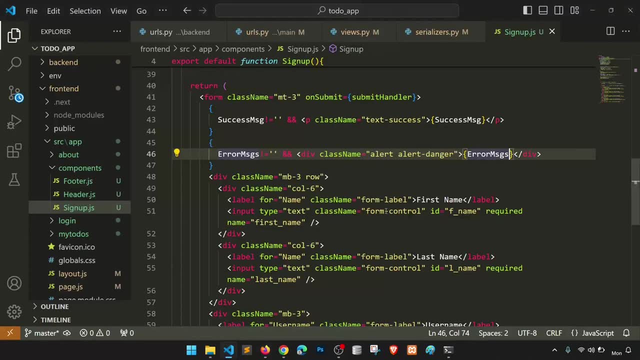 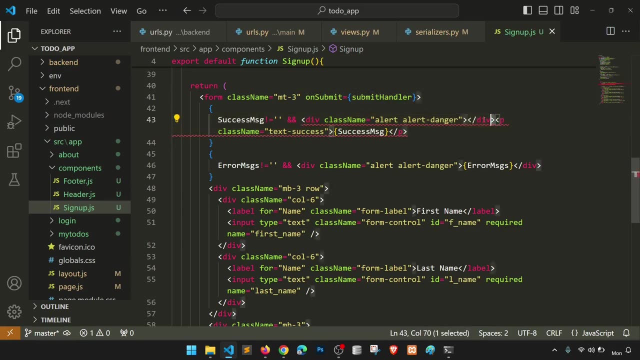 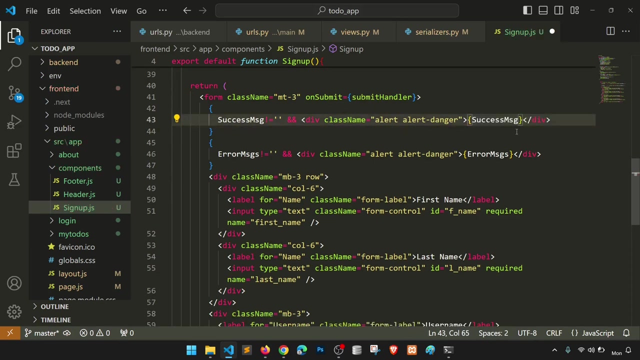 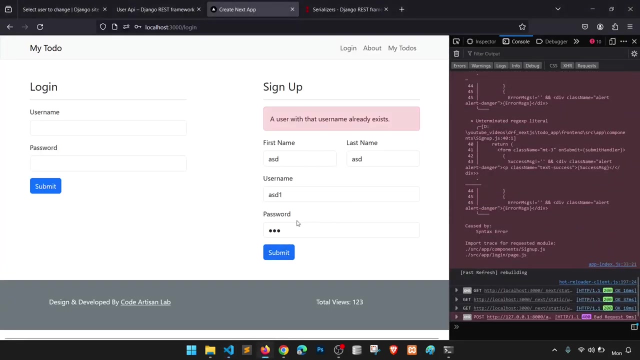 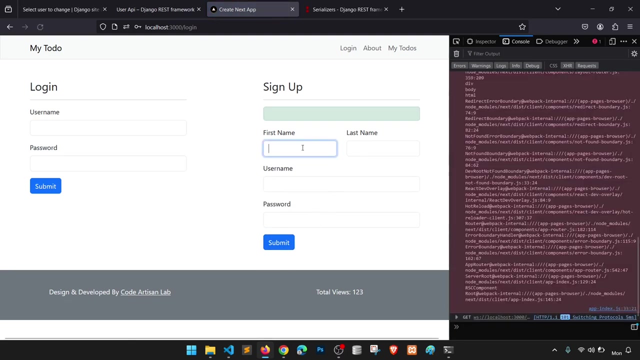 submit: okay, the user with that username is already exist. create one. thank you for registering with us. let's do the same thing for the message. this, so what is this? let's remove p tag. no need, okay, so success. correct. submit to okay, so let's go. what? what is this? 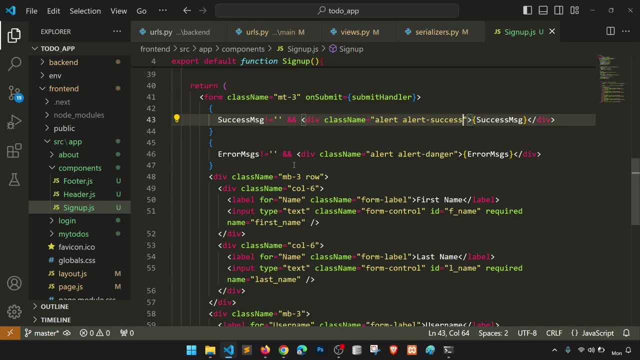 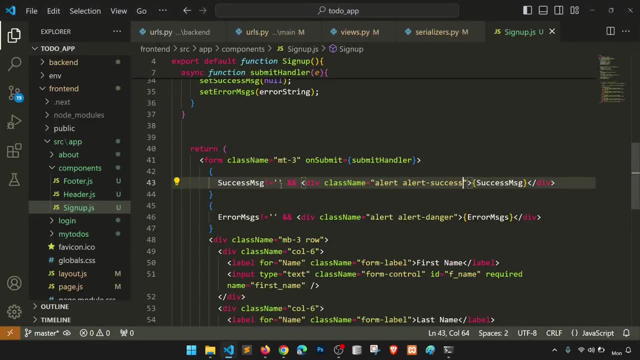 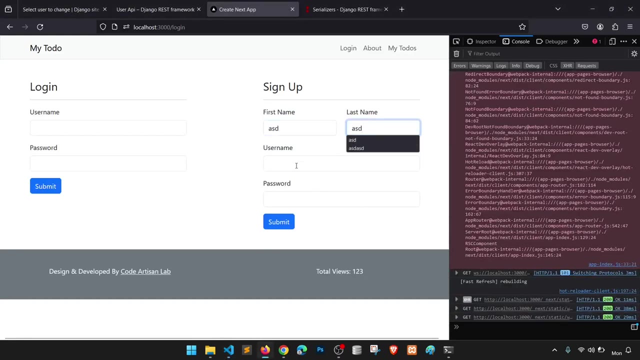 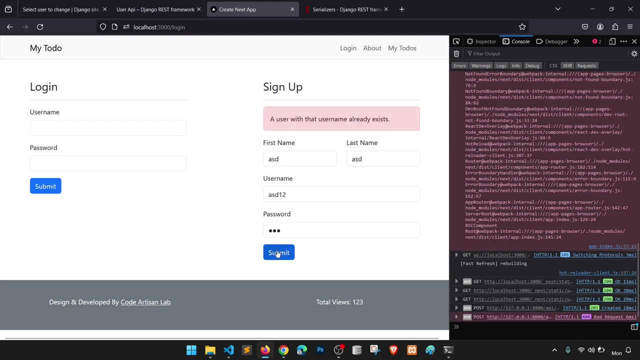 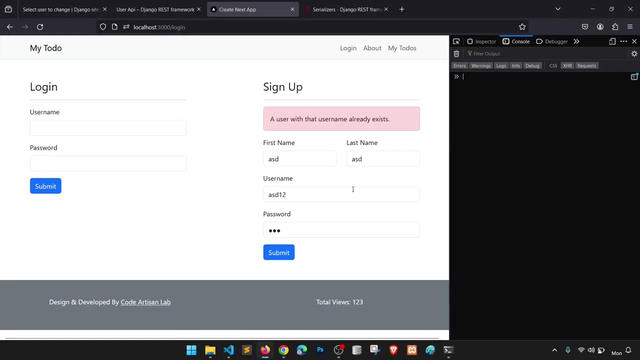 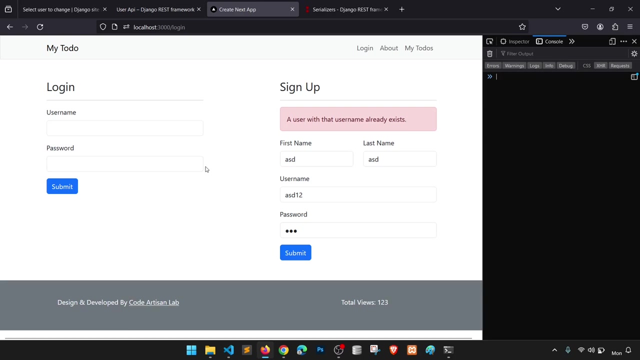 not equal to empty. then we have this thing. why this is showing this div? um, okay, let's see, copy, copy, paste. paste one, two, submit, right, it create. all right, so now it shows you all the errors and, uh, sorry, all the errors- and success messages also. right, so now we can move to the login and then my to-do list. okay, so let's start. 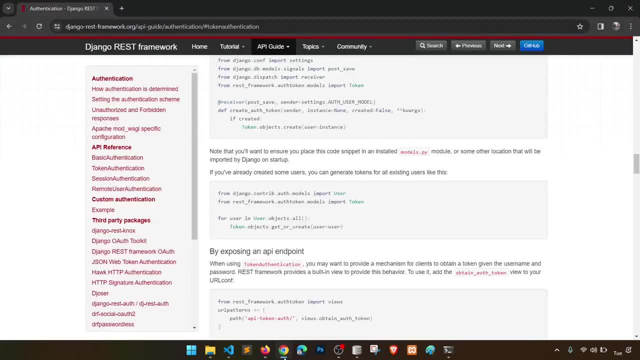 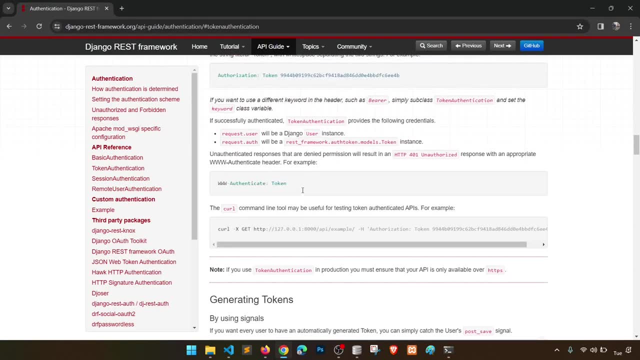 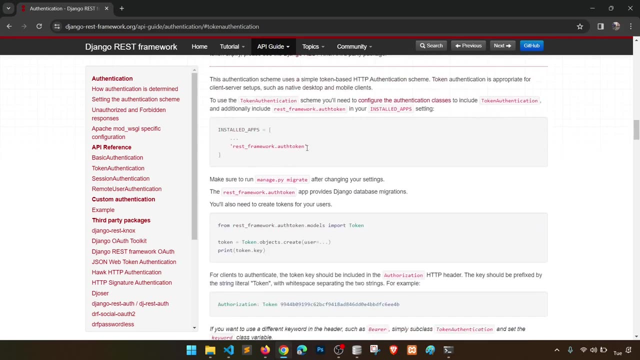 working on the login system. so for the login system, we need to pass the username and password and then, uh, it will give us a token, right, because we are using the token authentication. so first of all, we need to add this in our installed app. i think we added already. 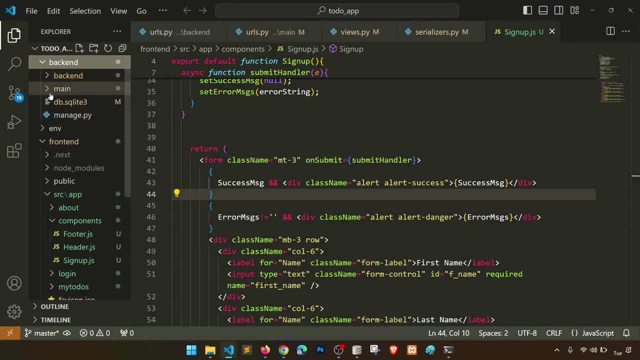 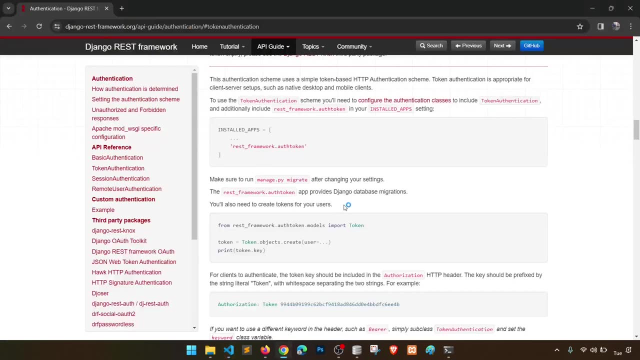 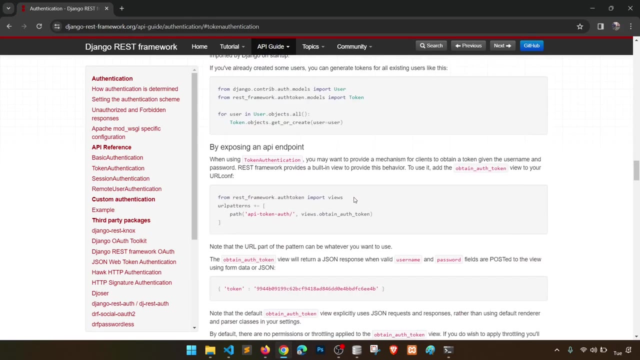 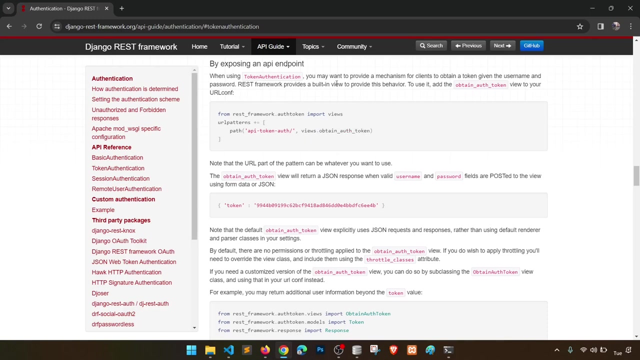 so let's check this. so if we go to backend, backend and settings, so here you can see that we have added right now. the second thing is we need to pass the username and password. right, so we will use the- uh, this thing, obtain auth token, right. so, uh, when using token authentication, you may want to. 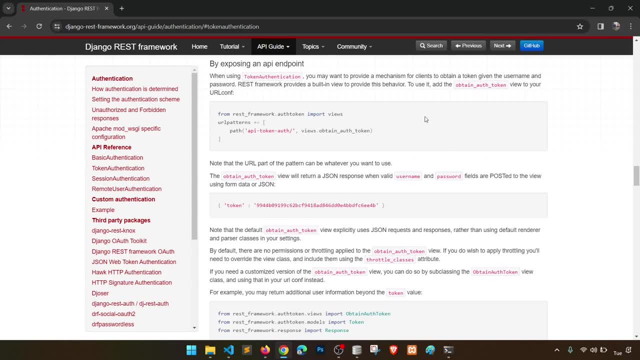 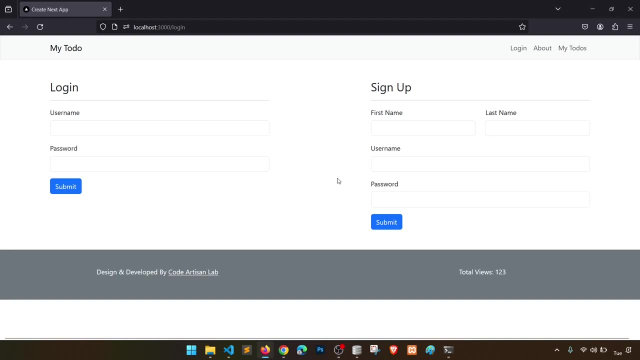 provide a mechanism for client to obtain token given this, so we need to pass username password. it will give us the token and this token will save. we will save in the local storage in the browser so that we can maintain the login state right and if token exists in the browser. 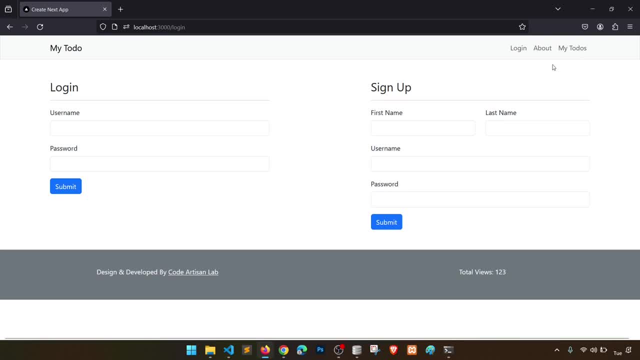 uh, then we can uh allow user to do the my to do actions, and if log out, then we will delete the local storage. so we are going to do this whole process in the login system, right? and if user is logged in, then, uh, user cannot access this login page, right? so, uh, let's, uh, first of all, let's. 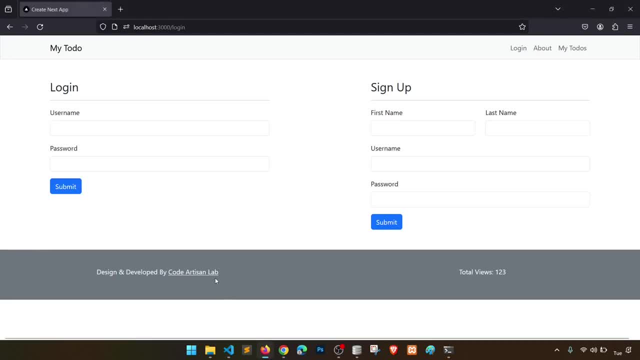 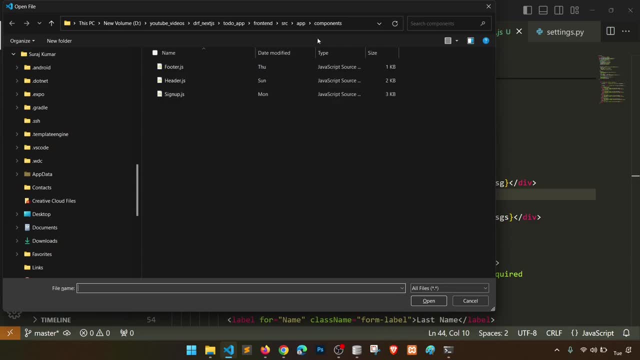 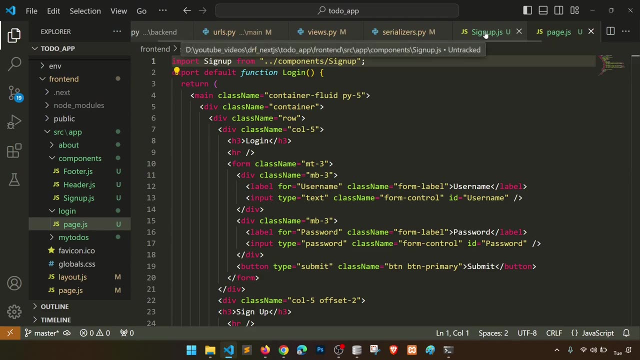 obtain the token with the username and password, right, let's open the login component. so here we have a sign up. and if we go to app and login, and here we have a page, right, so let's create the same thing as we have a sign up. so let's say: 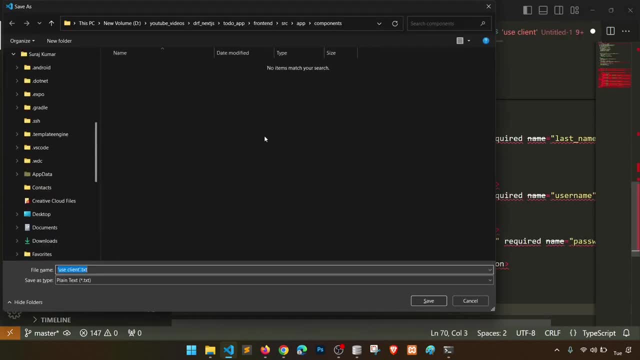 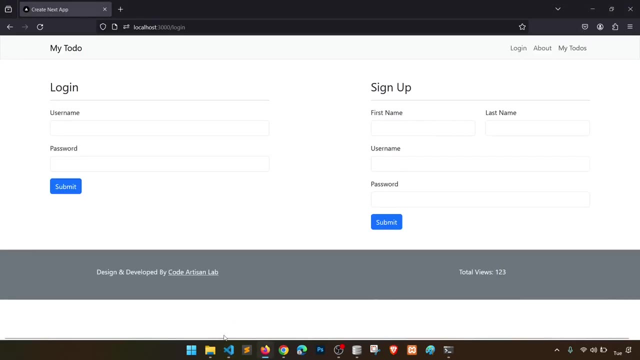 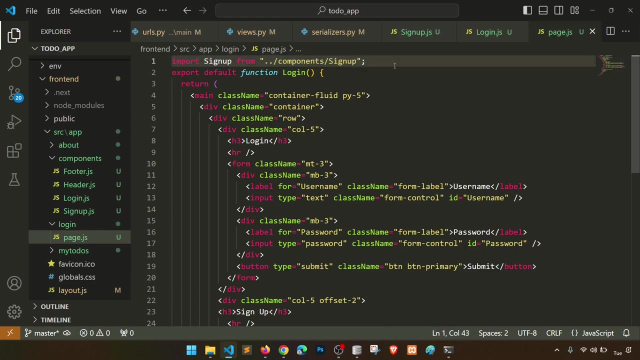 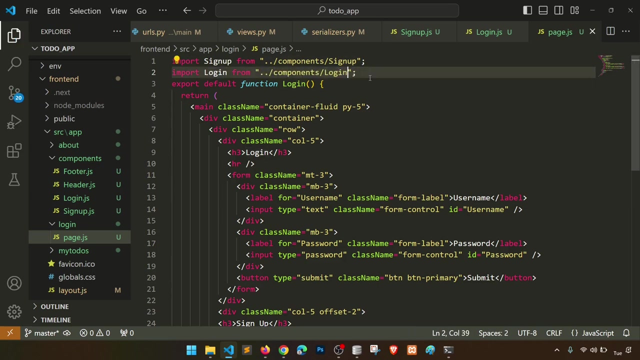 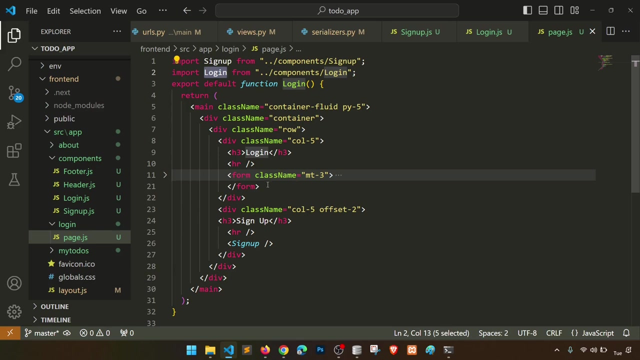 copy this and paste new and save this and we will say: loginjs right and uh, where is that? okay, so in the page we have we should have login component. so here we will use login correct and for the login here we have. so let's remove this form and i will simply say: 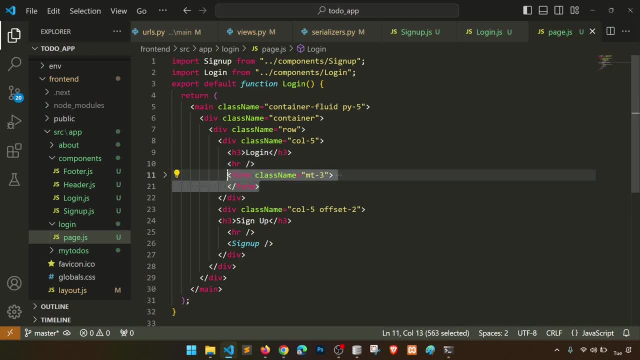 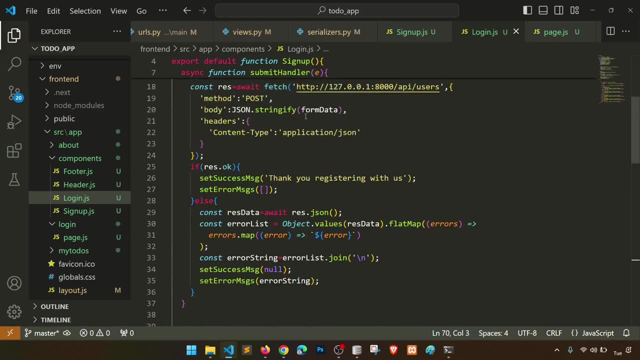 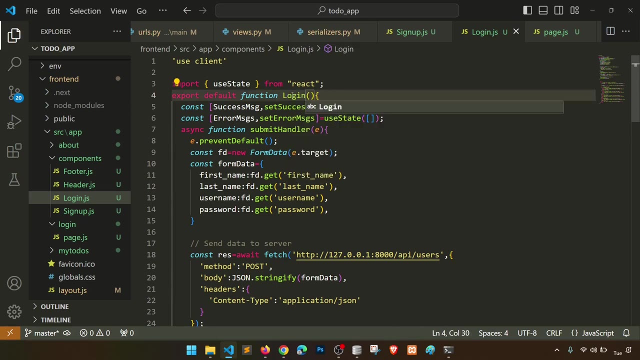 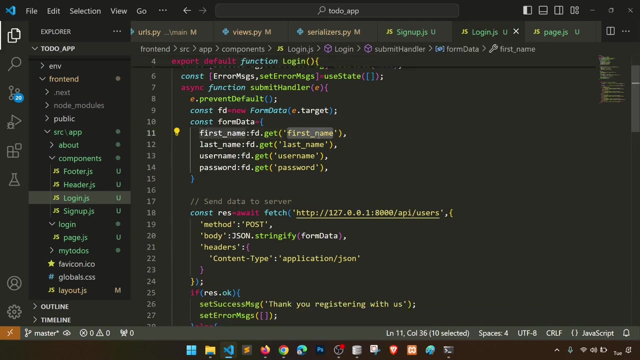 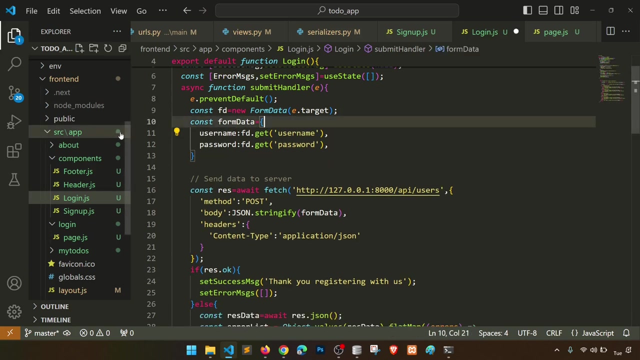 so here we have hr, this form right. so login component and in the login, what we need to do? let's first of all change the name, login, okay, so success message. error message is same. uh, form data: we just need to do username password. oh, we just remove this. two things right. method, post content, type, json, success. 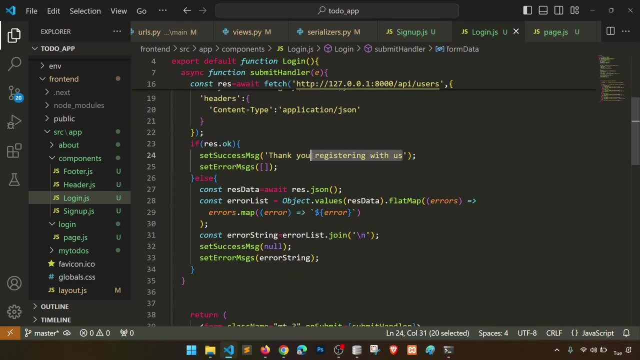 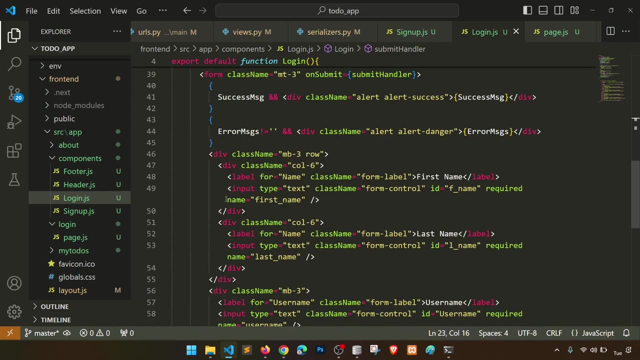 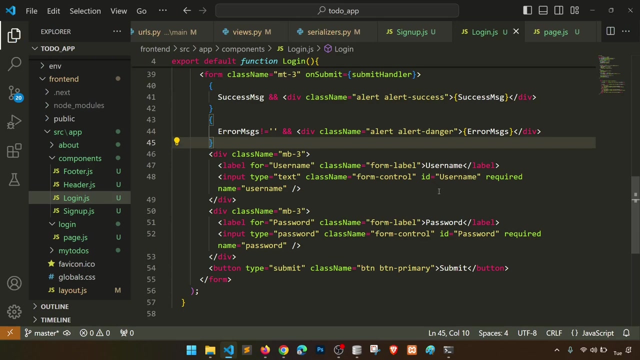 uh, thank you for login. let's keep it, then we will. later we will redirect. uh, we have error list. okay, we are showing the error. uh, submit handler. no need for the? uh this row, no need for this row. so username and password and then submit. so let's check the front end. uh, what it is saying. login to. 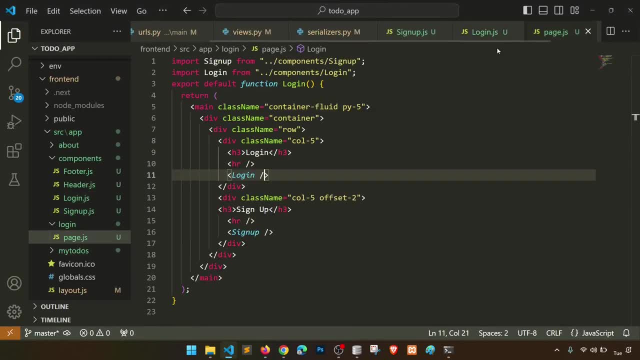 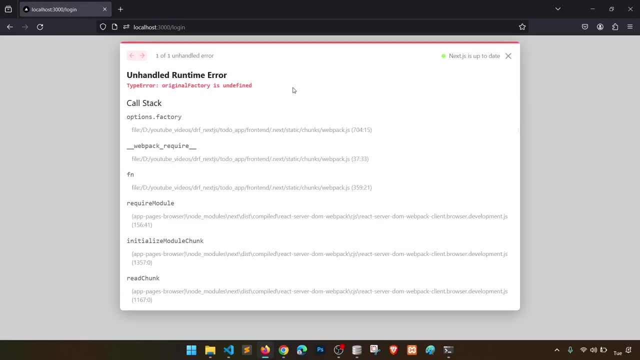 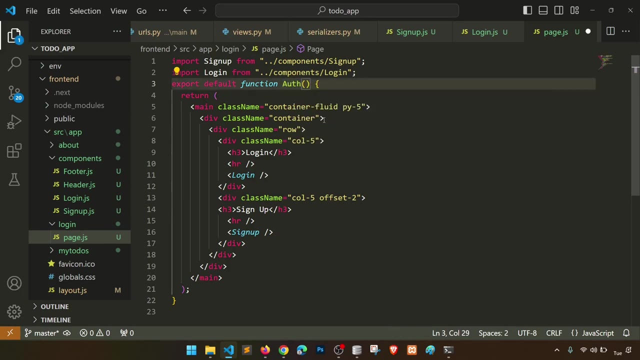 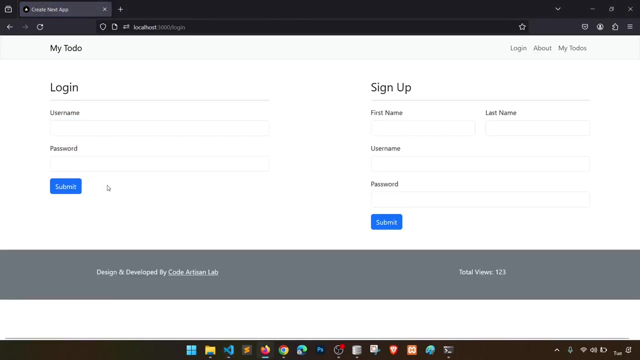 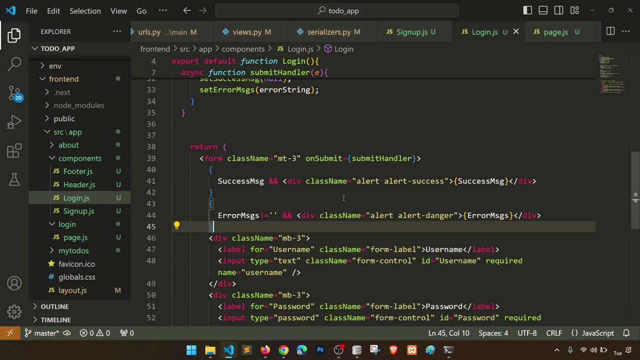 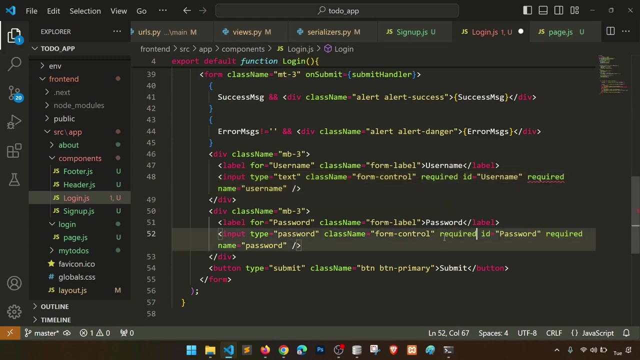 has already been declared okay. so we'll go to page and we'll say page original factory next up to date, uh what we can say. authentication: all right, so user element, password and we have a submit. uh, one more thing. uh, let's do the basic things like this field is required, right, and password is also required. 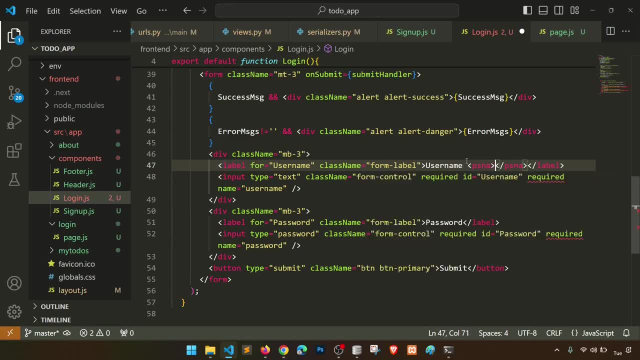 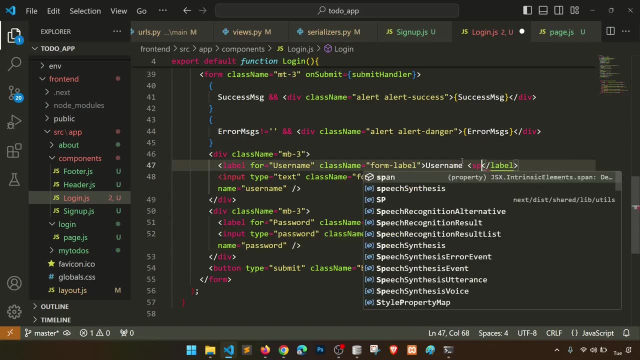 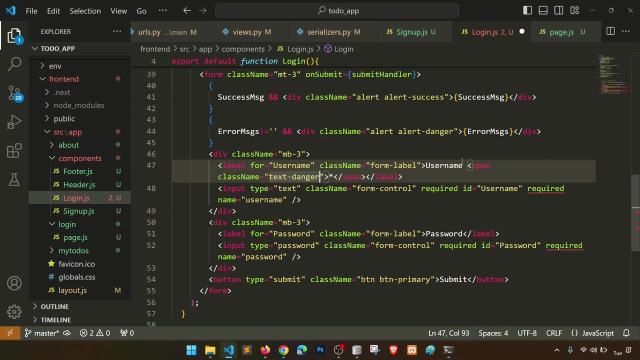 and let's also do one more thing: uh, let's do the span, right. so what we are going to do here, span and aesthetic sign and then class text, danger, right. and uh, we'll do copy this: required equal to required right space. why this is showing multiple entry with the same name? 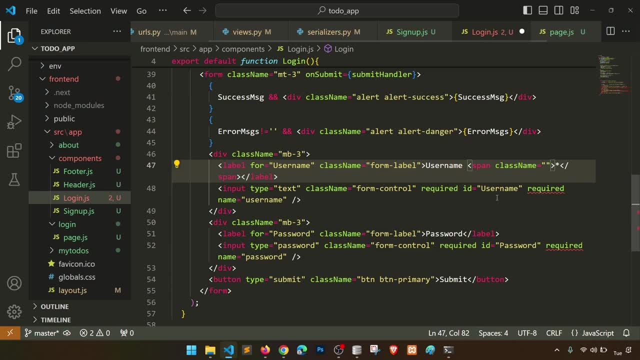 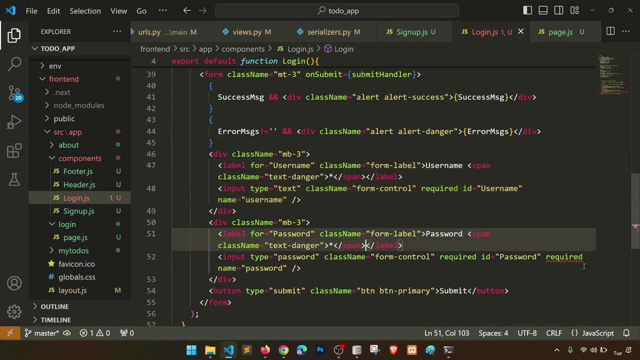 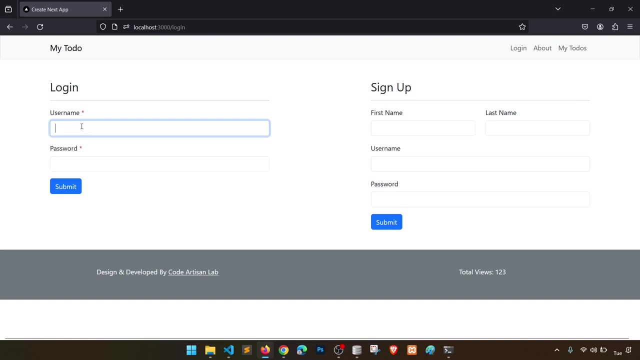 oh, here, no need to do this. let's remove this. let's say text danger and we'll copy this one. copy this one and paste here. let's remove this. we already done, i think. okay, so username, password: click here so it will show the. uh, it will show us the that this field is required we need to. 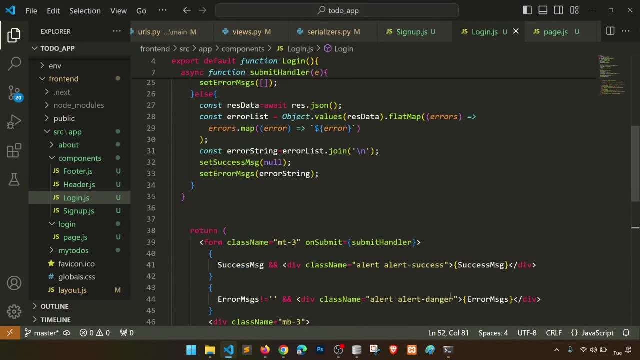 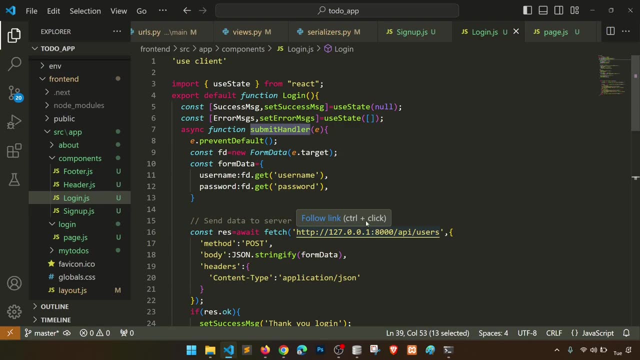 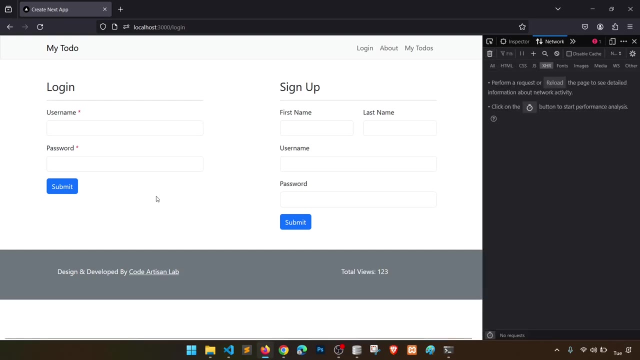 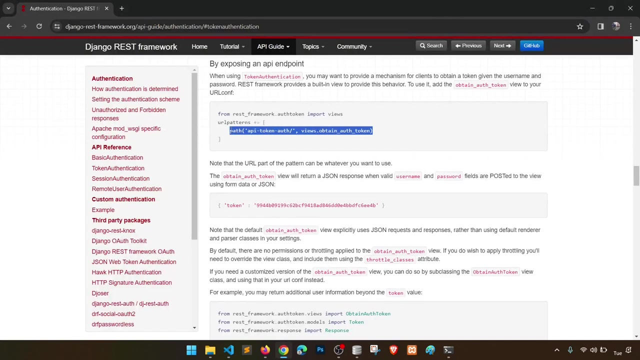 submit this. okay, so submit, this is submit handler. and uh, in the submit handler. this way we are sending this data. okay, so submit, this is submit handler. and uh, in the submit handler. this way we are sending this data. so if we go to network tab and we need to do one thing, we need to copy this one and open our 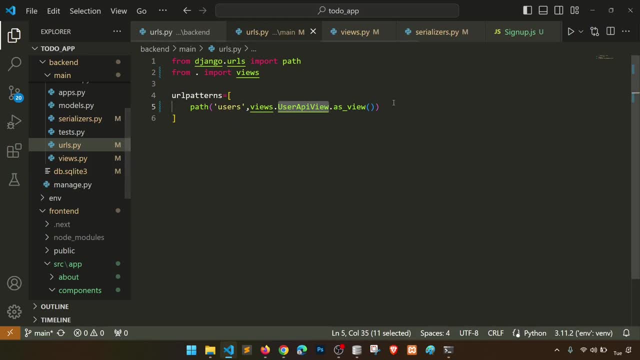 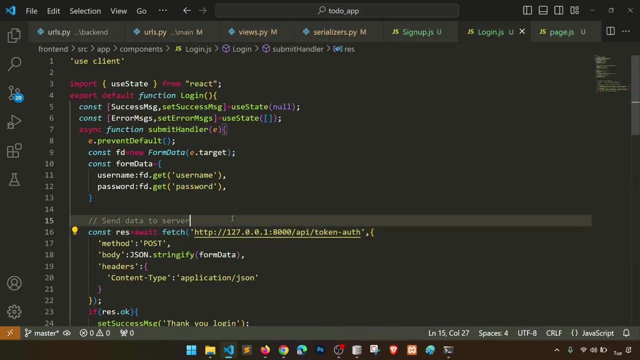 app level urls page. this one paste here and from the rest framework we will go up at this view. okay, token the token authentication- right, so what we will do? token auth. so let's go to login and we'll say: token auth- right, so we are sending the data. username, password. 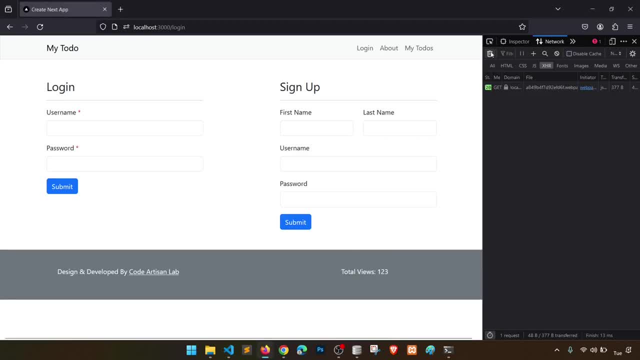 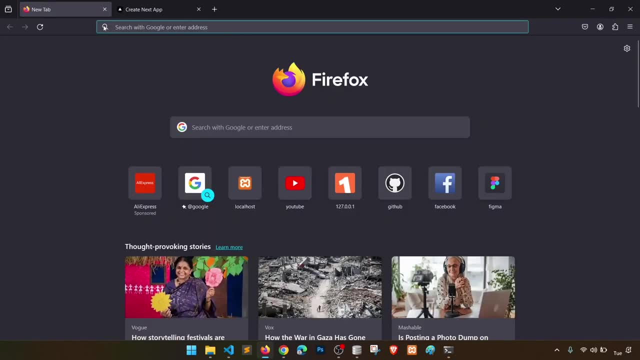 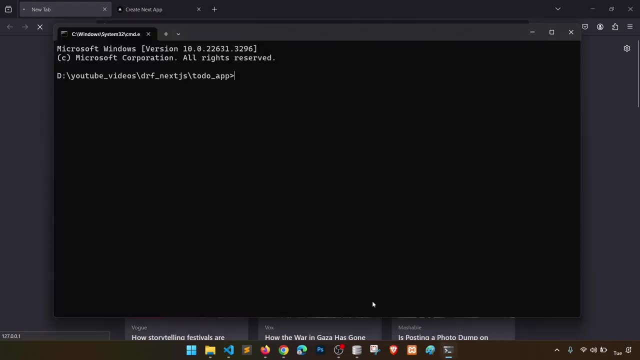 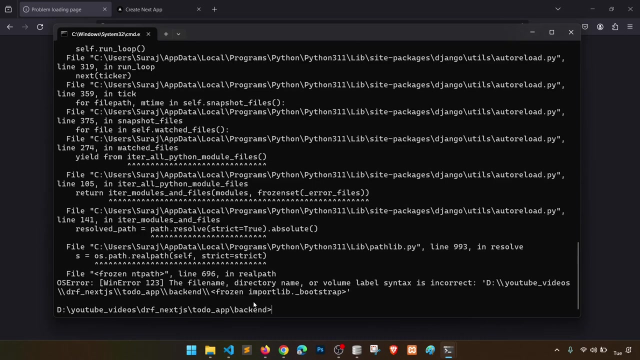 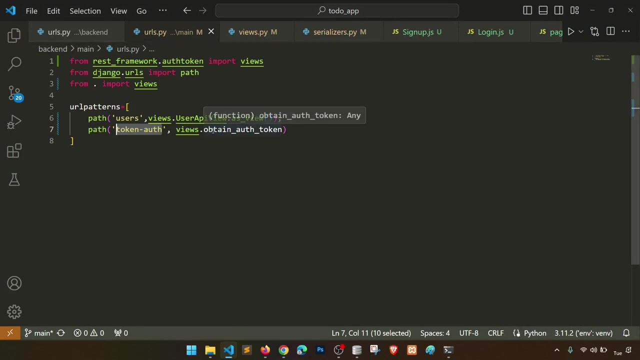 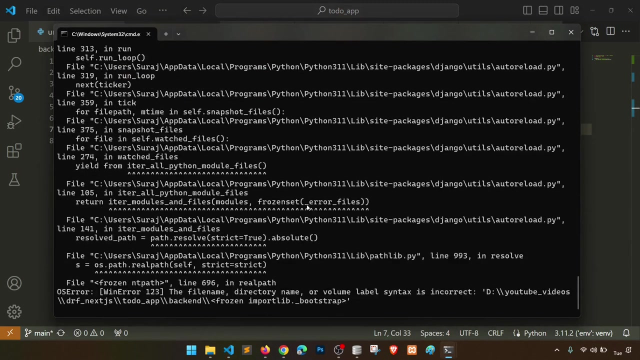 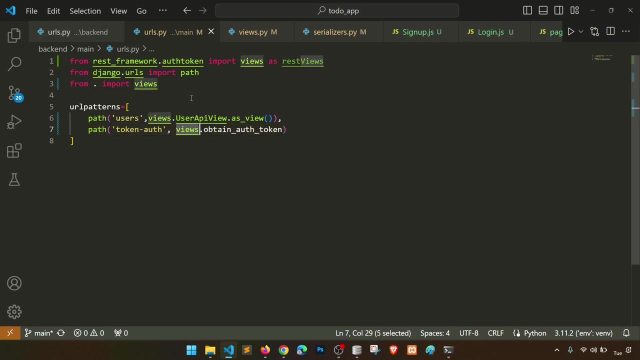 it should show the success message. let's see so how much data we have. let's do this. let's check this. okay, so, cd backend, py manage, dot py, run server. hmm, what are they saying um viewsoh as rest views, it should not be the same right. still, let's do one thing. 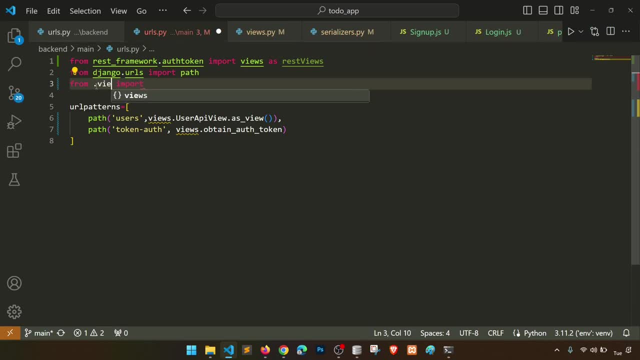 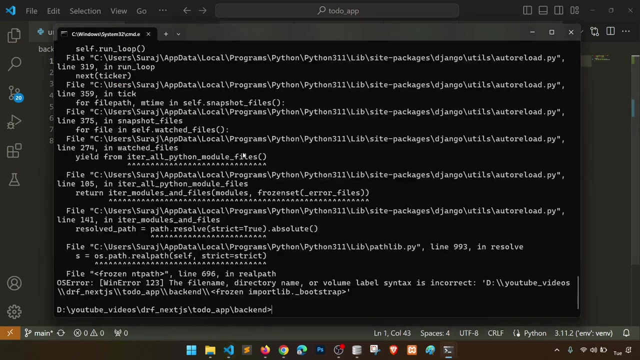 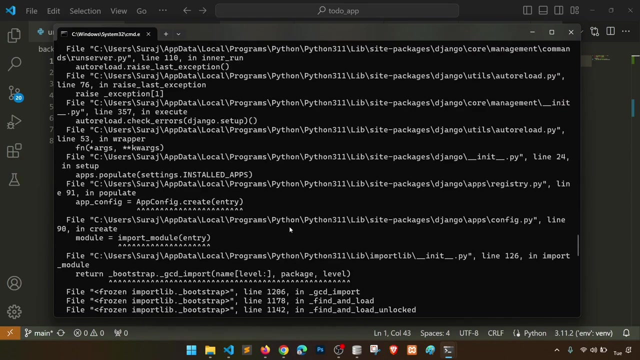 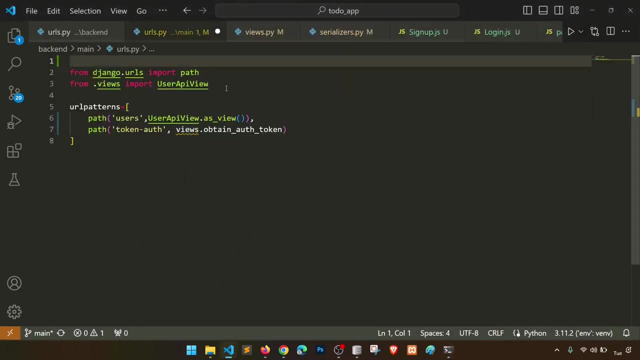 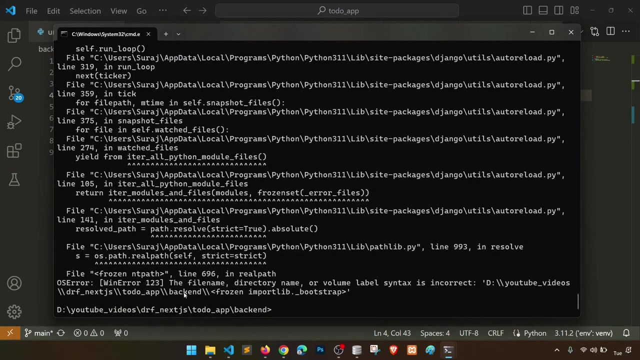 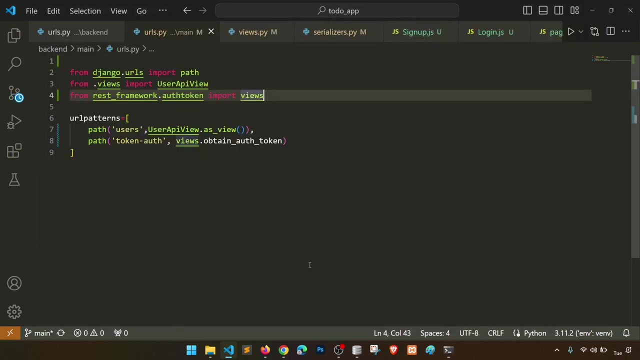 then views: import user API views: correct. okay, and let's keep it as a views. now let's see still fishing the facing the issue. let's do anything then let's open this and paste it here: frozen. the final ednaе was index incorrect bootstrap. okay, let's check it. 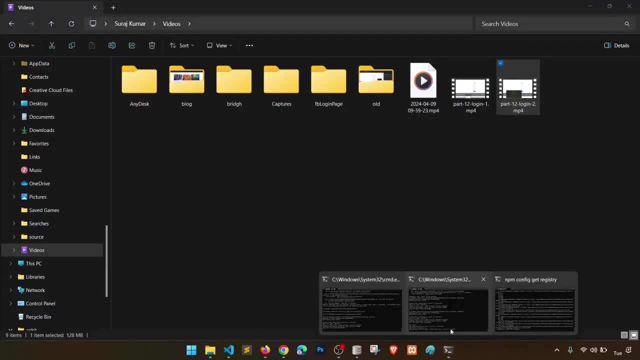 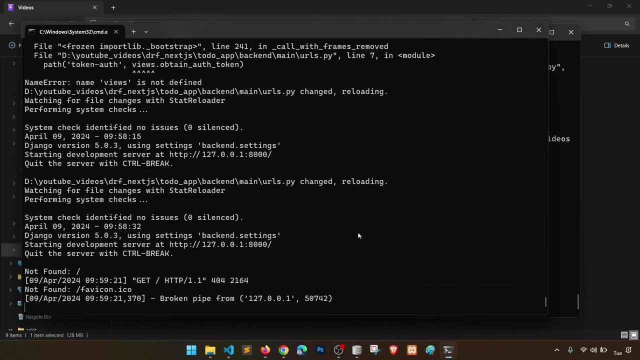 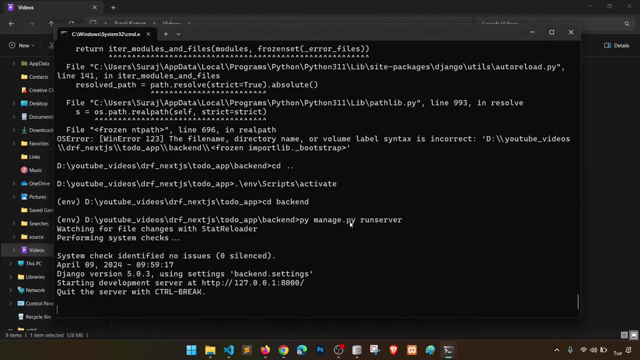 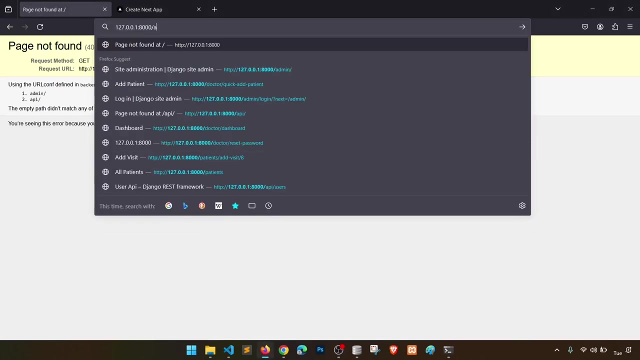 okay. so actually the issue was we didn't activate into the virtual environment or environment, or did we? i think we have created two things. okay, let's remove one terminal. so i was running the run server without activating the virtual environment, but it's working. so now, if we go to api, okay, so no need to go to api, we need to go to admin. 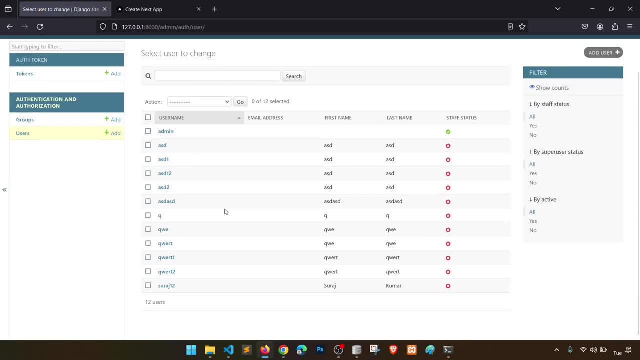 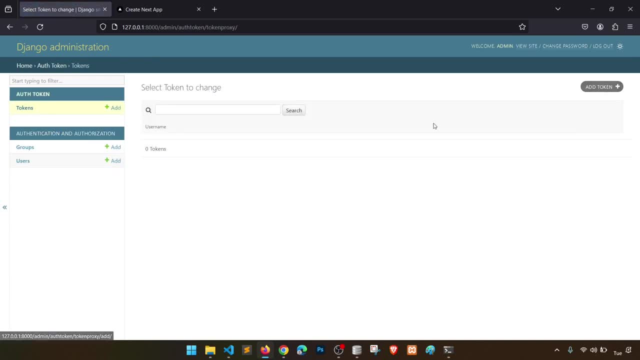 and we need to go to users and here we have a admin right and let's go to token. so we don't have any token. we will create that. we will add the functionality that how this token will originate when we sign up the user. but let's create one token for the admin save. so this was. 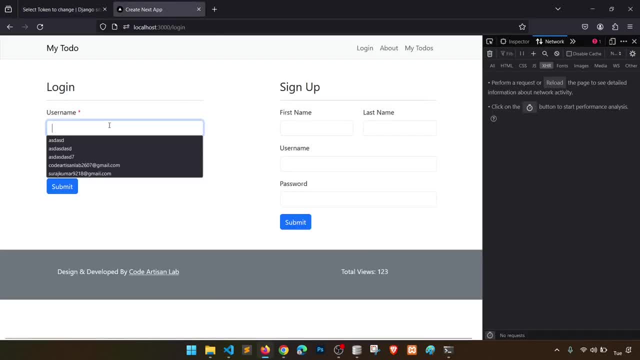 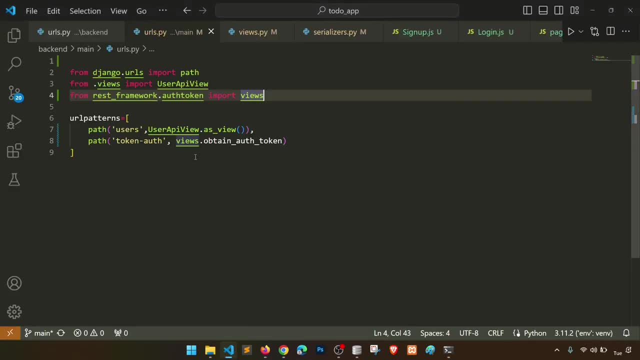 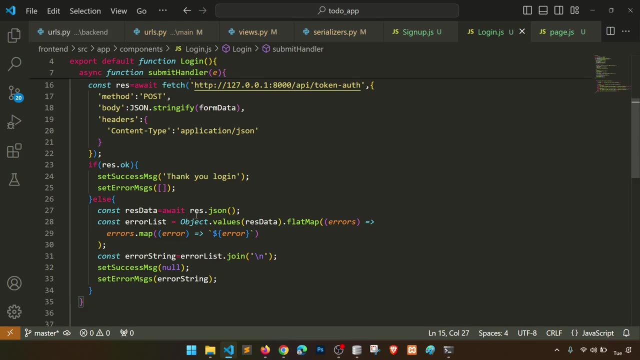 this is the token, and let's put the username and password for this user and we will see that what it is returned, right? so so the url will be this: copy and url is: okay, uh, uh, response dot data. okay, so, uh, let's do one thing: if response dot, okay, then let's console the response. let's copy this one and paste it here. 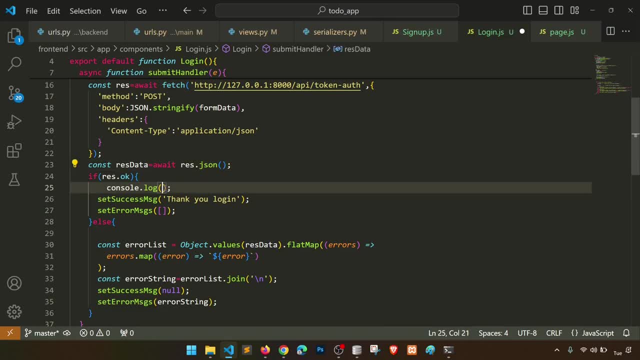 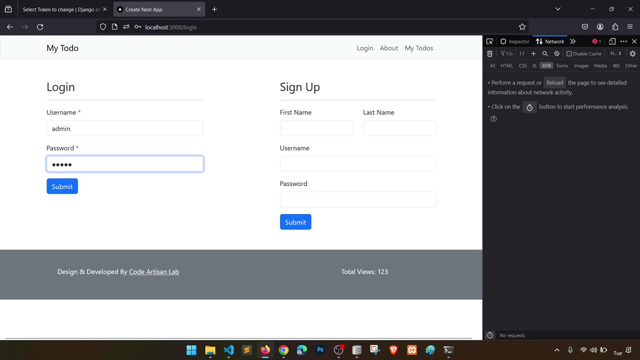 right and copy this right and paste it here. right, and uh, let's see how it is what it is returning. okay, so we'll say: username, password, submit tokenauts request. uh response. okay, so it is returning the token, correct, so. and now, and also it is saying: uh, thank you for log, right, so if it is returning the token, 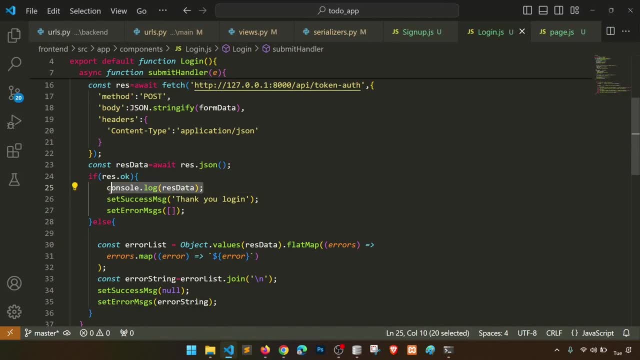 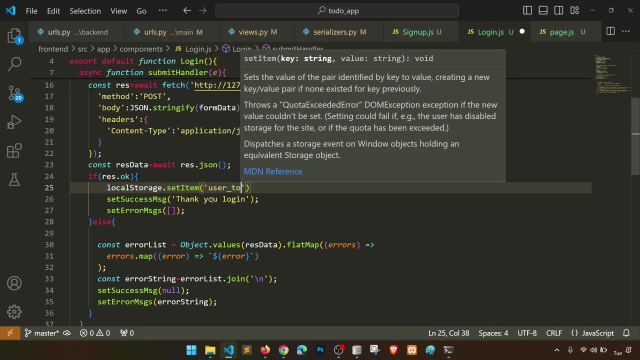 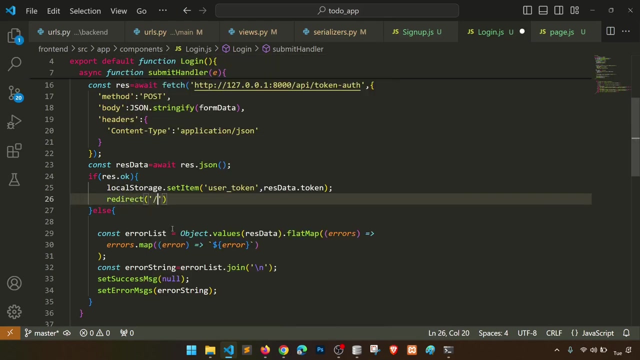 so what we will do. if response is okay, then, uh, we will say local storage, dot set item user token: right user token and response: dot data, dot token correct and no need to do these things. uh, but we will redirect to- let's redirect to home page, right? so return or no need to return. 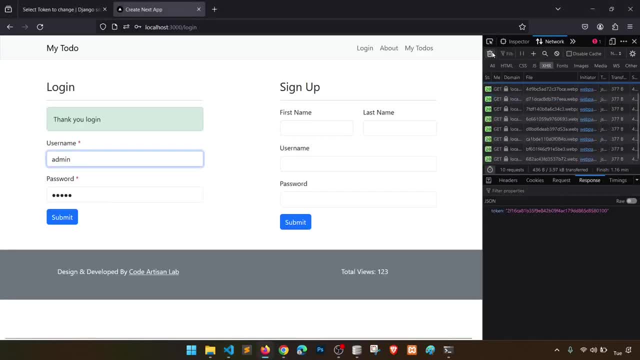 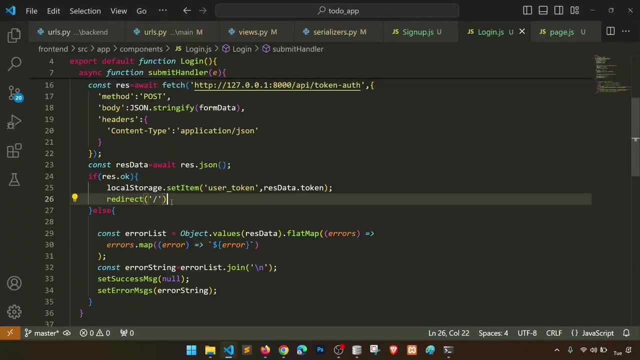 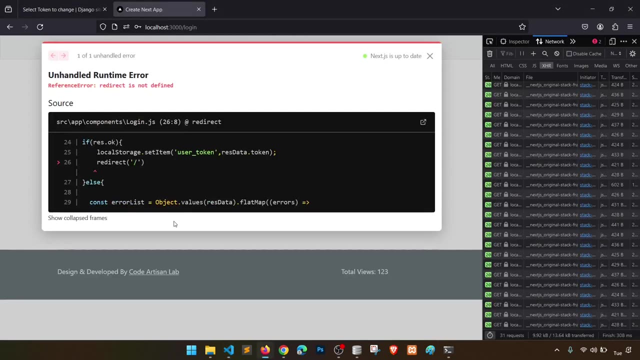 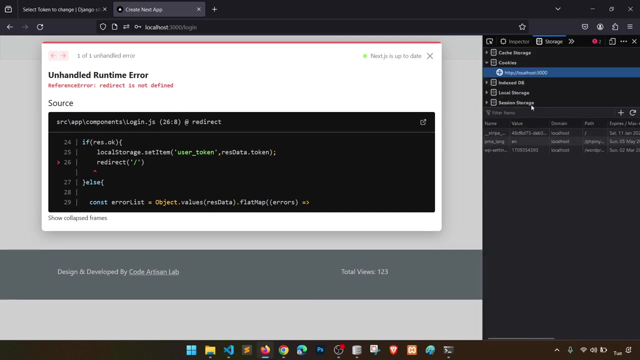 just redirect to home page, correct? so click here. what is the error? okay? so, uh, there is a different thing. that will uh a redirection. we can check it, so okay. so let's uh check that uh, local storage is working or not. so we'll go to uh storage and we'll go to local storage. uh, we have this one and uh, we can go to. 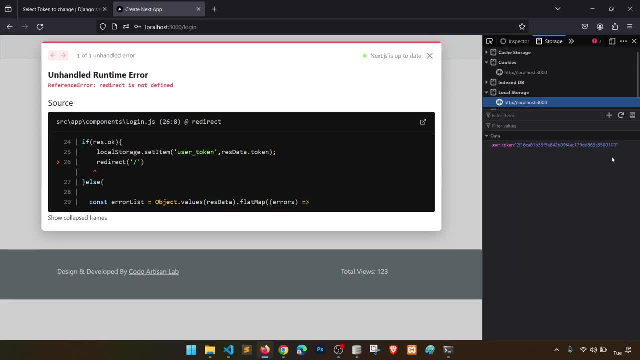 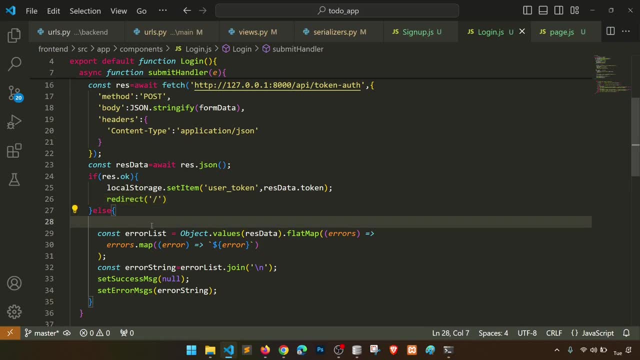 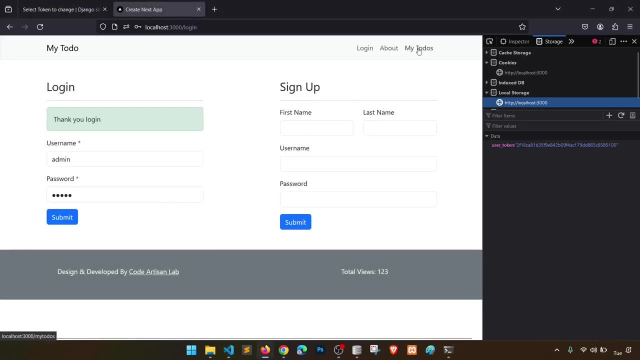 a user token. here you can see this is user token right and we'll see that why this redirect is not working. okay, and if user token is exist, then, uh, we will redirect user to the my to-do list. right, and this micro list only open if user token is exist. correct, and we'll show the logout thing. okay. 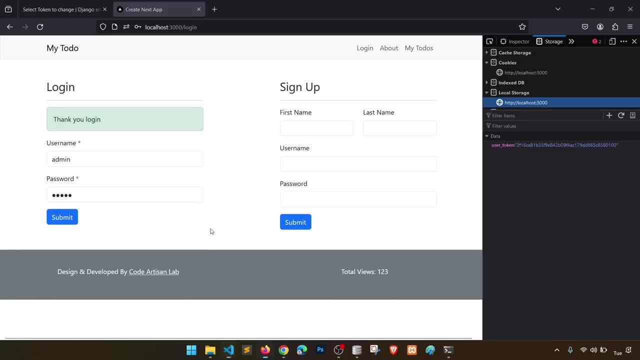 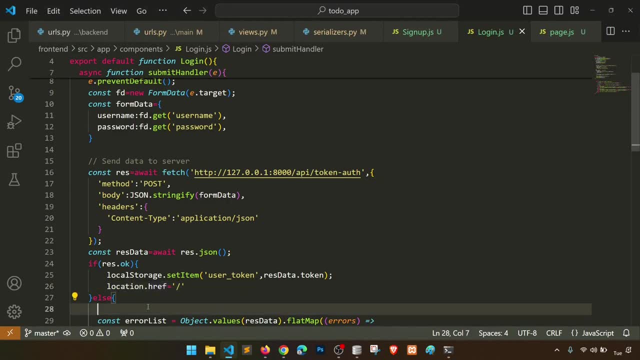 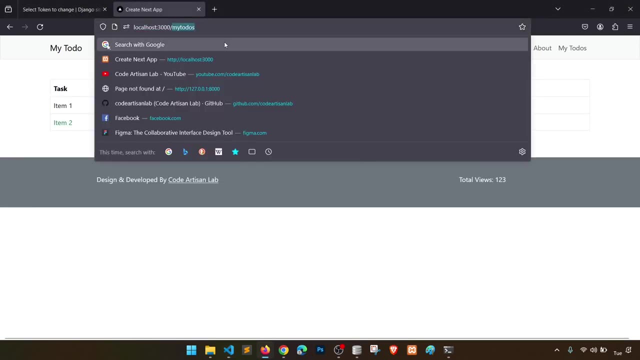 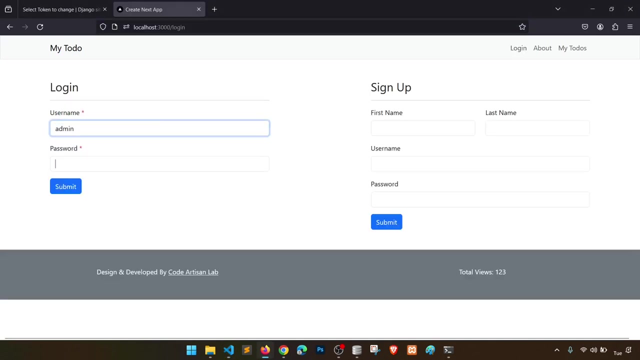 so let's see why this redirect is not working. we applied the old school method here: location dot, href, and it will redirect to the home page, right, but it should redirect to the my to-do list actually. so if we say my to-do's- right, so here, so let's go to here and login and submit and it will go to my to-do's. 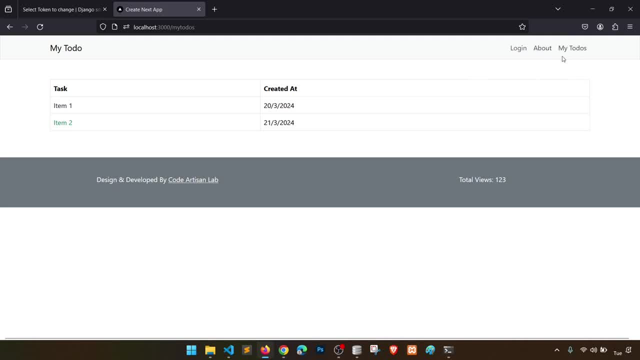 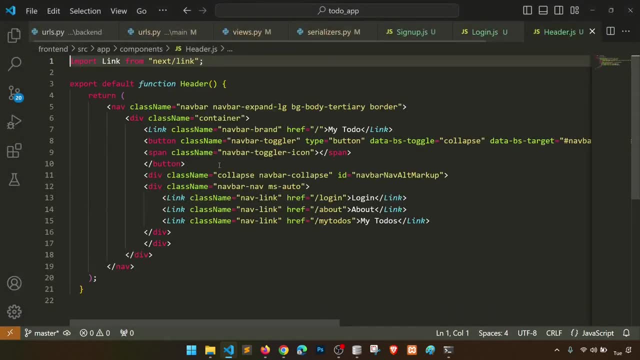 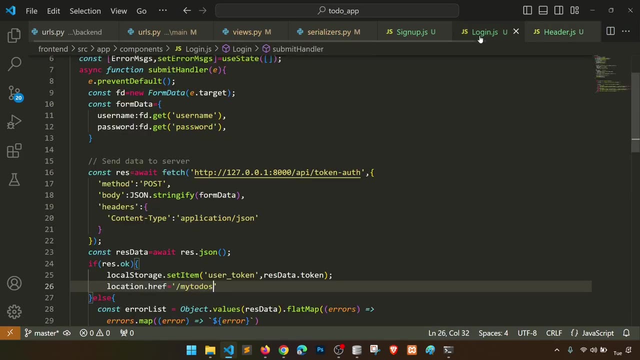 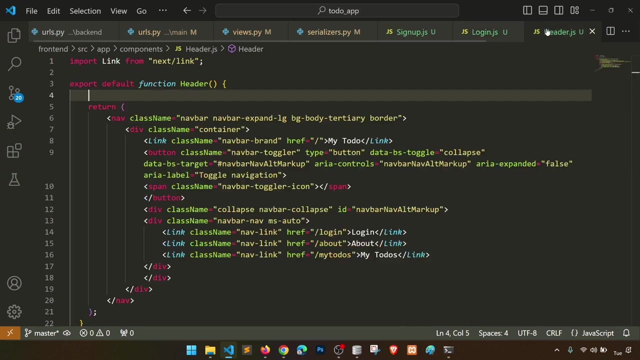 right. so now, when you also need to change the, the things. so if you go here and if we go to components header, so here we will fetch the data right. so we will see, uh, we will get the this one. copy this, paste it here. we will say: 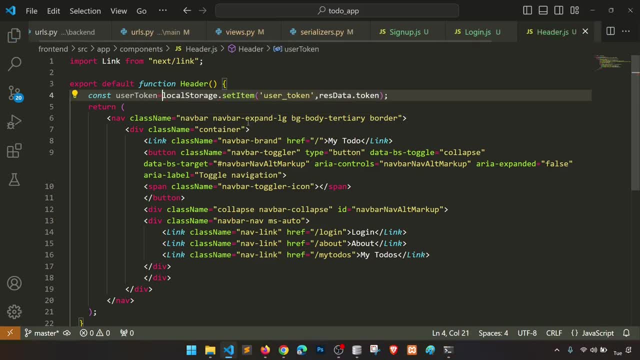 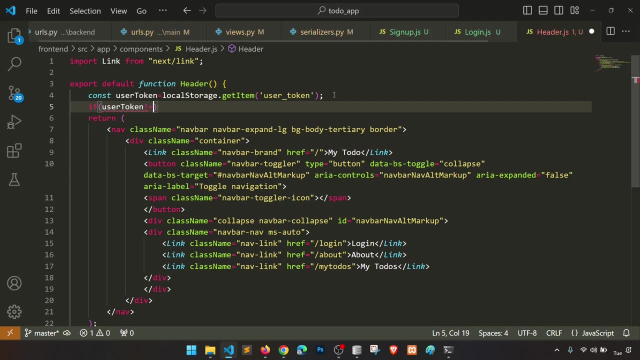 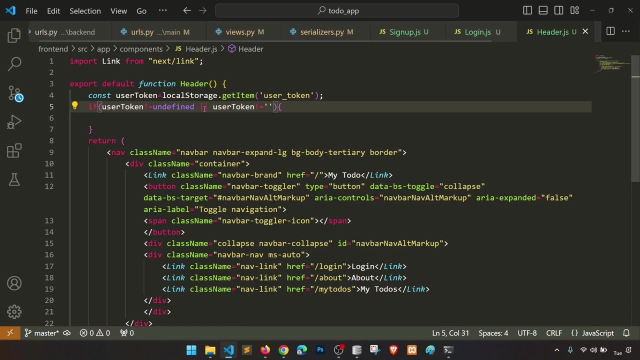 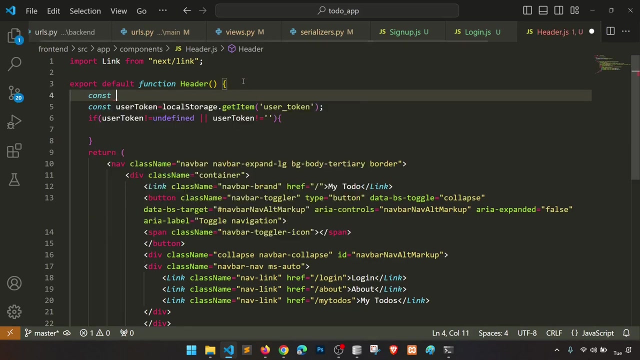 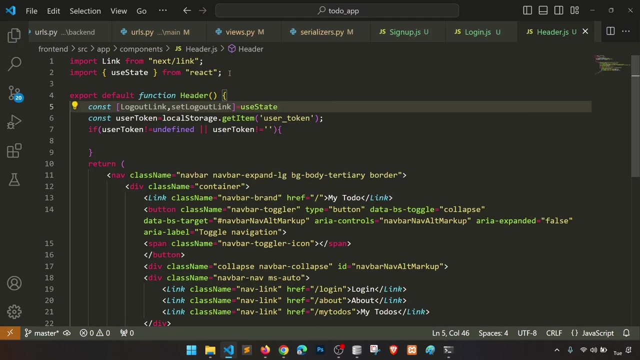 constant user token and we will say: get item right. and uh, from this. and we will say: if user token not equal to undefined or user token not equal to empty, then then we will show the logout link. so for the logout let's create the logout link. so we will say: constant log out link, set logout link equal to use state, right here, okay. 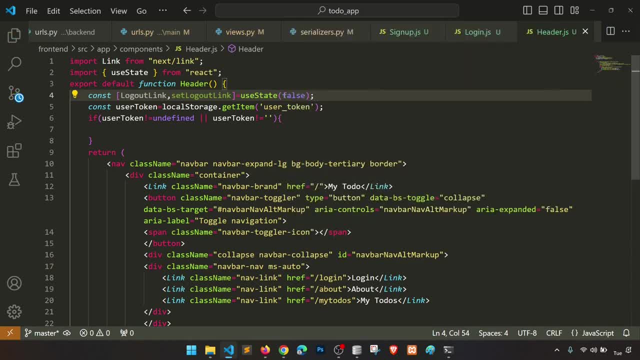 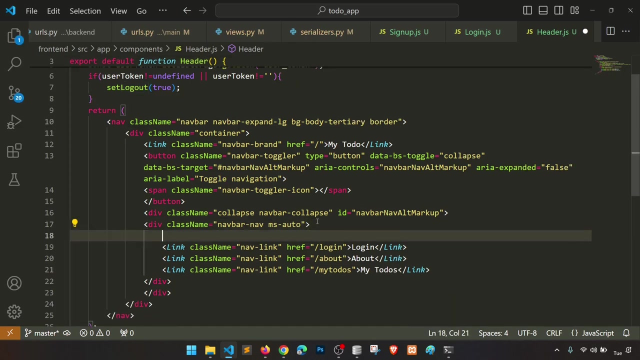 so false by default. false, let's say not say link, just set logo, okay, and then we can set log out through, correct, okay, and we can see here: log out, and then we can show this link to log out, if this, if not, uh, okay. so if log out, then we will show this. 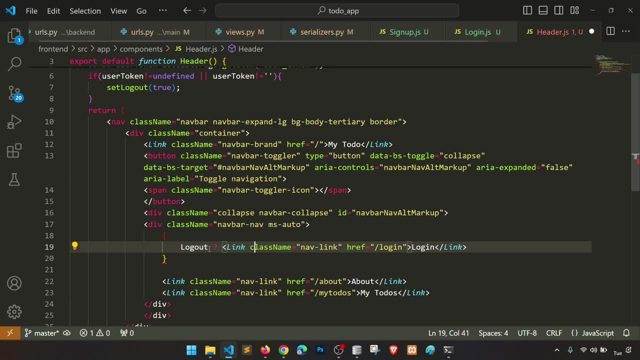 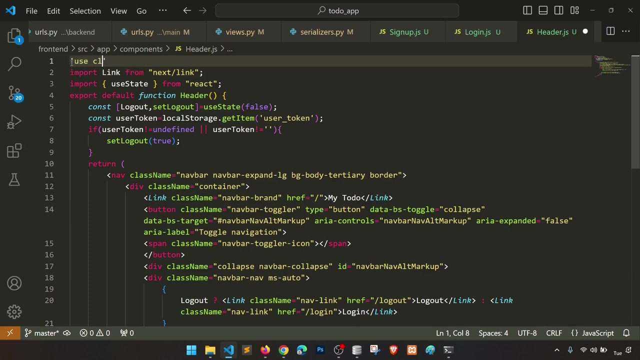 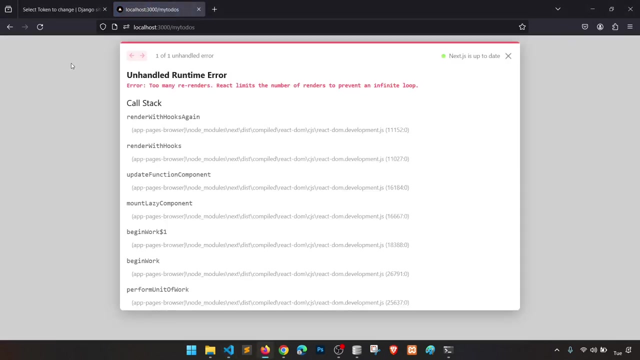 this right, uh, else we will show this okay. so we will say log out, log out and this is login right, okay, so what we need to do? we need to do this as a use client: correct too many renders directly on the number of error to private infinite loop. 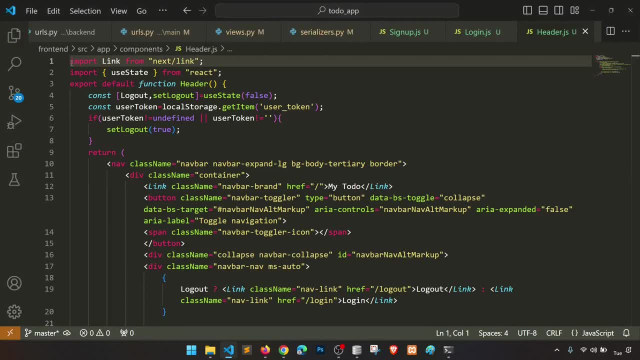 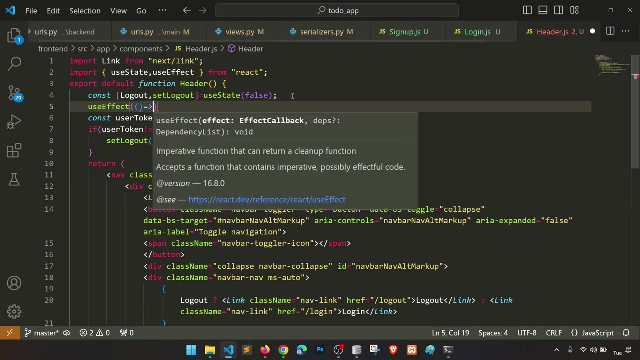 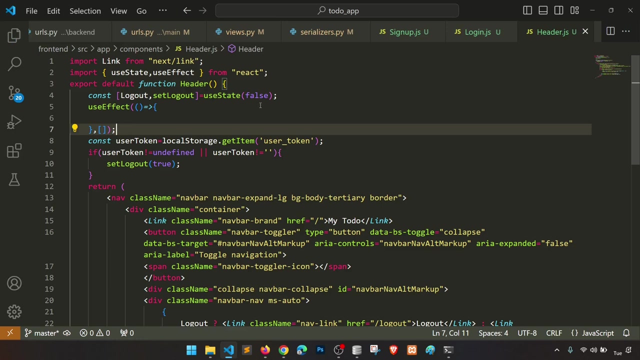 okay. so what we need to do here, we need to run this in the use effect. okay. so let's use effect okay, and then here we will run the function right. so no dependency. so we will say this one right and in the use effect we will do this thing. 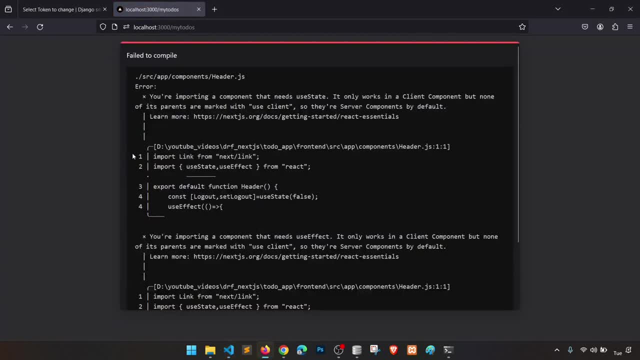 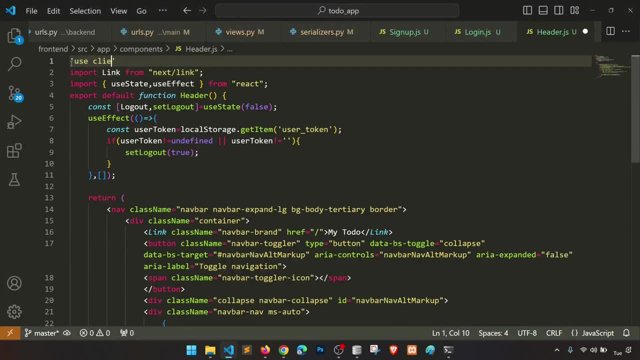 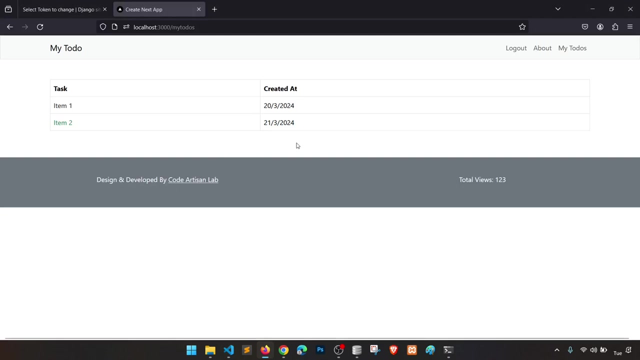 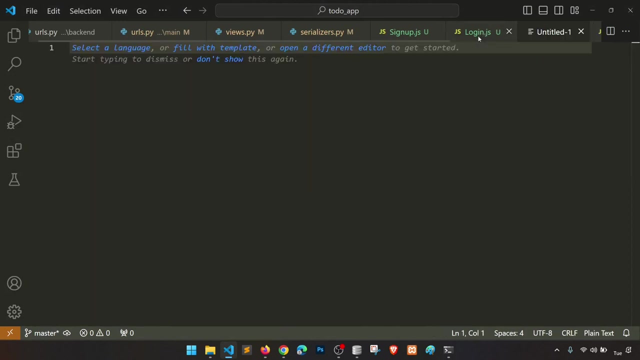 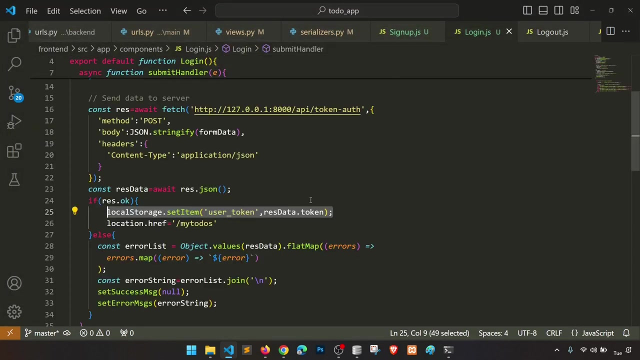 okay, all right. so we will say here: use line, okay, because use it only work in the client component, right, all right. so here we have data and here you can see logout. so let's create a one more thing: logout component. save logoutjs and in the logout component what we will do. 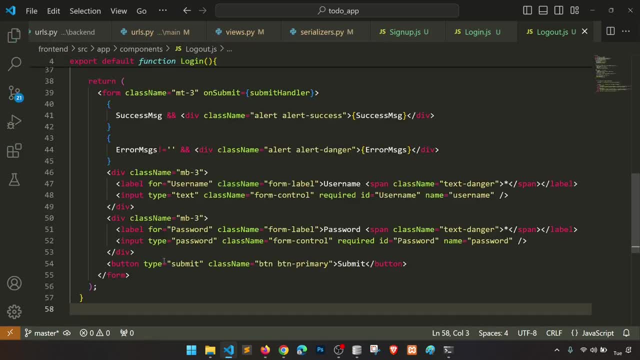 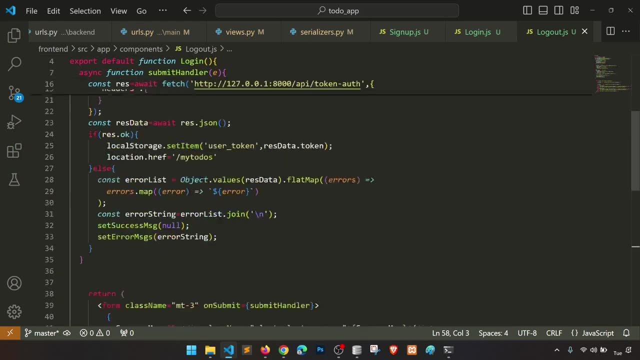 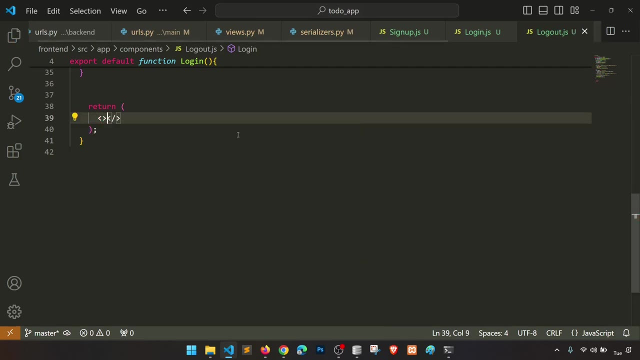 we will remove the data correct. so in the logout, when it comes to the logout component, when we will not do anything, here let's keep it as simple, this one, and just perform the action. so let's remove all the things. and here let's say no need to use client or do anything. uh, what we will do here, we just remove local storage dot. 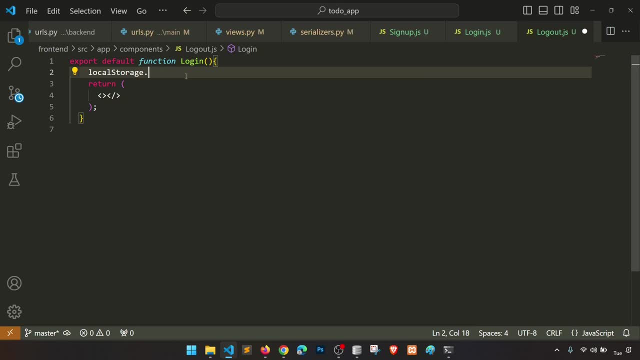 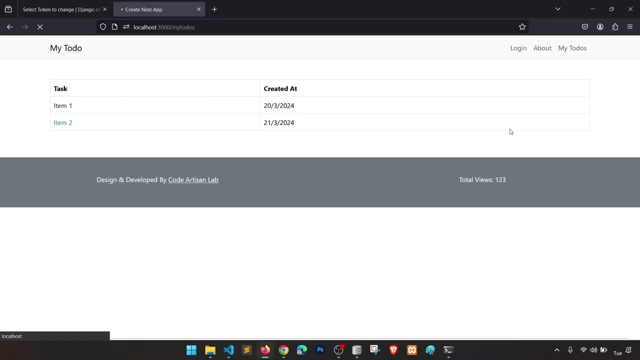 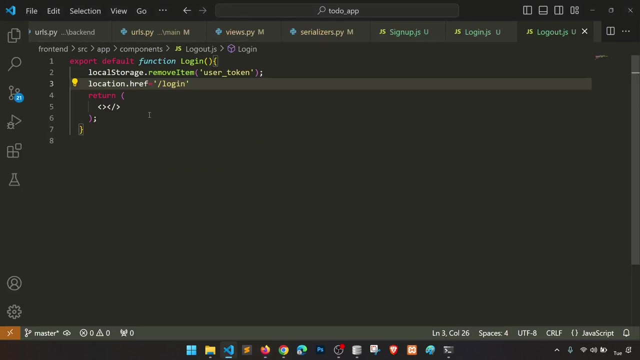 uh, local storage dot um. set item. or we can say remove item user token and then we will redirect this picture here to log correct. so let's see how this is working. so when we click on this log out, it will. it is going to log out, but it is not redirecting to the user. oh, oh sorry. 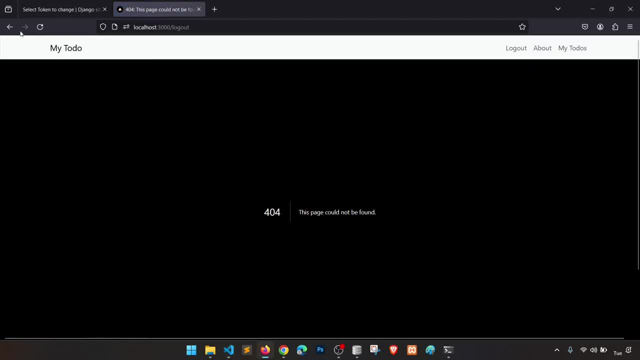 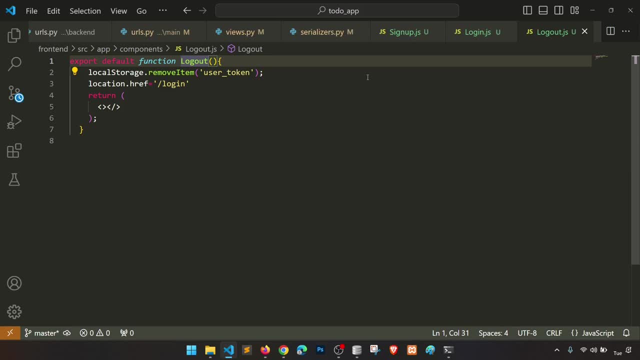 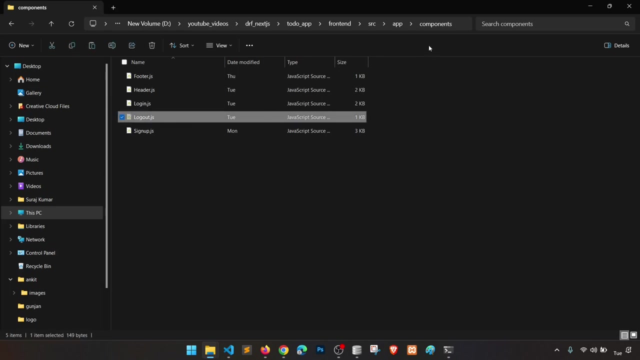 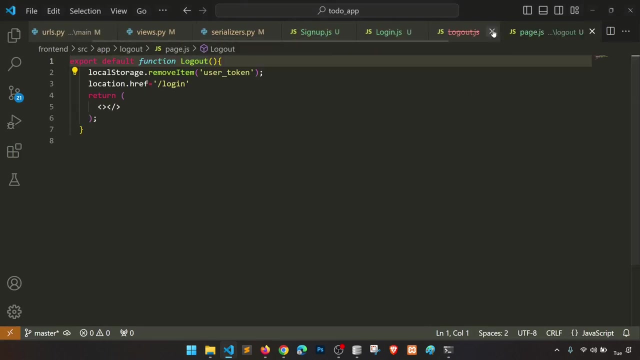 logout. sorry, logout page is not found. it is saying component. actually this should be log out, not a, not component, but it should be log out page. so let's do front end source, let's. uh, uh, let's go to app. uh, sorry, here let's create logout and in the logout paste it and name it page pagejs, and uh, it should work. so login, sorry. 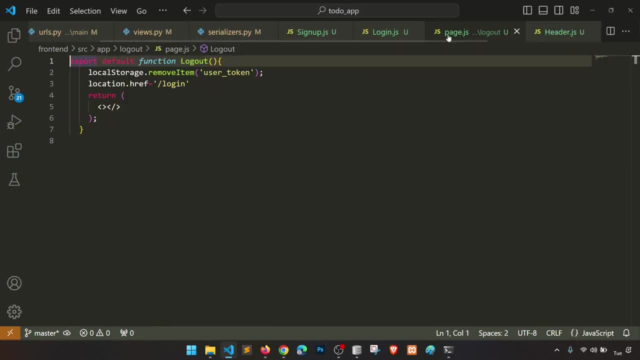 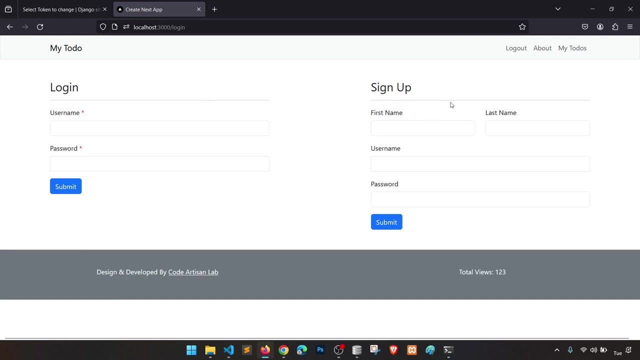 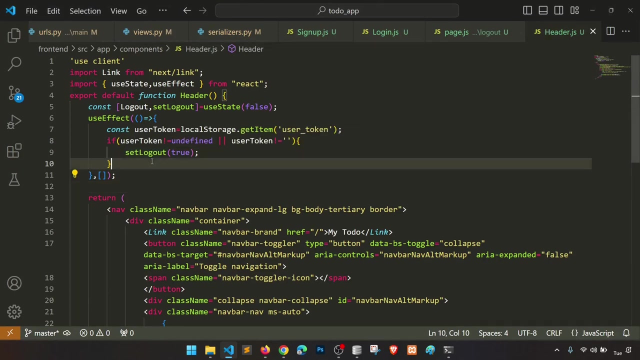 so when we click on this logout, then it will go to this page, right, so let's go here. local storage is not defined. where is that? uh? uh, local storage is not defined. okay, so this is server component. let's say use client. all right, so this is coming here. and uh, why this is showing header? uh, if let's. 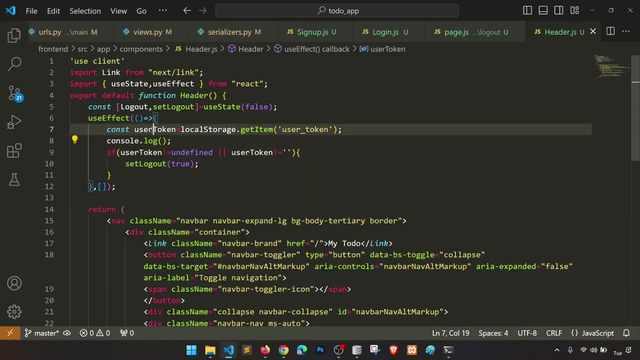 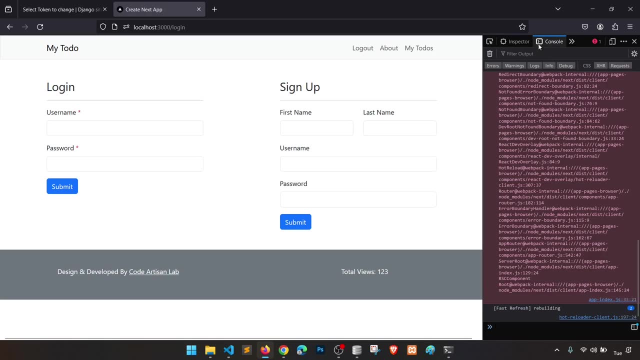 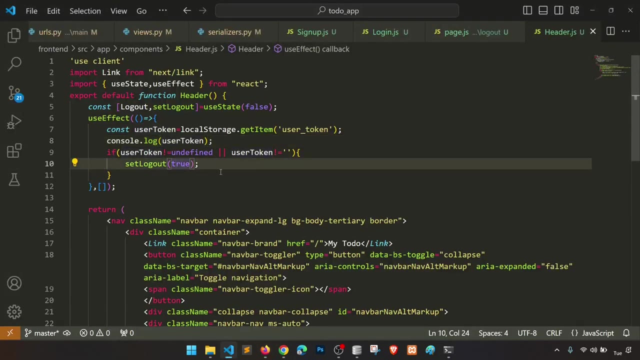 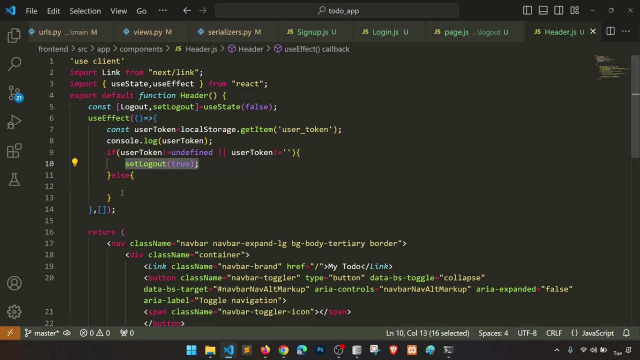 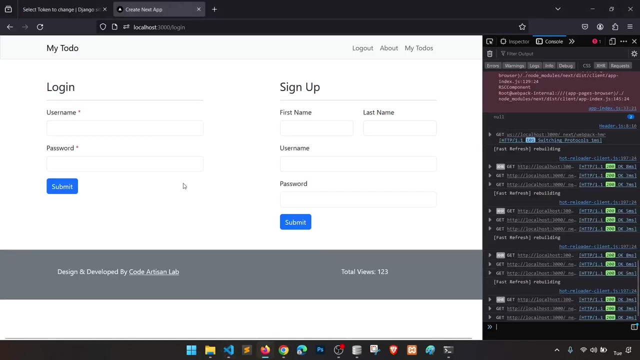 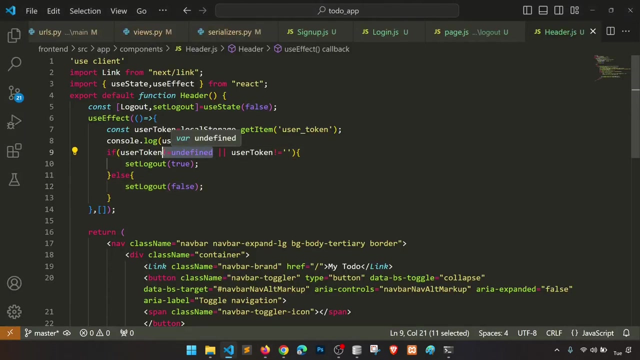 console this user token. oh sorry, console this user token. uh, this is null. so if uh set logout to true, else set logout false, false. so we are saying if user token equal, equal to uh, not equal to null or not equal to empty, then true, else it will false. uh, this is user token and uh user token console. and in this use effect, 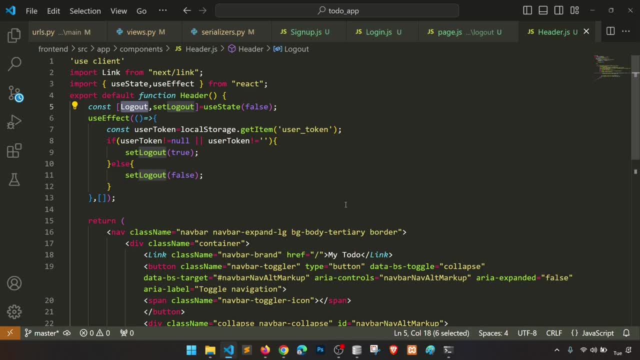 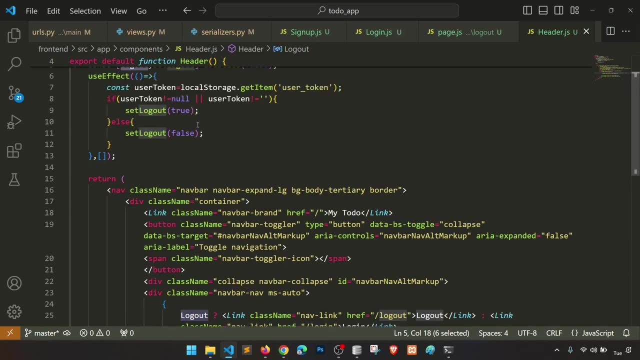 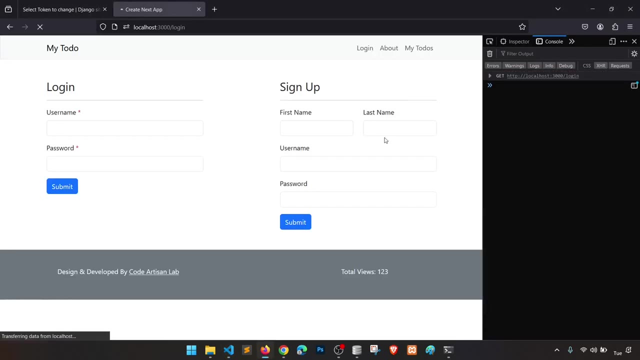 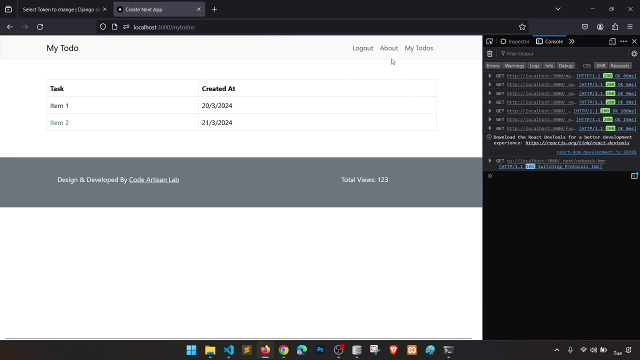 we have set logout and this logout we are saying if log out equal to true, then we are saying true, not equal to none. why this is showing: okay, this is correct. now, alright, so login. let's say admin, admin, submit. and here it is saying: and you can see, here this is showing log out. 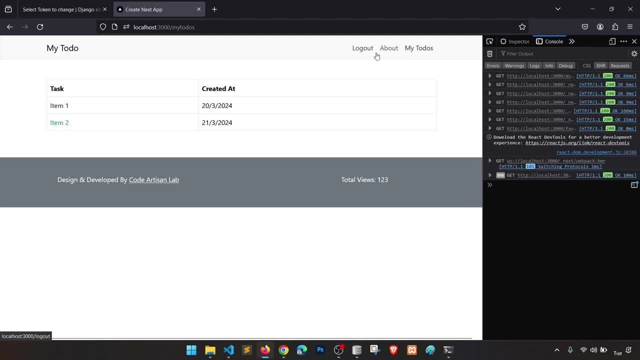 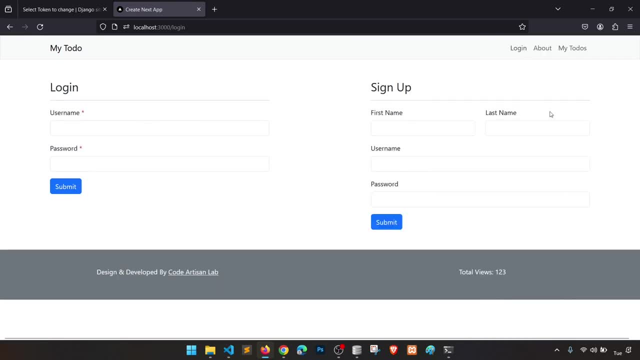 wherever we go, it will show the log out right, and if we click on the log out, then it will redirect to the login page and remove the log out link and convert it to login correct. alright, so now one more thing we need to do when we sign up. 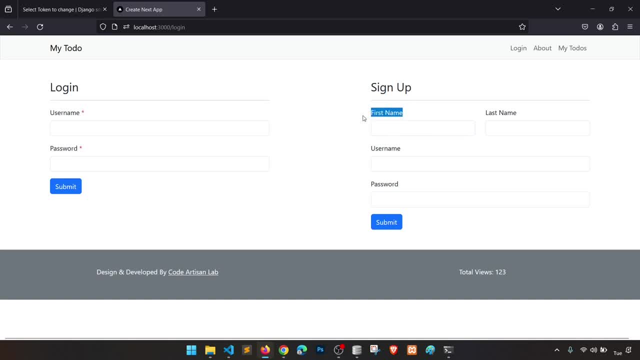 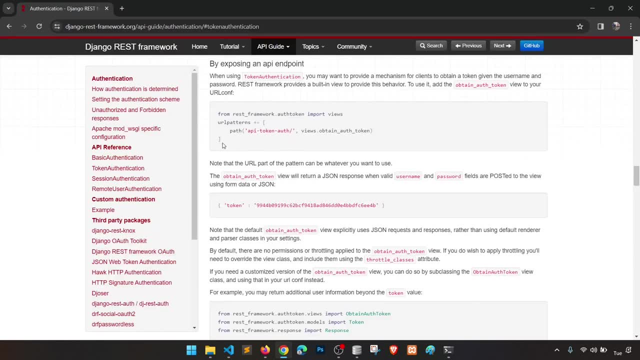 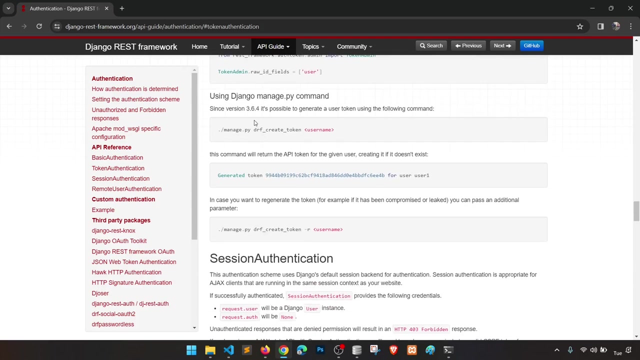 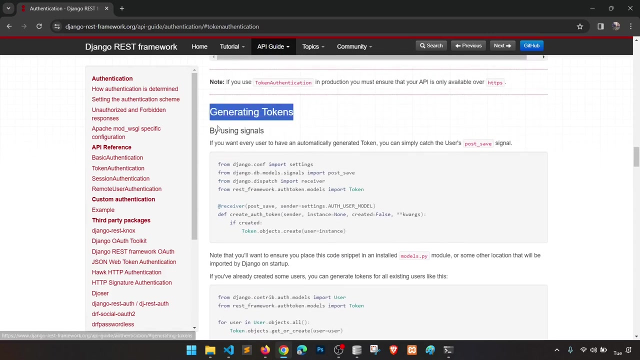 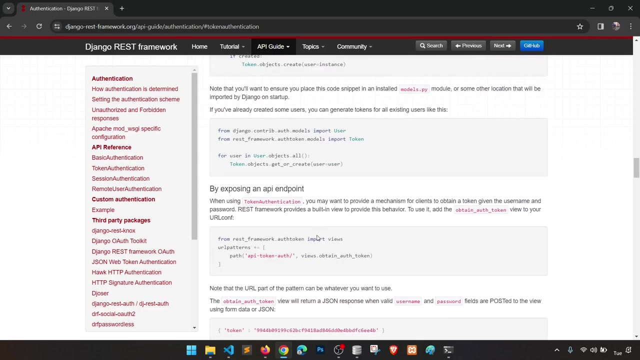 the user, it should create the token correct. so let's do this. you let's do this with the here using Django, okay, so where is that? let's say: let's generate: okay, so generating tokens by using signals- right, so we will. with the receiver, we can create the token right. so what we will do here? okay, so let's use the. 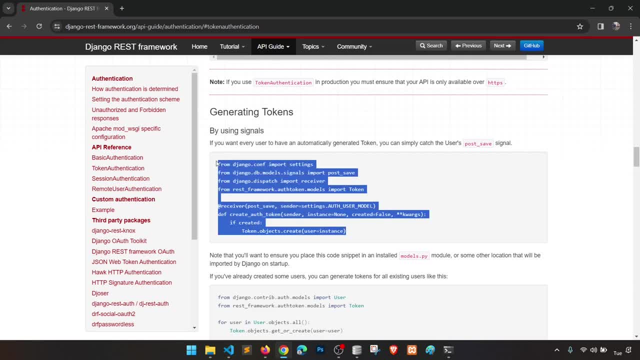 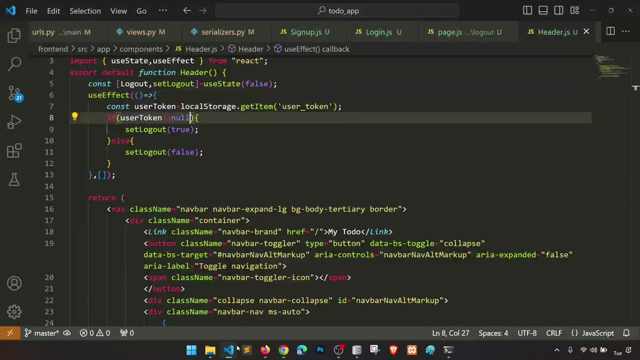 signals. so in the model or we can see: if you want to every user to have automatically generated token, then you can simply catch the user post save right, so let's copy this one. you can see that you're already doing it right, so now you can see inside there. 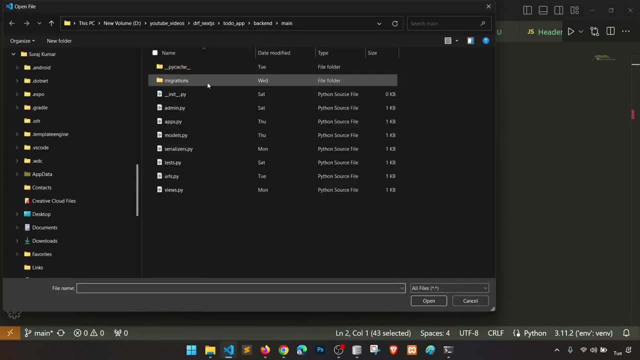 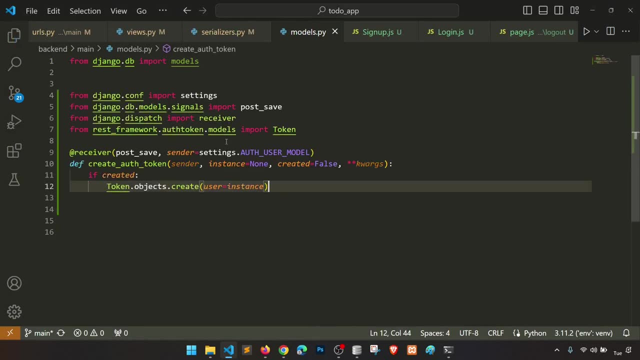 I'm gonna take. let's go one more time from here. you okay, and now you can see that you're in. the inside version of this model is generated here, so it has been knowledge sick is automatically generated, and nowadays we can also create direct Και. 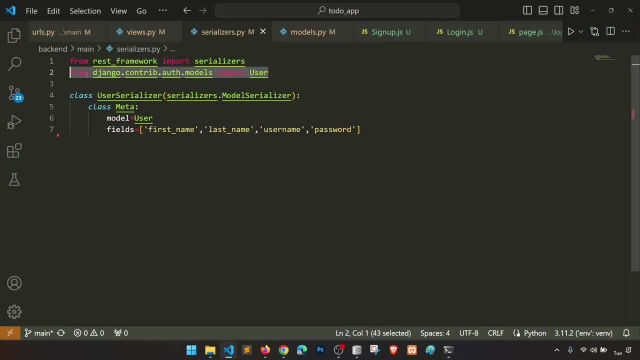 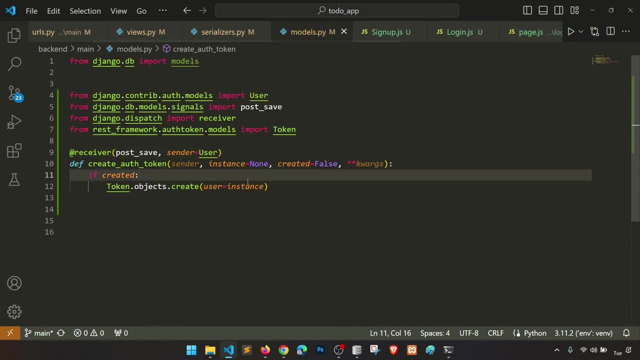 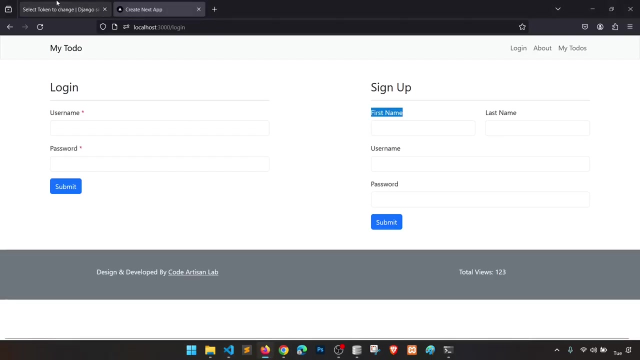 let's do serializer user here and paste this user here, correct. so whenever we create now new user will create the token, correct. so let's see how this is working. so here we have our tokens. this is for one user. let's create one more user. let's say john doi, john, password submit. 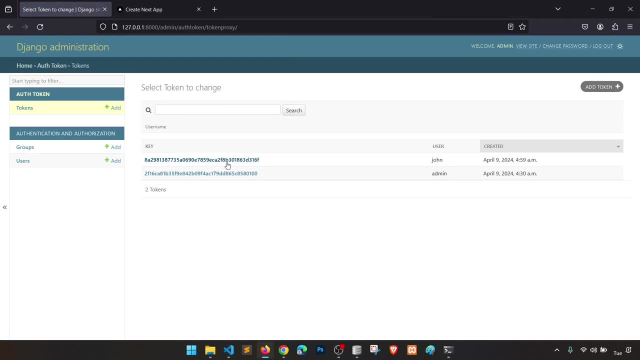 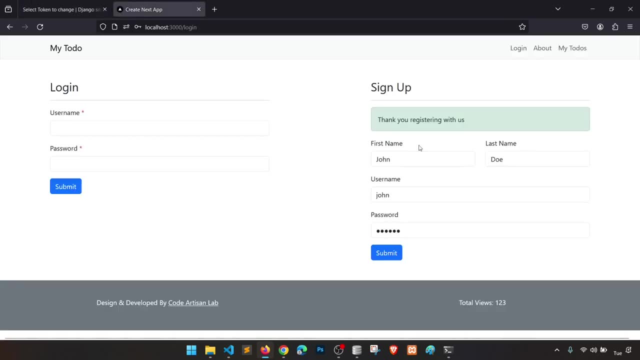 see, this is the token for john, correct? so we are creating the token and we are creating the user, and user can log in and user can. now user can browse the to-do list. okay, so now the next, next next step is let's go to uh, set up the to-do, fetch the data and do all the things. 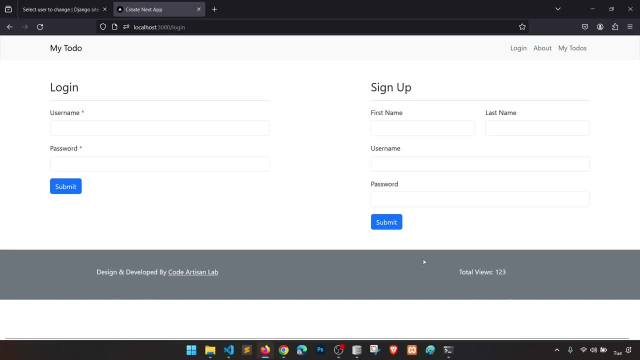 okay. so before the to-do, one more thing that we need to do: when we are signing up, then it is saving the plain password in the database, right, and when we are trying to log in, then it it it is trying to match with the hashed password. so when we are 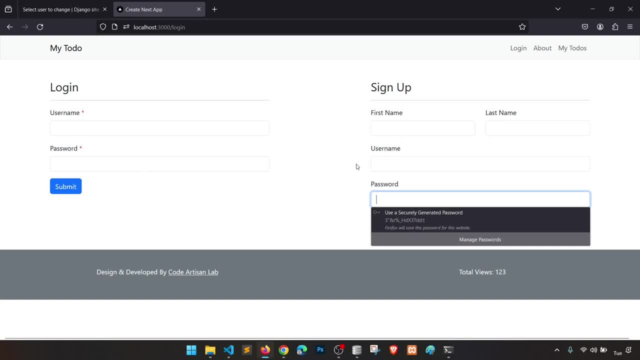 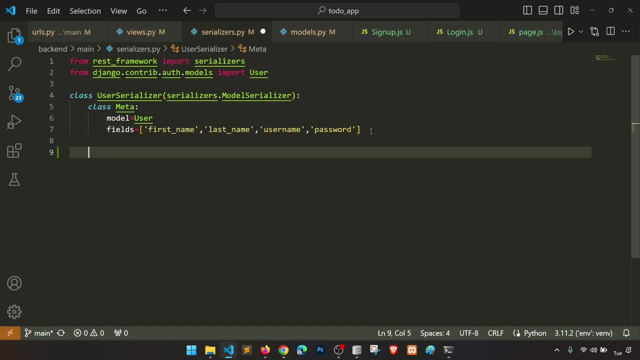 signing up, we need to convert our plain password, uh, to hash password, right. so for that, uh, we will open the serializer and here we will create a function over at the actually function self validated data, correct now, user equal to user, and we need to pass here data. so first name, last. 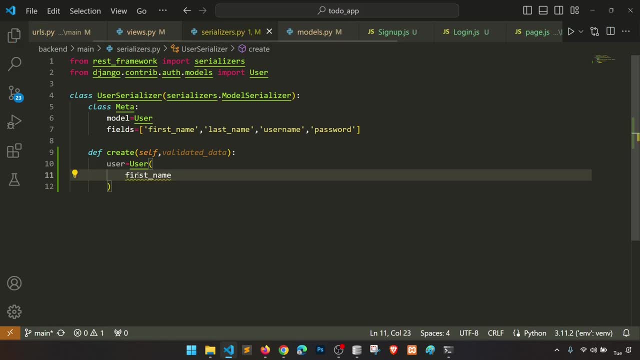 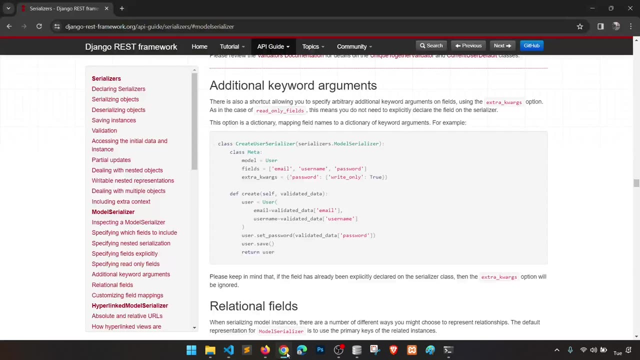 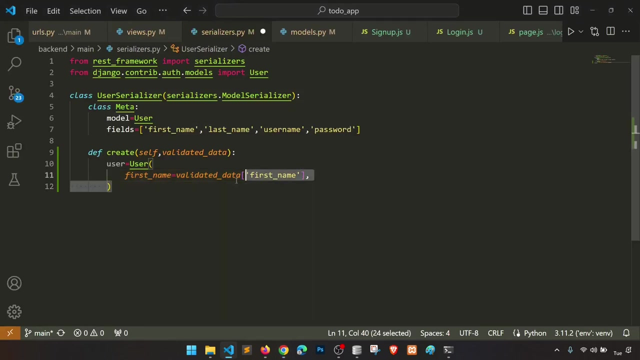 name. so we'll say: uh, first name equal to validated data. uh, first name equal to validated data. first name, right, as defined in the. uh, as defined in the you know official documentation, correct? then, uh, we have to say then last name and then username, so last name. 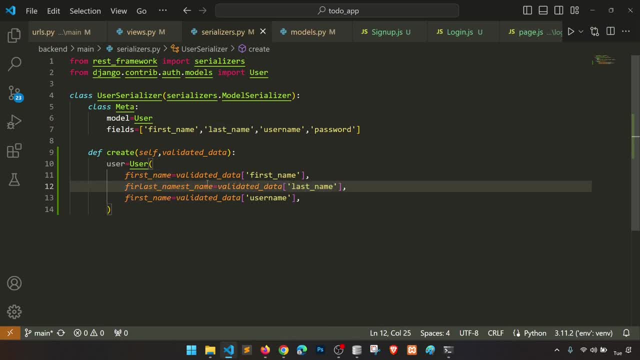 username, right? so last name here and let's say username and with this user dot set password and we will set the password from here. we will say password correct and then user dot save and then we will return user. so this, actually, we are overriding the create function, right? so? 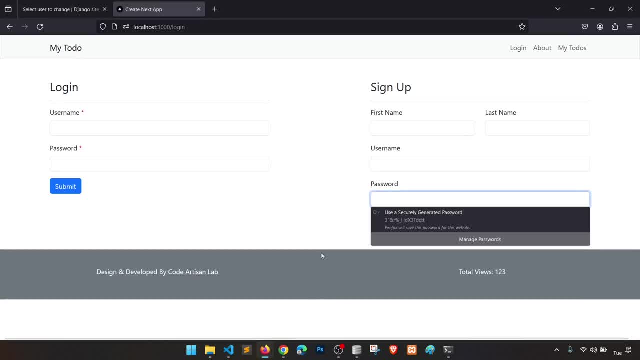 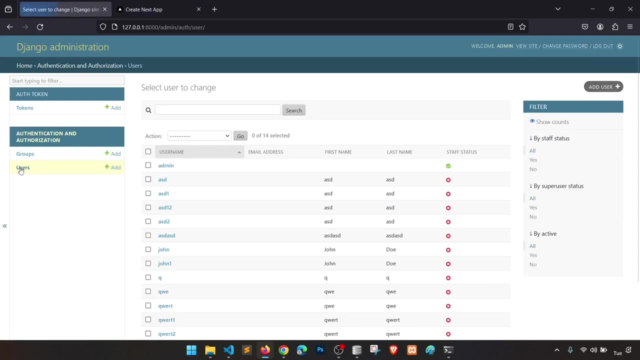 create method. so let's see now. so it should save the data in database, uh, uh, as a hashed password. so let's say john doi, john one and let's say john one, right, so save. thank you for registering with us. let's go here, user john one, and here you can see password is. 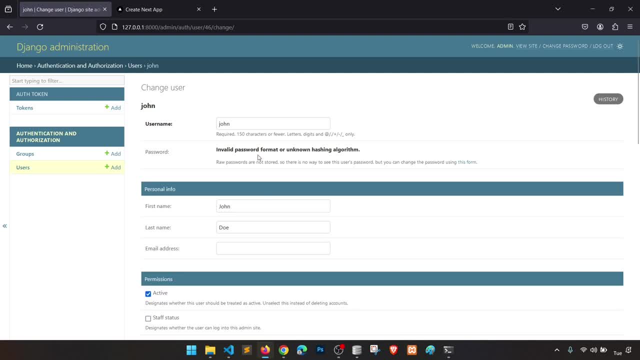 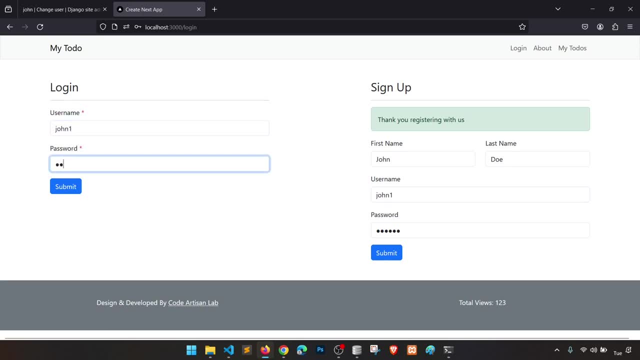 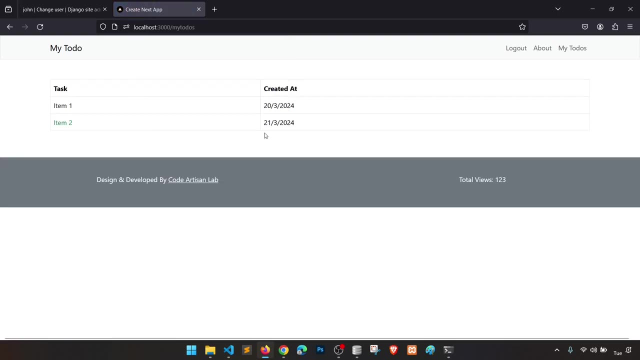 saving. now, if you go to the previous user, you can see here in value password. now let's try to login with this user and let's see login is working or not. so login is working and we are going to my to-do list, right. so now let's work on. now we can work on the my to-do list, all right. so this: 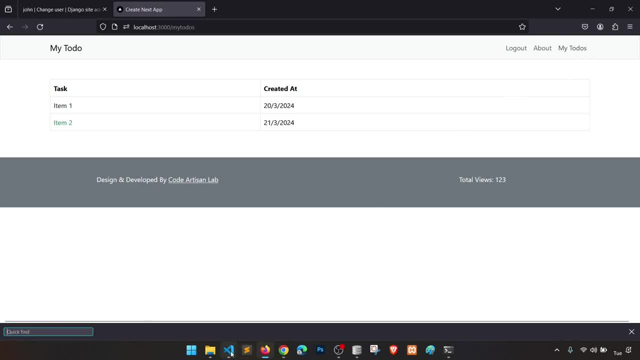 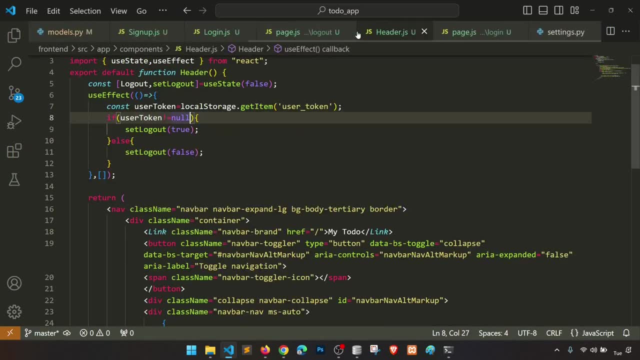 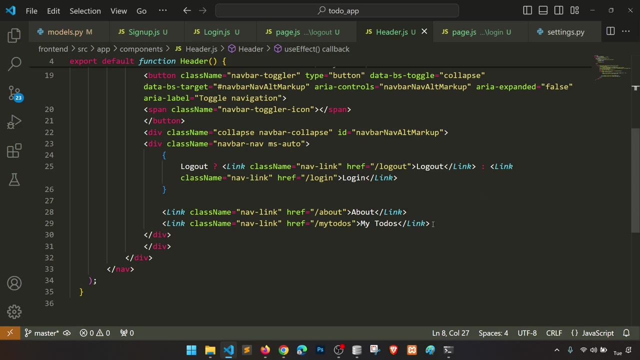 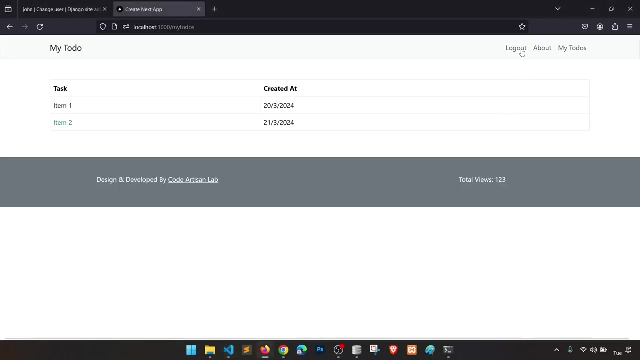 my to-do link will show only if logout is exist in the header. so let's go, sorry, let's go to header and we'll say this logout link and this my to-do link calls: right, so copy this one and paste it here. and we need to wrap this in some fragment, right, so this thing correct. so if I say logout, 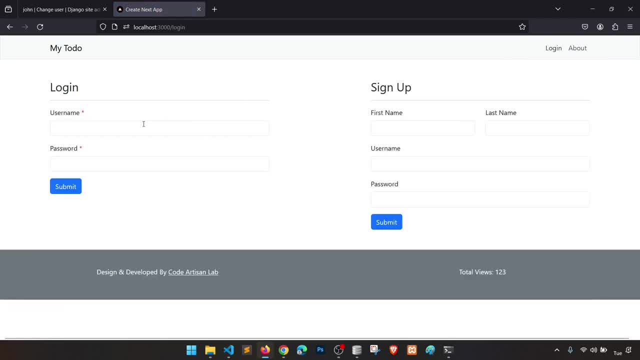 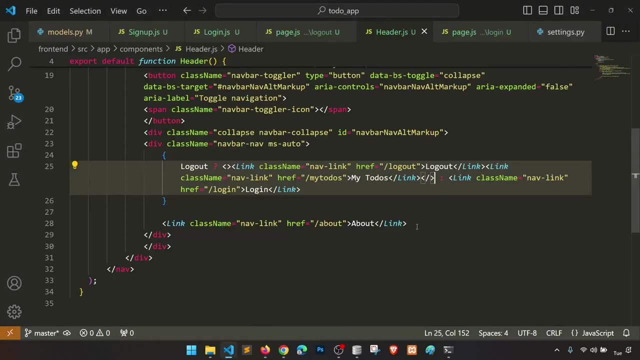 then will not show right. and if I say login, then it will show correct. so let's say John 1 and password submit. so my to-do and about link: okay. so yeah, this is fine, okay, okay. so when we click on this, my to-do this is: 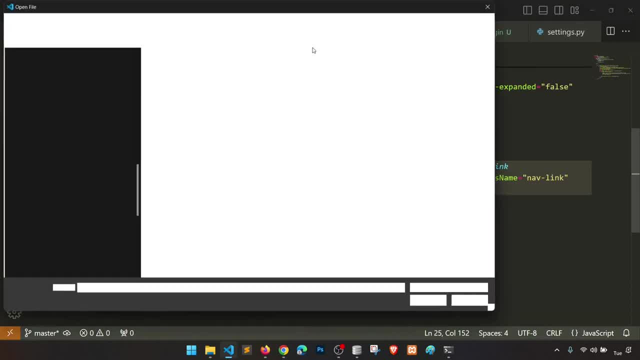 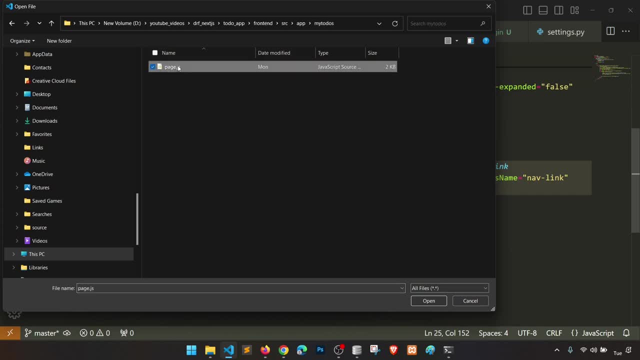 so let's open the my to do page. so let's open the my to do page actually. so where is that my to do page actually? so where is that my to do page actually? so where is that my to do page, right? so here we have a data. this is a. 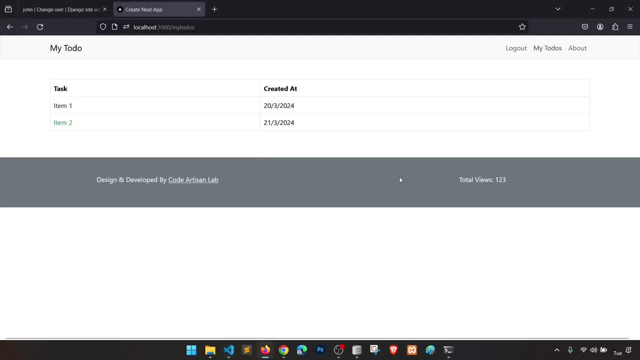 right. so here we have a data. this is a right. so here we have a data. this is a data which are, you know, static data. so data which are you know, static data. so data which are you know, static data. so let's create a button for adding the new. 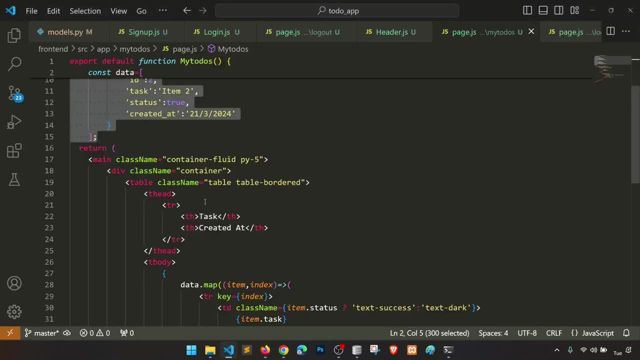 let's create a button for adding the new. let's create a button for adding the new list right, so task is created. let's list right, so task is created. let's list right, so task is created. let's create one more row right, and in this we: 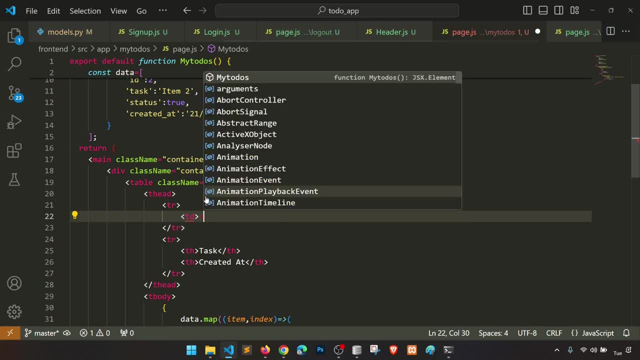 create one more row right, and in this we create one more row right, and in this we have have have, in this we should have called span 2 and called span 2 and called span 2, and we should have a, we should have a, we should have a link. 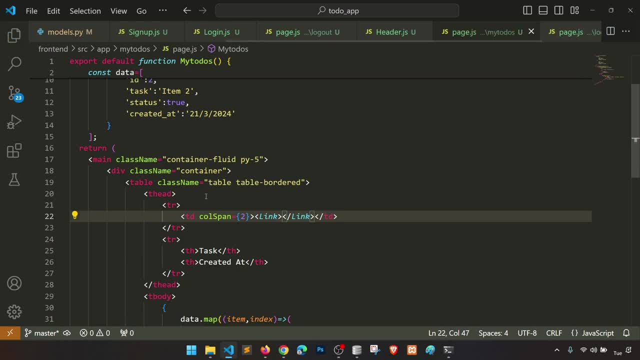 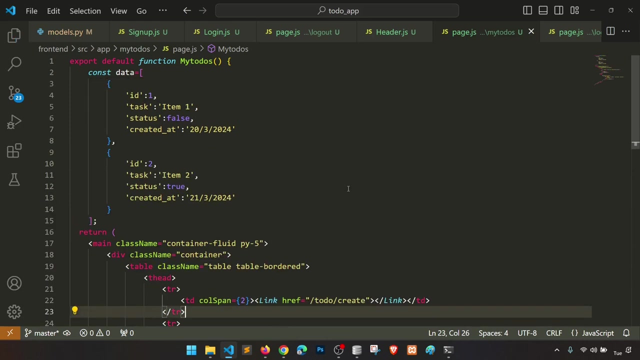 link link right, right, right link, link, link and link hra page. create, create, create. so we'll say to do so, we'll say to do so, we'll say to do: click, click, click, click, click. create correct and we need to import the link. create correct and we need to import the link. 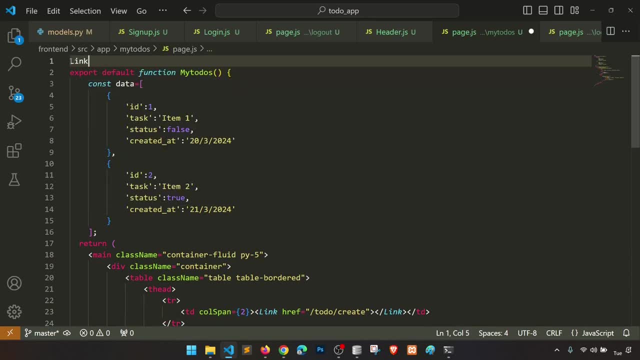 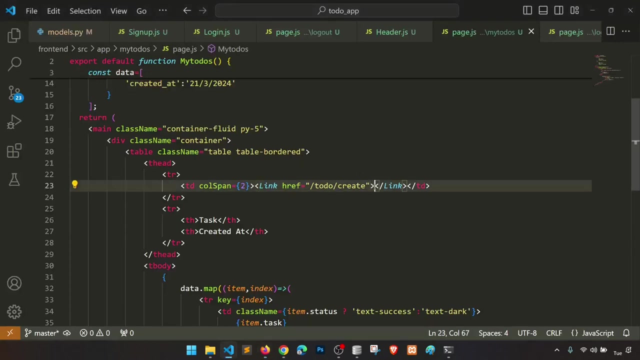 create correct and we need to import the link here. let's import this, let's import this, let's import this. next link, next link, next link, okay, okay, okay. so if i see here nothing is showing, so if i see here nothing is showing, so if i see here nothing is showing, let's say: 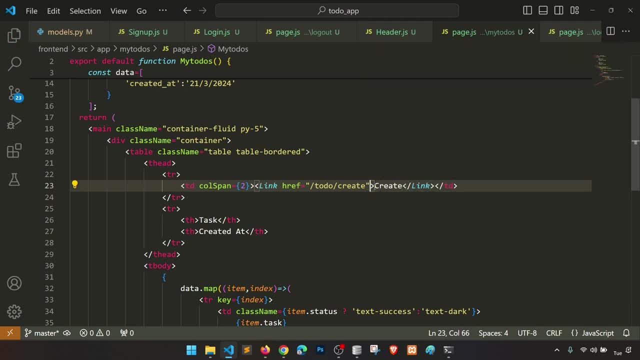 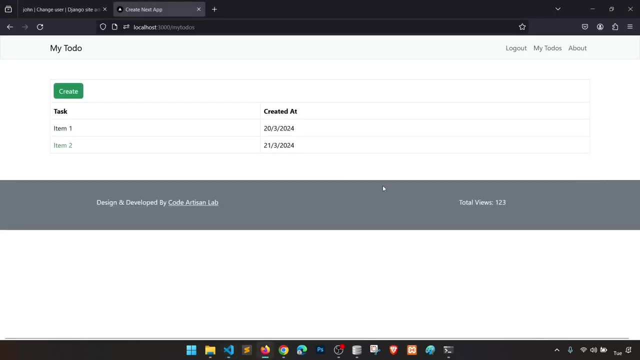 let's say, let's say uh, uh, uh, create, create, create and and and also let's create button button also. let's create button button. also. let's create button button, access, access, access right. and let's say: button s right, right, right. so let's remove all this. 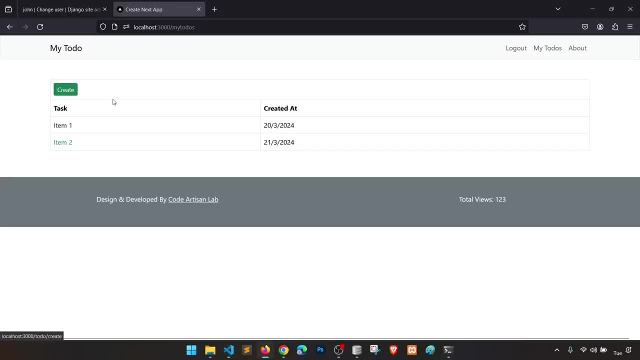 so let's remove all this. so let's remove all this. okay, so create when we click on this. okay, so create when we click on this. okay, so create. when we click on this, create it should open the form where we create. it should open the form where we. 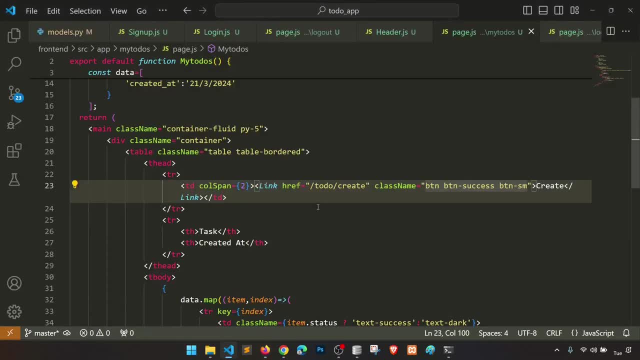 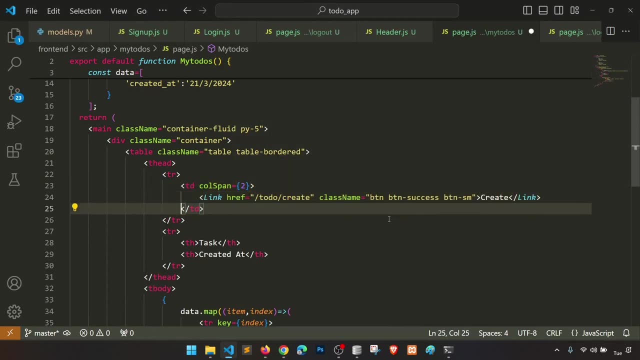 create. it should open the form where we can add the task, can add the task, can add the task, right, okay, so, okay, so, okay. so we need to create the component for that, we need to create the component for that. we need to create the component for that. and this is for showing the data. 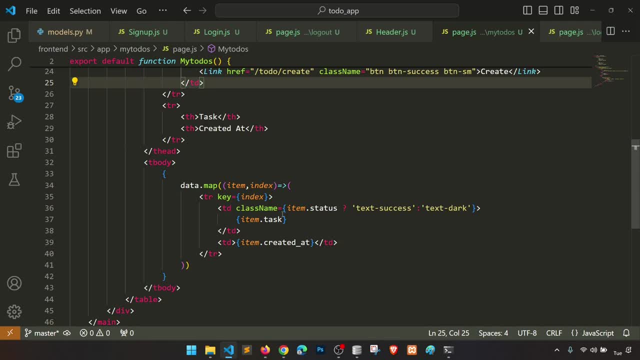 and this is for showing the data, and this is for showing the data right. we will also right. we will also right. we will also show uh, show uh, show uh. we will also create a small component for we will also create a small component, for we will also create a small component for this data right. 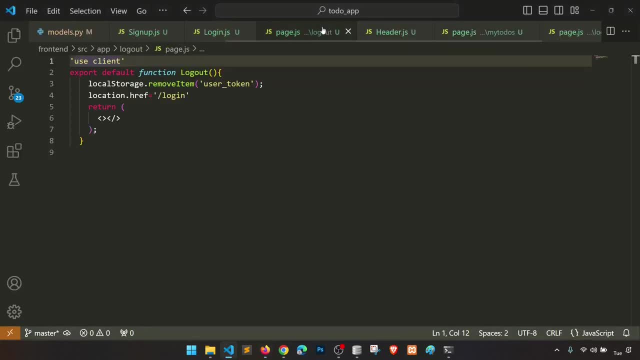 this data right, this data right. so what we will do? so, what we will do, so what we will do: here we have a, here we have a, here we have a component, component, component. uh, in this we have a lot of things. uh, in this we have a lot of things. 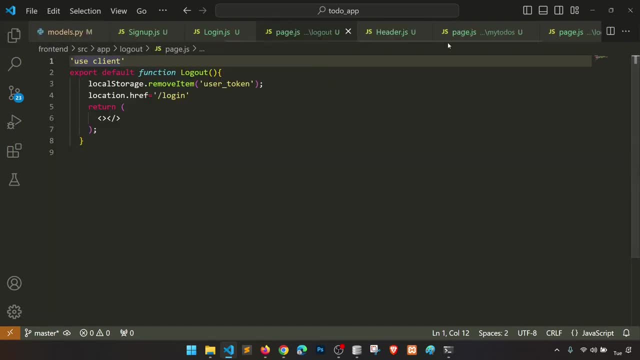 uh, in this we have a lot of things. uh, in this we have a component. okay, uh, in this we have a component. okay, uh, in this we have a component. okay, so we have a page and, uh, we all have. so we have a page and, uh, we all have. 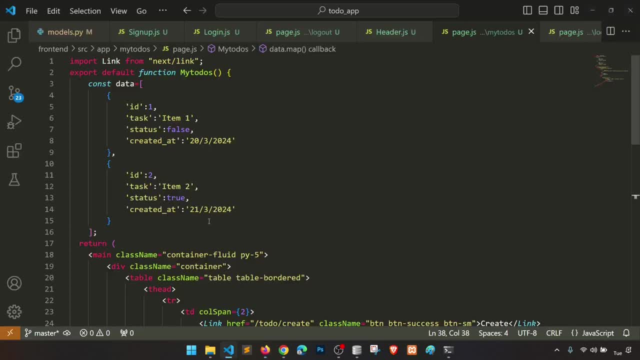 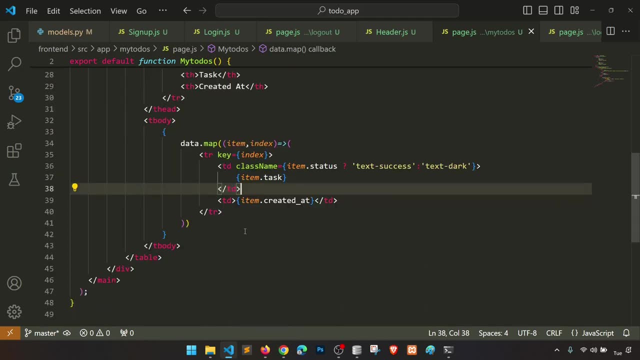 so we have a page and, uh, we all have this thing, this thing, this thing, so so, so let's fetch the data, let's fetch the data, let's fetch the data. okay, okay, okay, let's say, let's say, let's say, let's create a component. 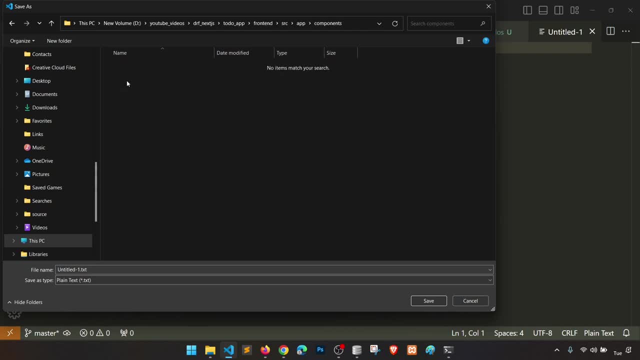 let's create a component. let's create a component. so here we have source app component. so here we have source app component. so here we have source app component. let's create, let's create. let's create to do, to do, to do list, list, list dot js. 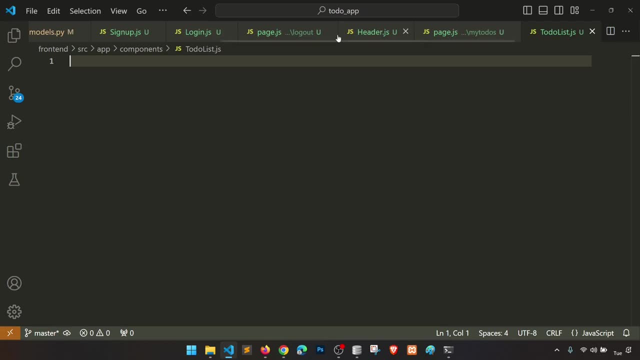 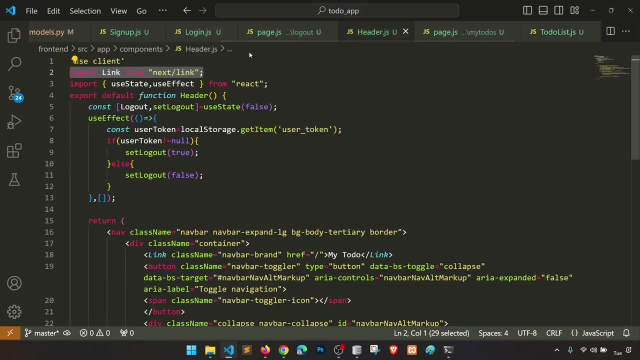 dot js, dot js, right, right, right. so to the listjs, and so to the listjs, and so to the listjs, and let's uh, let's, uh, let's uh copy any of the component, copy any of the component, copy any of the component. and let's say: 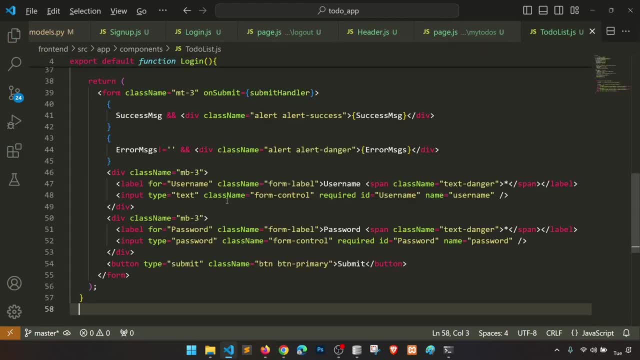 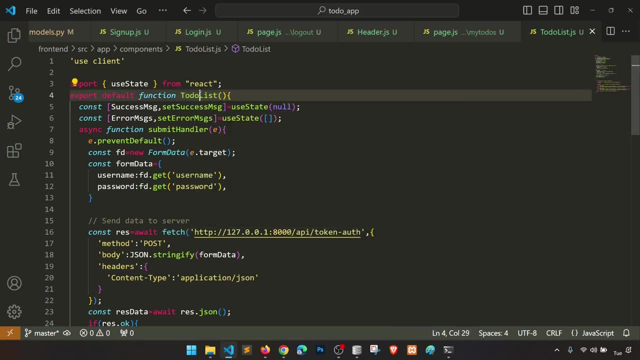 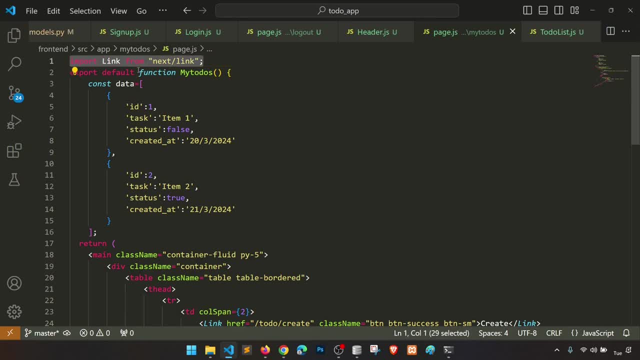 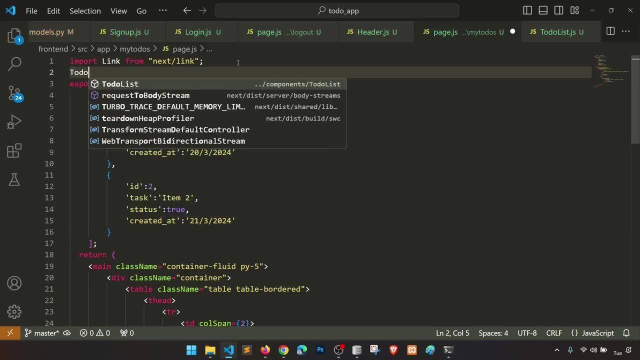 okay, and we will add this in our to do. okay, and we will add this in our to do: we'll import this, we'll import this, we'll import this, correct. so i will say, i will say, i will say: to do list, to do list, to do list. copy this. 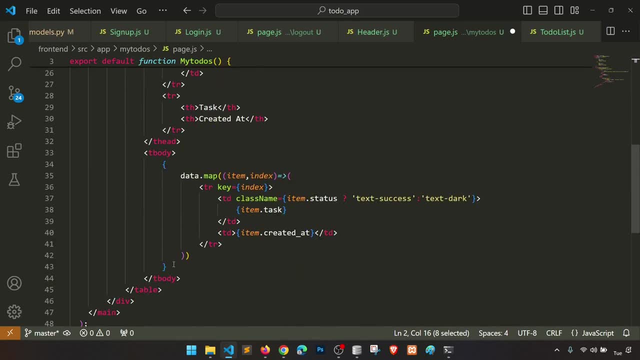 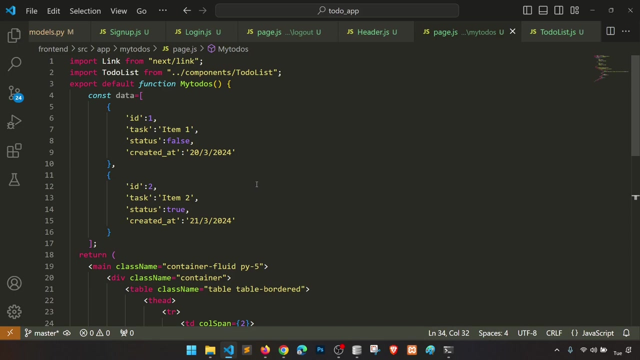 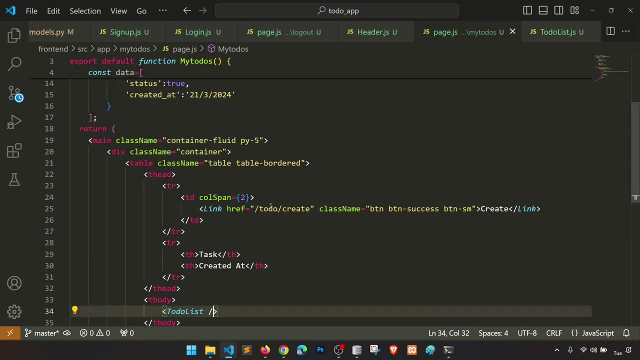 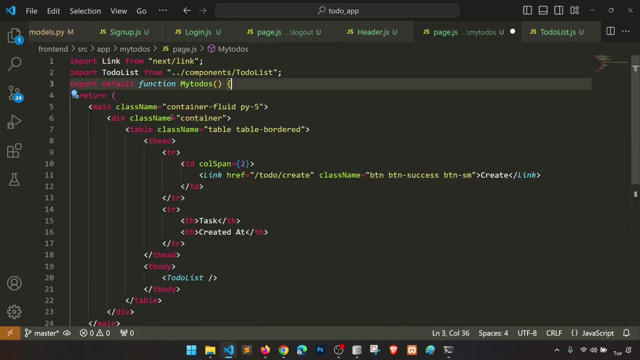 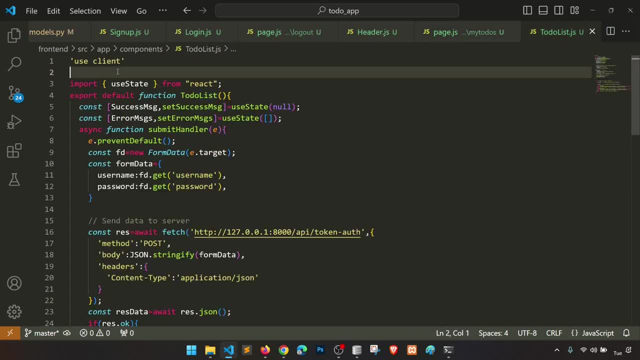 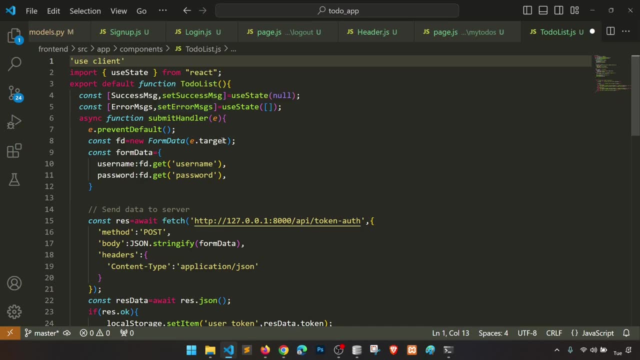 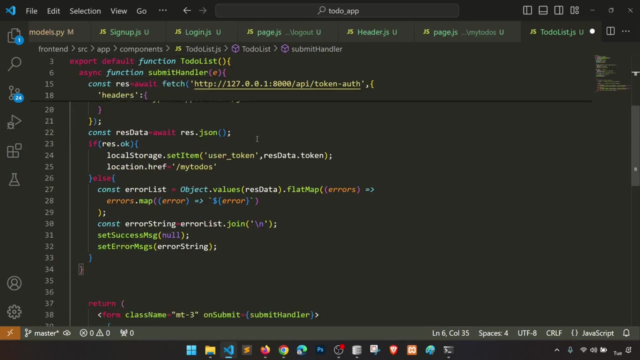 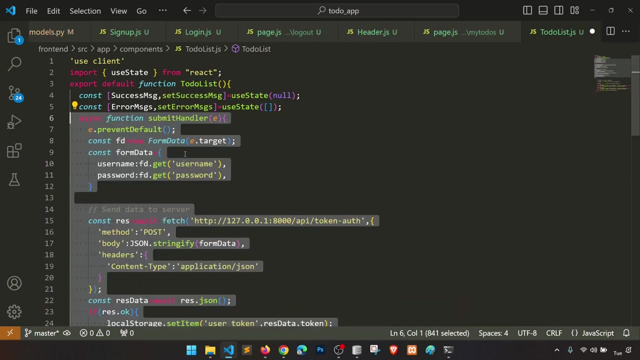 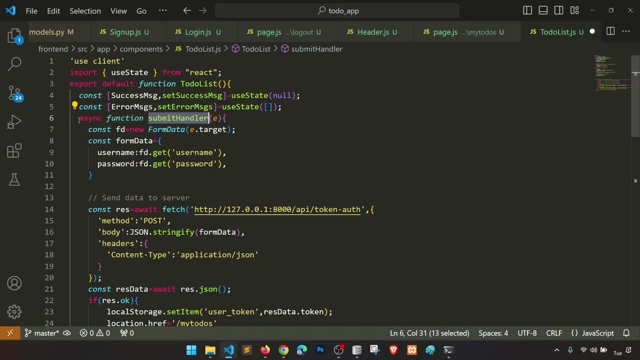 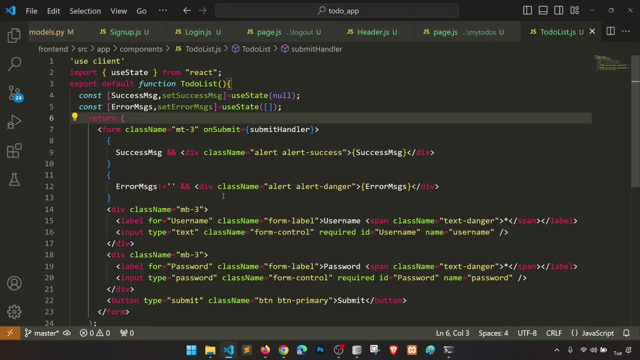 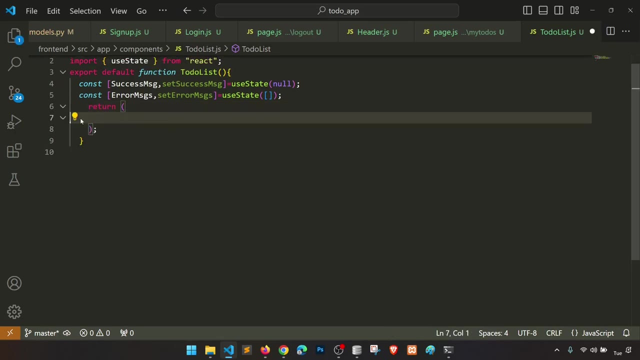 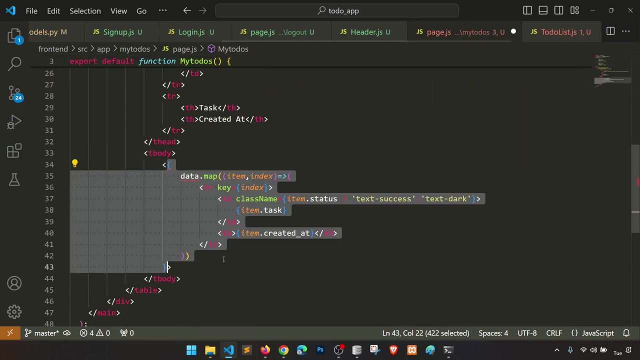 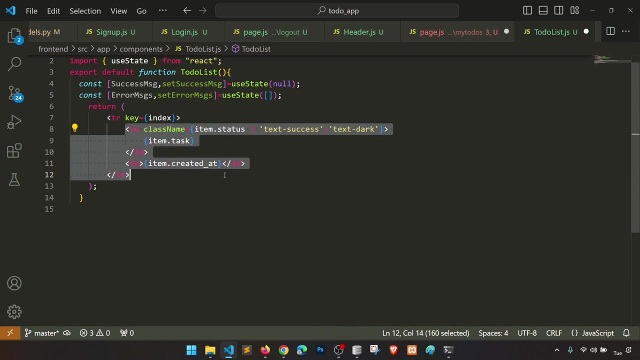 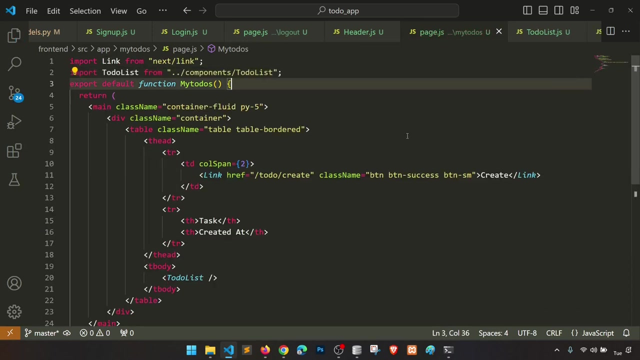 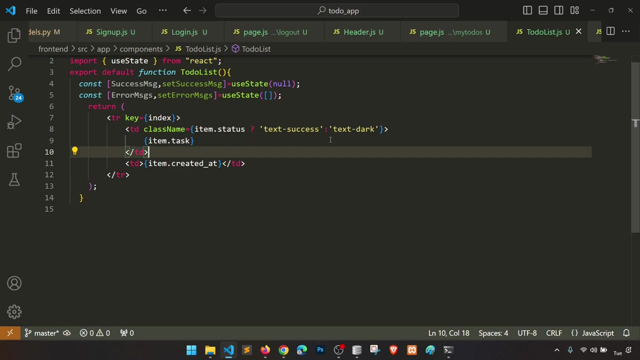 a sync function. let's remove this actually. let's remove this. all right, let's remove this one. also, no need for form, okay. okay, we need this TR actually, okay. all right, then to-do list and success error messages. and this one key status text. let's say one: no status equal. equal to true item: dot task: let's. 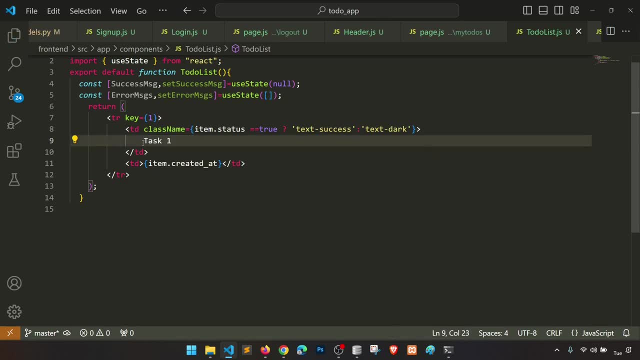 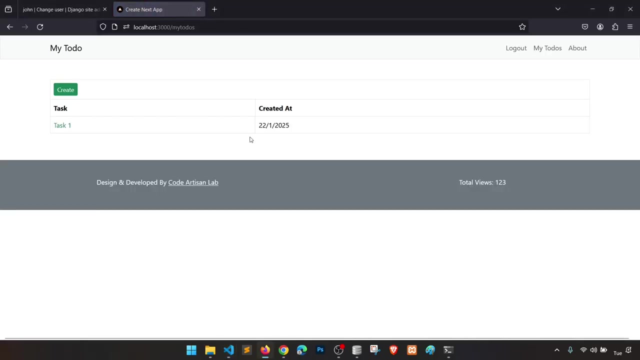 say: task one created it. let's say: this is: this item is not defined. against that, let's say this one: right, so task created and all the things. so this is working. now we need to pass that task to the next one. okay, so now we need to pass that. 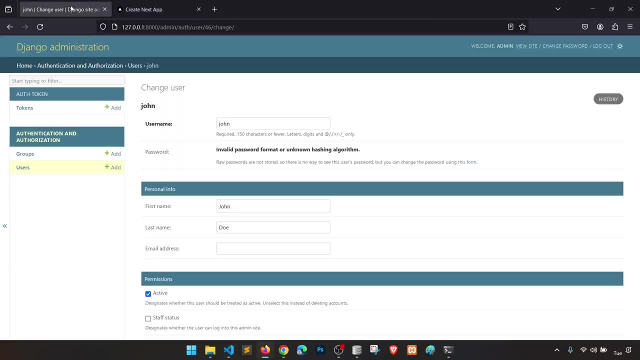 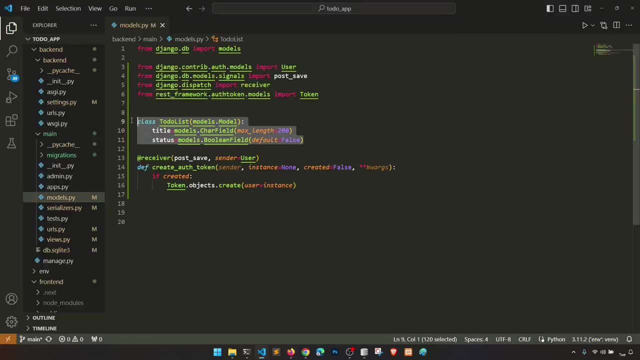 this one isohn, so förs traffic is done. let's see, we need to pass this starter, so user is lifetime node. and now we need to call dataset container web file. so I need to create some model file. so here let's create a new one, so this: 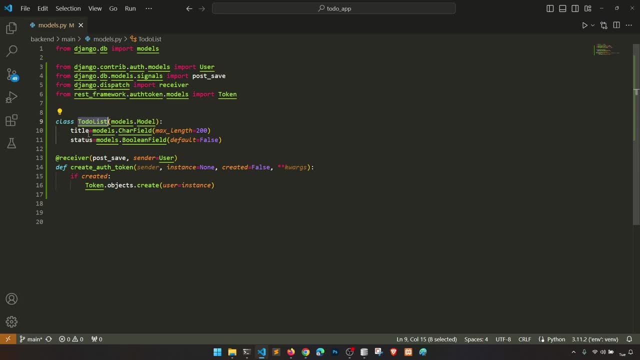 is a program calledument, which will provide us data in which we have we're an idea here, so I have written the data that we will execute in thisации a. well, so first step when we are creating the data here, right? so for fetching the data, first of all we need to create a model in our database and we need to create a API. 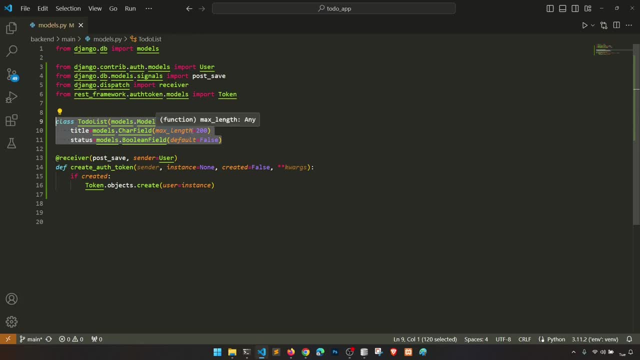 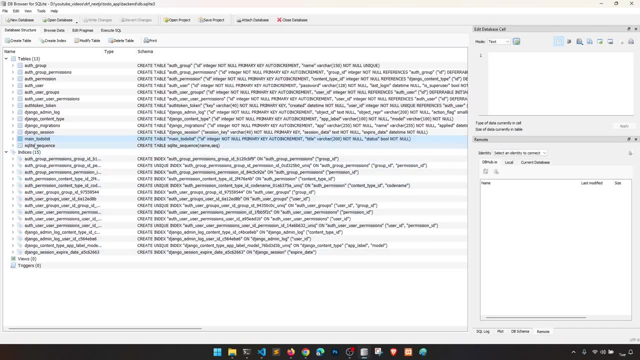 so let's do that. okay, so, for to do API here, we have a created a model right in the model file in us right and, uh, we have created the app for the simple steps you know make migrations and migrate right. so this created the table here. okay then, uh, what we need to do, we need to create. 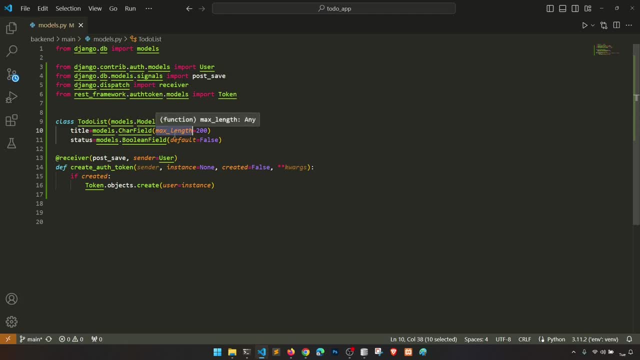 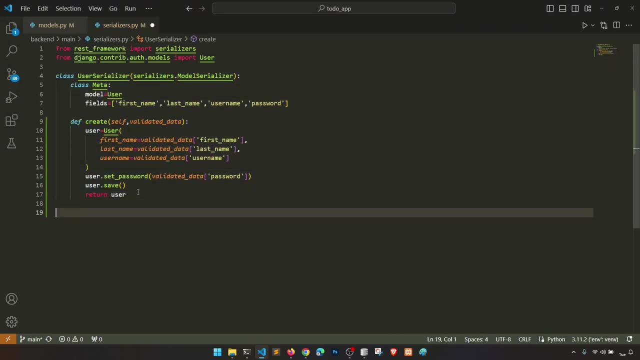 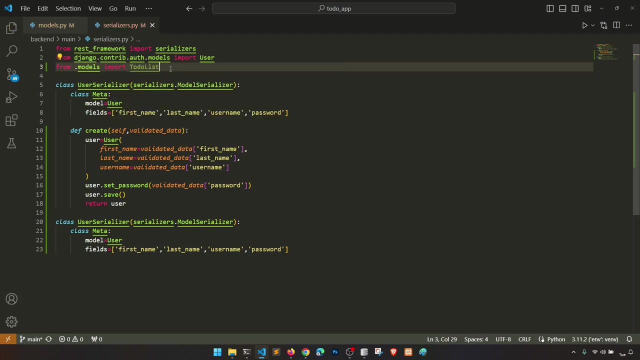 an api from this model, right? so let's open the serializer, okay, and let's copy the serializer. no need to customize this. we just need to remove this thing and we will import the frommodels import. we will import the to-do list: correct, and from the to-do list we will just need a title. 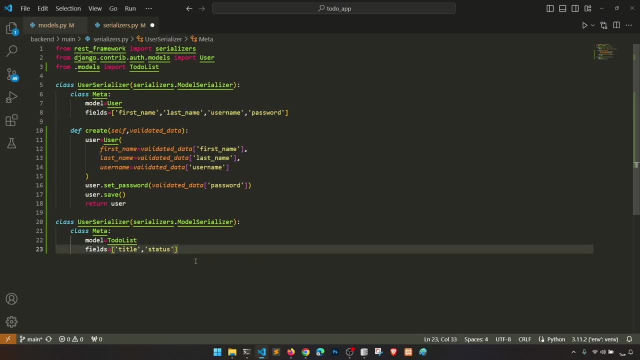 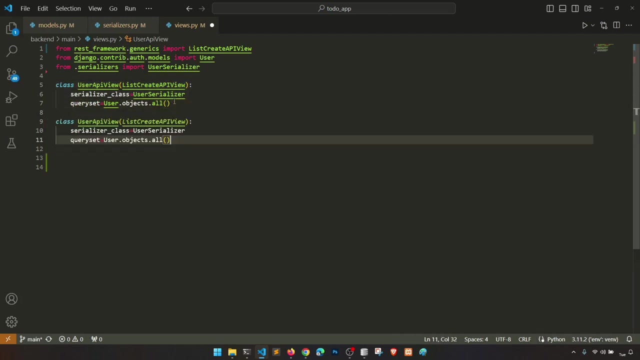 status correct and this is done. okay, one more thing we need to do to do test serializer. okay, now let's open the views. in the views we will copy, this, paste here and we'll import the to do serializer and here we will add the serializer and from the model, from dot models, import to do list and we'll add. 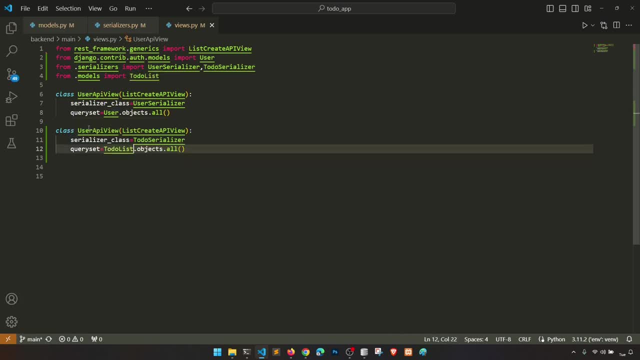 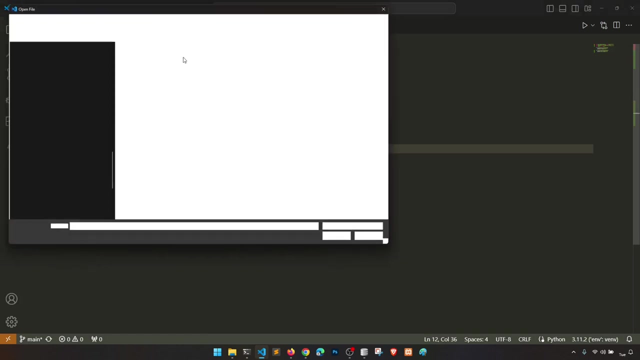 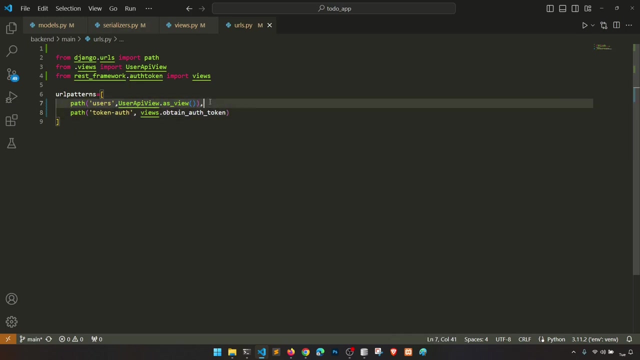 the to-do list here. yeah, okay, so we'll say to do, to do list view. okay so, list create API view. and the last thing we need to define the URL. so we'll copy this one right and we'll say to do's and okay, so from to do list view to do, let's say, API list view. I know that we. 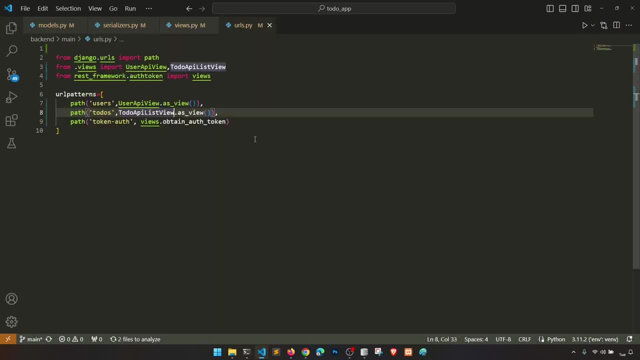 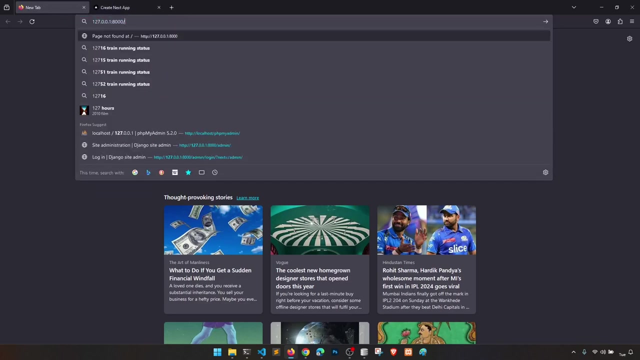 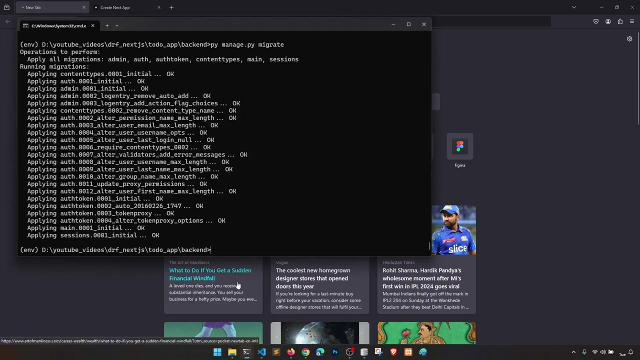 need to change the name, so let's change the name here. okay, so we have this thing. so users and all and all, so let's first test the will test the API. so this one api slash to lose. okay, service running or not? no, so we're not running, so we'll say pi py. 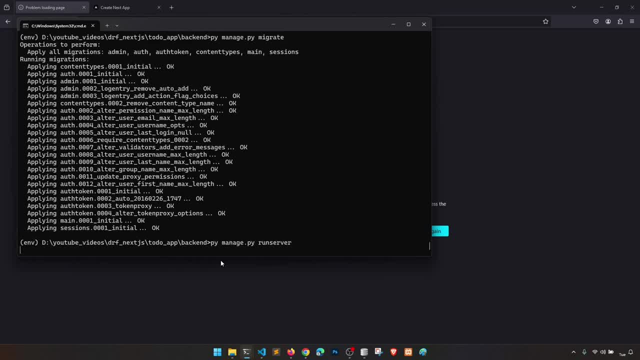 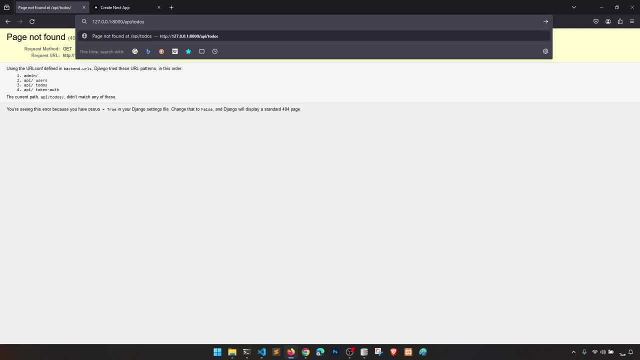 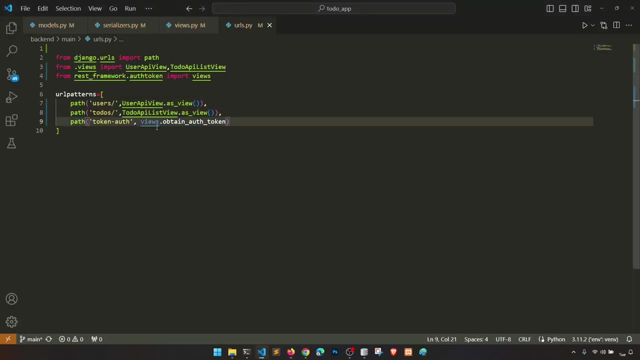 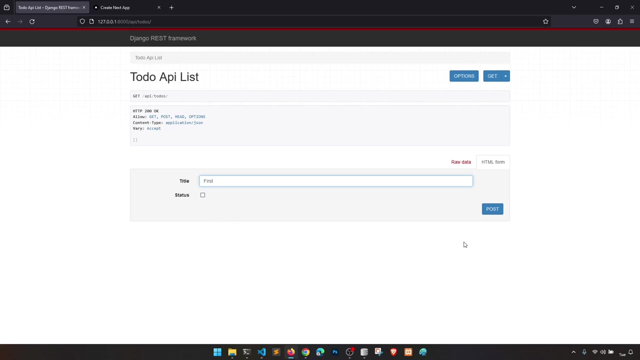 manage dot py run server. all right, so let's remove the slash from here. okay, so let's add the slash. if it's going to slash, then let's add it. okay, so this is to do, and let's say here first: by default it's disabled, so post. so by 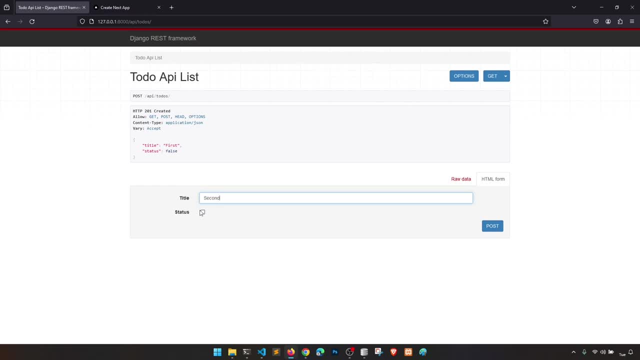 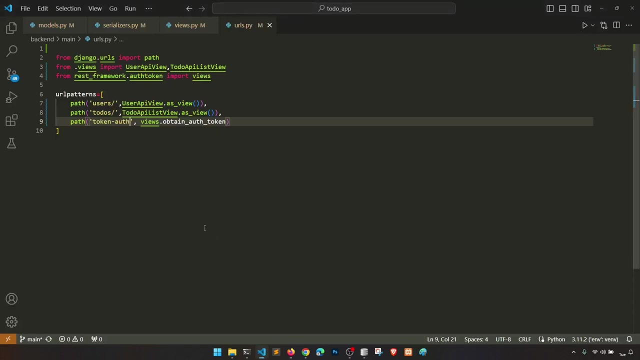 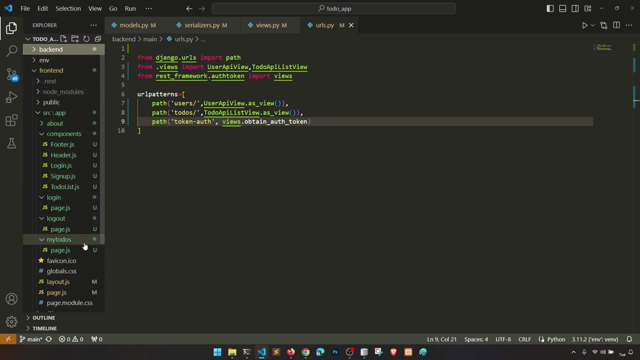 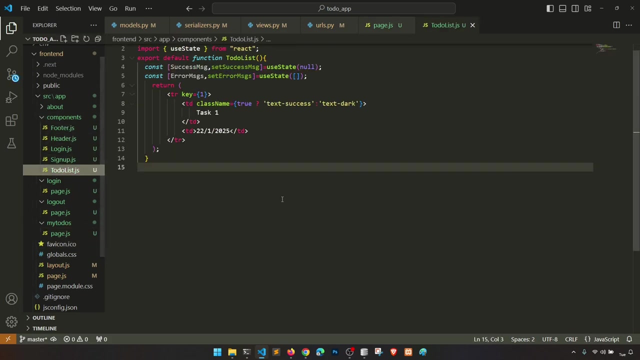 default this one, then second, second, right. so if I click here then you can see first and second. this is true. this is false. right now we need to fetch here, right. so let's open the front-end, like that front-end and page right, and here we have a to-do list. so we'll go to component to-do list, right, and we are. 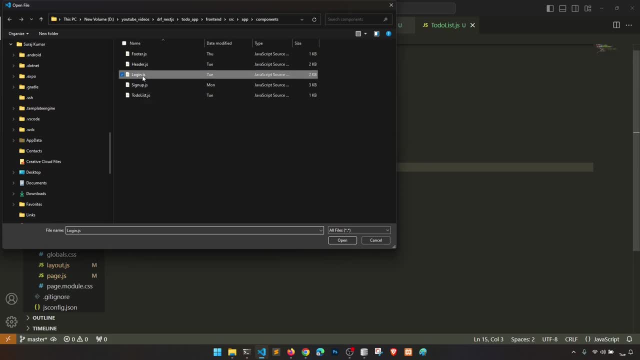 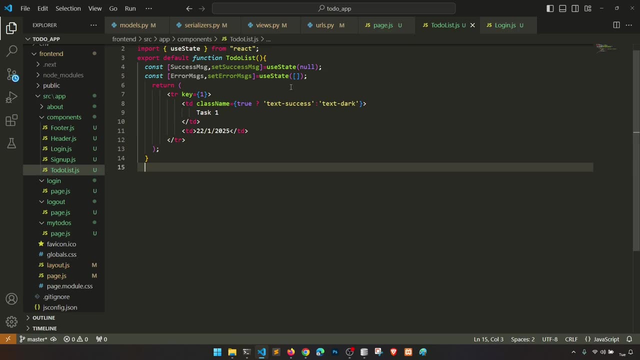 fetching the will fetch the data. so I will simply press, I will simply run this thing. so what we will do here, I will create a function, right. so this is our. let's create a function here, let's remove this, okay, let's create a function of sync function and get to do. 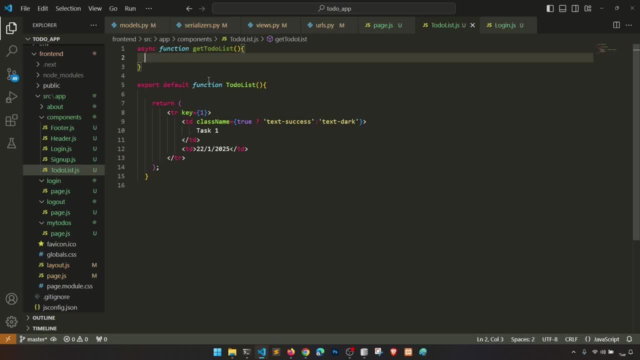 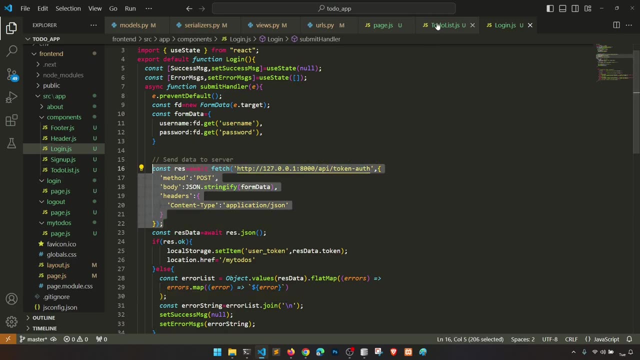 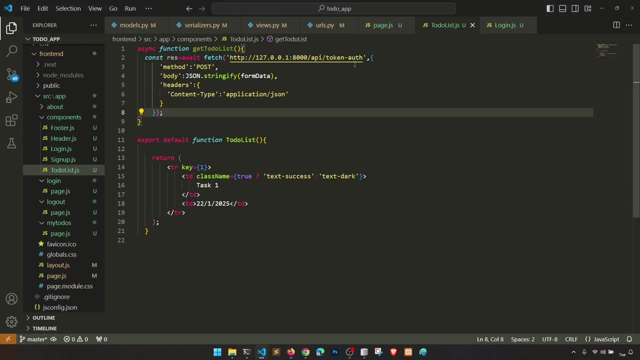 list right, and then we can run this one. let's copy this one, see here. and we need to run this URL right and just remove all the things, because no need to send any data. oh sorry, this URL is this, so let's remove this one, right, and then we can say console, dot, log and we'll say response. and here we. 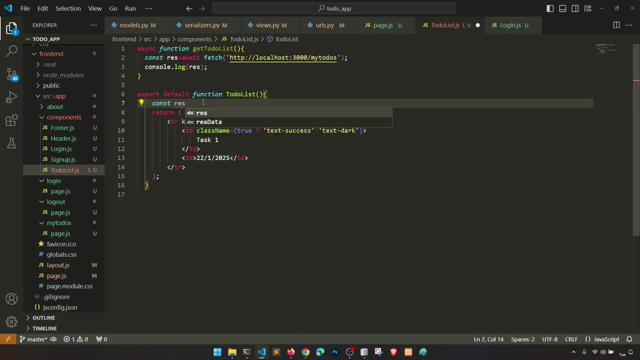 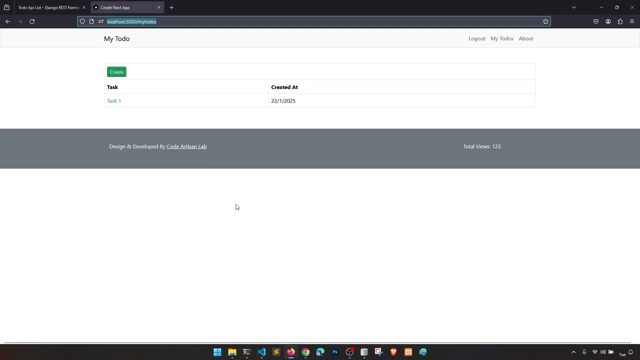 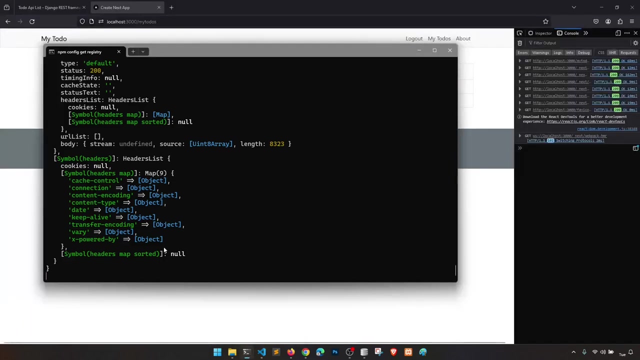 will see constant response data equal to a bit. get to the list. okay, so right. so no, we can console this. okay, we have. actually, we are running this function, so just do this thing. okay, let's see now here. so if I console this, then we have to. we are showing the data here. 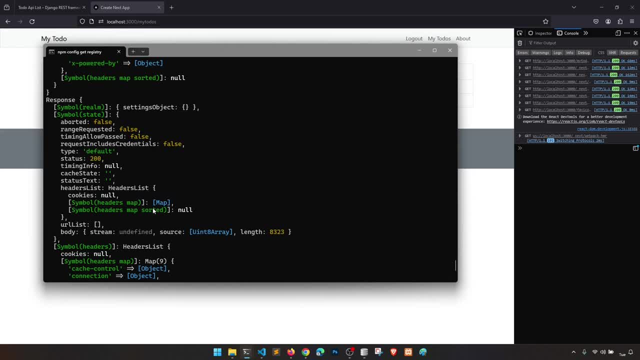 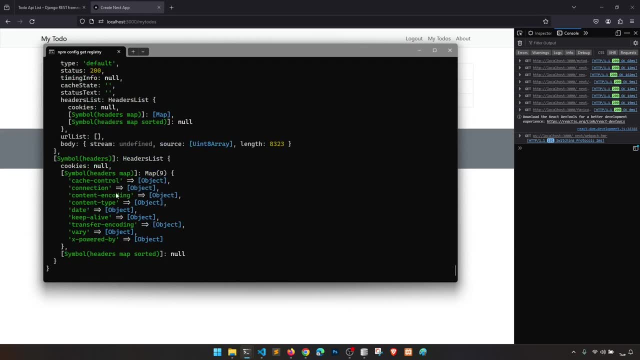 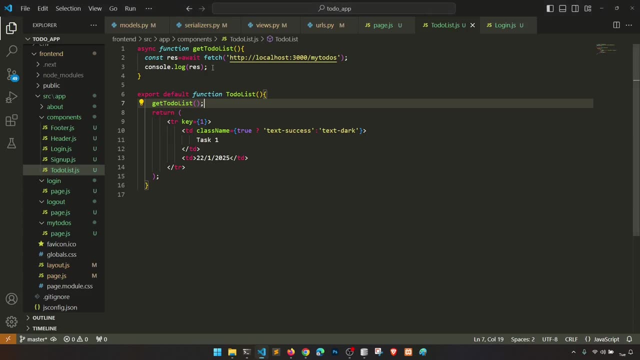 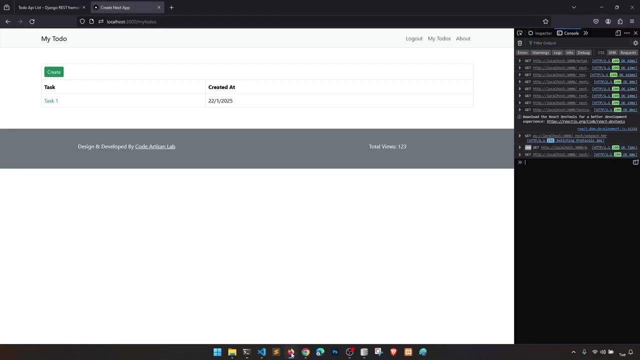 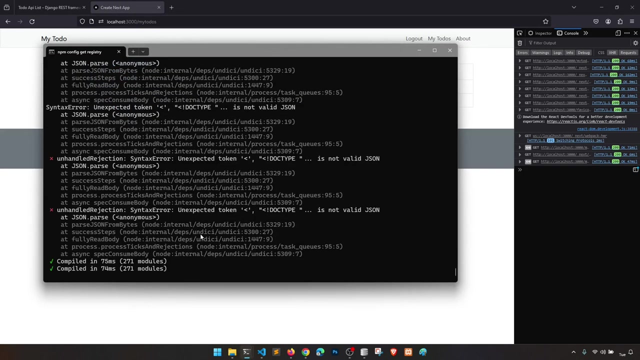 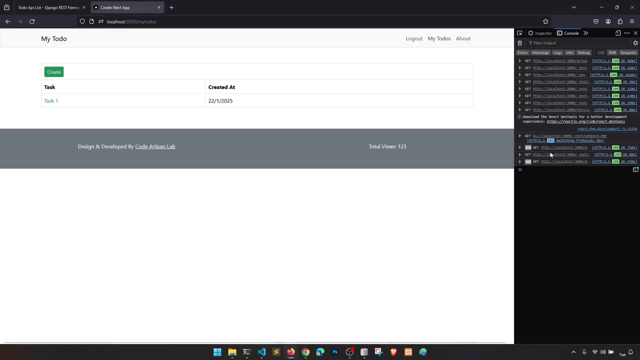 so status is 200 and data is not coming. where is the data cookies? let's see. it should return the data, okay, all right, then, if I click on the to lose, what is this? this is not valid, Jason. okay, let's go to network directly and let's see here. 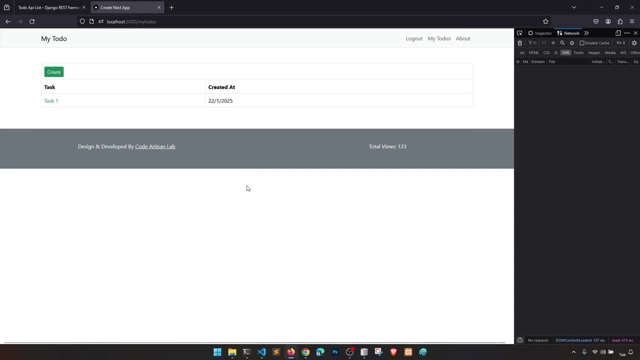 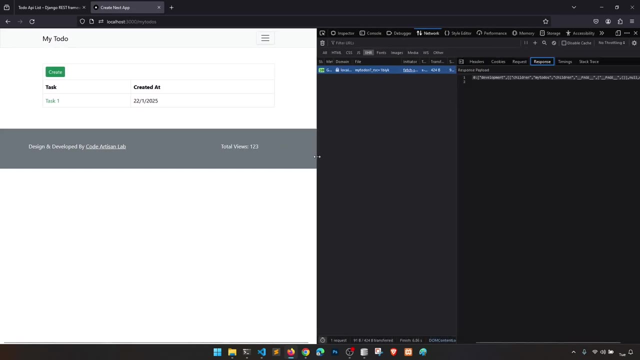 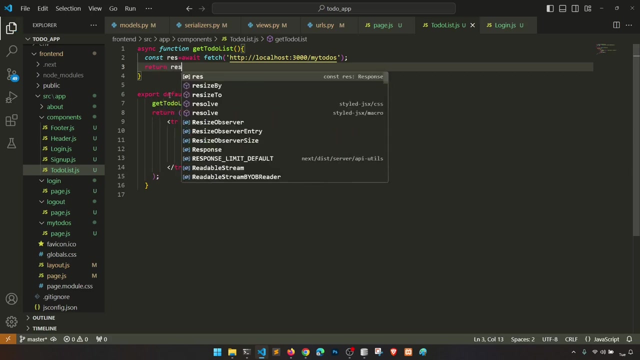 why this is not showing. let's see my to lose. click here our response. okay, request response. it is not showing the data. why this is not showing the data page null. okay, let's see here. let's return this. return this response. actually, um, let's run this function here in this, in this component, correct, and then we can. 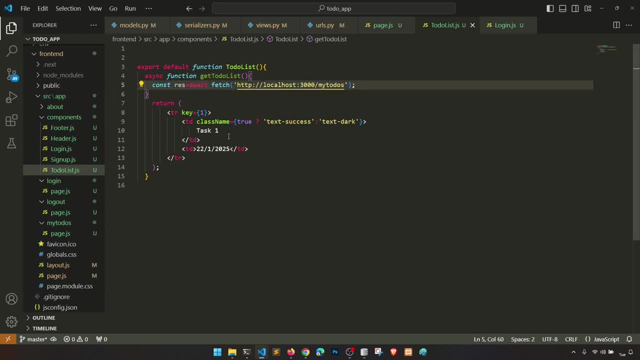 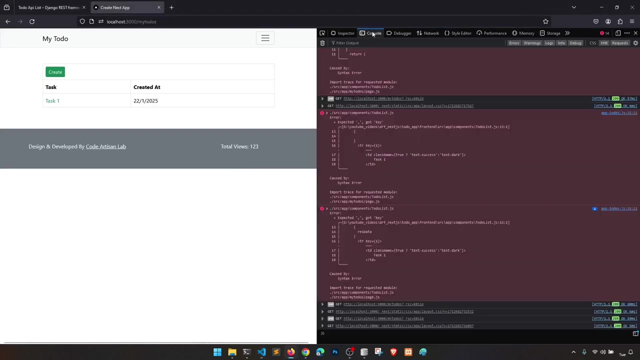 do one thing. this is response. let's say if, if response dot, okay, then what we will do: constant response data equal to response star right, jason json. wait, this is else. response dot data is empty. let's say equal to json json. actually, let's console this data: response to us data, okay, so what it will do, what is going? 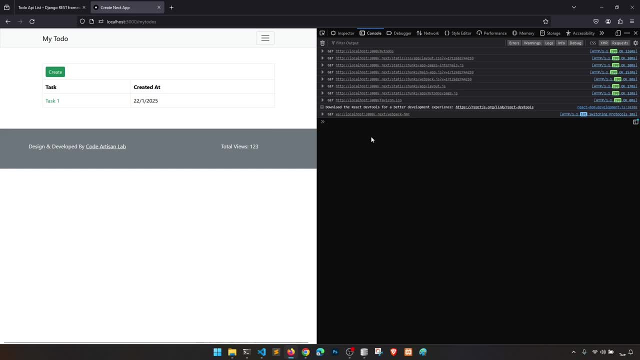 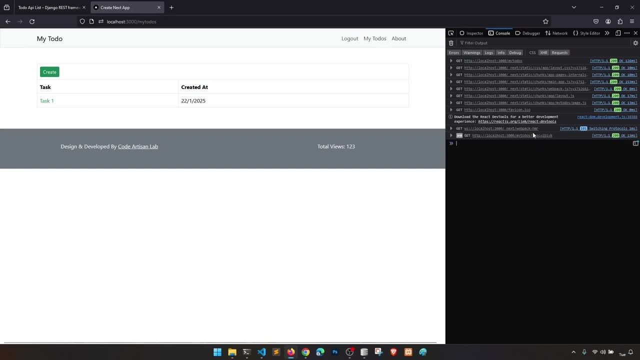 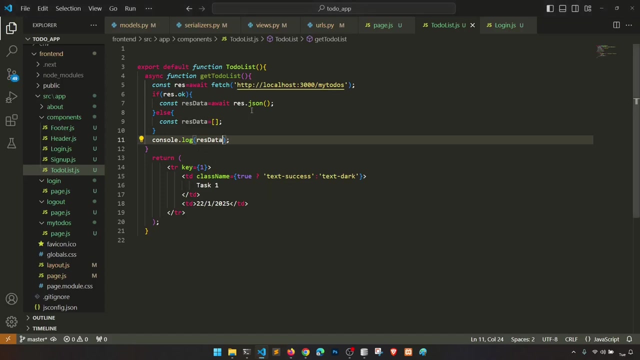 sorry. so my to do's here, my to do's and response. not sure why this is showing like this. well, this is not showing the response, but let's try to do that. mmm, we can do one thing and let's map this response. dot map. the first one is item, second one is index correct and? 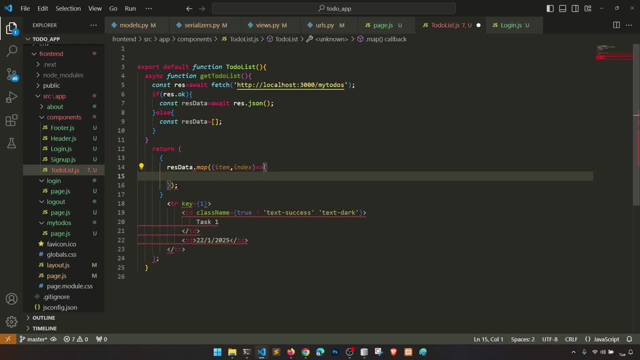 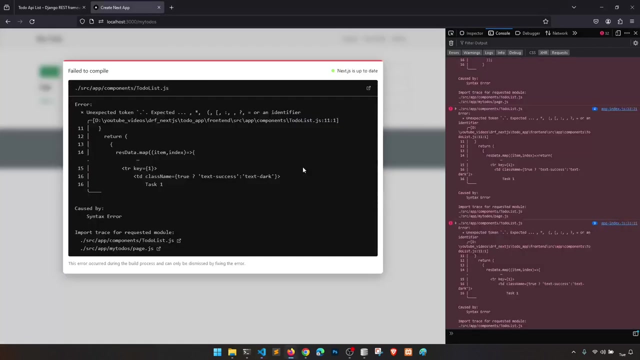 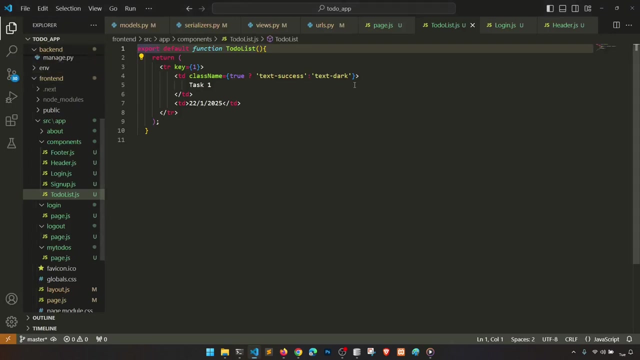 we need to return here, return this one. so we need to return this thing. okay, let's remove this here, all right? response: dot data, dot map. okay, so I think we should. let's do this with the simple way, right? let's not do this in a complicated way. 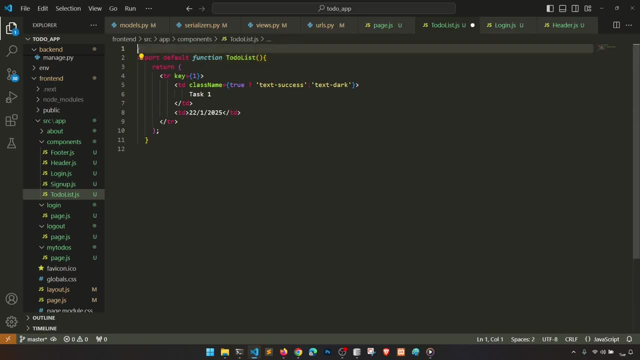 so what I'm going to do here: first of all, let's define this use line right, and then here- uh, not here- let's say use state and use effect right. use state and use effect we can use only in the client. uh, pages or component, all right, then use effect. 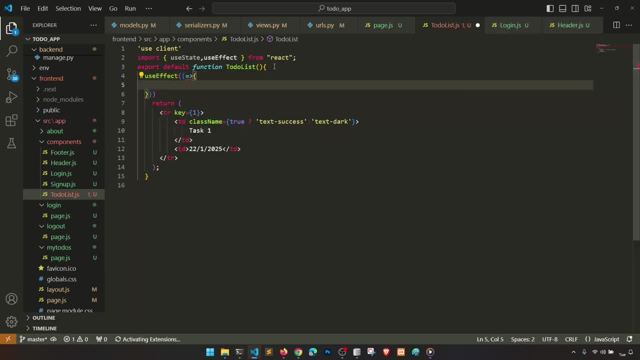 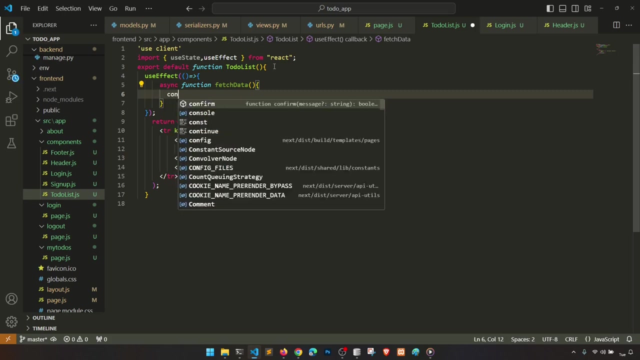 what is this? okay here. and then let's create a function: fetch data and constant response- okay. so we need to create a function first to move this pattern. if we have a function ready from first, we're going to develop this recipe. there is I less the IP here. so what we need to do is that I just need a define. 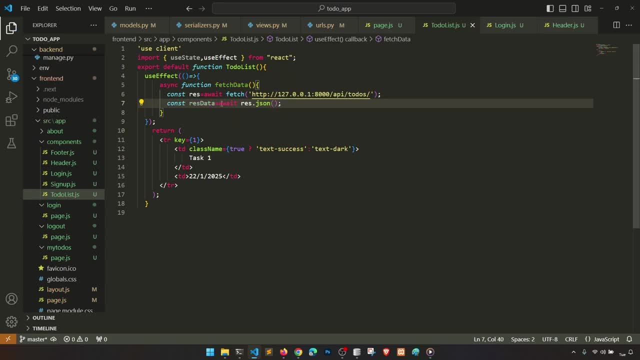 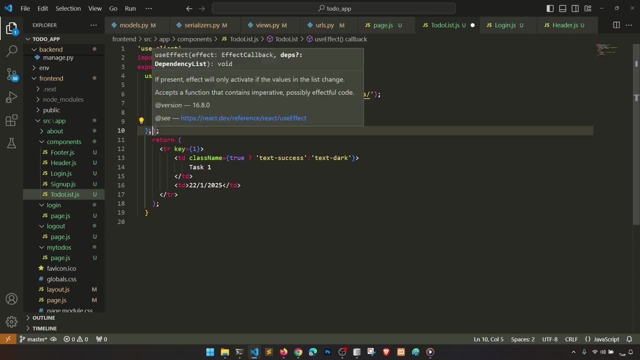 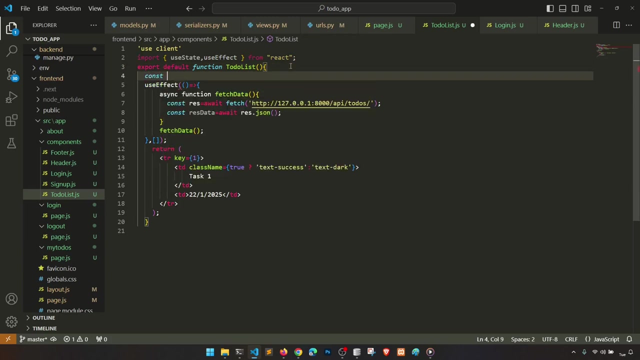 ssi equals the status option and the default, and please also define the status dot this value right here, that which is like this: this is going to be for the przyszely, so use effect will run without any dependency. okay, and we also need to create constant. 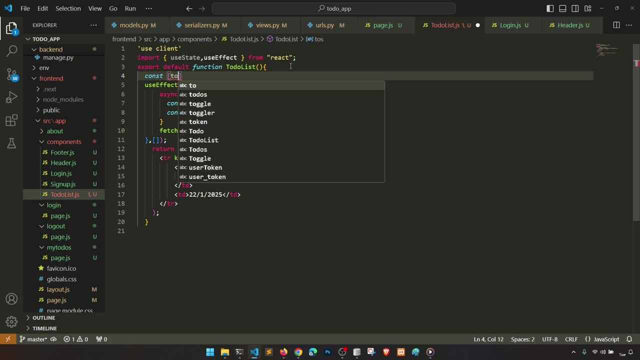 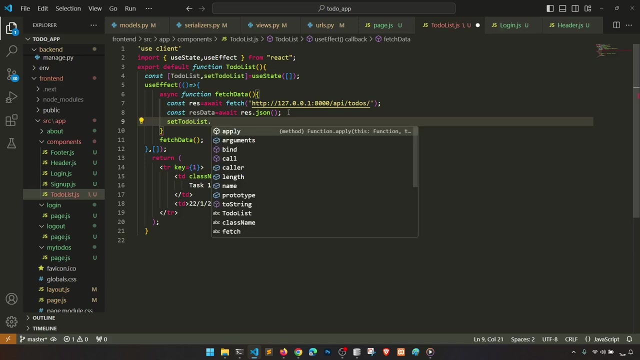 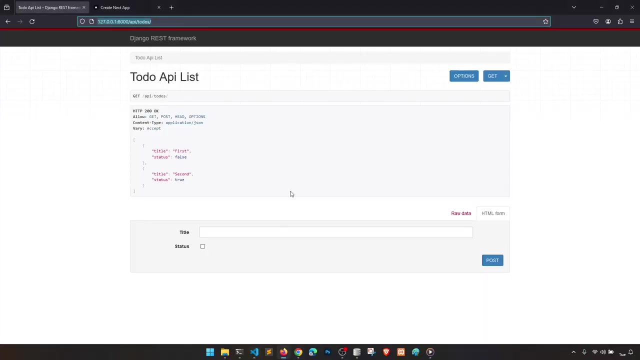 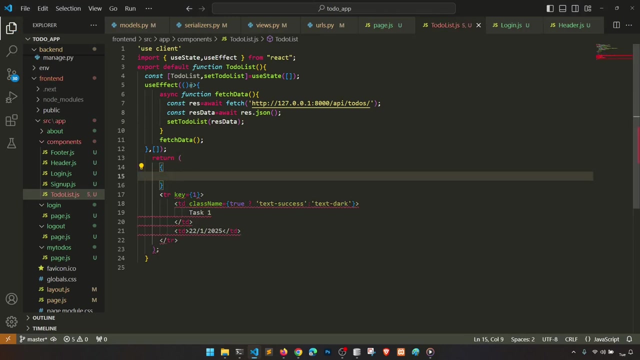 let's say, to do list, to do list, set to do list. by default it will be empty right and here, dot of search. this is response dot. indeed, okay, and uh, let's see now. then we can simply uh this: to do list, dot map, and then we can map this. 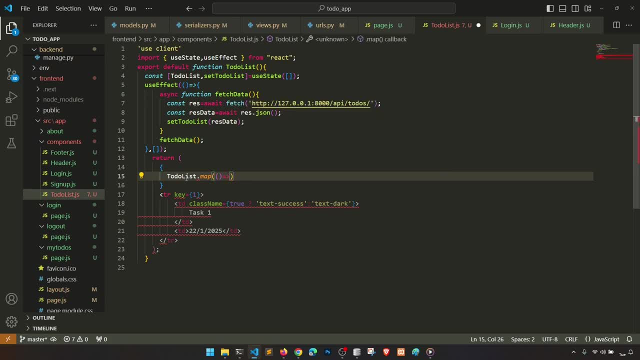 or we can say: uh, return, not return this thing. why this is showing map? oh, sorry, item index. and we can do this with this right and not sure why this is not. this should be, uh, in this right. so to do list. uh, here is a to-do list. and here is a to-do list dot map. 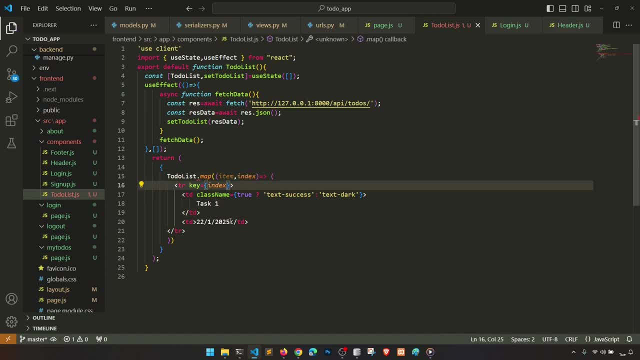 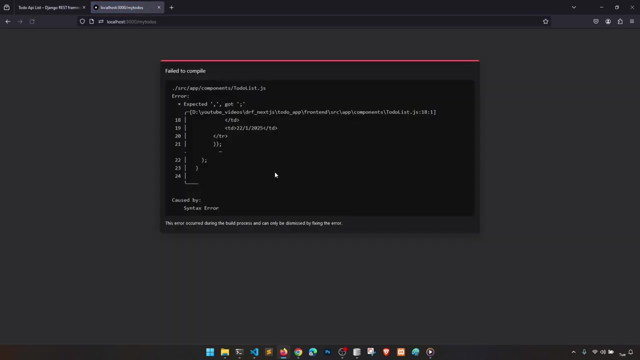 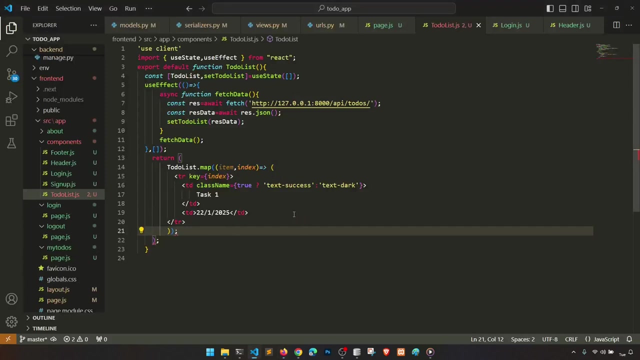 uh, let's say this is index return. i think this will not come, okay, all right, then let's go to next app. and this is showing 18 number line. issue why this is showing? uh, this function is closing here. this is closing and i think it should be. 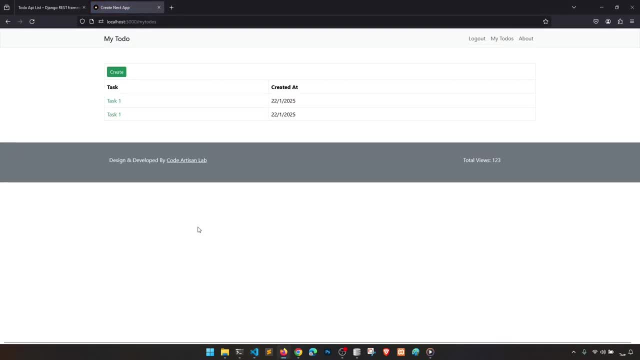 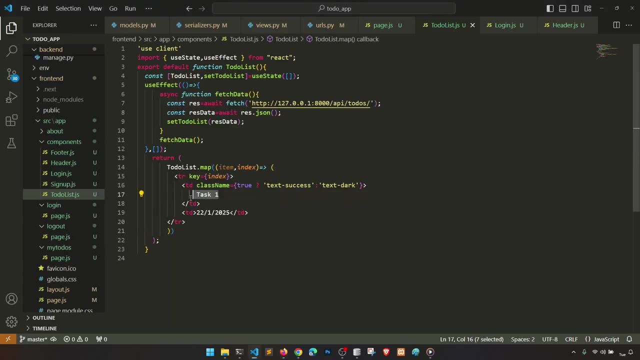 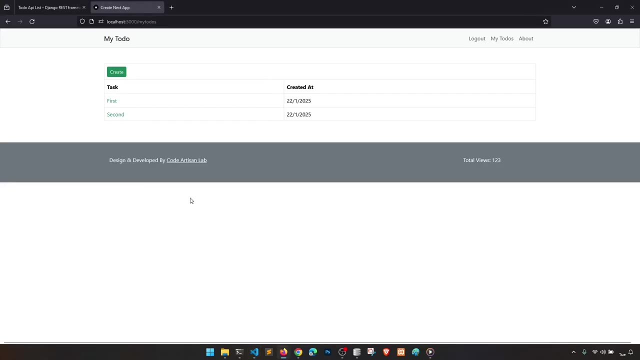 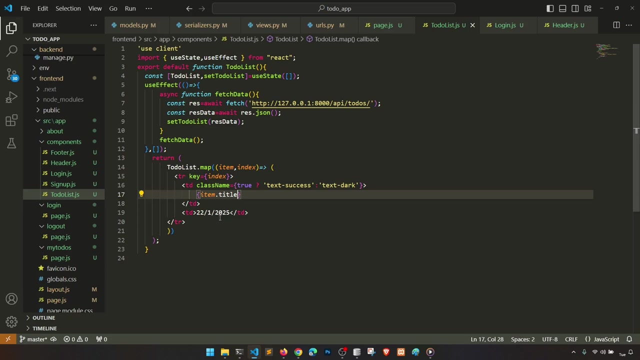 where we are doing wrong. right, no need to close this here. okay so, task one, task one. so we just need to do uh, item dot title plus second. oh, oh, we, we forgot one thing: we need to create a auto add field, but we didn't create that. okay so, and let's add a condition if 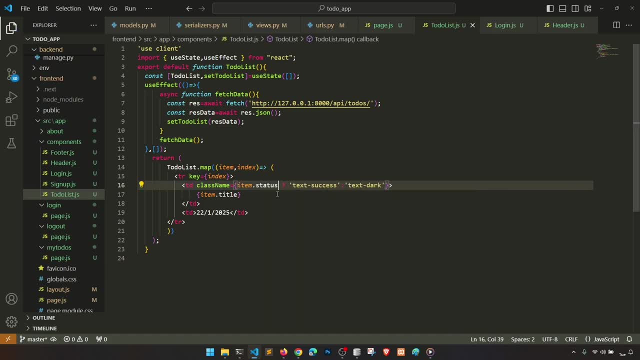 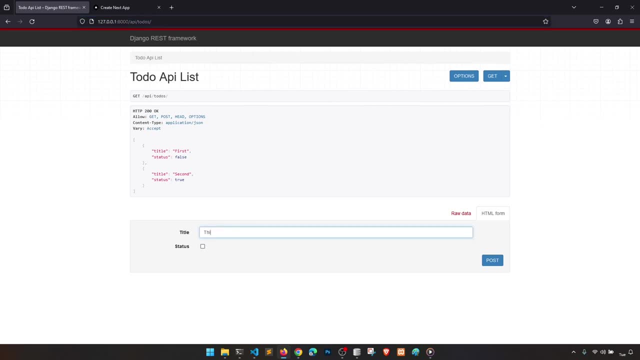 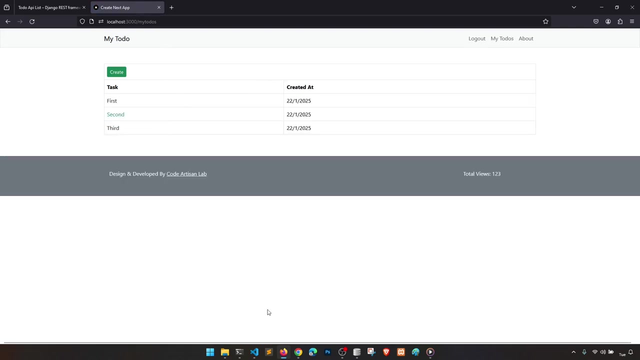 dot status, then text success, else the text dot right. so you can see here: this is a first step here, this is true, and let's add third one. let's post this and if you refresh this you can also see in third, this is not done, okay, so now let's add the uh auto. add auto date, add field when. 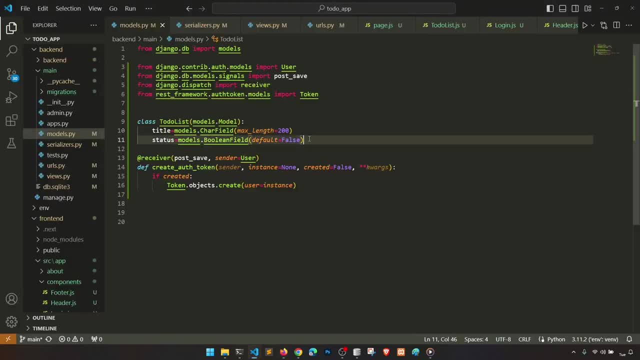 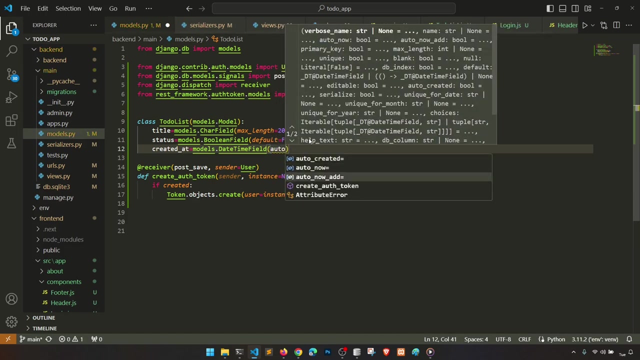 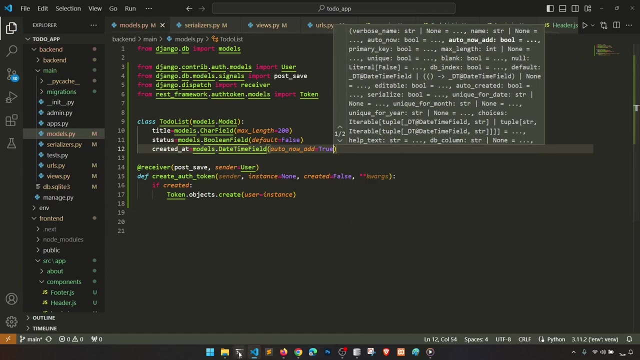 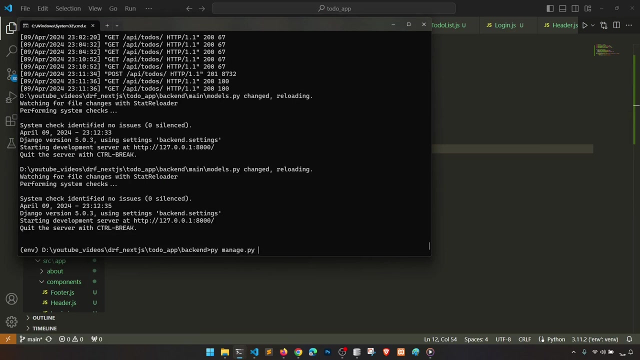 it's creating to-do list. okay, so in the model, what we will do? uh, we'll say: created at equal to model store, date field, date time field, and then auto will be true and it now let's run the migration here. py manage dot, py make migrations. 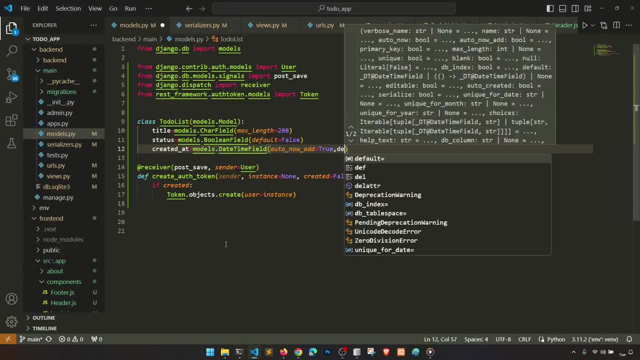 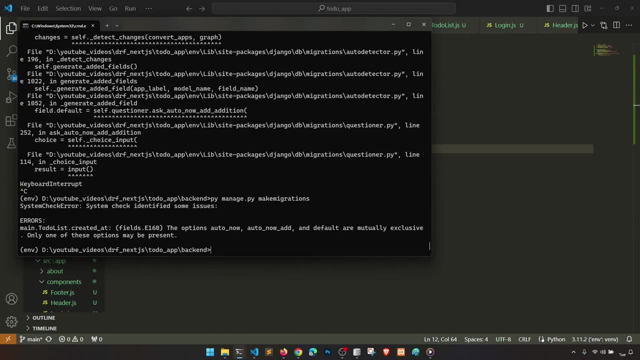 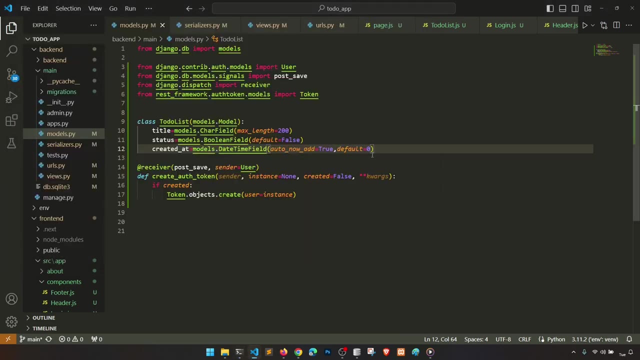 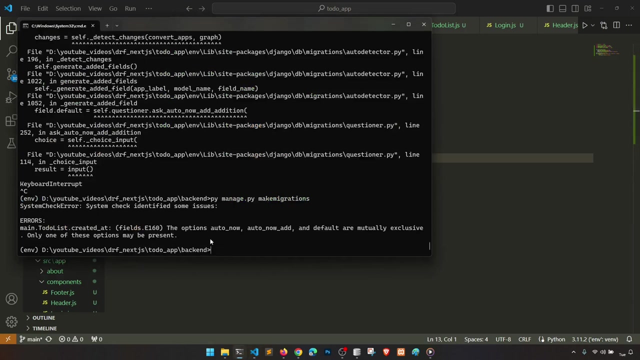 okay, it's saying: create a default. we need to define something. default equal to zero. let's say one migration: uh uh, default manager auto now after now. add what is this default? we need to define the current date and time. so it is saying the option and autonomous is one of these fields may be present. 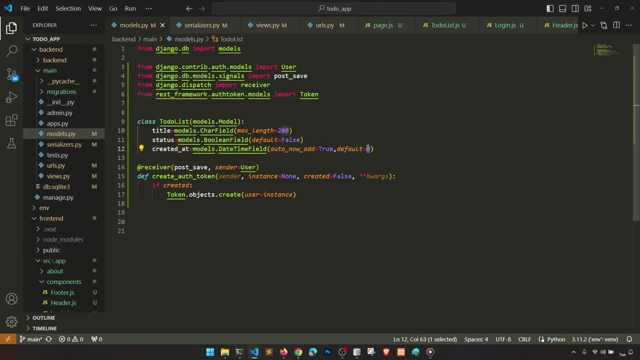 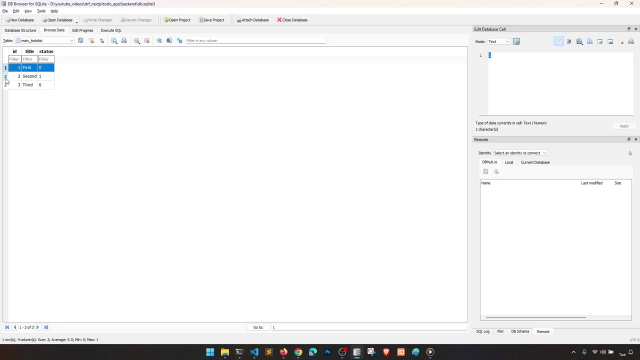 on. let's say, uh, today's date, so we need to import the date time, import date time and in this, date time dot. oh sorry, date time dot today. this is default, or we can do one more thing. let's remove this. let's go here. ah, let's uh browse this table. let's delete all the data. 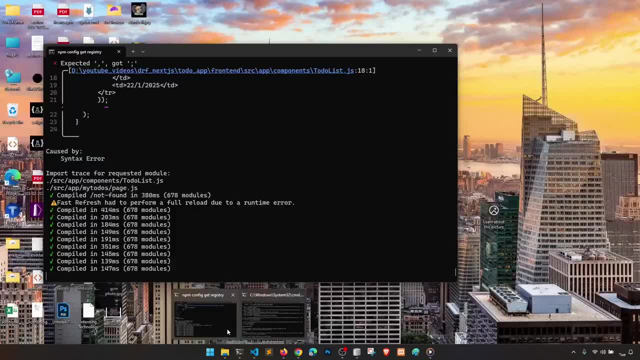 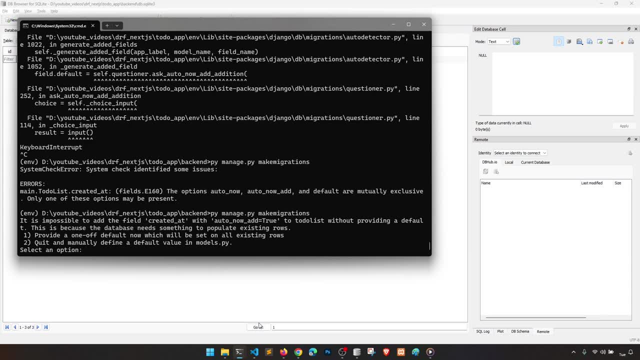 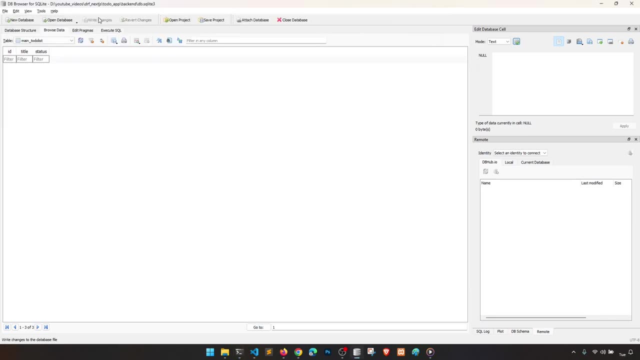 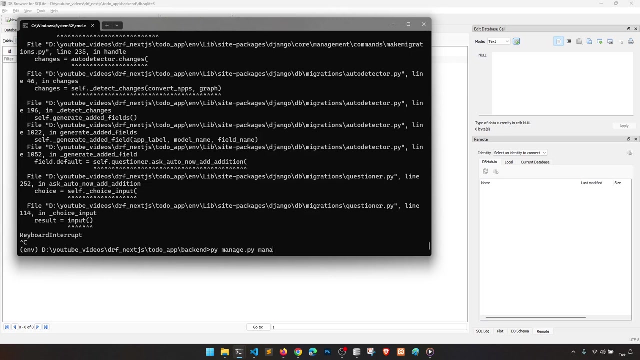 right, so let's delete all the data. then let's run the migration again. still default because data. we need something for existing row. oh right, changes, we don't have save. close, I think we have data structure, my to-do list, browse- no data, so let's run the migration again. 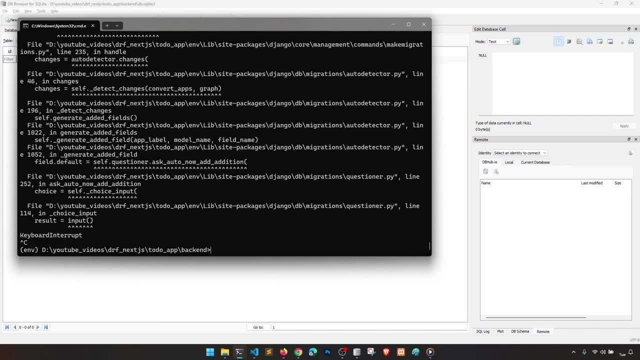 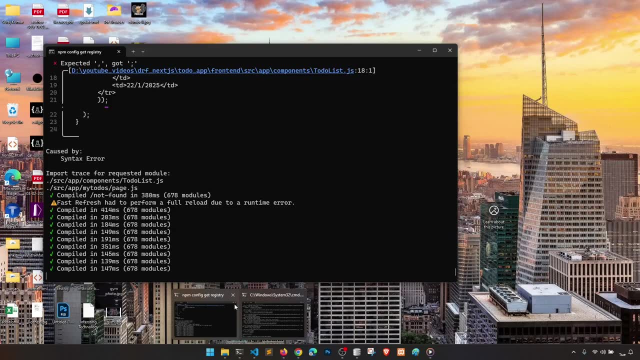 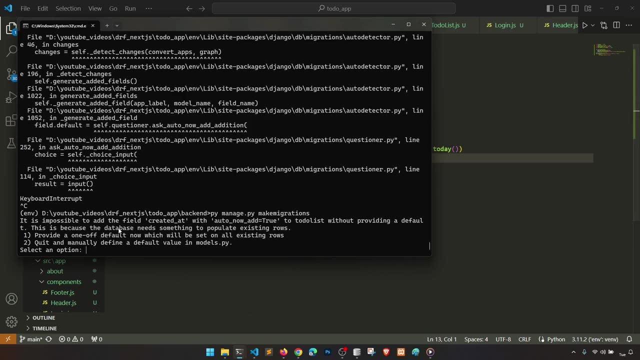 okay, let's define the default whatever. okay, let's define this all right. so make migration what is. it is impossible to add filter data to be the ordinary to default. this is because the database needs something to populate existing. provide a on of default now, which will be. 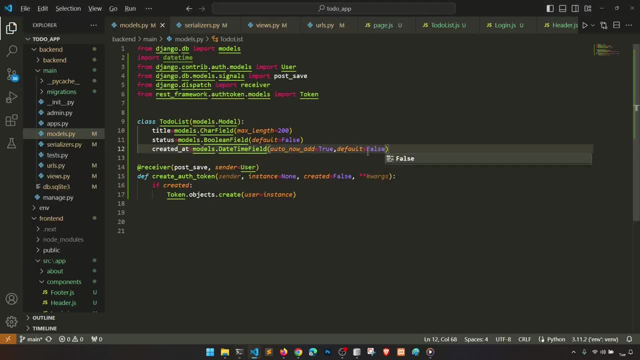 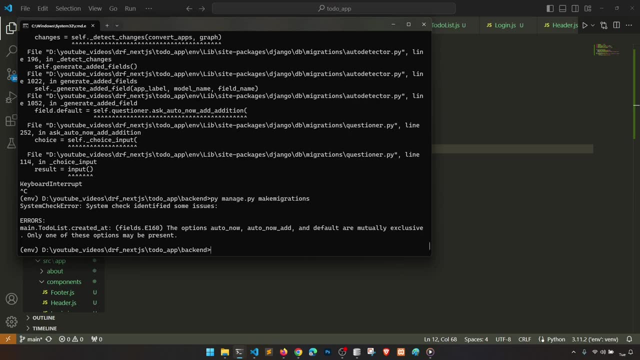 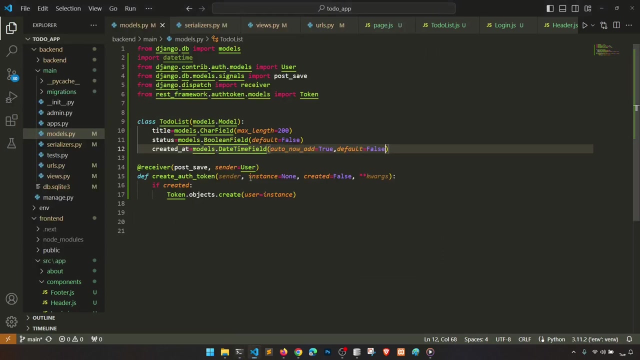 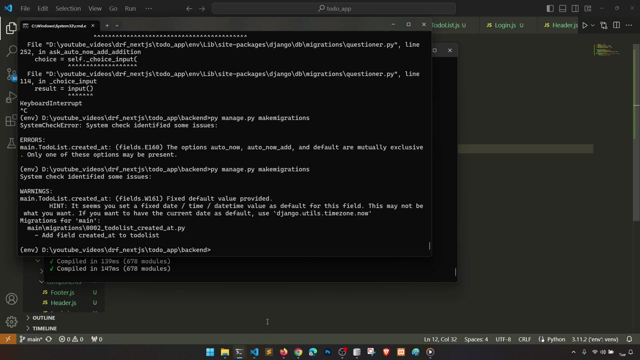 on off. let's say default. all friend, okay, let's remove this. then and and, and, and, and. okay, let's do one thing then. if it's not allowing this, then we can do date time dot. date time dot today, right, and this is date field. okay. okay, let's do this okay. 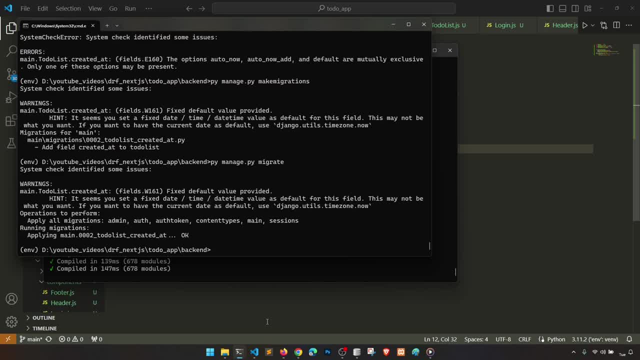 nspy migrate right and then managepy to enter method every time. lovely this. as you can see, everything is working like this and I hope you liked the video. In the next slide we will be talking about formatting. Okay, so here you have to click and install. 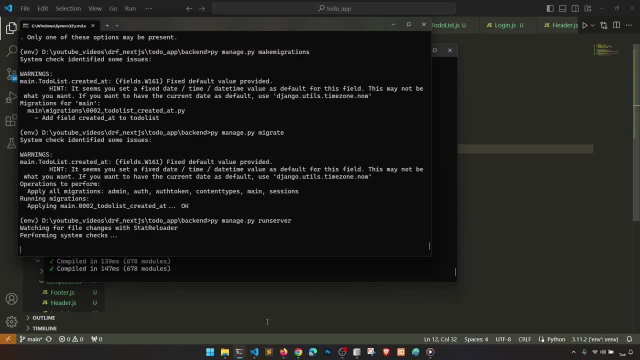 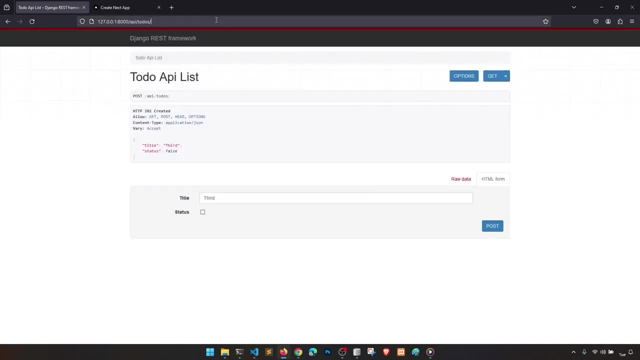 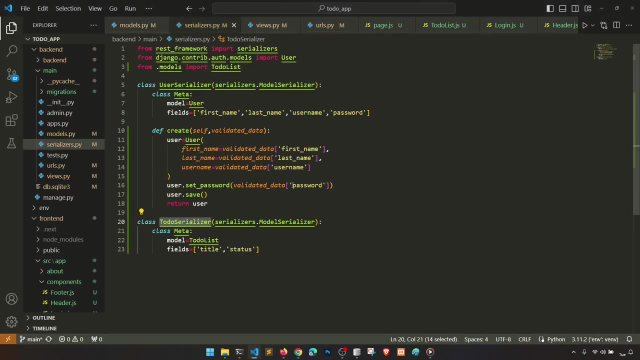 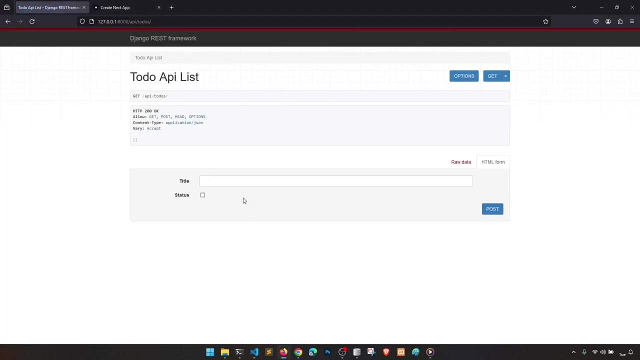 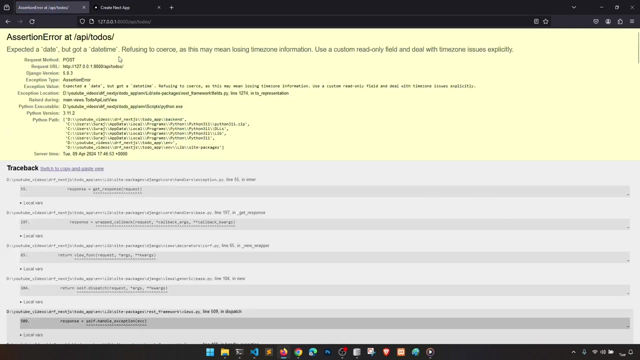 py run server right, and if i go here and click here, refresh this page, oh sorry. and one more thing we need to add in the serializer also. so this is: this will be created. all right, then this is title post expected, but got date time refusing to, refusing to. okay, uh, this is. 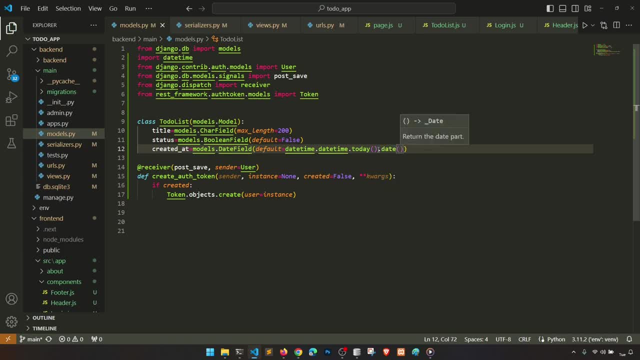 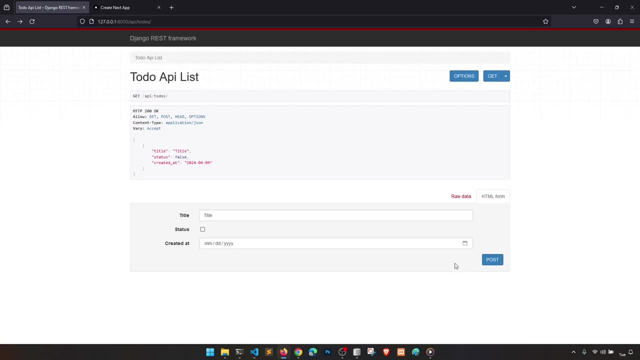 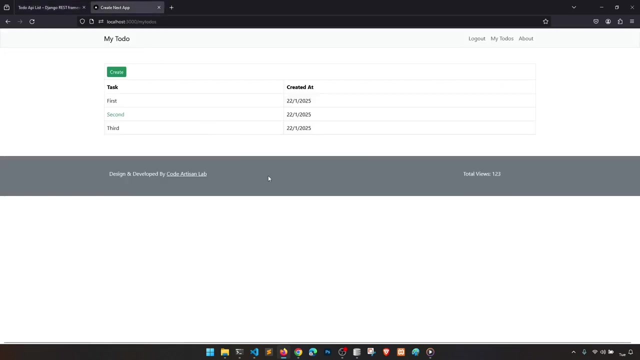 torch date. okay, i think it should work. now. let's see refresh title: calendar 9- post data is posted, okay. so, uh, it's working now. and if i refresh this page, we have uh two datas and uh two datas. let's show the data also. so here we have. 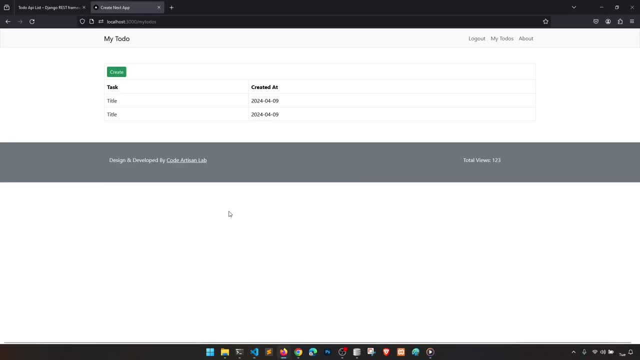 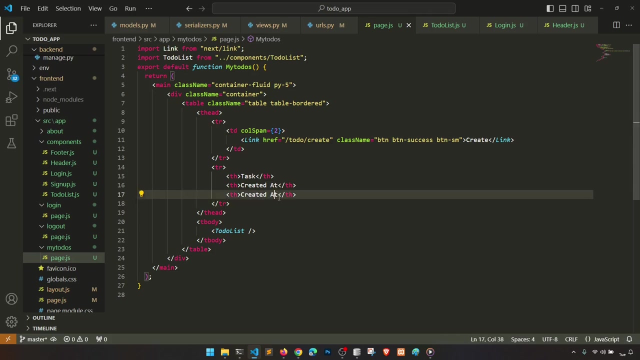 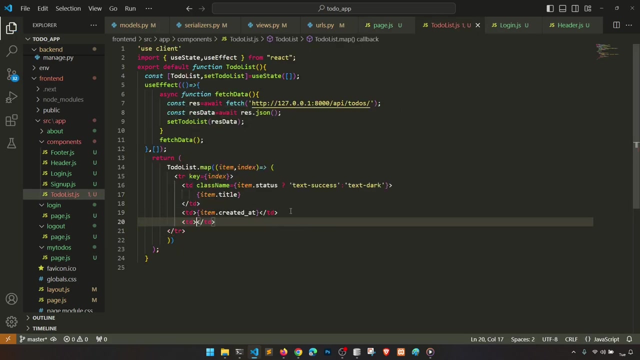 uh created, right. so this is the data. now we need to create the ad form and we also need to show the update data, right? so what we will do- uh, this is to do list task created at: if we have a page, let's copy this one and let's say actions, right, and in the sections we should have this thing and, uh, we. 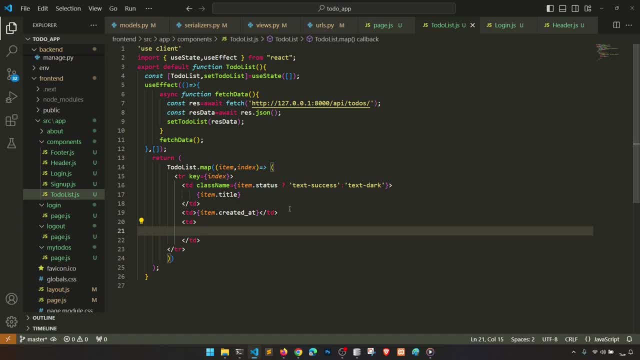 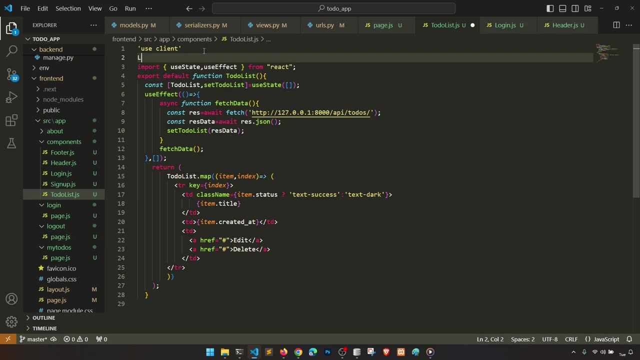 will define our two links: hr here we will say edit and we will say delete, right, uh. and also we need to do a link, we need to import link from from next link. i'm not sure why this is not working. it should work, but let's see. 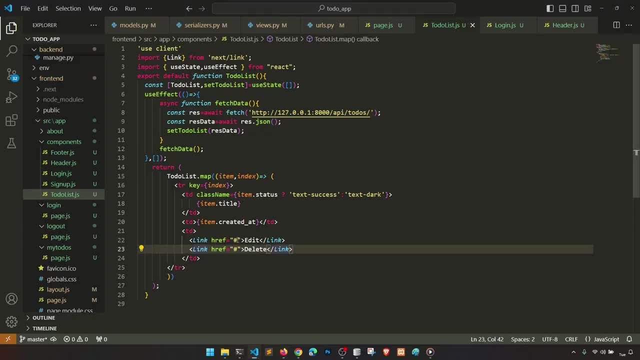 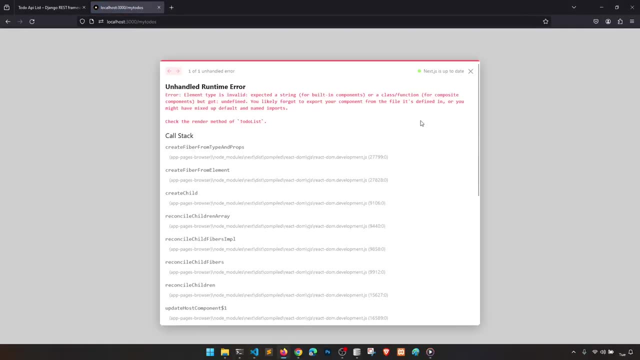 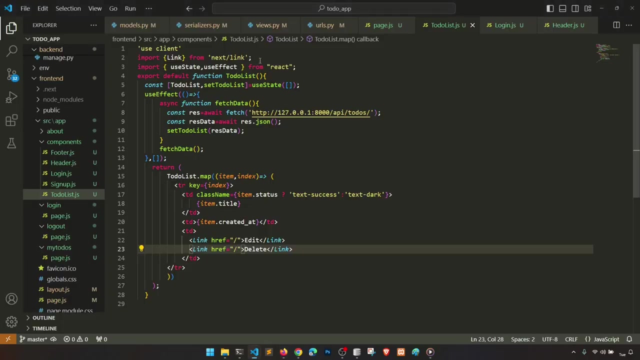 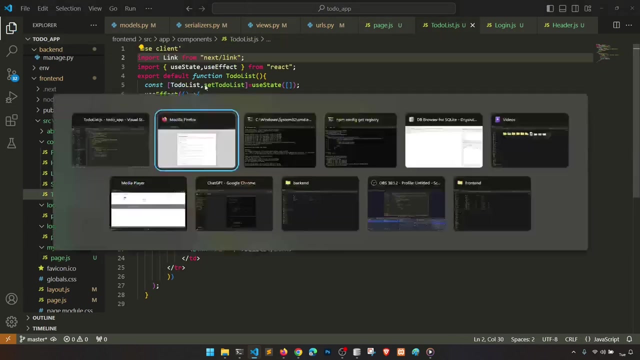 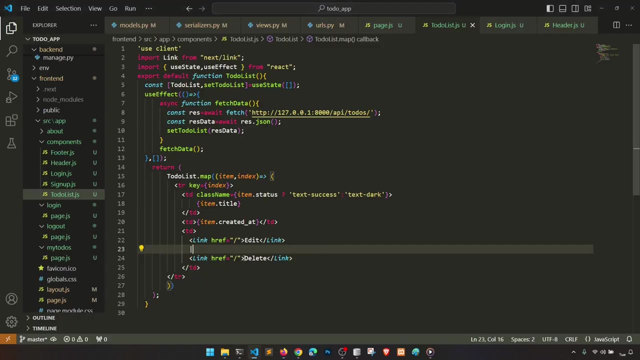 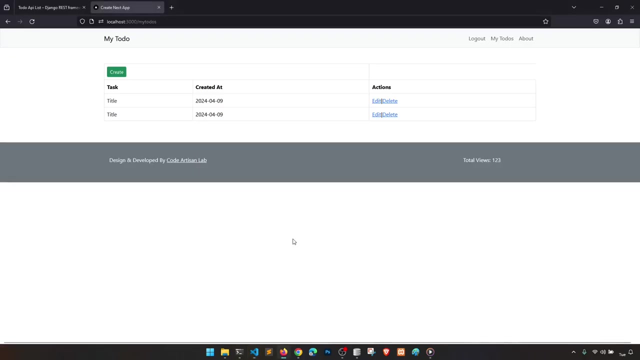 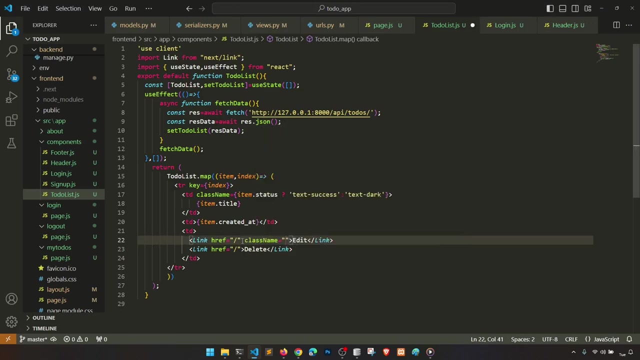 all right, okay, let's say, hash element component is exporting link from: oh sorry, all right, so edit, delete. uh, let's do one more thing: separator, separator, this kind of thing not cool, not cool. then let's make it cool. button button, info button, sm right and then class name button, danger, and then margin, start to. 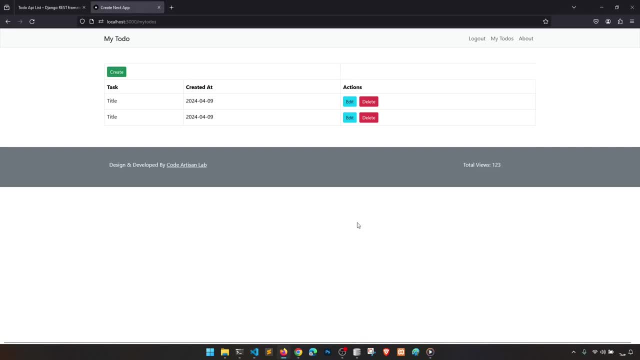 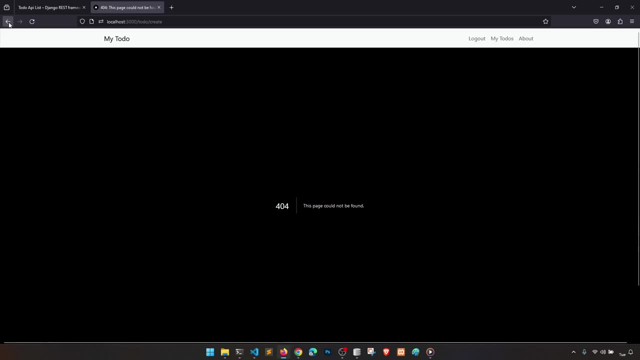 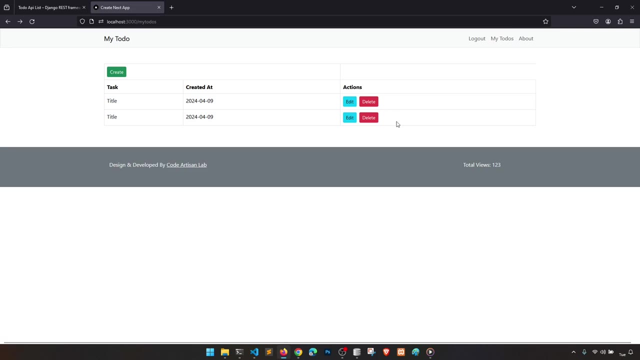 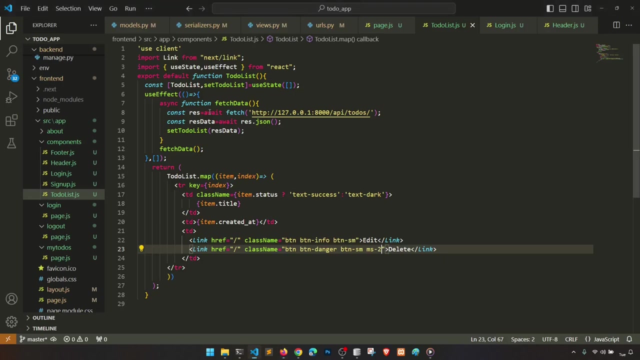 okay, so when we click it, it should open the update form. when we click this, it should open the create form. uh, not here. when we click this uh, then it should delete the uh task, right? or we can say: uh, come, let's say. we can say done. we will say success, right, uh. one more thing: i'm still thinking: if i do the 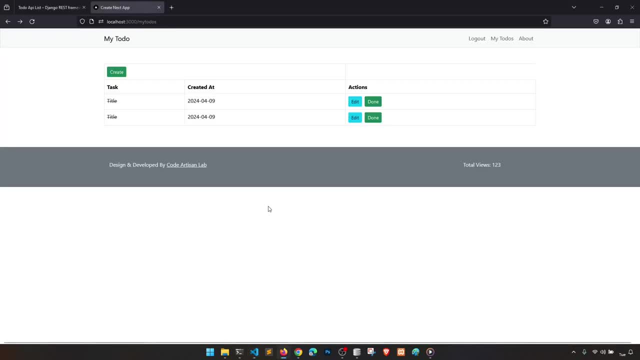 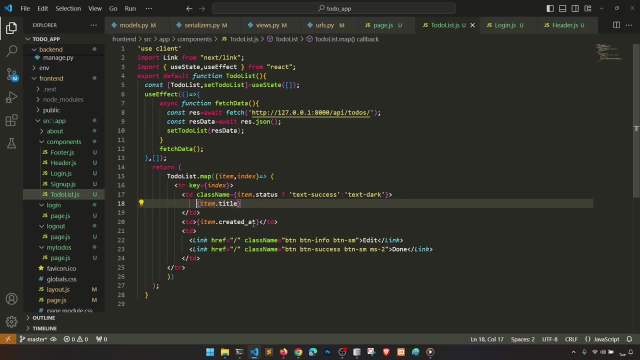 s in this. okay, great, so if status is uh done, if status is done, then what we will do here? i will do one more thing. i will add a link here. okay, so let's do one thing: let's not add this class name, but let's add, if status this one, then 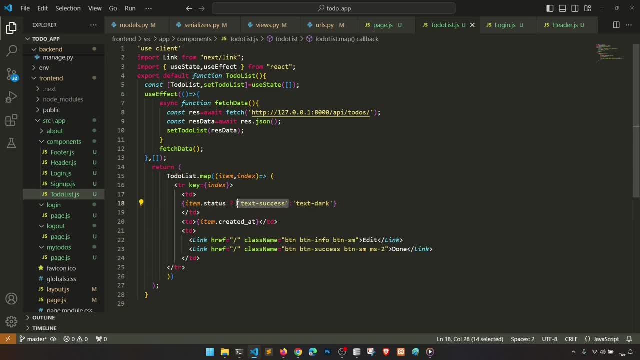 we will do s and here we will do item dot title right, else it will normally show item dot title, always the issue: where is the issue? where is the issue? I think issue is here. issue is dollar here and then dollar here. okay, um, why this? is saying text dark. 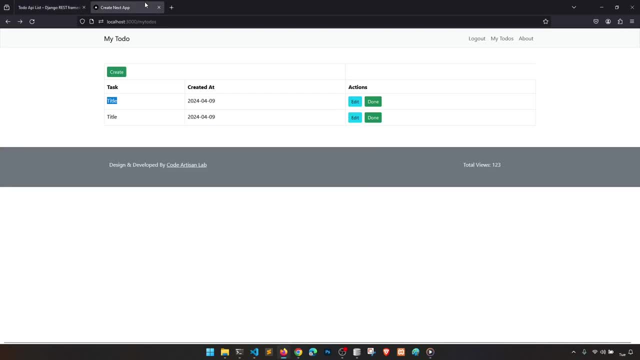 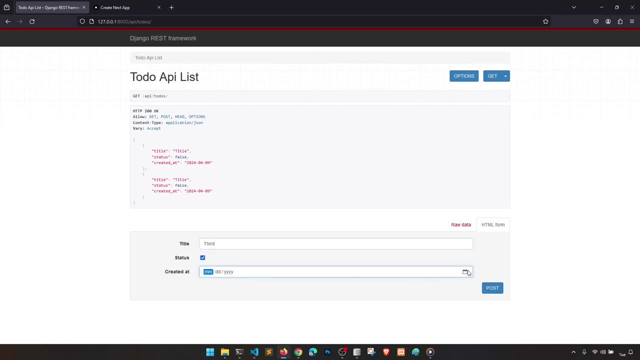 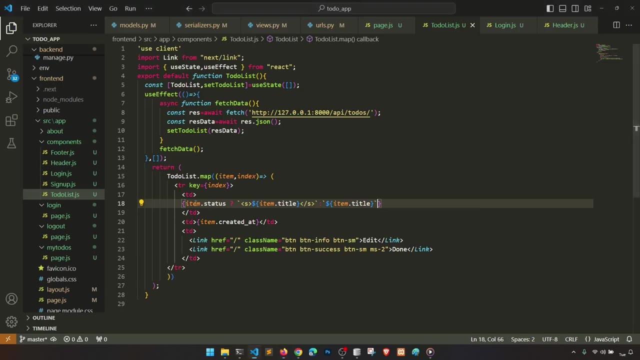 all right, so this both task is not done- false. so let's add one more task, or done, and date is here. host refresh: Oh great, this is showing as a string, but we need to show as a data. let's remove this one. okay, so this is done, and if it's done then we no need to show this button. done, right. 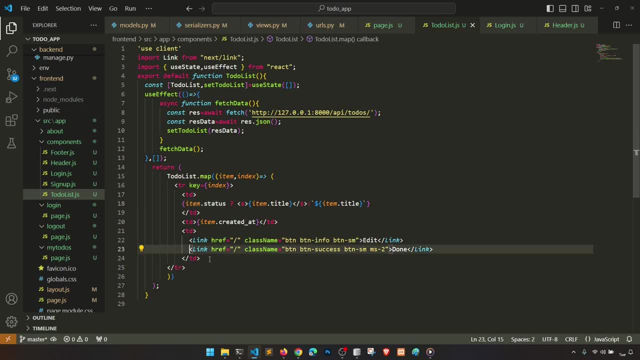 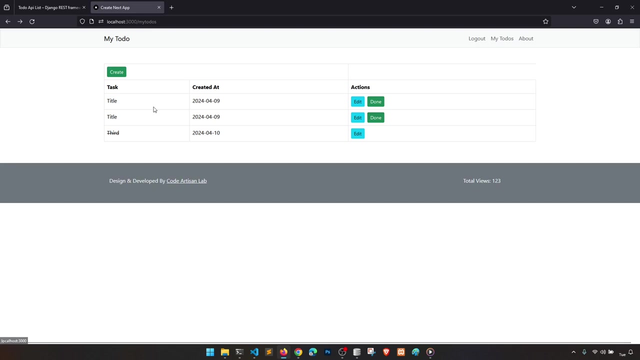 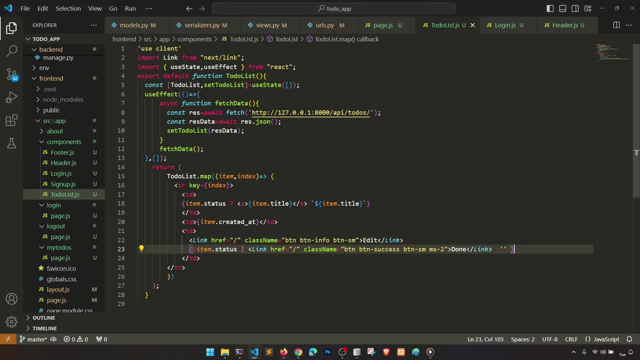 sorry. so if not, then we will show this button, else we will show nothing, right? so this is so. when we click on done, it will add the strike, right? so i think i think we should add the strike and we should also make it some class name. sorry, sorry, i'm taking too much time. 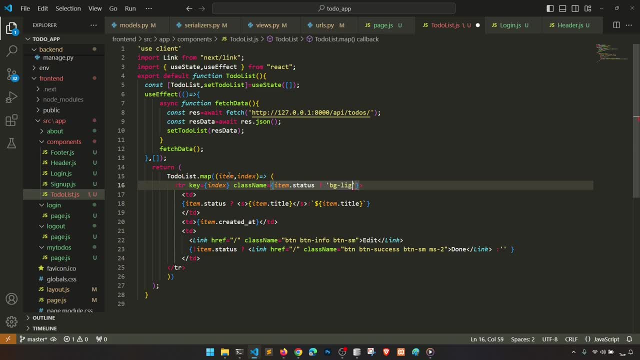 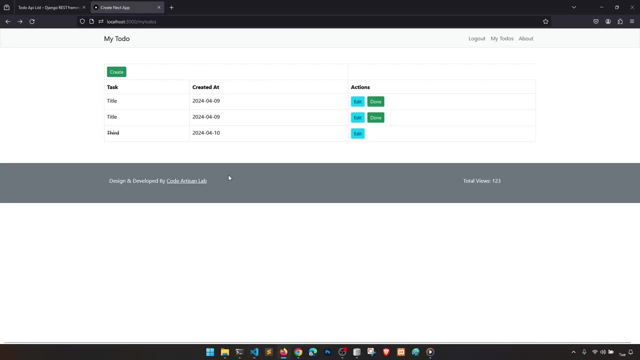 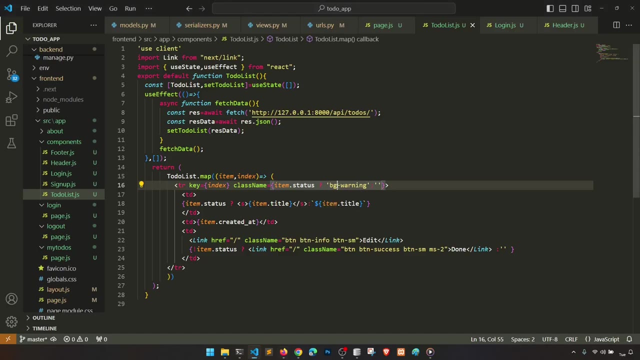 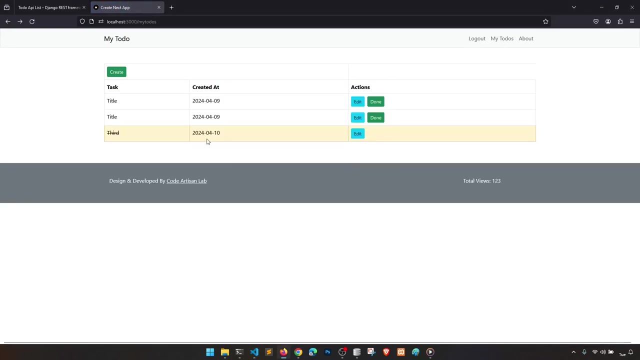 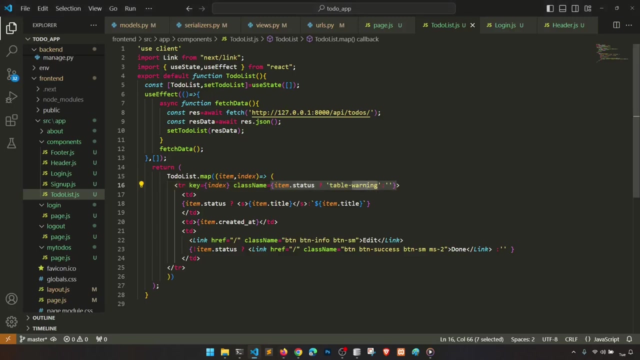 so i will say bg light, or we can say bg warning right, and then else nothing, right, so it's not, it's not taking the okay, now it's taking. so third, and this is warning okay, or we can say: uh, secondary, okay, so when we click on this, no need for edit. also, 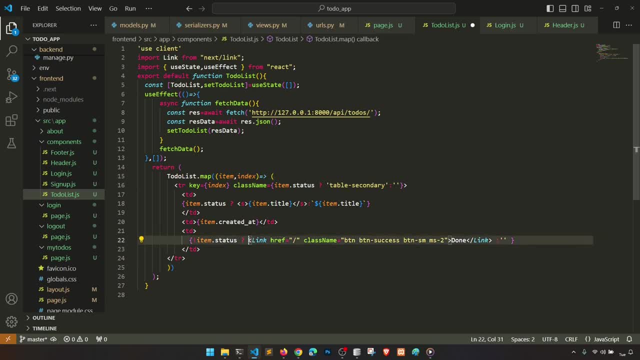 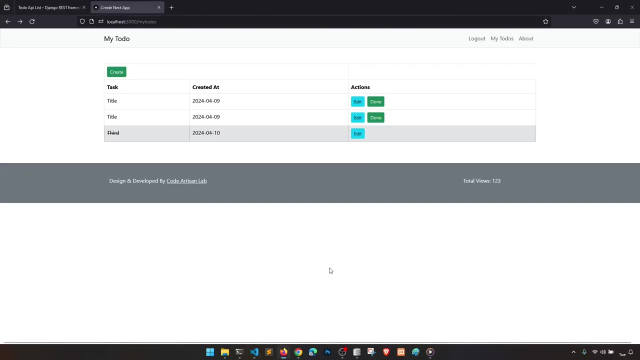 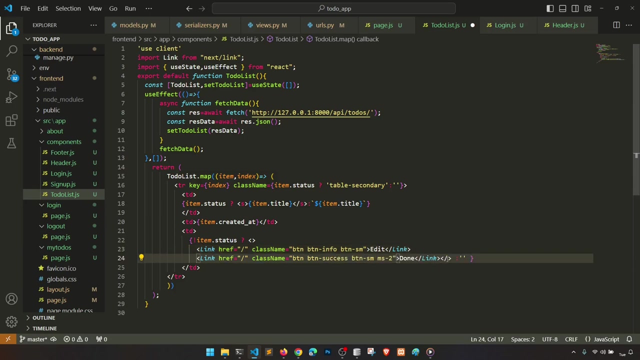 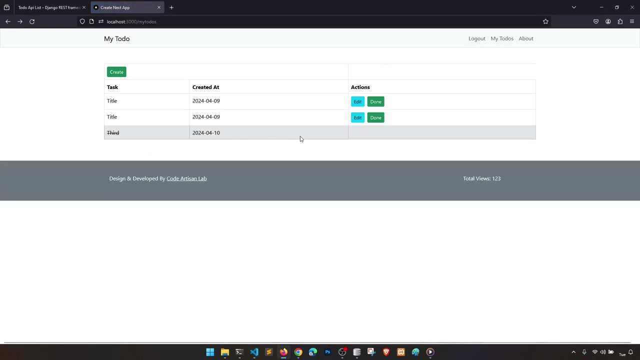 okay, if task is done, it means done. okay, we need to define this thing, fragment, or we can see the parent tag. okay, all right, here we have the parent tag. okay, so now this task is done. so now let's uh work on the done section. when we click on done, 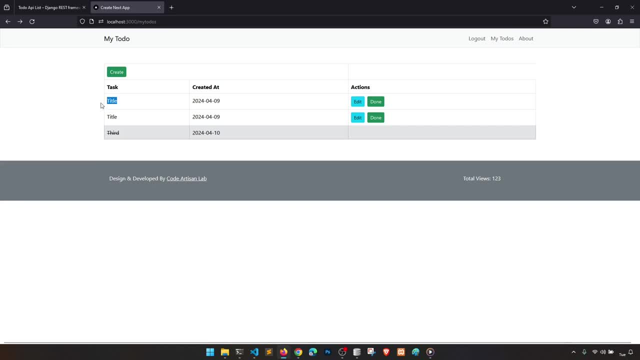 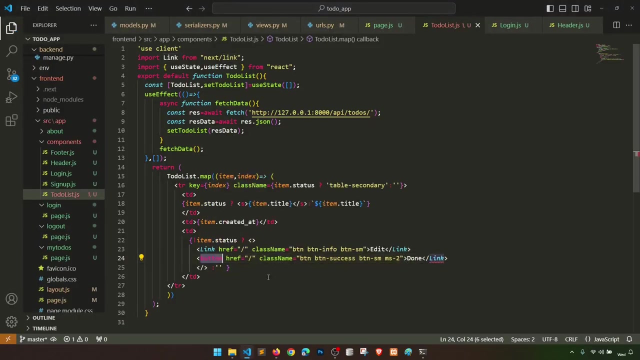 it will add the strike on this task, okay. so what we need to do, let's do on. let's do work on the creation right, all right. so when we click on this turn, it should add the strike right. so for this, first of all, let's make it a button, right, then this button will go here. 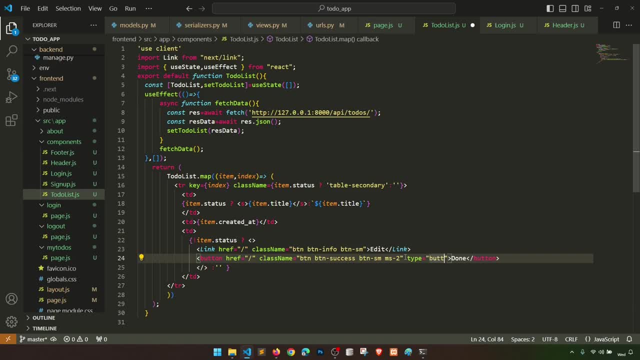 and then this will be type button and we will add the on click function. so on click, task done, handler. and we need to pass the id right. so item dot, id right. then we have to make it a function right. so task done, handler right, and then we'll create a function here. function. 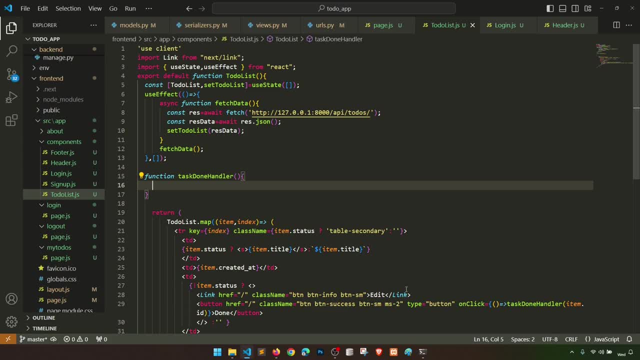 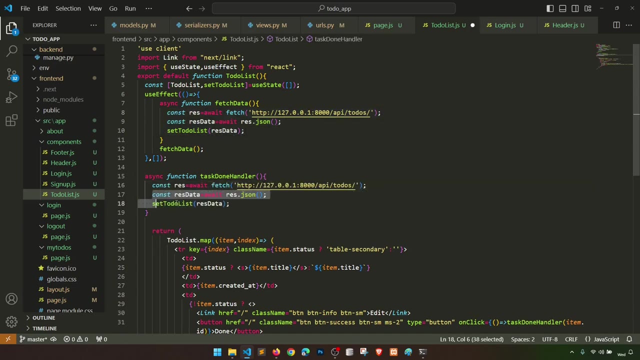 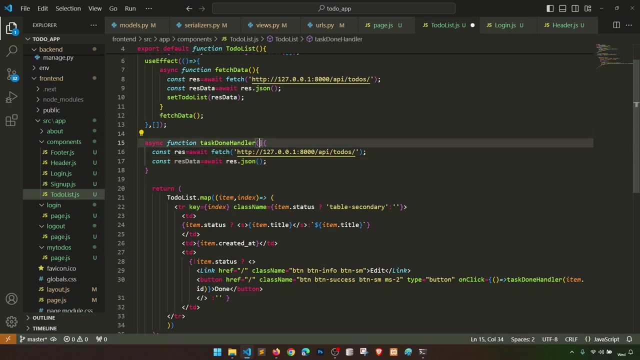 task done: handler right, and uh, this: uh, we will create this function as a a synchronized function and we will do this copy paste, right, okay? uh, let's do one thing: set to do list. okay, so no need to check this. uh, task done. so here we have a task id right, api to do. uh will pass here. 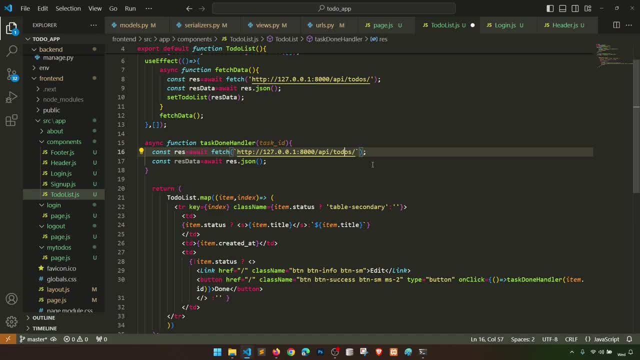 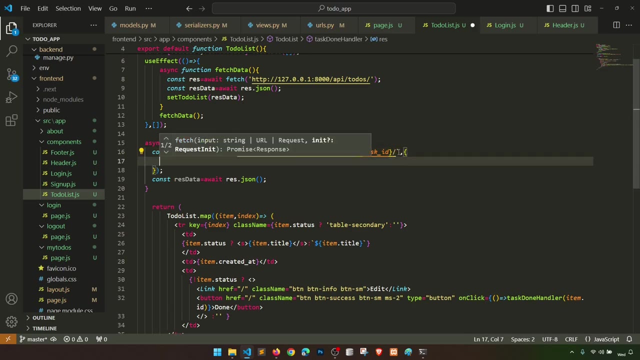 we'll pass here the task id. we also need to create the function. uh, we're going to create the api for this. we'll create that. so this is the task id and we need to pass method equal to foot, because we are updating the data right and then we need to. 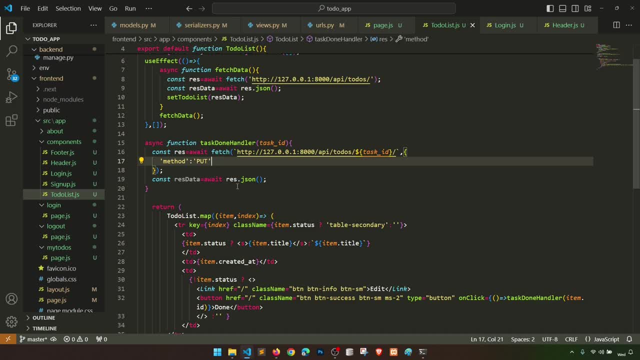 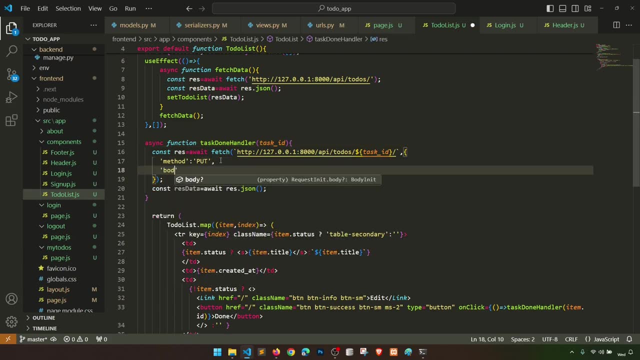 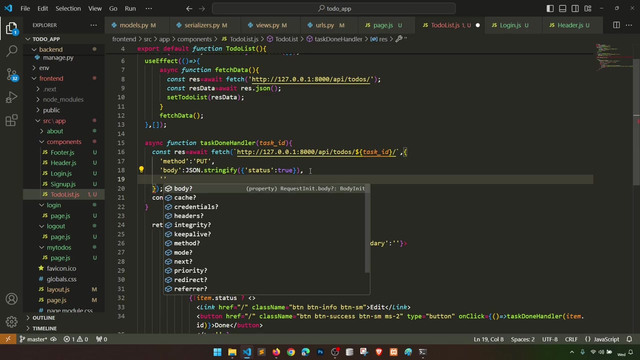 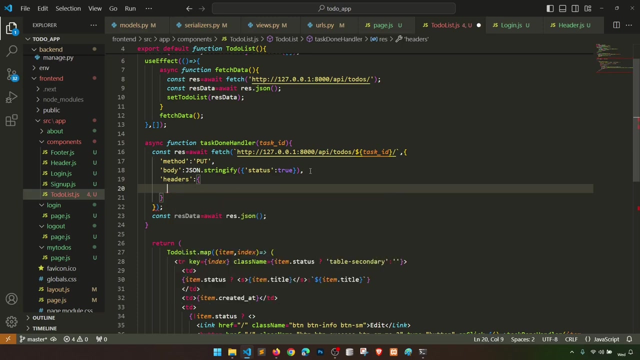 okay, so this method is put and we are passing this thing and we also need to pass body. the body will be: json dot simplify status false. uh. status group: right. so the json dot stringify status: true. and then headers: content type: content type application: json right. so this will give us response. let's 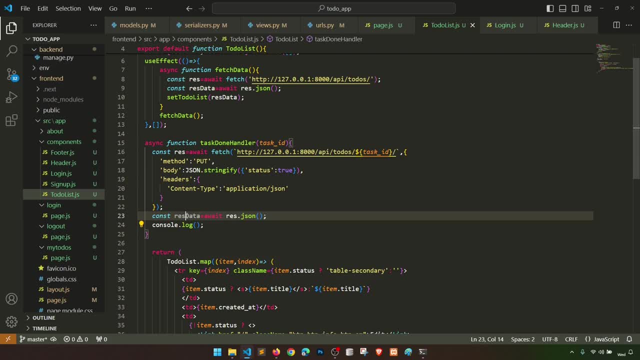 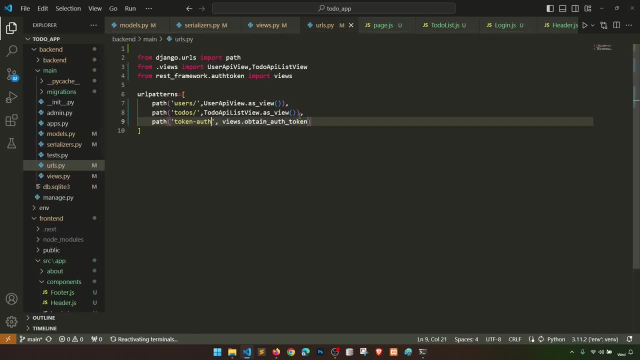 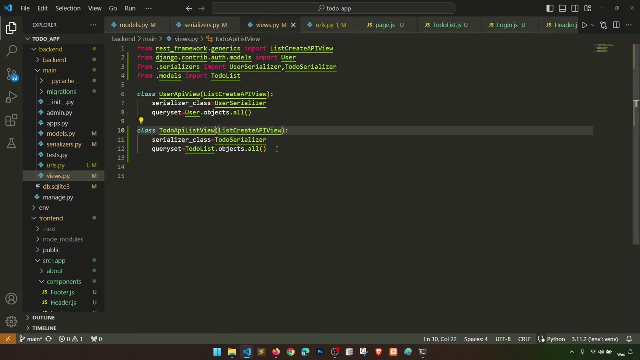 console the response. okay, console this response. so, and we also need to create the api. so let's create the api also. so copy this, one, paste here: and we need to pass the pk primary key. uh to do to do api, update view. right, so let's create the update view. copy this: 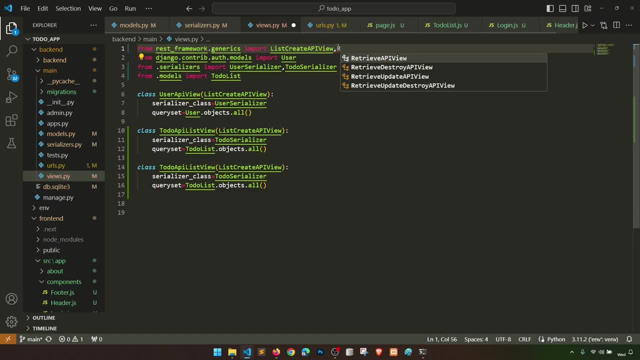 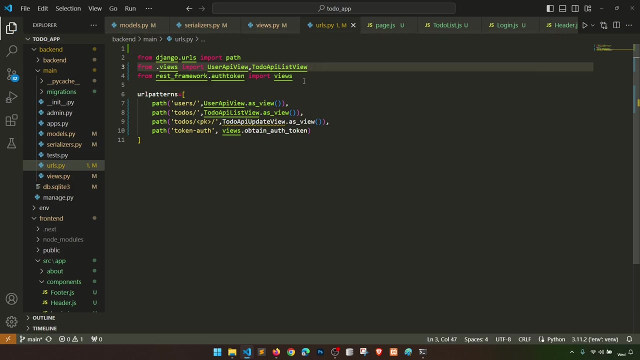 uh, we need to fetch the retrieve destroy, retrieve update, destroy view. okay, so with this single mixing we can. we can update data, retrieve data, deleted, right, so to do list. this is, uh, here we need to fetch this to do. is that views dot, sorry views, api views here to do list update. 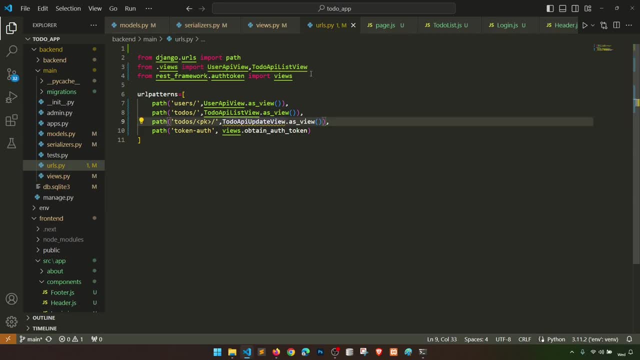 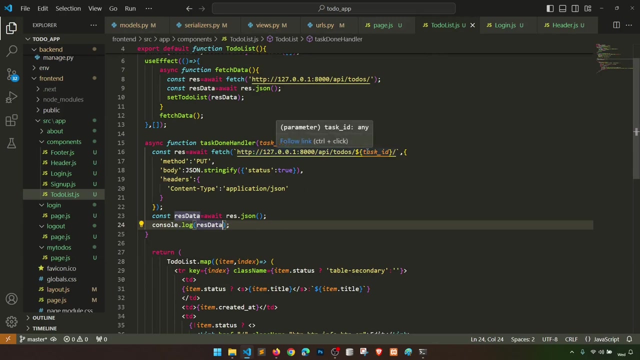 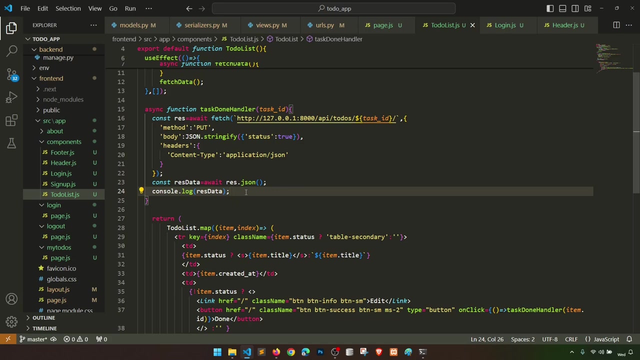 copy this and paste it here. okay, so now. uh, from from here. so when we run this function, it will go here, and then it will go in the view, and it will. it should update the data, right? so, and we also need to do, one more thing we need to do. let's say: 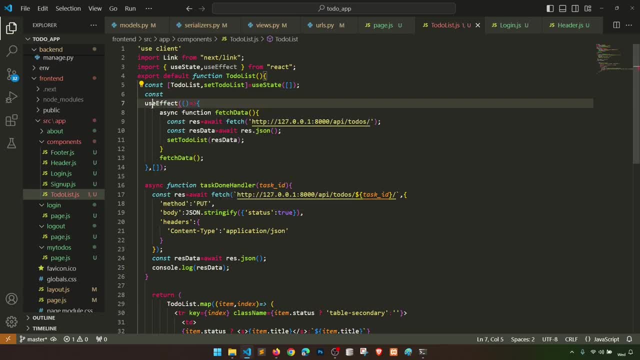 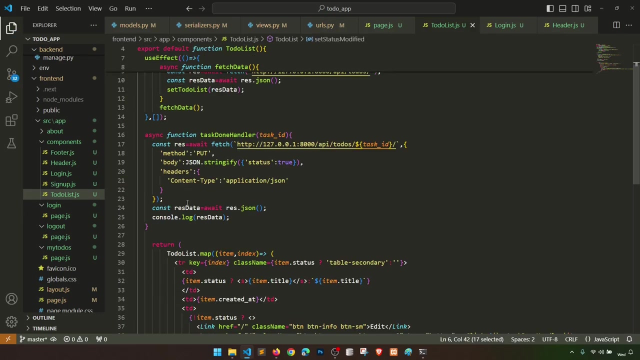 constant because we want to run the use effect, and use effect run whenever we change the state. so let's create one more thing. uh, let's say: status modified, that status modified, right, so by default it's false. use state: by default it's false. and after: uh, if we say: 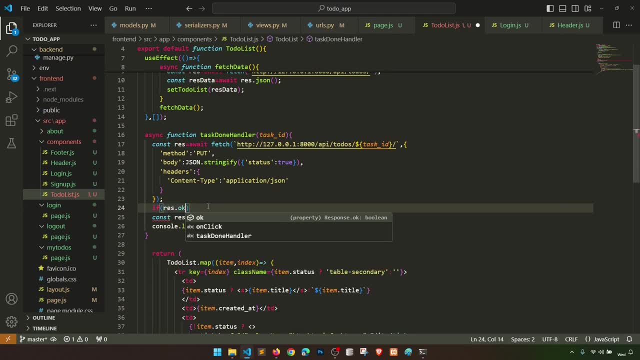 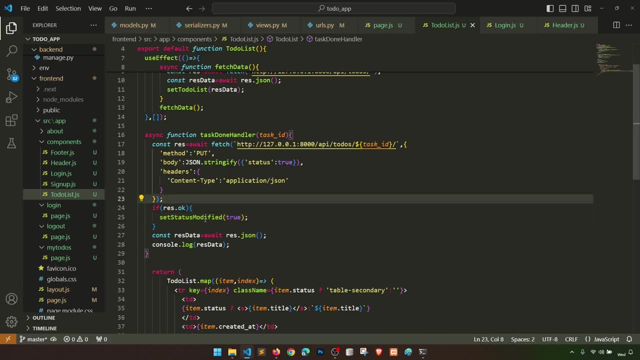 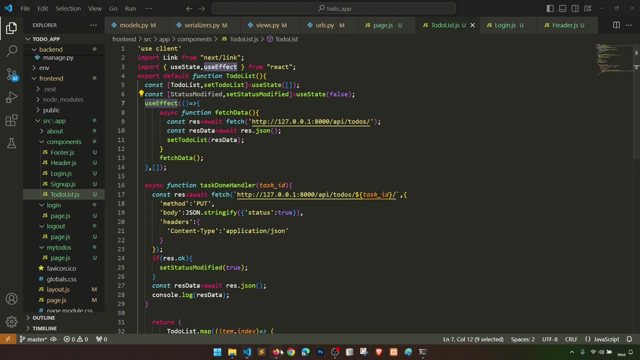 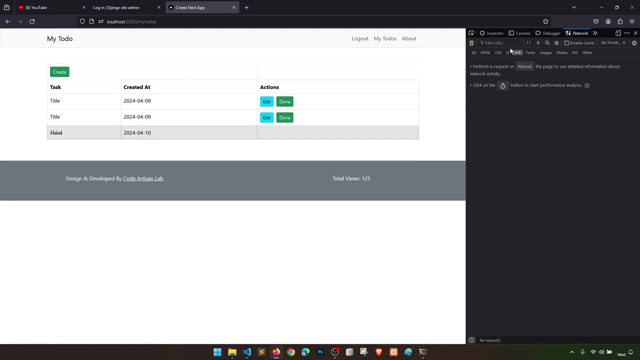 uh, if a response dot, okay, then we will say true, right, so whenever we change the state it will run this use effect. okay, so now let's try to check this. so when we click on here here, here done, let's say what it is saying. now it will say: uh, 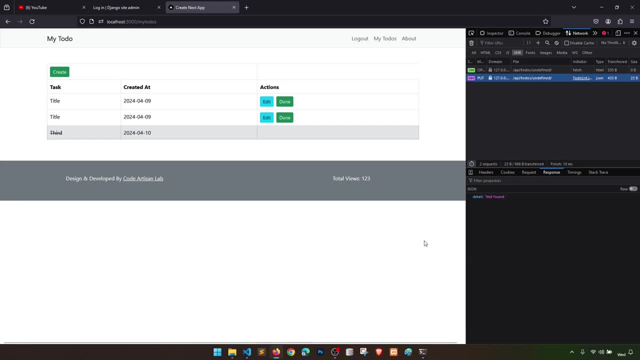 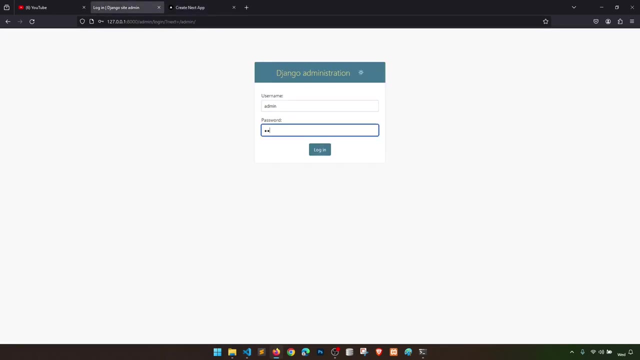 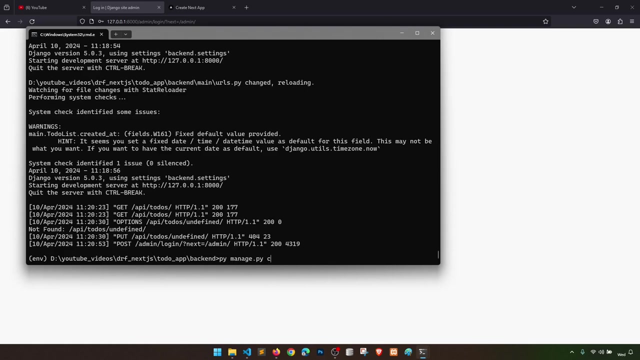 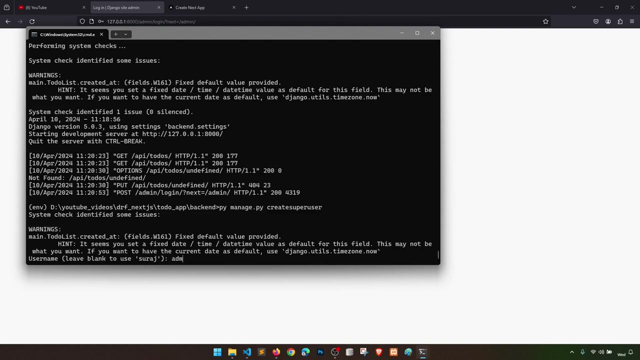 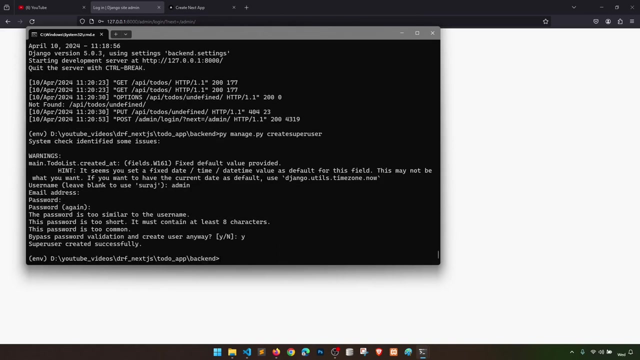 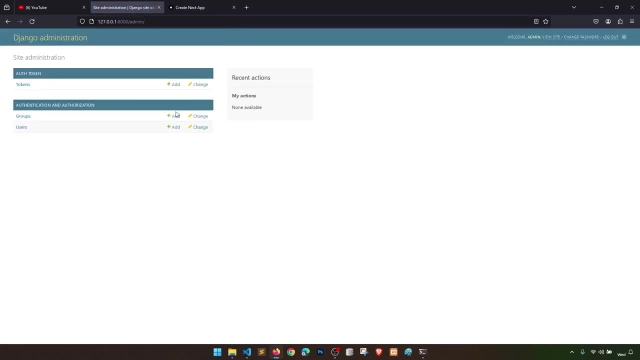 response: detail not request status: true and detail not found. let's go to admin and let's try to run the app api from there. what is this it's not using? let's create them: py, manage dot py. create hyperuser. okay, server login. and then we have. 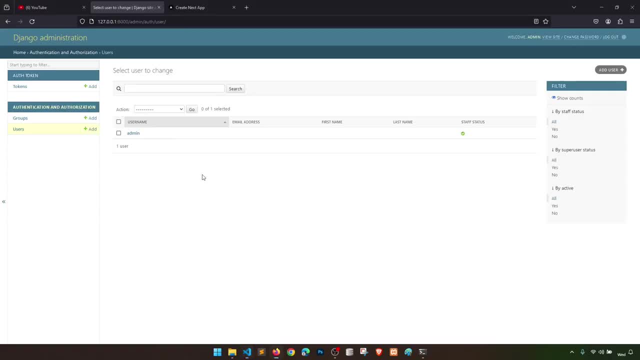 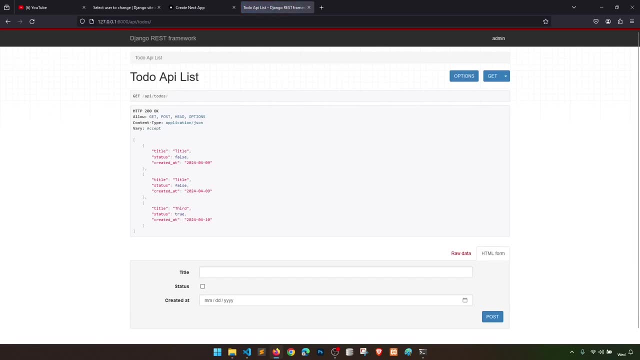 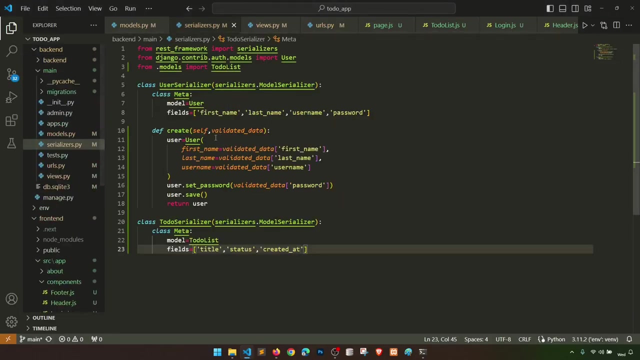 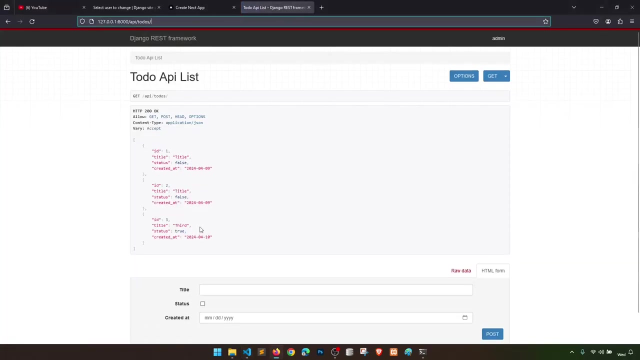 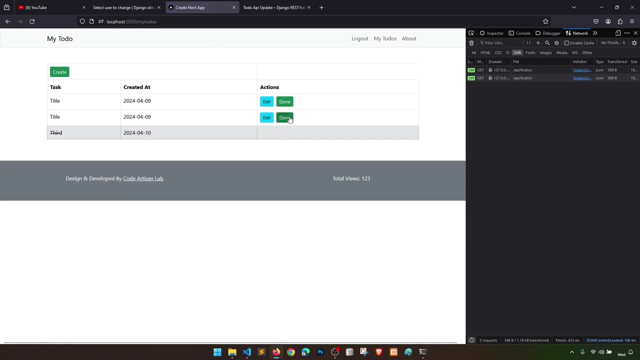 a to-do list. okay, we did an to the to-do list. okay, let's go to API. then here we go to. API is to lose. let's go to to do. Oh, one more thing in the serializer we have to add ID here, right, so ID, let's save on. so this is saying the data and if I click here, done then. 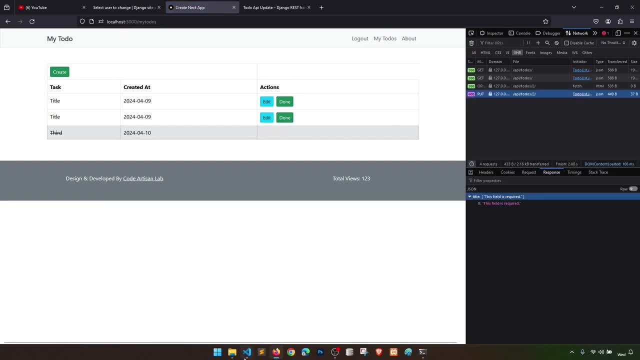 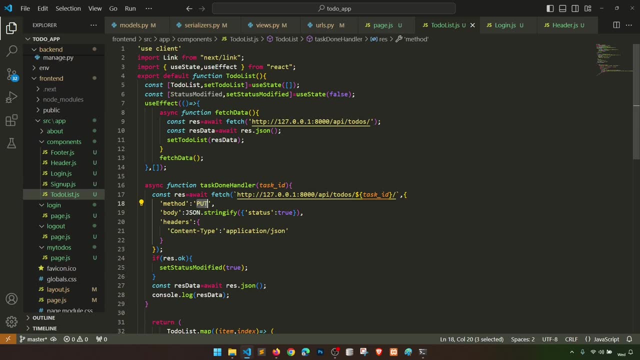 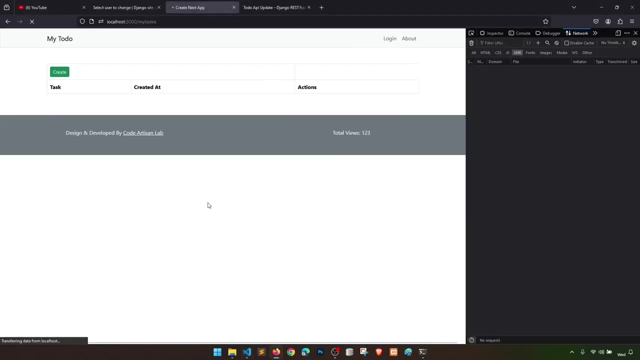 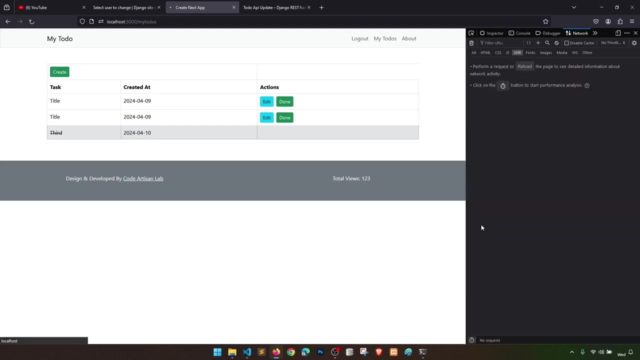 it is saying title field is required. okay, so one thing that we can do: update, update patch. click here and see this. so this is saying status: true, and if I refresh this page then it is working, but now it should. it should automatically add the strike, right, so it. 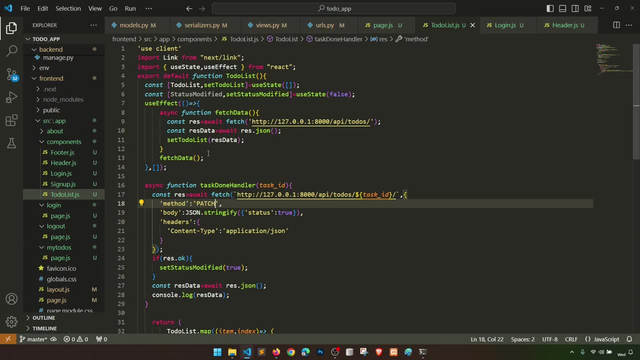 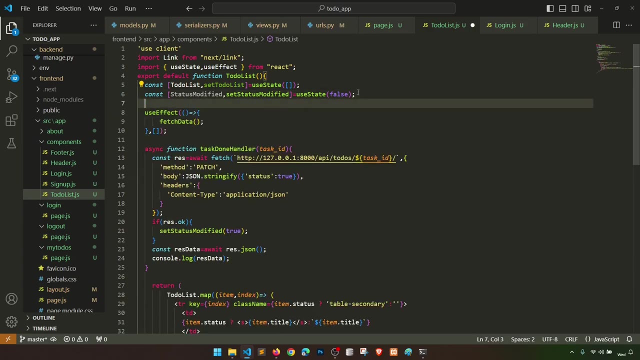 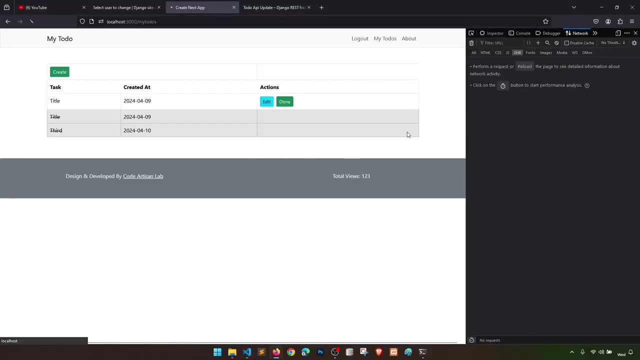 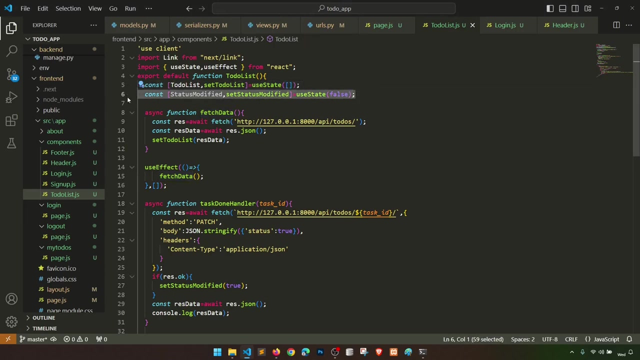 means it is not fetching this function, okay. so what we can do here if I say copy this, right. if I say copy this and paste it here, okay, then what we can do with it, okay, and in the use effect we are doing this, so no need for this status modified. 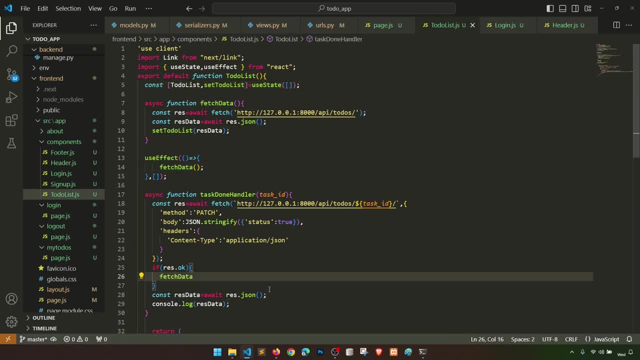 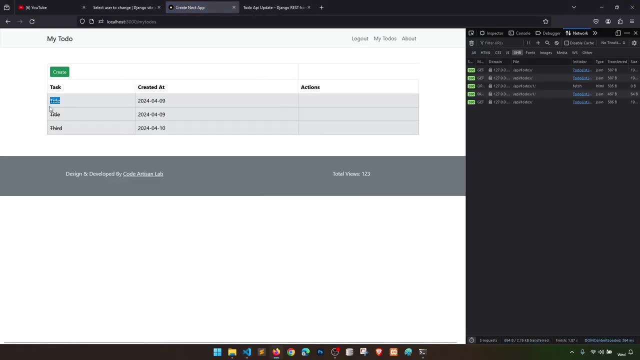 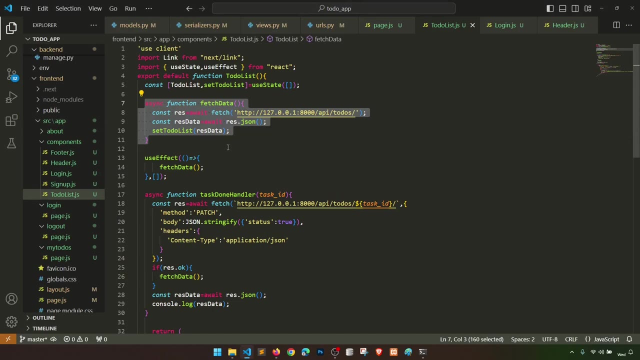 but to turn okay, fetch data. if response is okay, then fetch data, right. so if I say done, you can see this. so if I say done, you can see this right. so it means are done is working. and this is the function that we can fear: fetching the data in the use effect it's running and if response is okay. 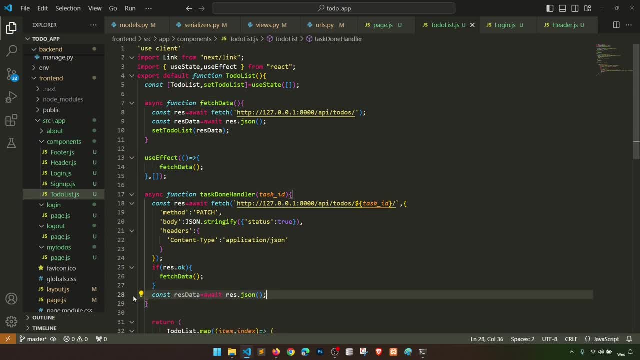 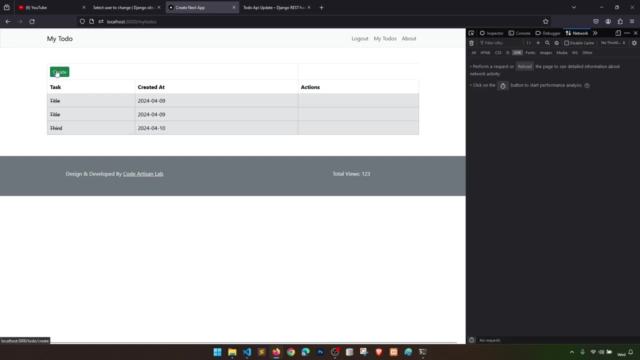 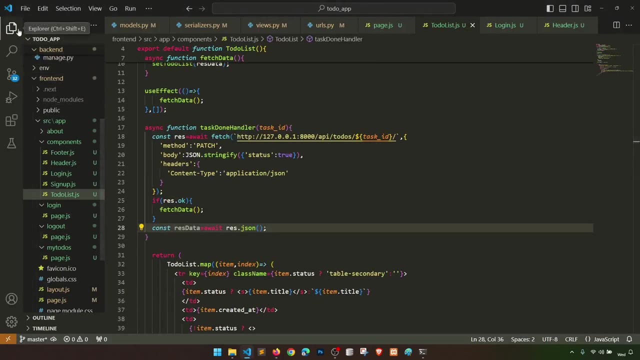 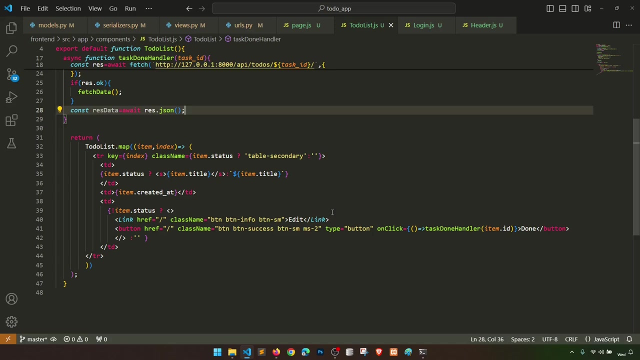 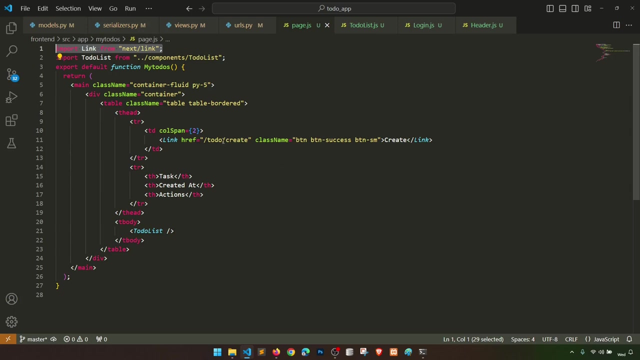 then it's also running right, so all data is done, correct, so now we can work on that. create. right, so let's work on the create or create. we need to create a one more page, or we can say one more component: right, so this is list. and when we click on this, okay, so this is page. so we are going to do this to do. 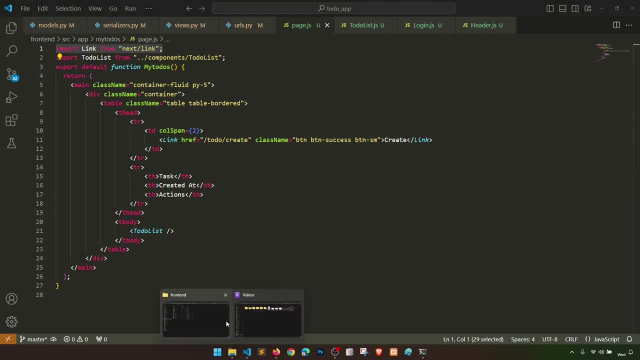 create right. so let's say, in the front end, in the source, in the, my todos. okay, so my todos. so I made of one page one, one, two, three, so this is three, so we have reached the opposite side. let's see, I made of one page one more forty five, sort ofría. 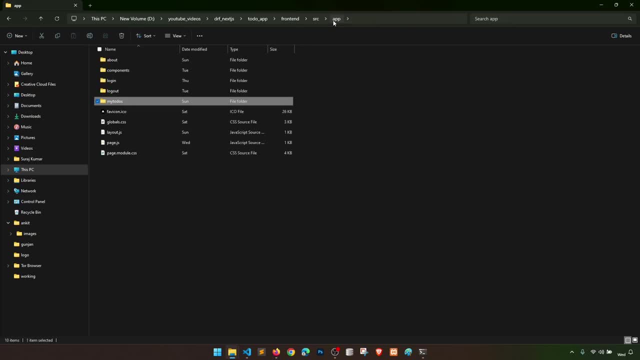 my todos, so my todos, and it is to Okay, so my todos actually saved first from this here. okay, if I Marla in the process like a search on various page, will någonting and let's add these together, okay, so I. Well, now it's. 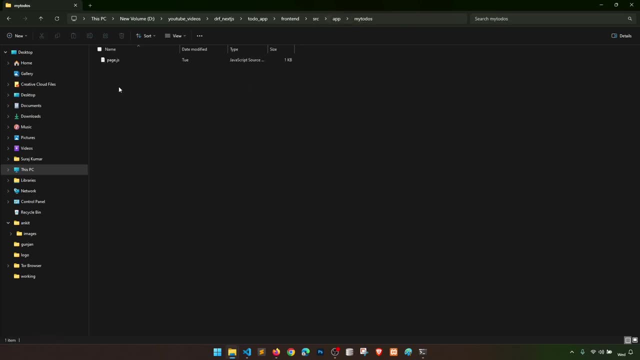 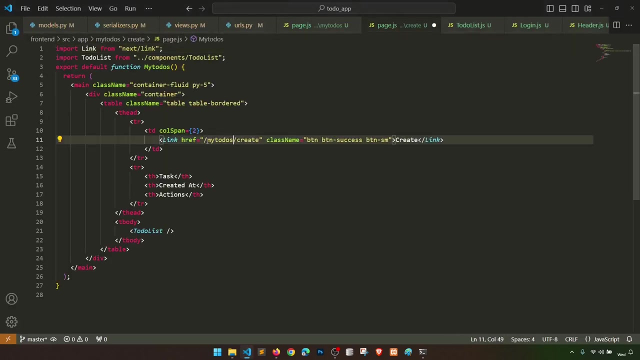 to right, but I wrote: see, yes, So here I'm going to add some more things to this. So a so in the my to do's, let's create, create, and in this, create will create a page, right, okay? so the link will be my to do's- create, right? so where is this so? 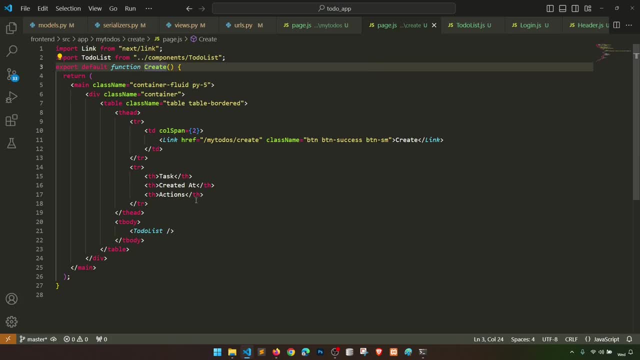 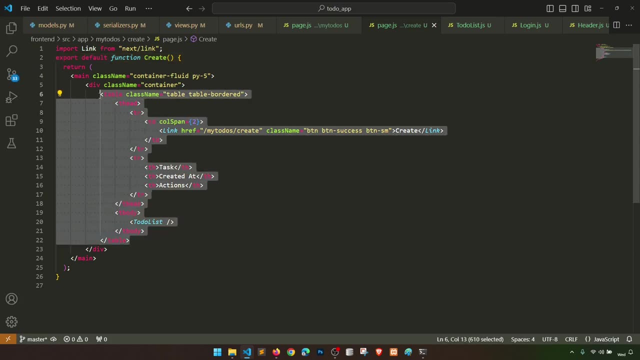 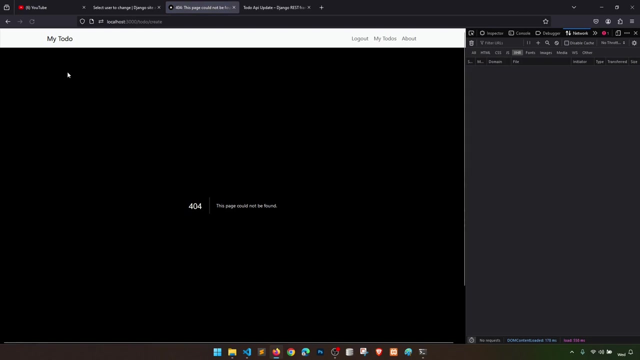 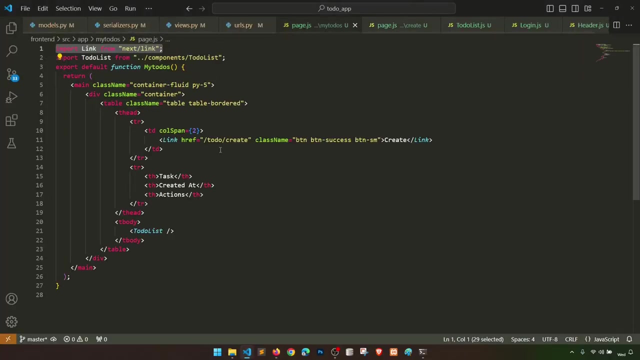 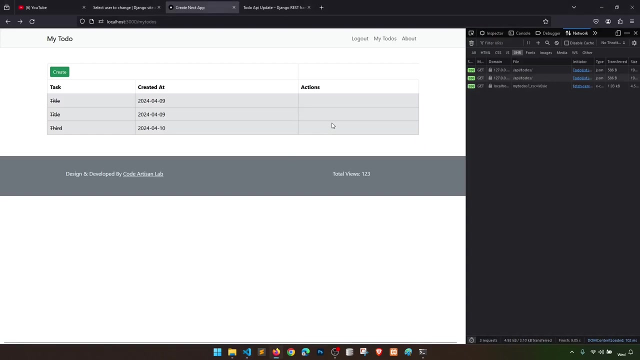 we'll say: create to-do list. no need for to-do list link is fine, let's remove this table, all right? and if I click on this, where is this? okay? so let's go to my to do. oh sorry, my to do's. is this okay? so create. when we click on this create, it should open my to do's dot. okay. 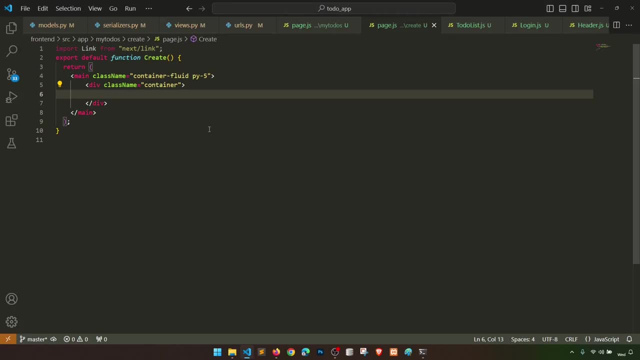 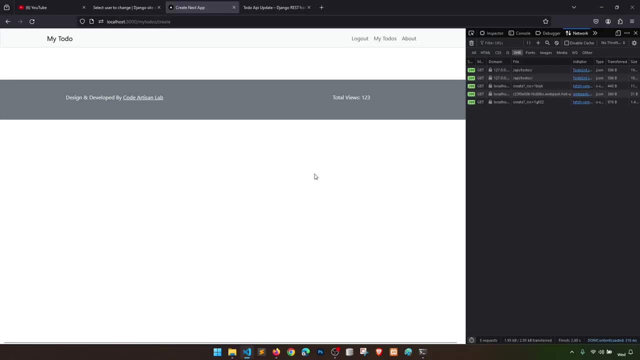 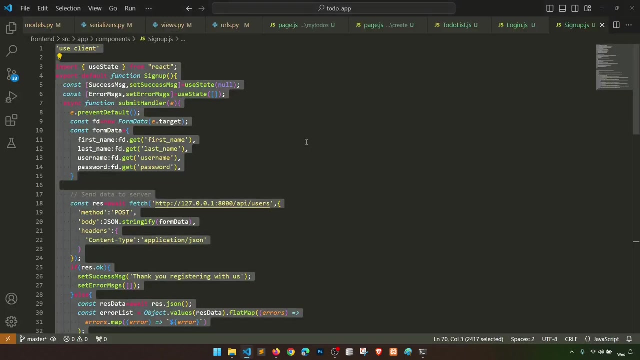 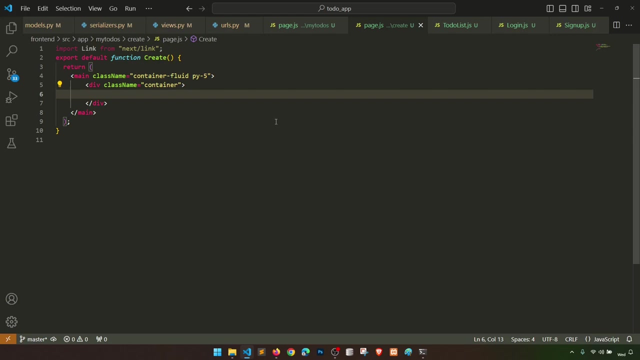 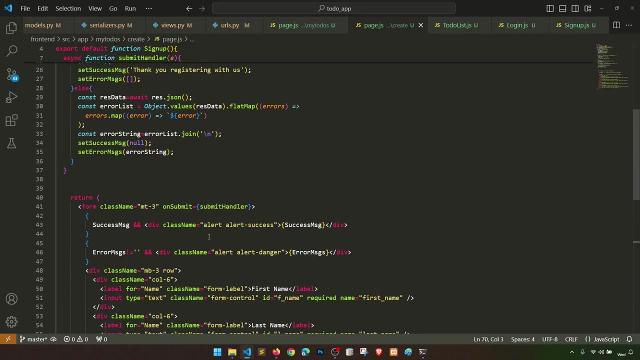 so this is opening now. so this is our page. I will go to signup page. right, I will go to signup page, then we'll see. okay, so this is our signup page. I will copy this. go to this is page create. right, so we can. let's take paste here. we need to do all the things. 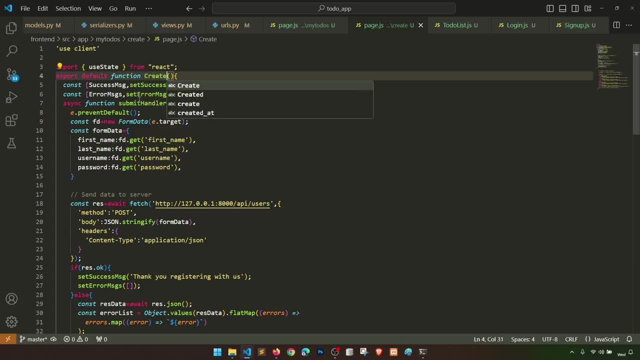 so let's say create okay, success message, error message, form data. so in the form data, when you only the title right and here we need to do to rules right, I will do two rules right and I will change text. so if I change text I need only one. error message. so I will change text here. right, and here we need to do two rules. right, and here we need to do two rules. okay, we can go to some투 Status and we can create a page, create text and paste on your. see the can I mostly also an. 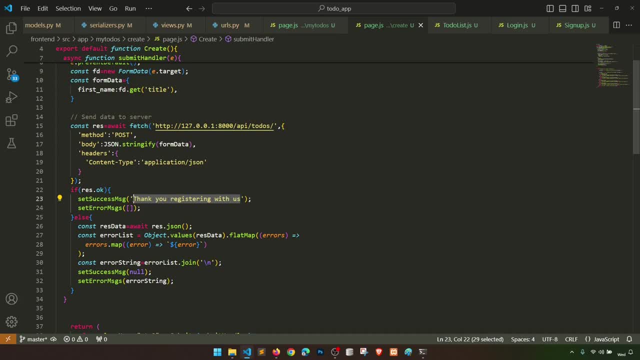 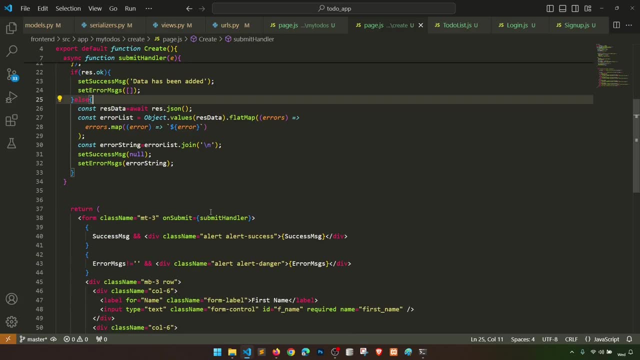 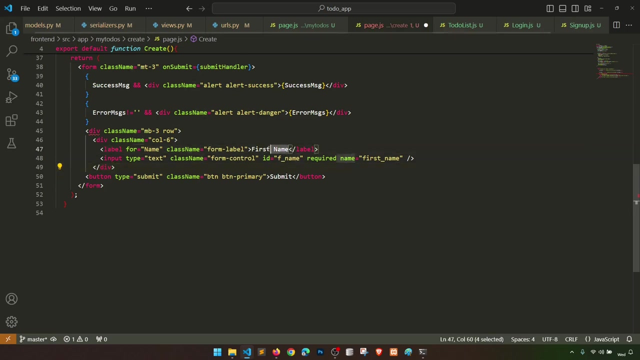 everything. think your data has been added. we'll say data has been added right and if any error, then we will show the error. let's remove all the things. we just need title, right. so title: a name will be ID will be title, name will be title and it's required field, and this row should be close after this. okay, and 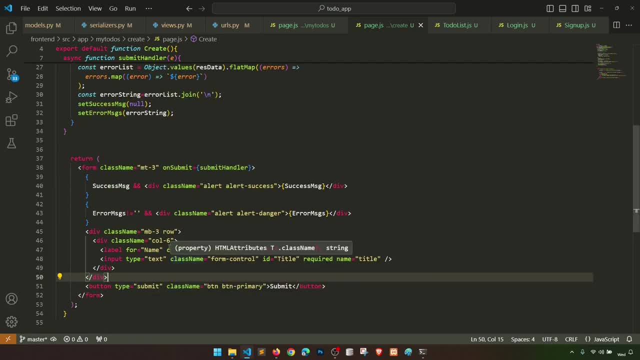 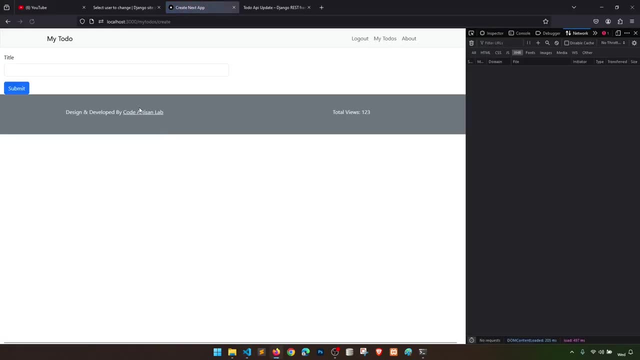 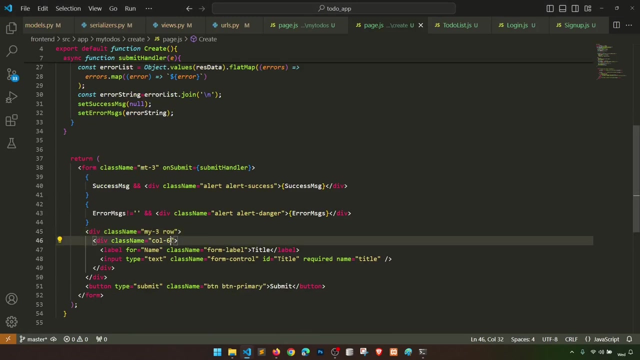 this is six. okay, let's see, this is showing first name, last name, but it should show only the title of it. so this is fine, you margin bottom, not margin only bottom, but it should show the margin top bottom, all right, so this is the. let's give them offset. okay, let's make it, let's put this: 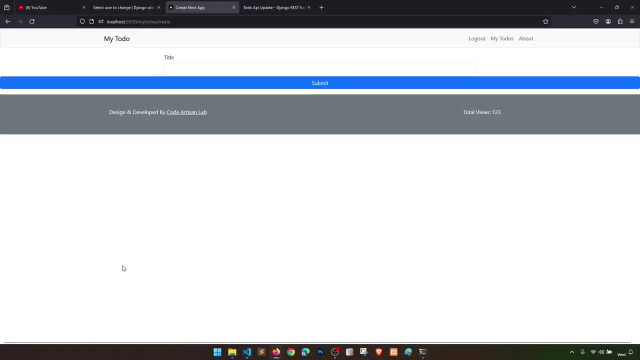 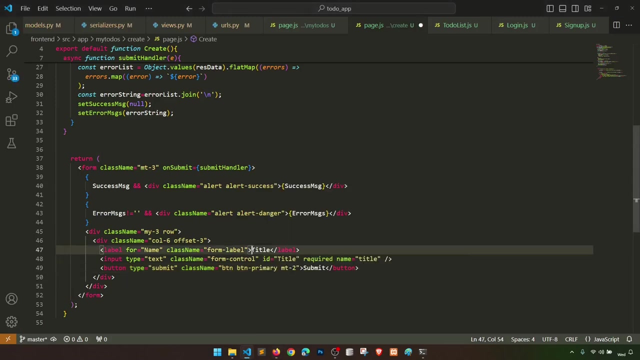 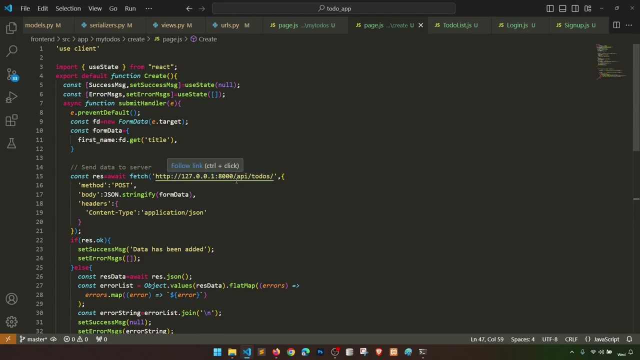 button into this column. what is this after this? okay, let's give some padding now. sorry, margin. so this is our title, right, and to do title, task title. you can see right, and when we click on the summit, it will. it should add the data and it should show the message or error. 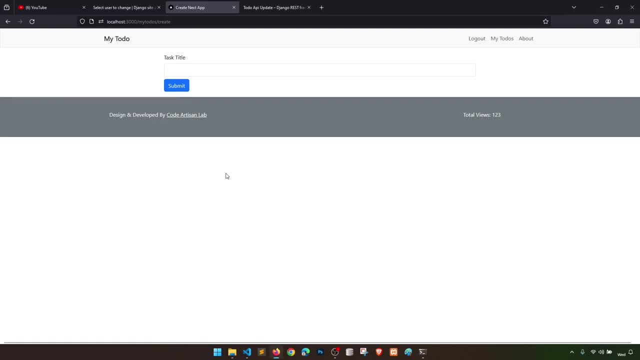 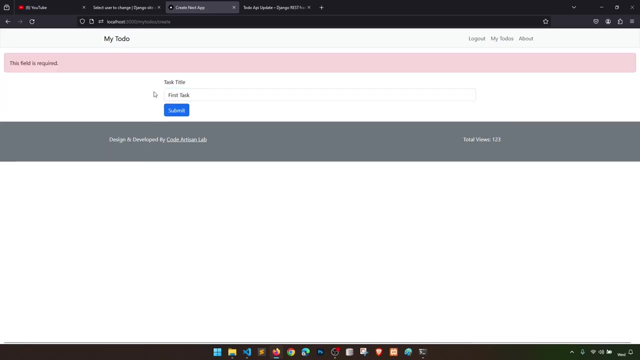 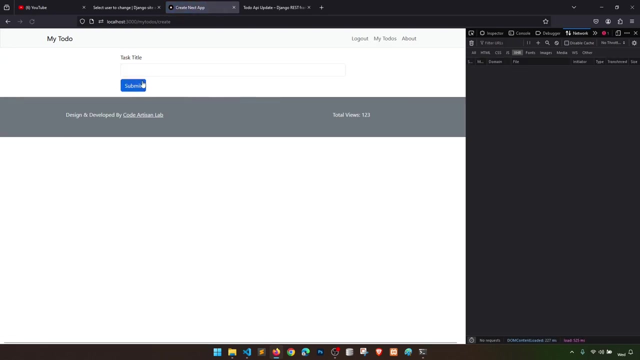 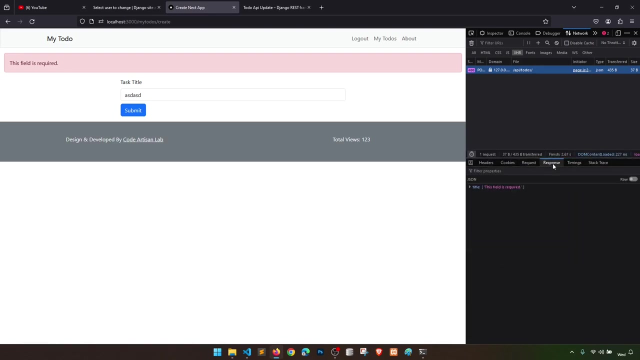 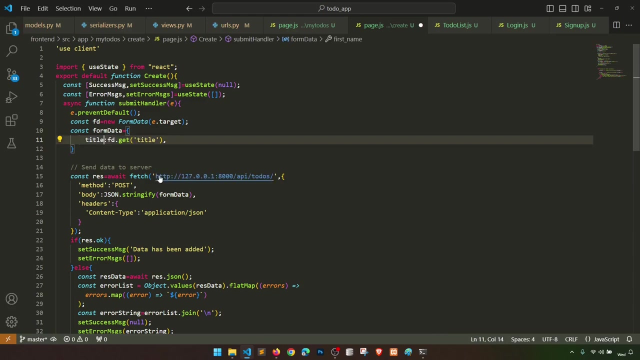 message, whatever we want, or we can redirect to to-do list, but let's add this. so we'll say: first task: submit the. the field is required, which field is required. let's go to here and let's submit this: which field is required? so let's say: response: title, name, title. oh, sorry, we should. we are sending this data. 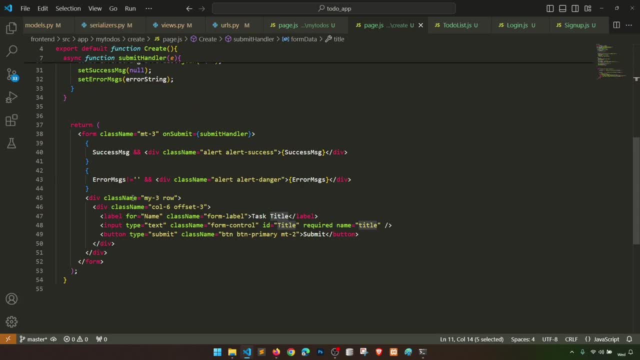 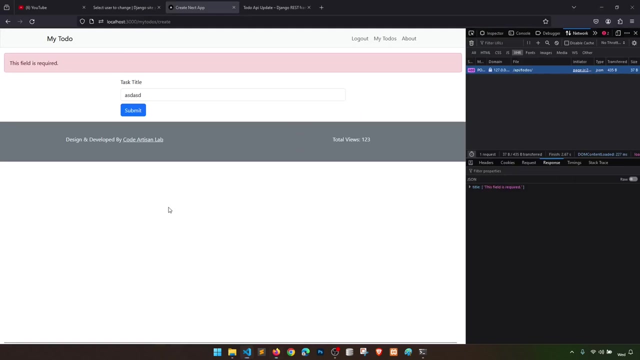 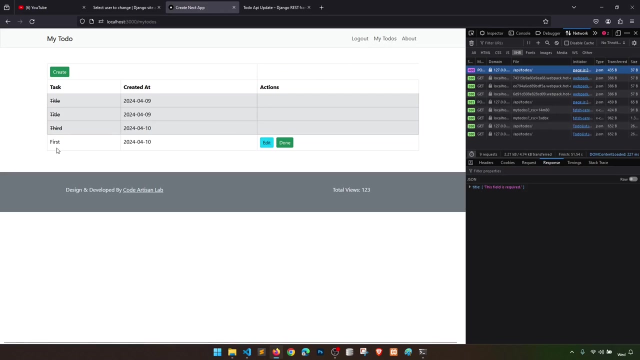 so it should be title okay, and for the messages it should become in the arts. it should come in this, all right, so this field is required. now let's say first and then let's say submit. data has been edited. if I go to my to-do list, so first is showing now correct. so if I 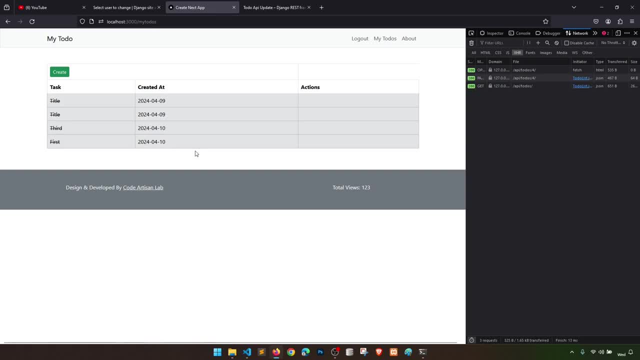 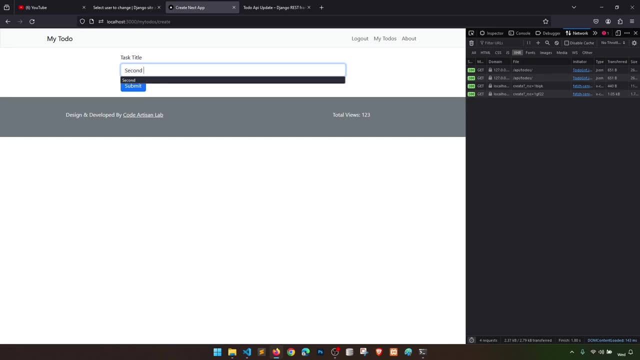 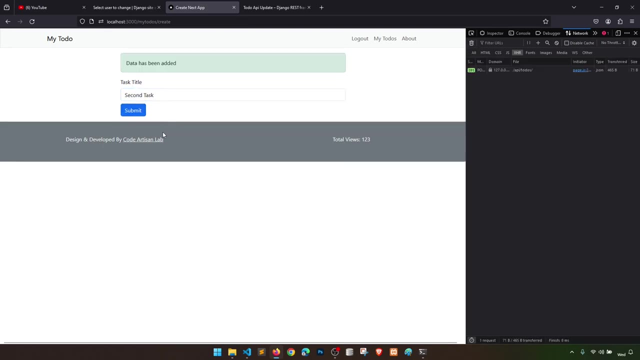 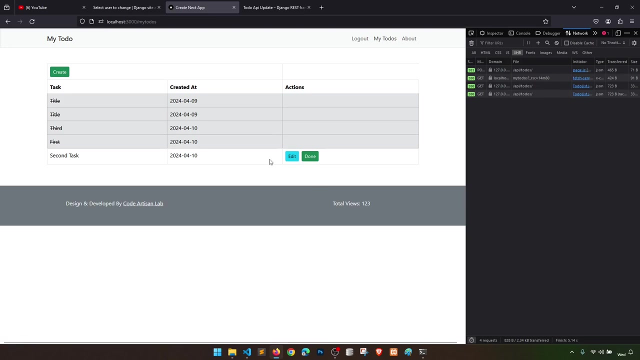 click here- done, then data has been done. right now we need to do one more thing: create a, let's say, second task, right, and then we submit data has been added and we go to my to-do list. we need to work on the edit- right, so done is working. create is. 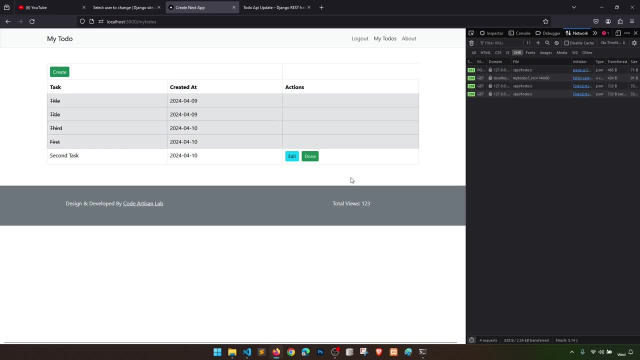 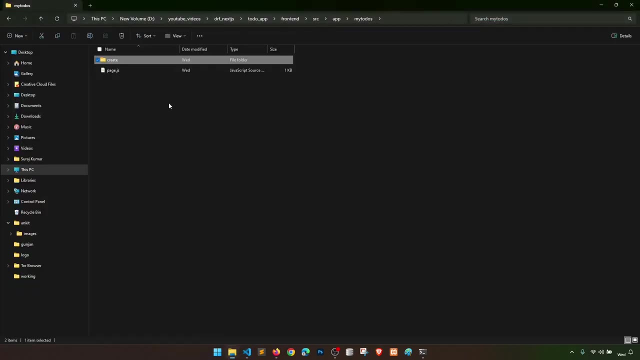 working. we need to work on the edit. let's work on the edit, then we will see how we can perform this. total views right, okay, so now we need to work on the edit. so what we will do, we need to do here- we will create one more. one more field will say: 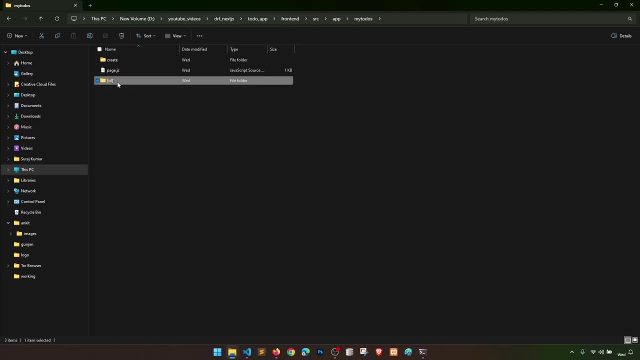 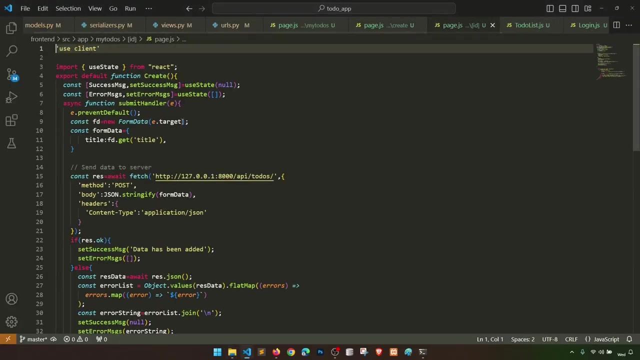 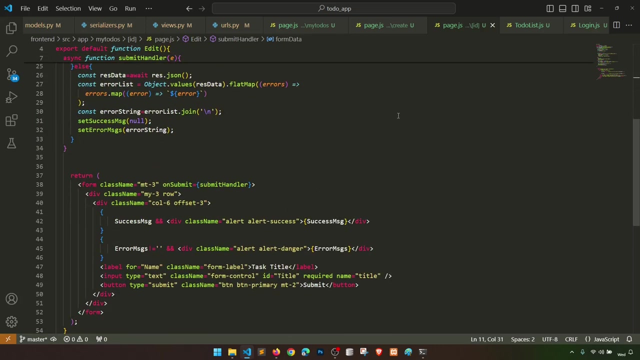 ID right and in this this is my to-do list, this is create and let's copy this one, let's copy this page, let's paste in this ID right and let's open this and we will see what we need to do. okay, so first of all, let's see: is this fetching? 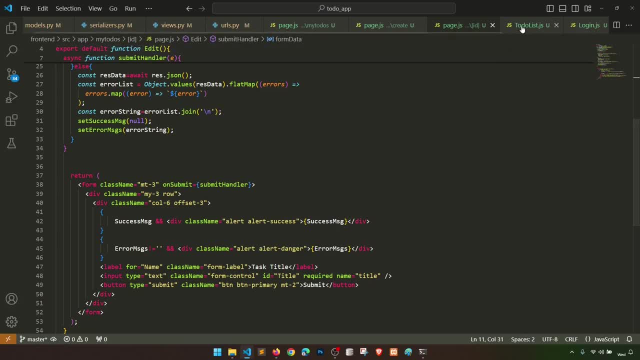 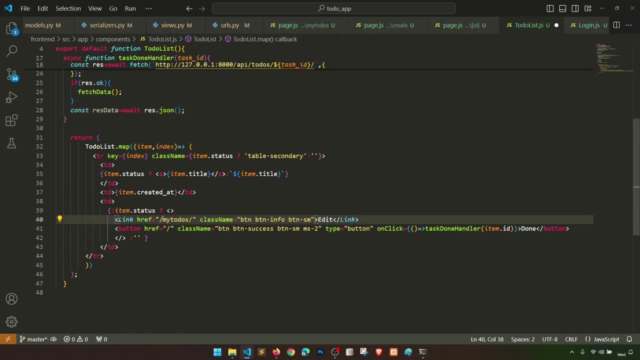 the proper data or not. so in the to-do list we have edit. so what, we will do. my to-dos slash. my to do's slash- ok, let's do this in a proper way. my to do's slash item dot correct and this will be end with slash. 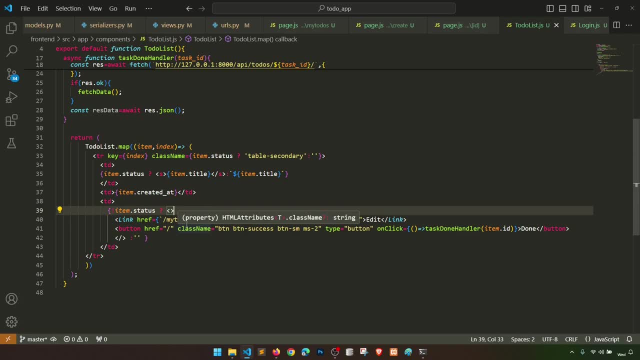 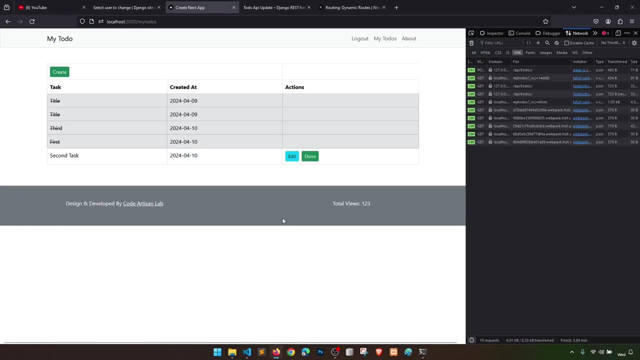 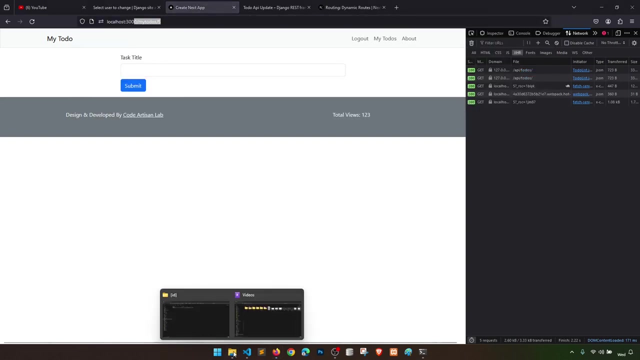 right. so when we click on this it will open that page right. so let's go here, click here, so it is opening this page. you can see here. so we are using the pages route, so my to do's, and then the dynamic thing, and then we have a page right. 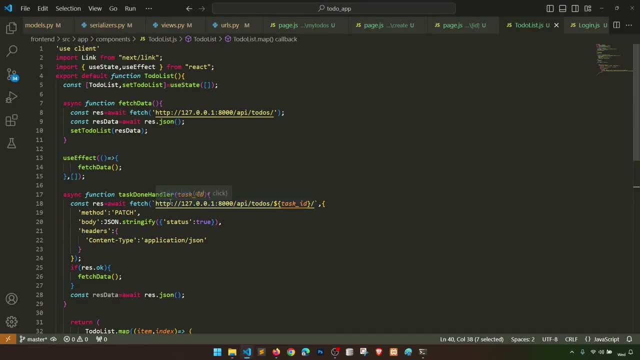 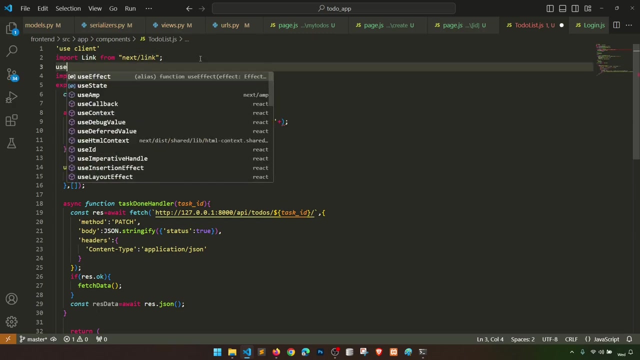 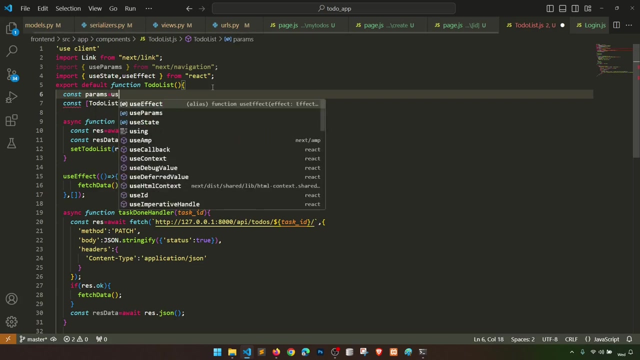 so first of all we need to fetch this data right. so for fetching the data we need to pass here the id right. so we will use what we will use here. use params right from the navigation right and here constant params equal to use params correct and we will see. 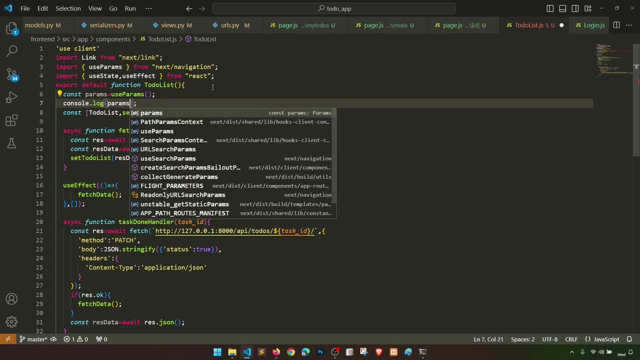 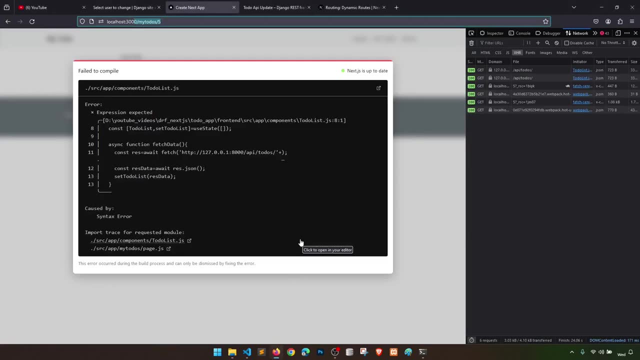 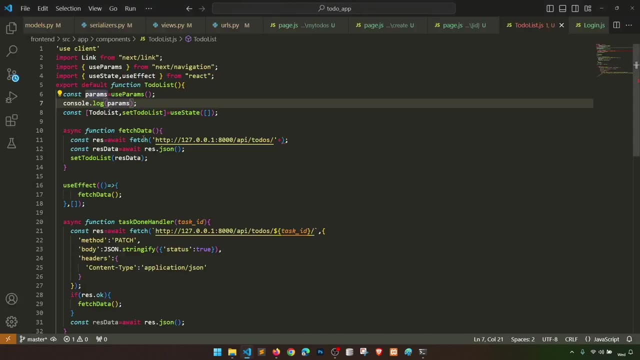 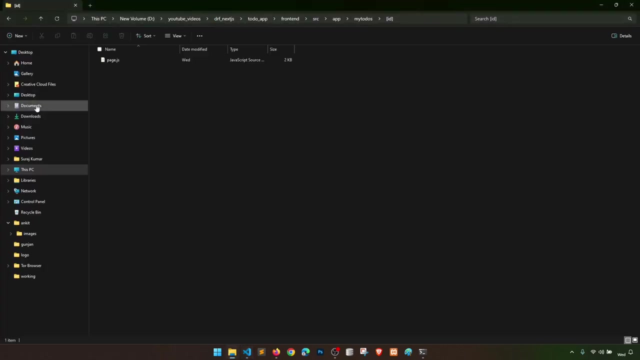 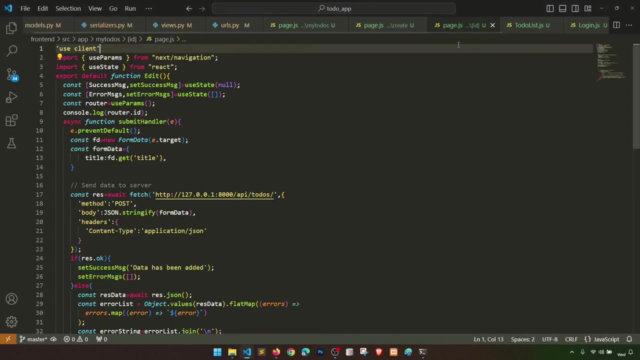 what parameters we have correct. so if I go here, ok, so let's go to console. ok, it's saying syntax error. so where is the syntax error? ok, let's check it. all right. so we were doing the thing I was doing in the to-do list, but we need to do in the 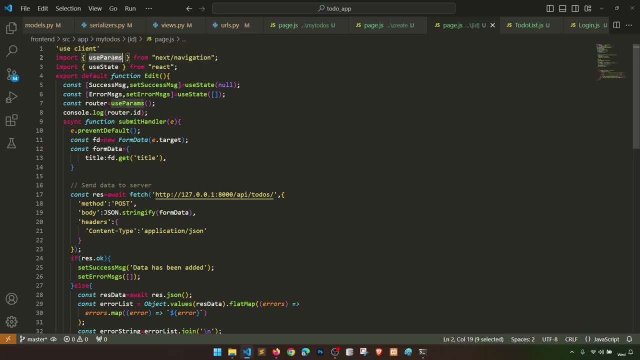 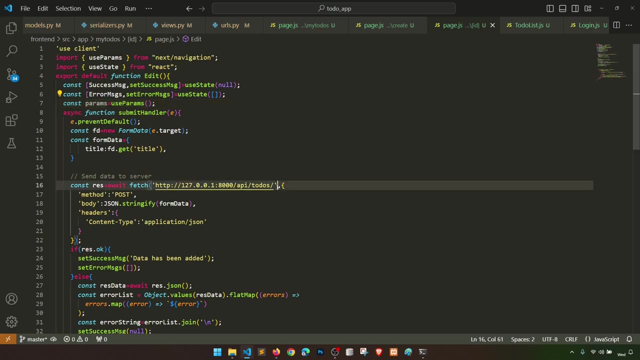 id page right. so here we have a use params- and this should be params- and from the params we can fetch the ID right and from the ID we can get the data. so this will be how to set data to it: from the parents we can effect the ID right and from the ID we can get the data. so this will be and we can get the data. so this will be. 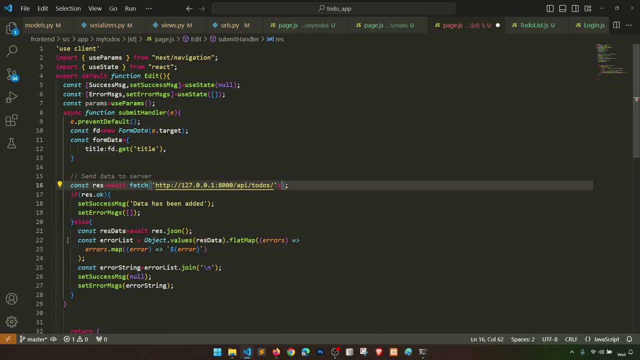 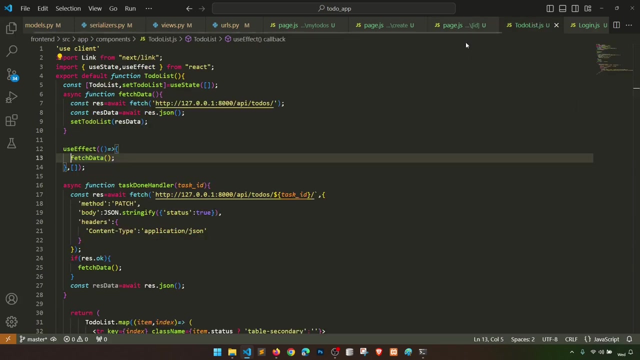 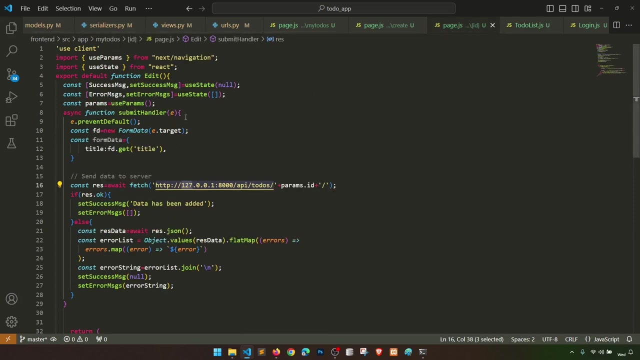 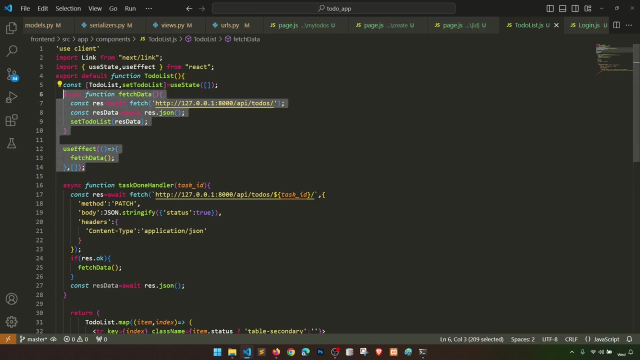 uh, we need to remove all this and this will be params dot id. right, so this will give us data, so we will fetch the data. let's go to to do list. uh, we'll use the use effect. where is this? this is submit handler, actually, but what we need, we need simple functions, so this is the function. 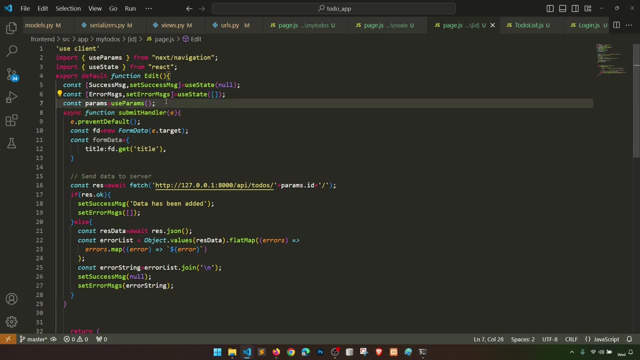 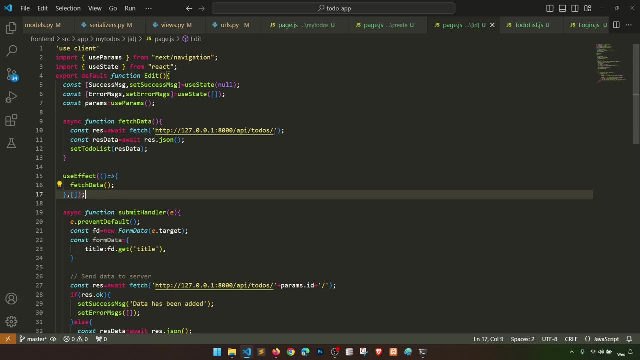 submit handler. we will do that later, but let's fetch here, let's paste this, so the fetch data will be here and this id will go here also. right, and this params: okay, so now we need to press the data set to do list. uh, actually, we just need one to do, so we'll copy this one, paste here. 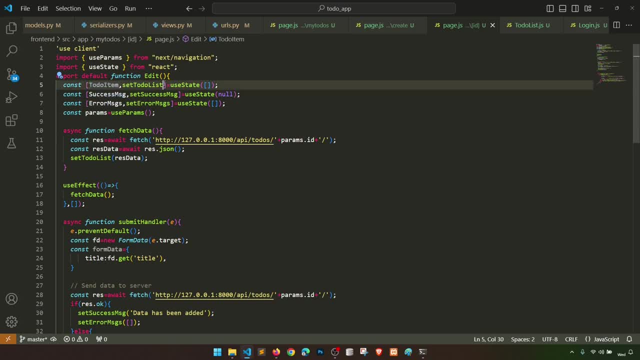 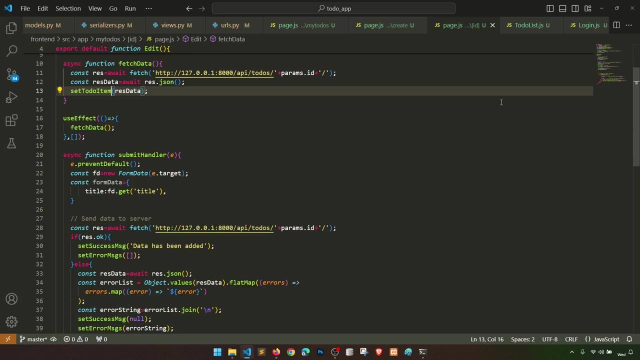 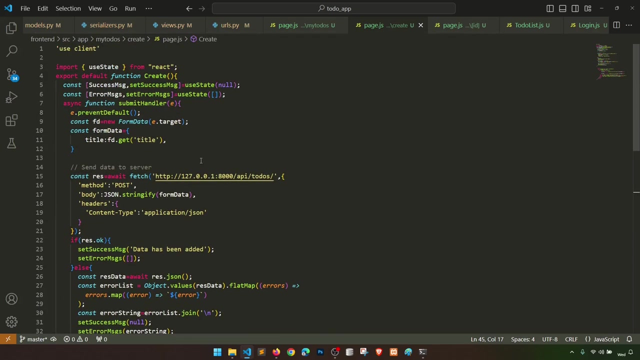 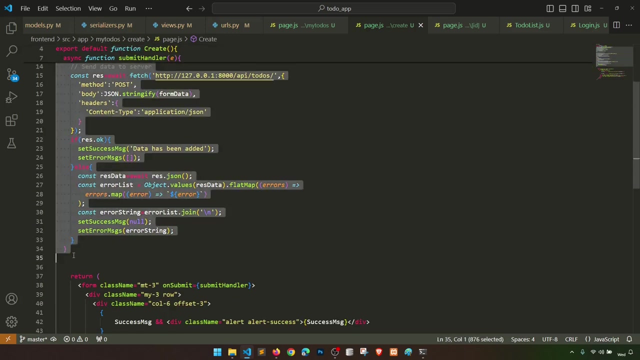 to do item. set to do item right, and here we will set to do item and fetch data right. so fetch data will be here and when we submit the data here, my to do here will create. so in the create we have a submit handler, so we'll copy it from here to here and the use effect will same. this is from here to here. 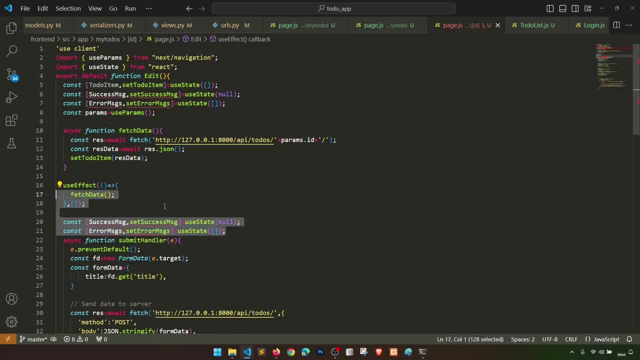 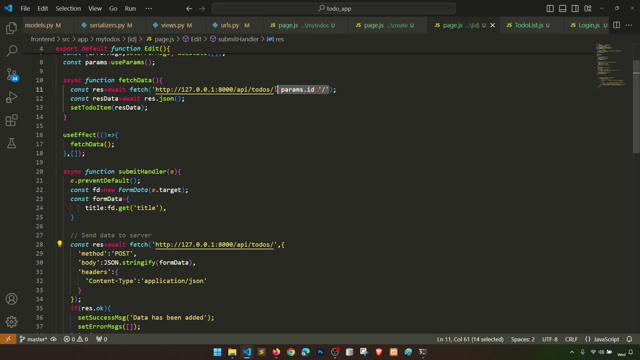 this is success message. we have, i think, already exist. so success message, error message: now, this will fetch the data. this will run the function when we load the page. this will fetch the data. but we only need specific data, so we only need to update specific data. so we'll not post, we will use the put method because we are sending okay patch, sorry when you. 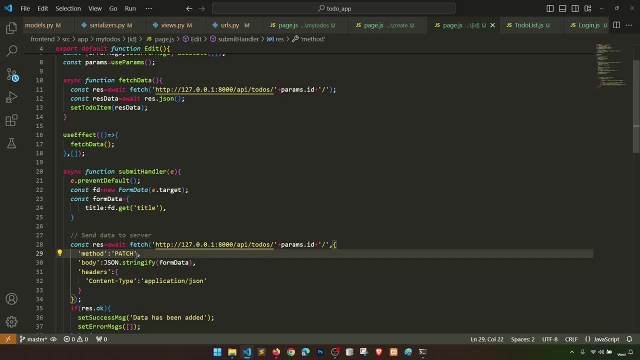 are sending any single uh field, then you can send patch. or you can send any single field, then you can send patch method. or if you are sending all the data, then you can set put method right in the status. we are sending put uh, sorry, patch, and in this we are also sending patch right. 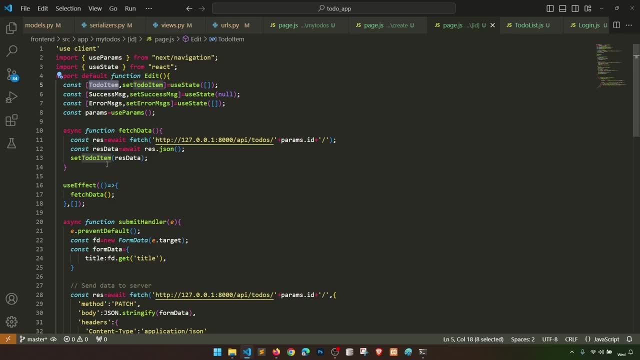 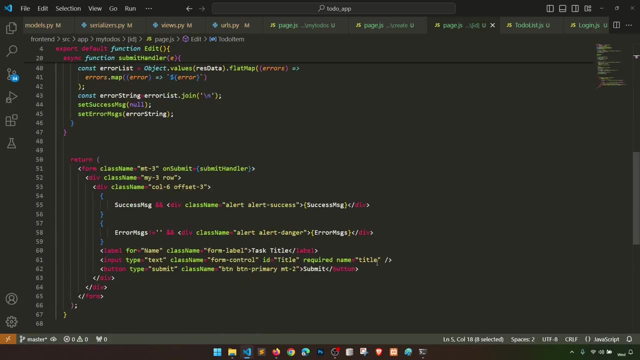 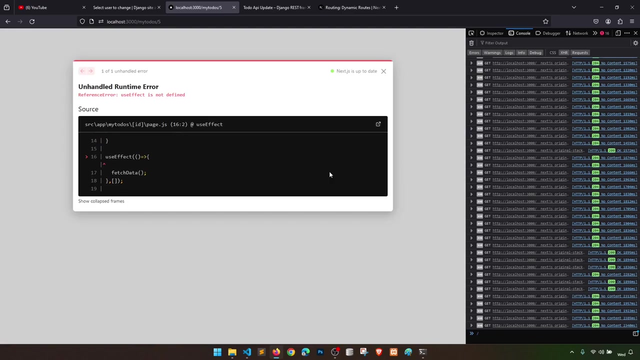 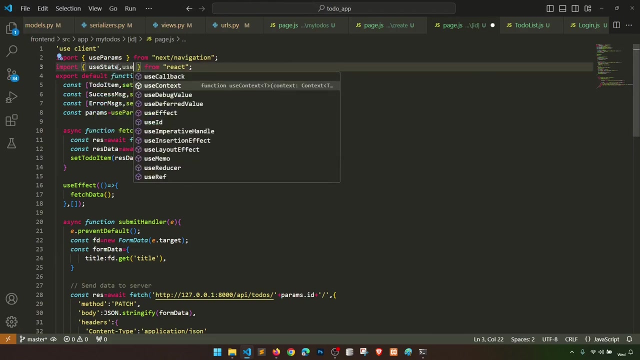 so we have a to-do item here and we are setting this to do item when we are fetching the data and what else. so let's say: value equal to to do. I don't dot tight right. so let's see, use effect is not defined. okay, great use. 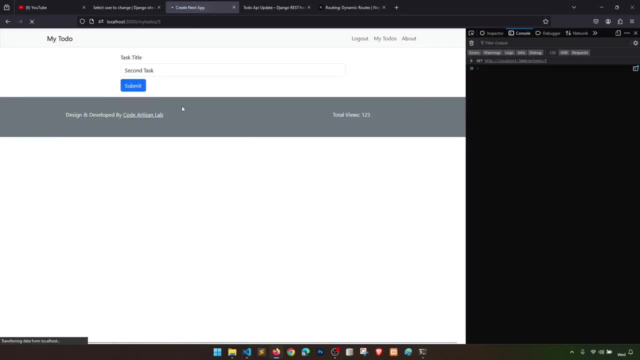 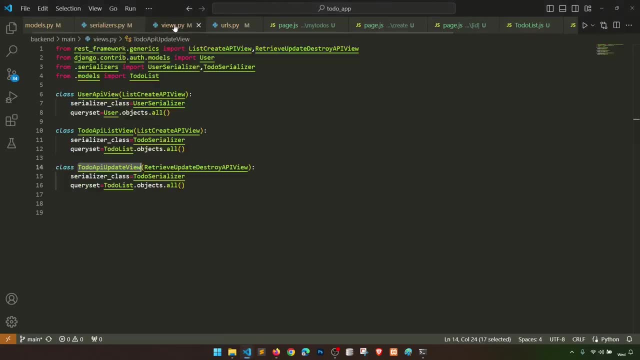 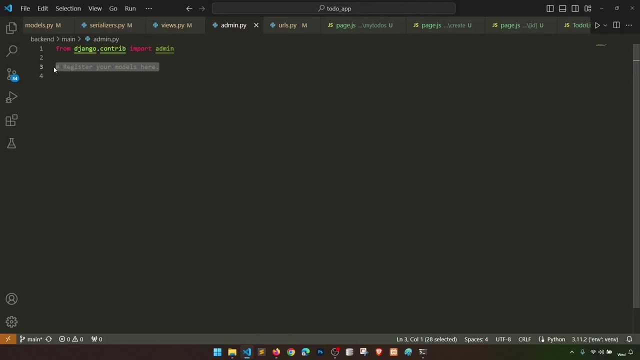 now it's defined right. so this is saying second task and in the model- we didn't edit this- let's add in the model also. so in the admin let's say admin dot site, dot register from main dot models, import and import to the list. right, and it's to the list, right, and let's see now. so here: 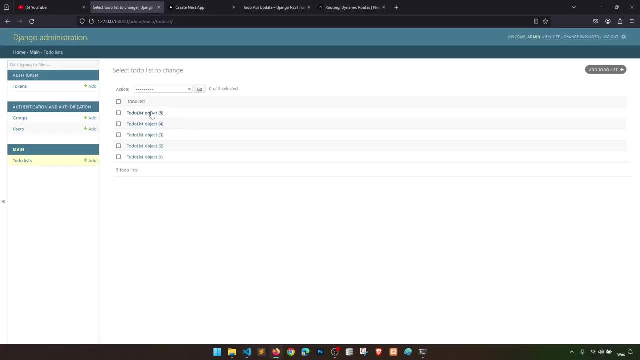 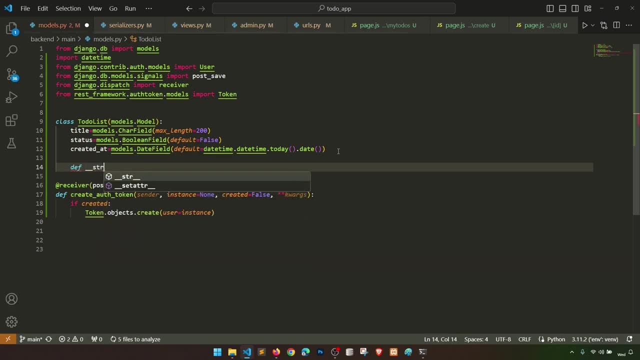 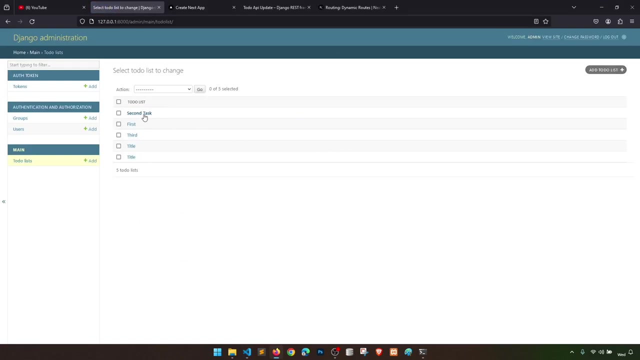 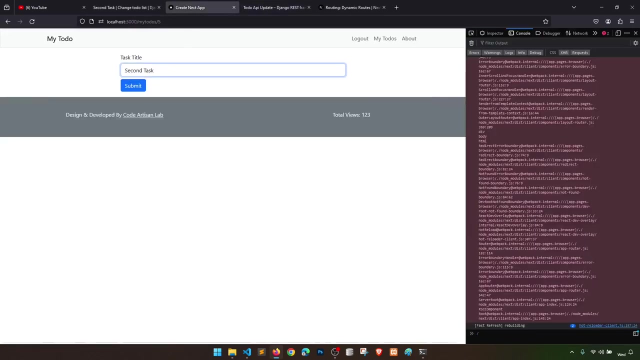 we have a to-do list and all the data. this data is doing object. so let's do one more thing here. let's define the string return title. okay, okay, okay, okay, okay, okay, okay. self-protected, okay. so this is second task. right now, let's update this task. we'll say: 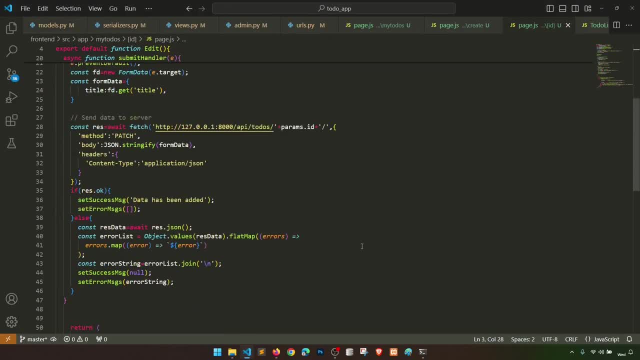 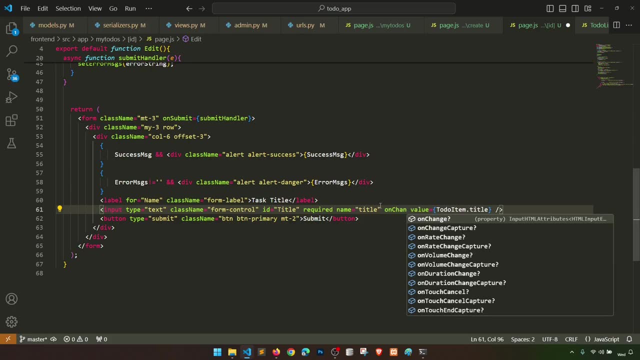 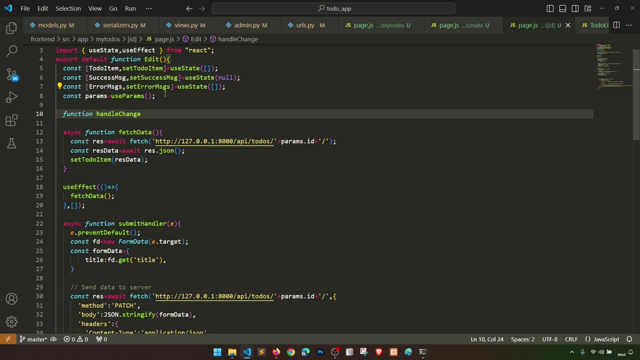 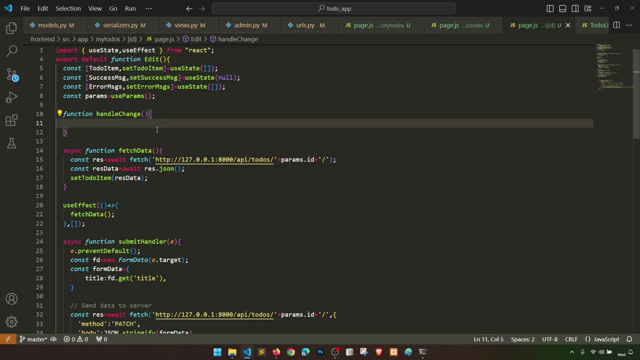 update it. oh, one more thing. okay, so from here we'll say: on change, on change, change right. and uh, we'll create a function here, function handle change, okay. and then we will say: uh, e, so what, we will do that to do item title. by default it should be: 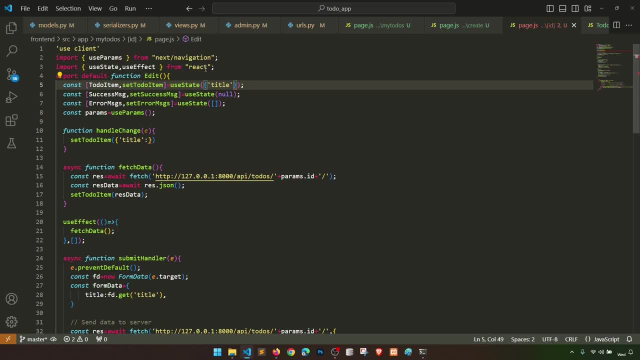 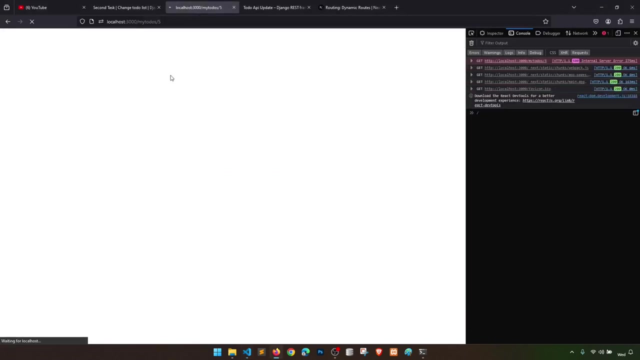 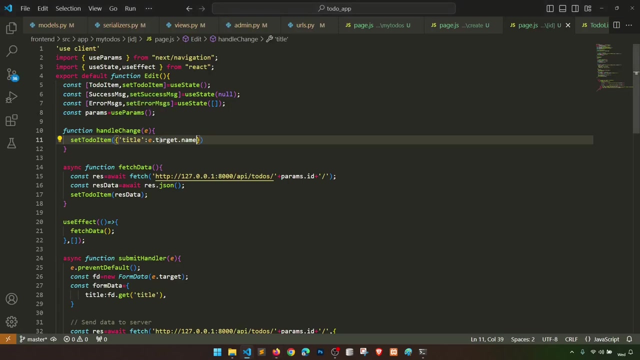 object. so by default, title will be all right. so let's create this like this. so by default, set to do item title will be e, dot, target dot name, right, so okay, uh, to do item is not defined. where is that? to do item is not defined? why this is not defined? 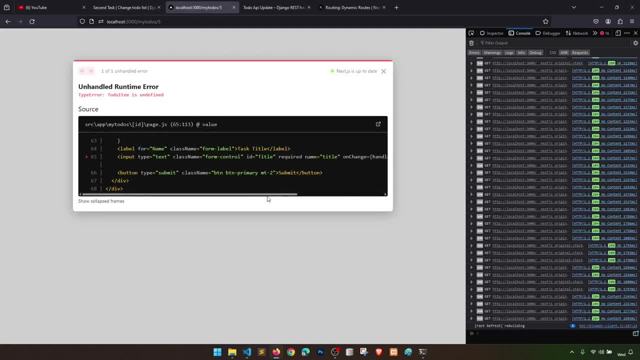 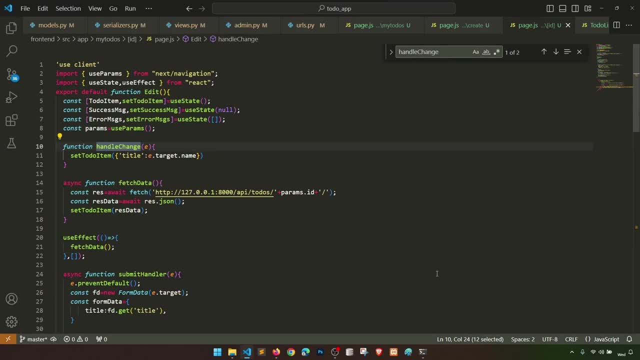 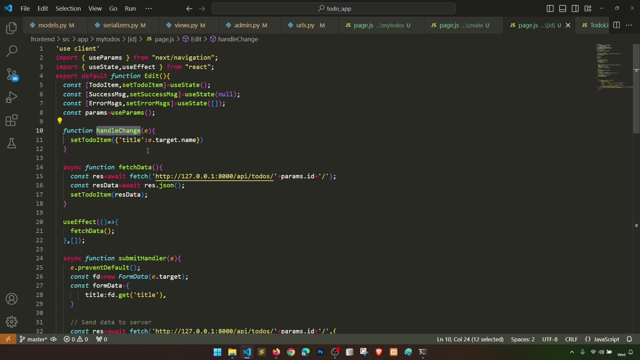 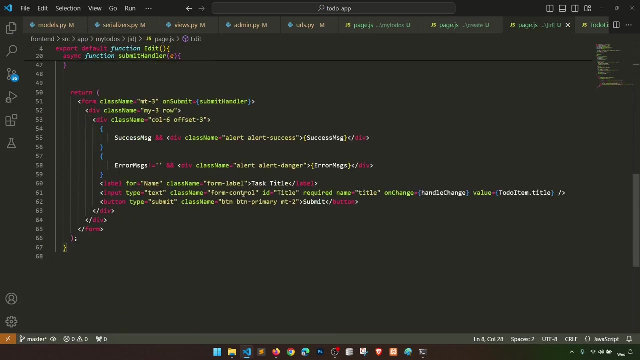 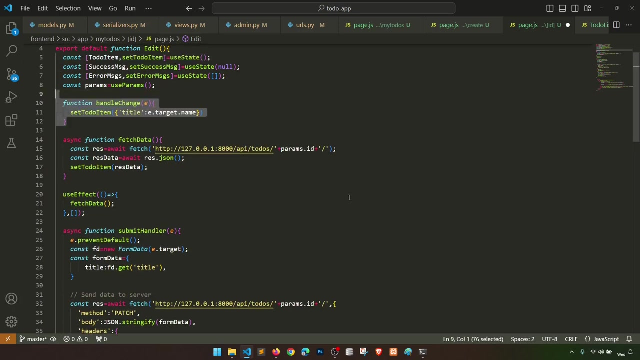 to do item handle change and this is uh change handler. this function is also working. why this is not working? this function? patch data change handler, submit the form actually. so what we need to do here? so we need to use the ending here, um, to do item handle change. let's see this. 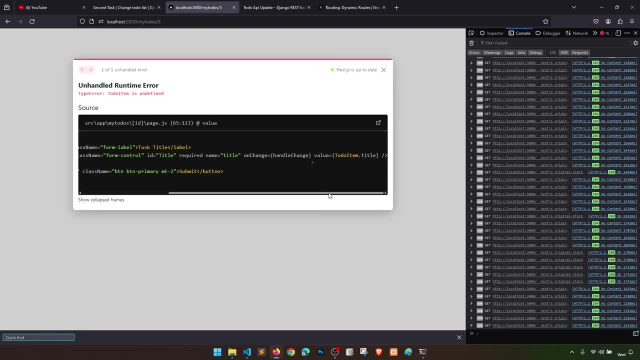 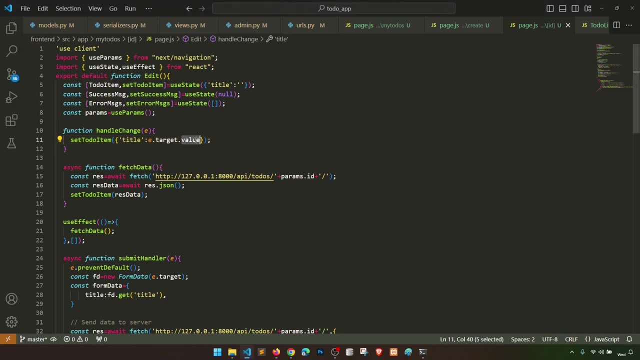 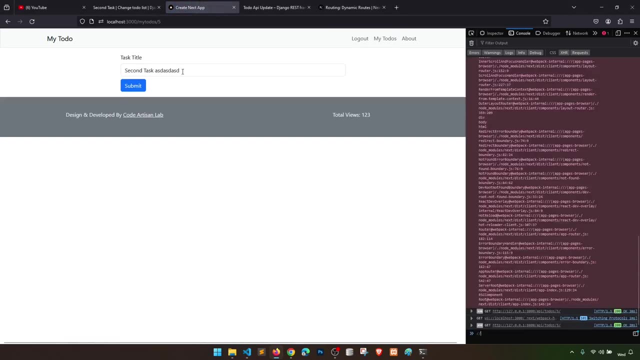 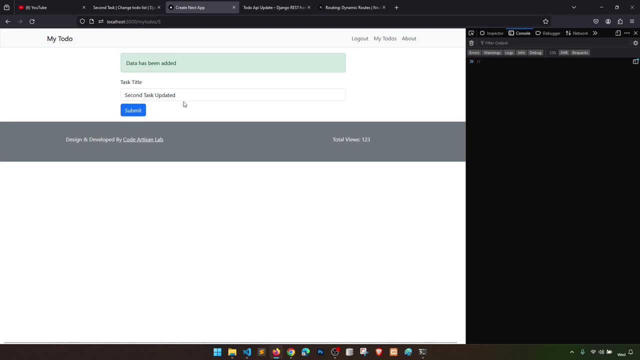 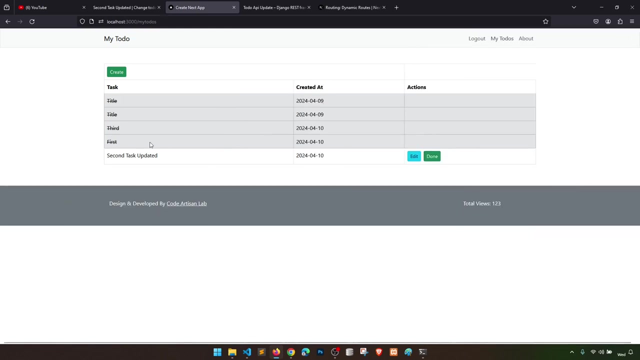 sorry. okay, so we were doing one thing that i forgot to mention. here we are doing the name. actually, this should be the value always coming the title. right now we'll say updated, submit. okay. so if I see here task updated right in my to do and here you can see, so I think everything is. 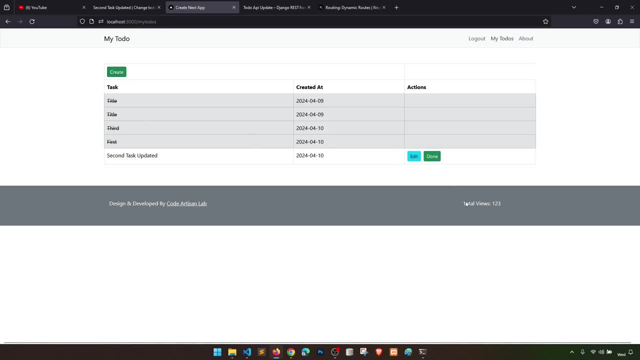 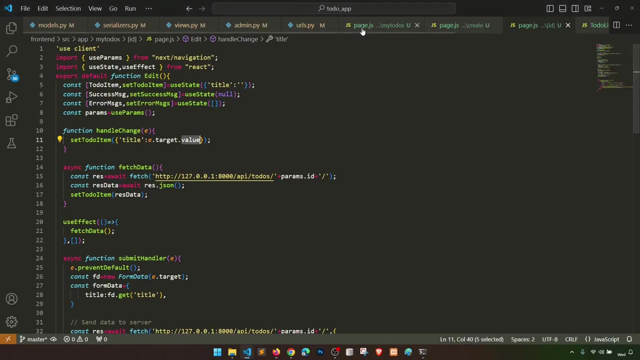 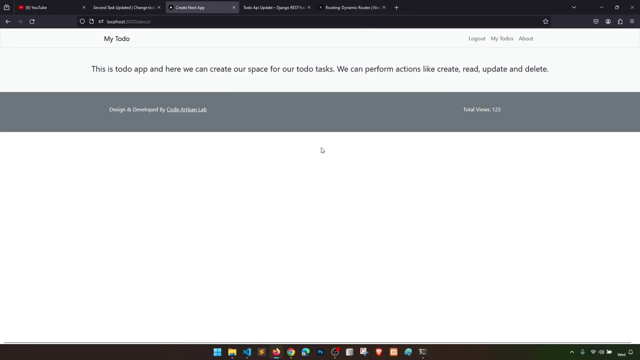 working. create is working and it is working. done is working. now we need to increase this views whenever we load the page. okay, and in the about you can see here the data. so if you want to change the data, you can go to the about page. so my main motive is to create this small app to do app that we can learn the. 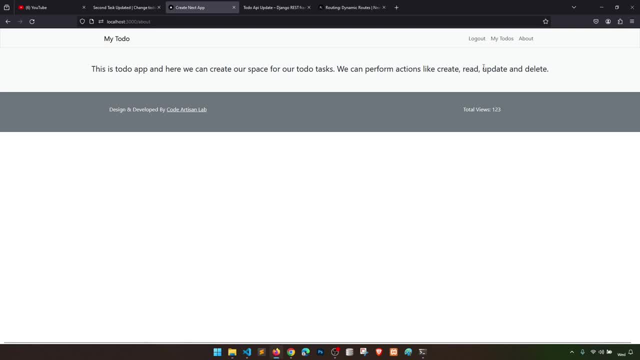 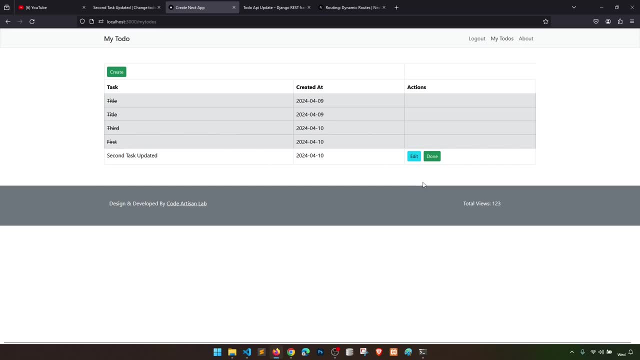 authentication. we can learn the APA working. we can learn how we can do crud. we can learn how we can interact with the. you can learn how we can interact with the events in the next years. right, we will create a lot of more projects in future with the next years and Django. right, maybe on more technologies like Laravel. 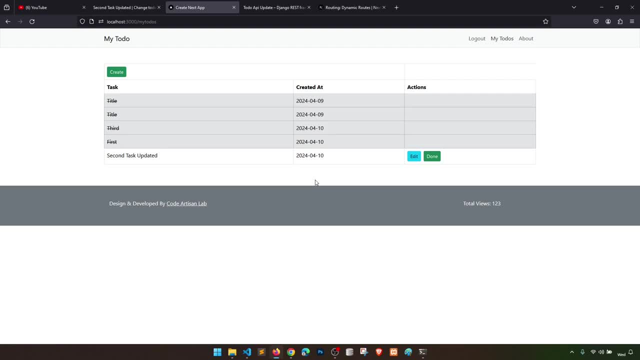 and other things, right? please comment your technology related views. that which technology should we use? right? so let's do this: total views, and then we will upload this project to get our posts posted. so if you want us to click on this, you can do that, and little bit. 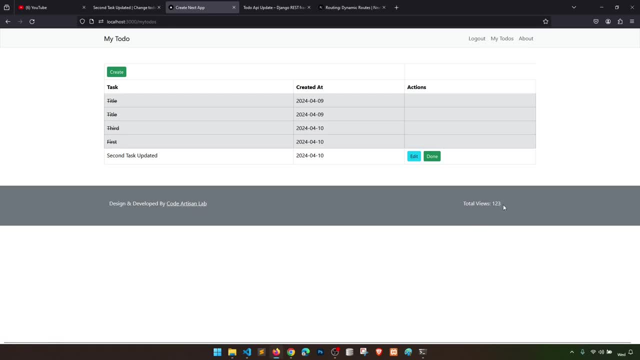 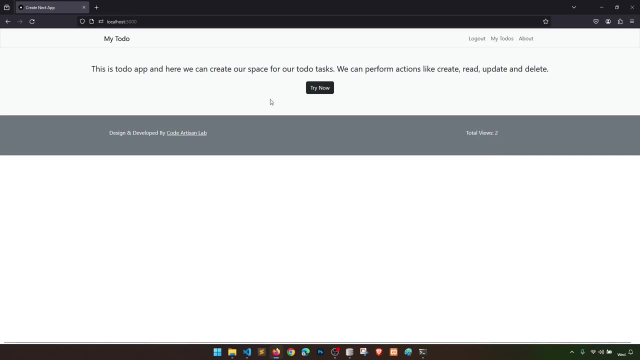 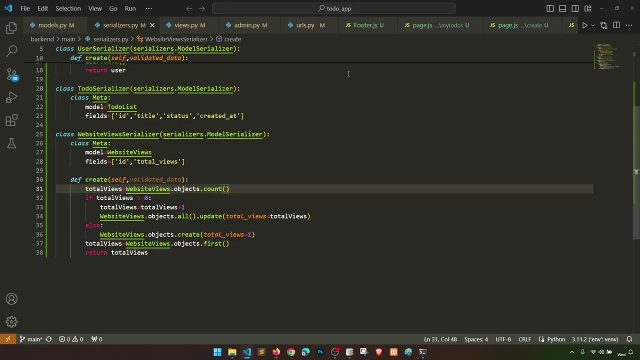 notifications. if you want, we can up so you can check, you can download, you can learn. ok, so this project is free of cost of us, right? so let's do this to interviews, okay, so we need to get that total views or update the total views whenever we load the photo right or whenever we load the page. 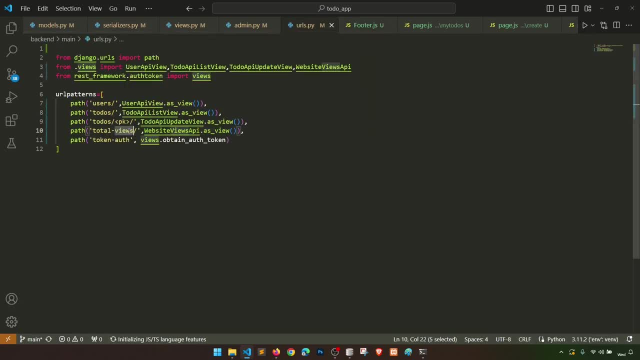 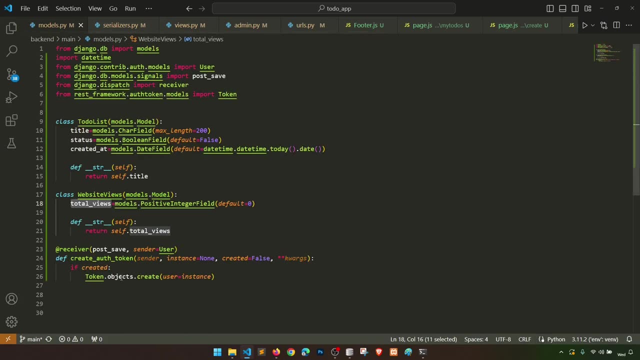 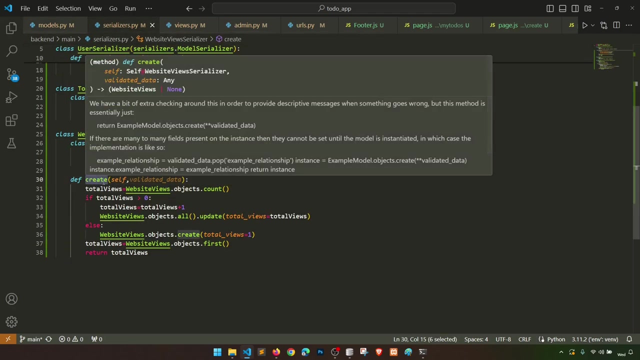 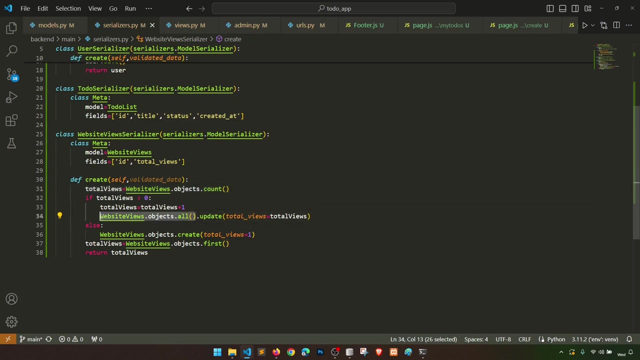 method. we are calling this url total views and i have created the correspondence serializer and model and views, right. so here you can see website views: total views. in the serializer. i am overriding the create method, so we are counting. if row greater than zero, then we will fetch the total counts, right, so we will say total views from the first row. so we'll say total views. 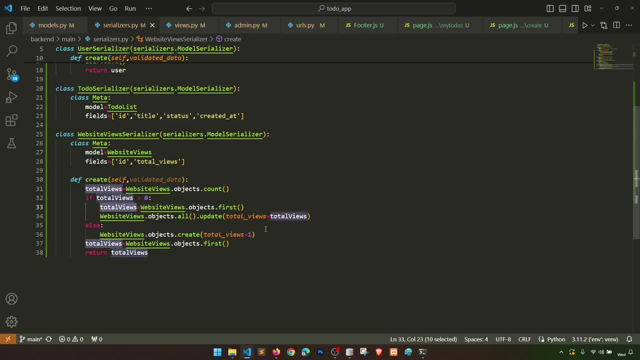 we can say: not total the total views dot. total views plus one, right. so from the first row we are. from this first row, we are counting the total views and updating right. if not, then we are creating the new room. great, so if you see here, you can see three. 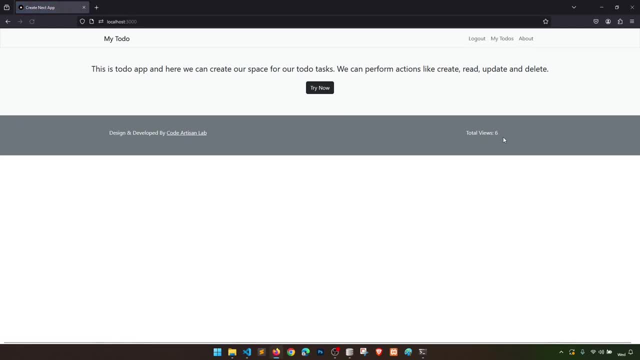 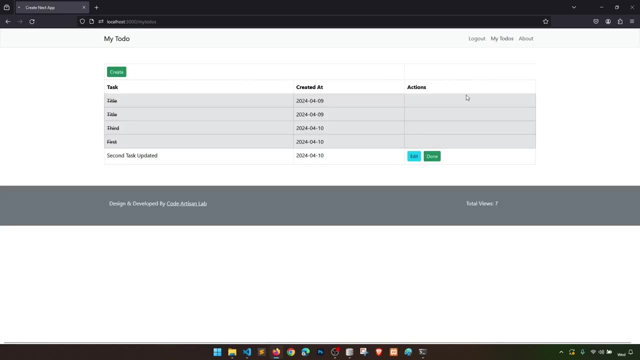 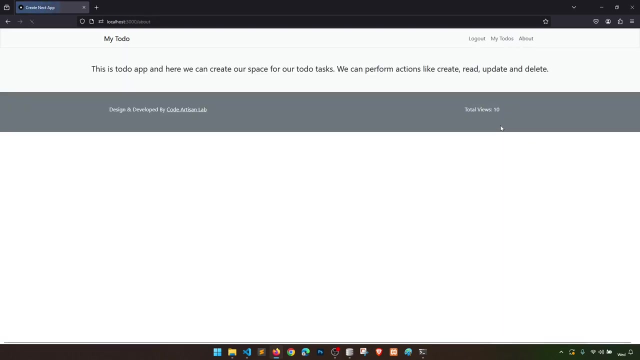 you can see uh, five. you can see six, seven, right, so click here my to do, right. so whenever we load this, then it will uh update the views. okay, so, but for the views, you need to refresh this page, right? so this is about okay. so this is in the footer and this is loading. this is 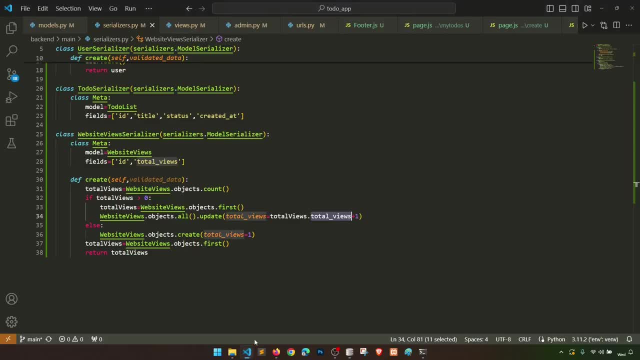 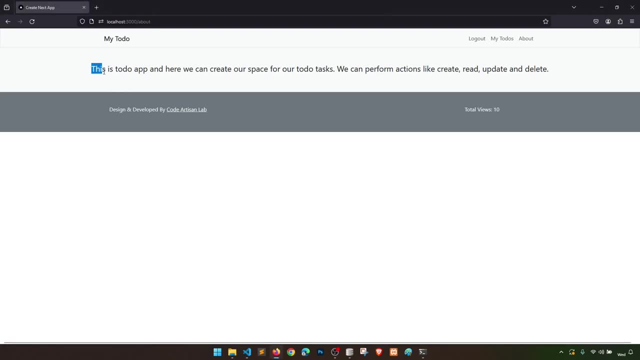 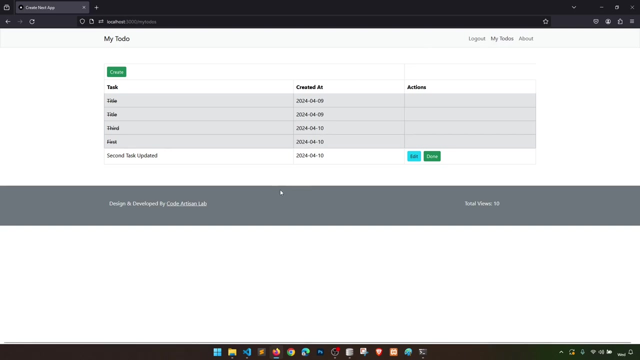 upgrading the views correct. so I think we have done with this app and I have. I will upload this app on the github and this is free of cost. and I will add that is that this link, a github link in the description right and in upcoming videos I will create, like I said in the my youtube community, that will create a 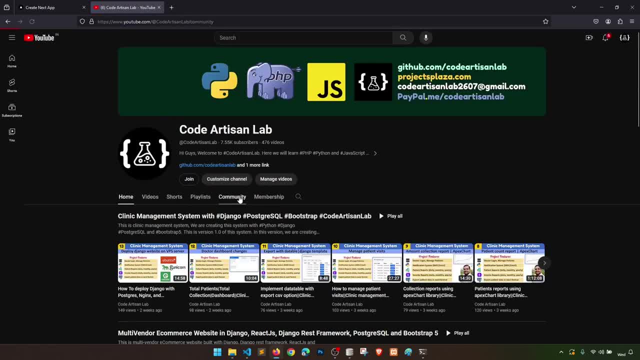 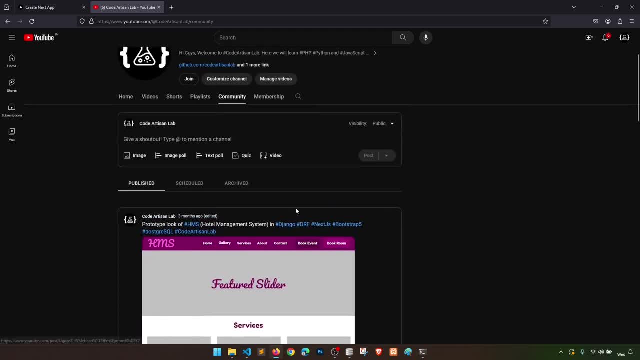 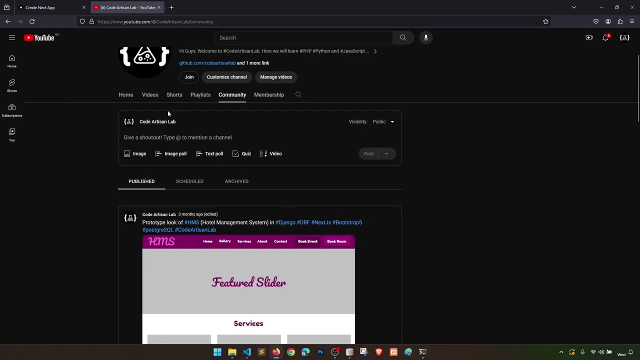 total management system that we will create, definitely. so I will create in the next. yes, right, this will be our theme. okay, so I know that this is late, but I will do whatever I have committed, okay, you? so please share, subscribe, like this channel and, if you need source code of 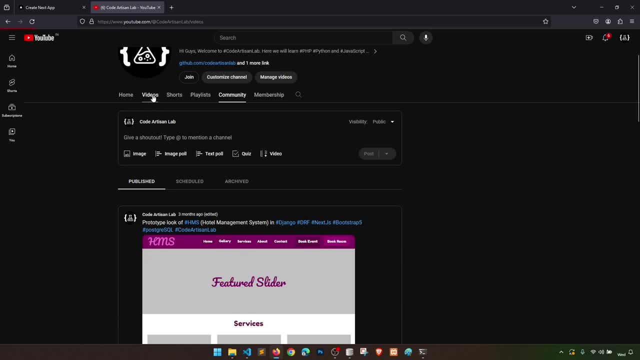 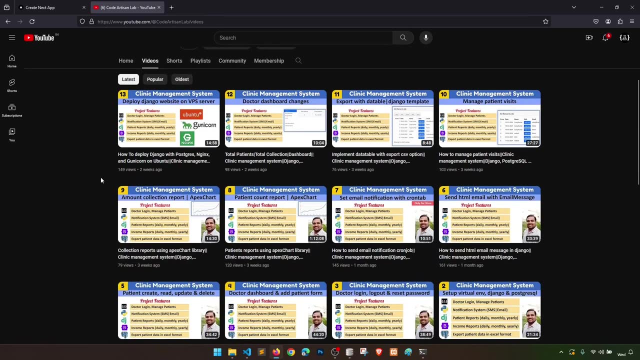 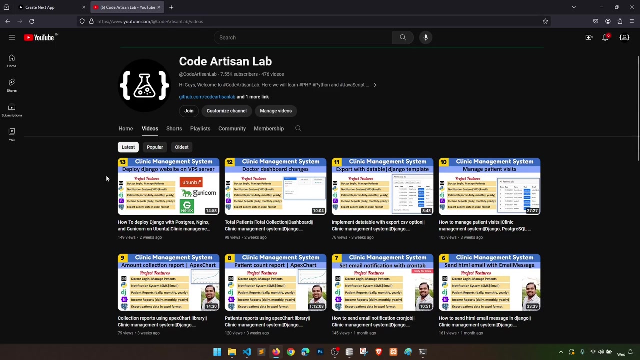 any of the project. some projects are paid right. some subscribers say that you should give it free, so some projects are free but some are paid. but you can see that tutorials- if you are actually want to learn, than tutorials videos are free. you can learn from free, but if you need the code, source code. 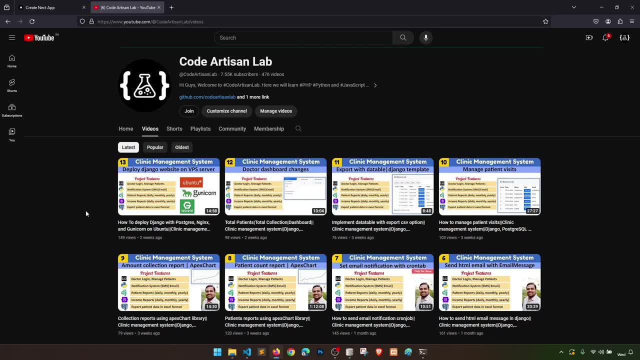 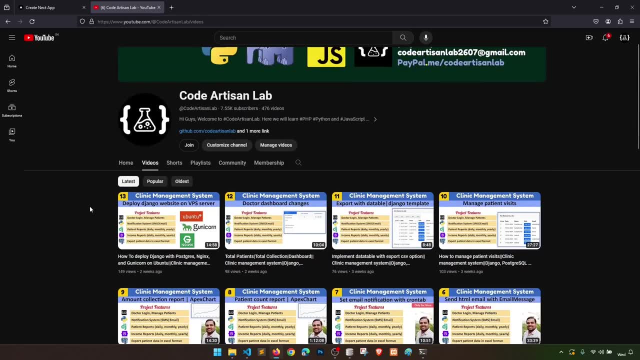 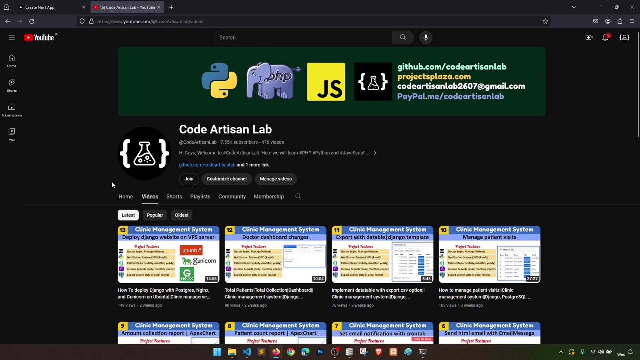 then you have to. you have to, you know, support me. or you can say: pay me some amount, okay, and then it will be, it will be good for me to run this channel smoothly, right? it will motivate me. if you support me, right, and give me projects, idea, so I will create, okay. so let's see how far we.